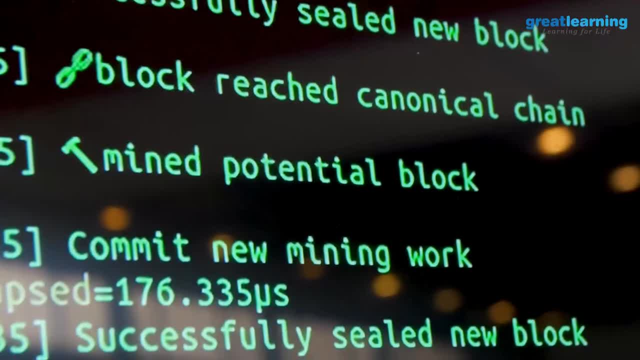 Clustering is a powerful and broadly accepted data mining technique which is used to partition huge data into different clusters, and it is the most important unsupervised learning algorithm. It deals with finding a structure in a collection of unlabeled data. Keeping the importance of 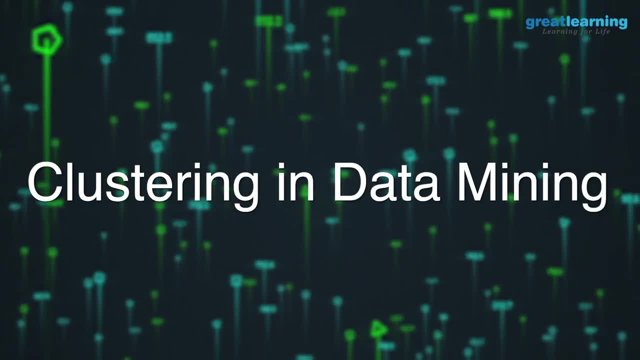 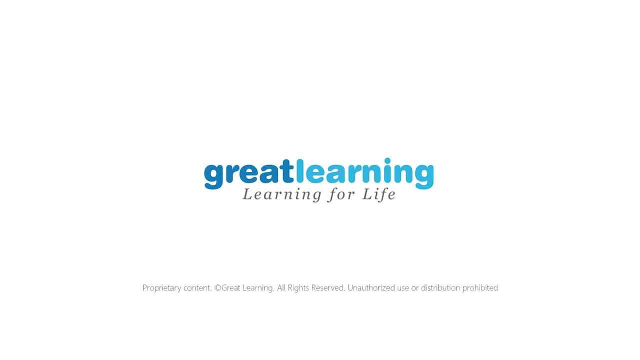 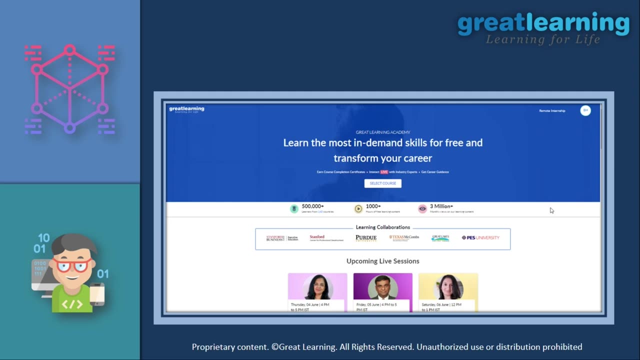 clustering in mind, we have come up with this tutorial on clustering in data mining. Now, before we go ahead with the session, I'd like to inform you folks that we have launched a completely free learning platform called as Great Learning Academy, where you have access to free courses such as AI, Cloud and 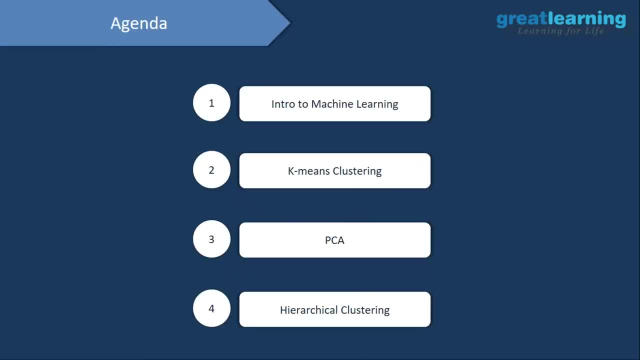 Digital Marketing. You can check the details in the description below. Now let's have a glance at the agenda. We'll start off by understanding what exactly is machine learning and then look at its categories. Then we'll dive into the concept of k-means clustering. After that we'll learn in brief about 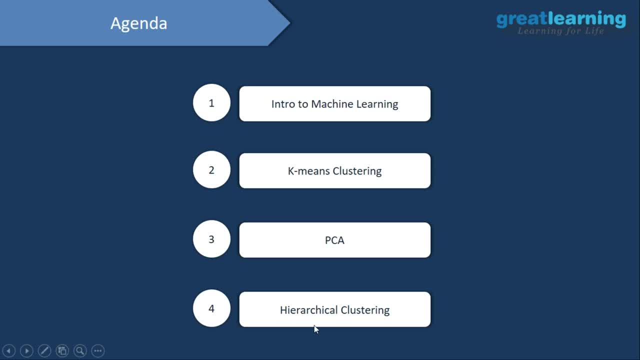 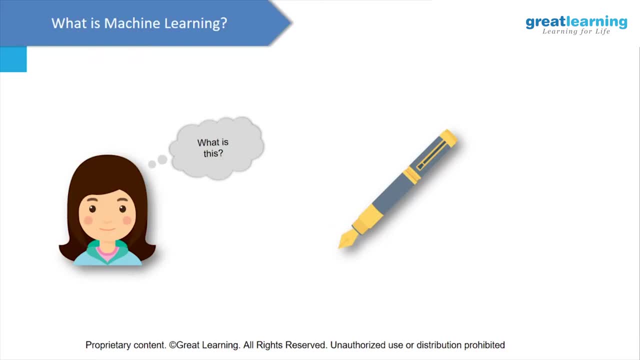 PCA and finally, we'll learn about hierarchical clustering. So let's start off with a very simple question: What exactly is machine learning To answer that? let's take this example over here. So what do you exactly see in this slide? What is this? It's a pen, isn't it? Now what is this again? Well, this is a pen. 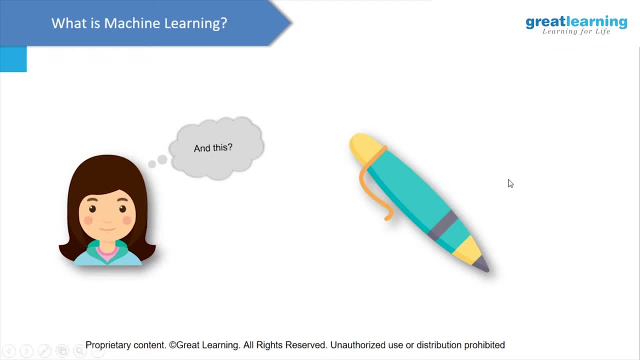 too. And what about this? Well, this, again, again, is a pen. now, how do you know? all of these are pen. you know, when you immediately saw the picture of this, your brain immediately recognized that this is a pen. how is your brain able to do this? well, this is how our brain functions. so when you are, uh, when you're, let's say, very young, let's. 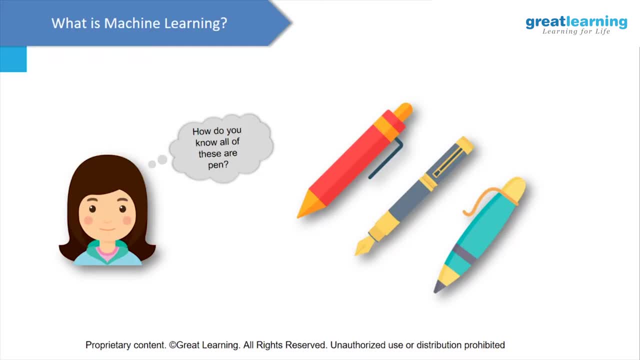 say, when you're in kindergarten, then maybe you were told by a kindergarten teacher, or maybe your parents, that this is how a pen looks like, and your brain automatically registered the features of a pen. you know, so it, your brain automatically understood how does a pen look like? so these. 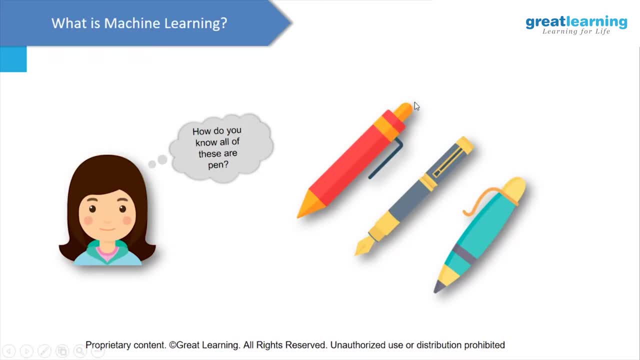 are all the features. so, basically, it understood the boundaries, the outer boundaries, of how a pen needs to look like and it immediately registered that. and whenever you would come across a picture of a pen or you would come across another pen, then you would immediately recognize that there's a pen. 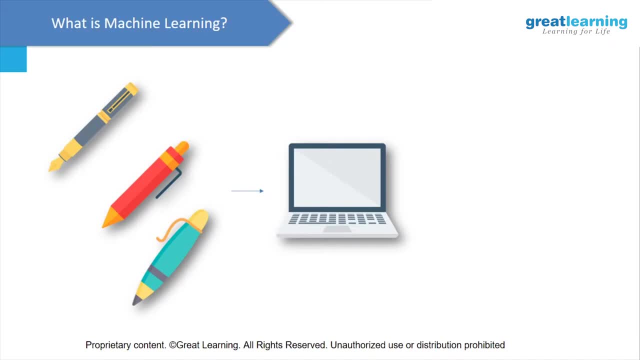 and that is how our brain functions. now, that is all. uh, you know, that is about how our human brain functions and that is why we, as humans, are intelligent. but what if i actually use these images and i feed these images to a computer? so how will a computer be able to understand that these are actually pens? 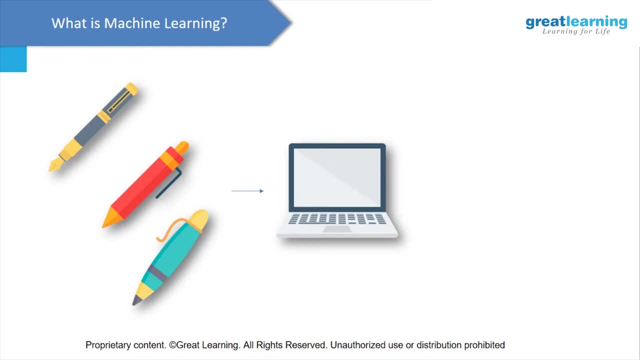 because i mean, we have a brain. but does a computer have a brain? well, it has a cpu and that is what works as a brain for it. but the question is, how will this computer recognize these images as a pen? so what we'll do is we'll implement the same procedure as our brain works. so our brain it was for. 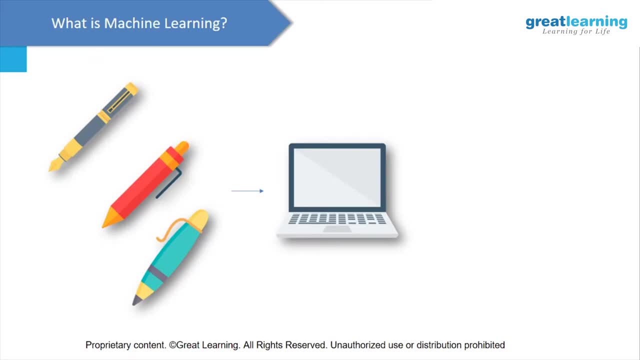 our brain. it was basically reinforced that when you looked at a pen, you were told that that is a pen and that reinforcement of the picture of the pen is what. and that is how your brain learned that whenever you- uh, whenever you see a new picture of a pen, you will immediately recognize that as a pen. 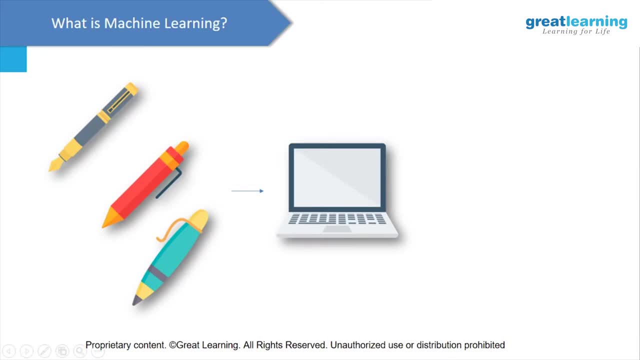 and that is what we'll be doing over here. so what we'll do is we'll take millions of pictures of pens of random shapes and sizes and or different colors. or you will take a ink pen, you will take a ball pen, you will take a gel pen, and all of them would have different colors. and what you do is 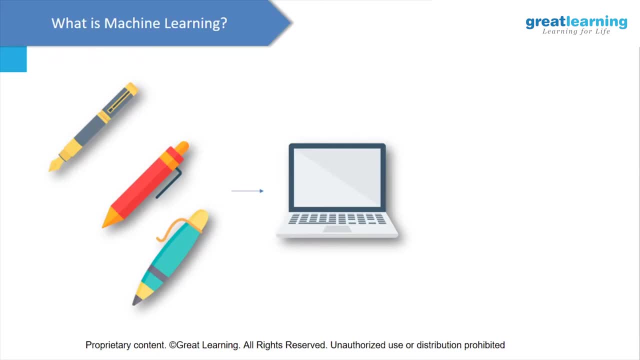 you'll just have these millions of pictures of pens and you will keep on feeding them to this machine. Now this machine learns all of the features from all of those million pictures of pens and once that is done, this is known as the training. So what we're basically doing is we are 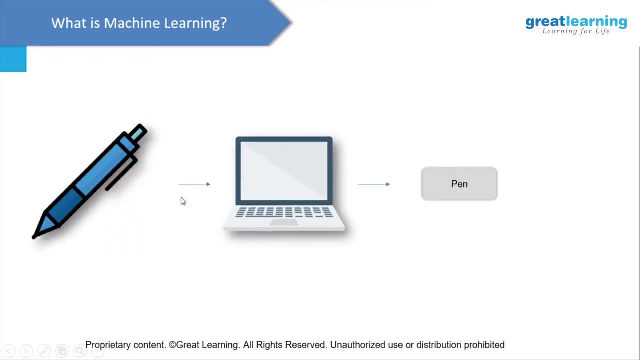 training this machine over here, and once the training is done, we'll try to understand how much the machine has actually learned. So this is what is known as this computer. Now, if this machine is able to identify this pen or label this pen as this, then so instead of let's say pen, it could. 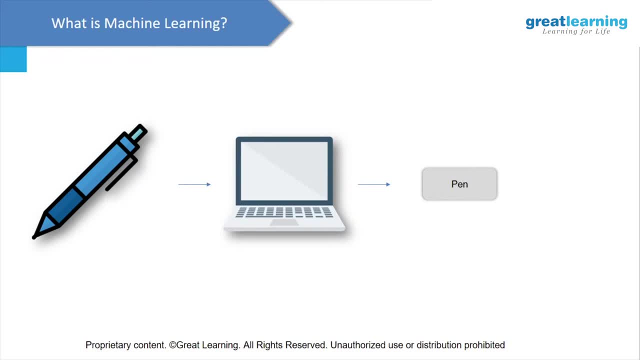 tag it as a pencil, or it could tag it as an eraser. so that is totally up on the machine, and if it, if it actually tags it as a pen, then that would mean that the machine is able to identify the pen and label it as a pencil. So this is what we're. 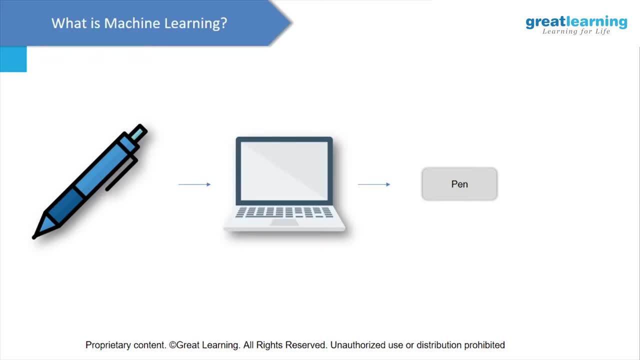 going to do So. this machine has learned that it has passed in the test, So it's training was done successfully and it has passed in the test. and this machine has learned enough that whenever I give it a new picture of a pen, it will be able to tag it or classify it as a pen. and this, my friends. 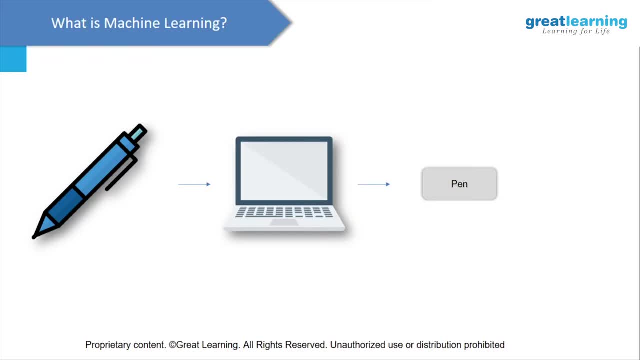 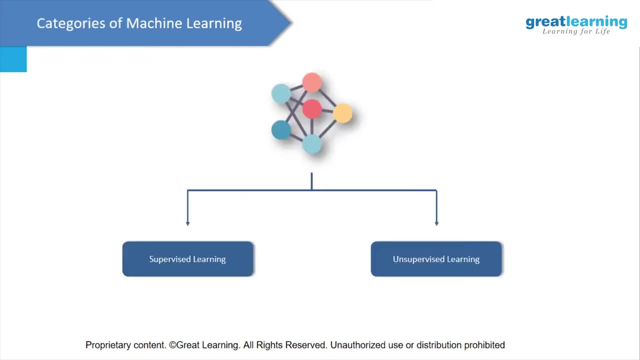 is what is known as machine learning, or this is the underlying concept of machine learning. Great, so this was the underlying concept of machine learning. Now we'll go ahead and understand the different categories which are present in machine learning. So let's start with machine learning. So normally we have supervised learning, unsupervised learning, and there's also 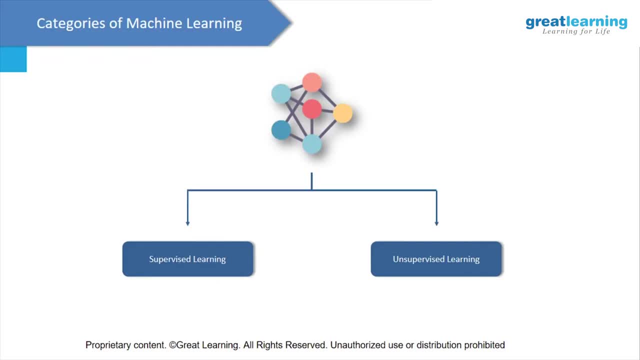 another category called as reinforcement learning. So reinforcement learning is mostly covered with respect to deep learning topics, so that will not touch upon today. and then today's class will mostly focus on supervised learning and unsupervised learning, which are the primary categories of machine learning, if I may say so. So first let's start off by understanding what exactly is. 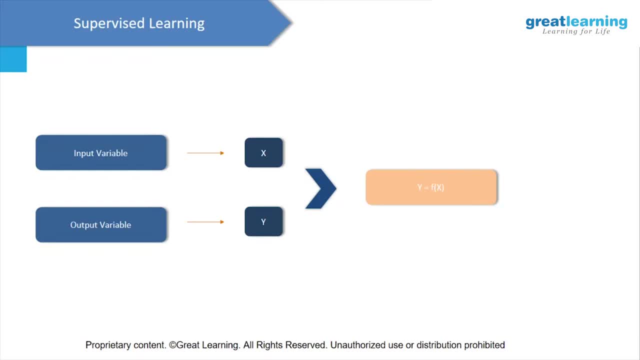 supervised learning. So in supervised learning we obviously are dealing with data, but this data is divided into input variables and output variables. So the input variable is denoted with x and the output variable is denoted with y, and what you're basically doing over here is: 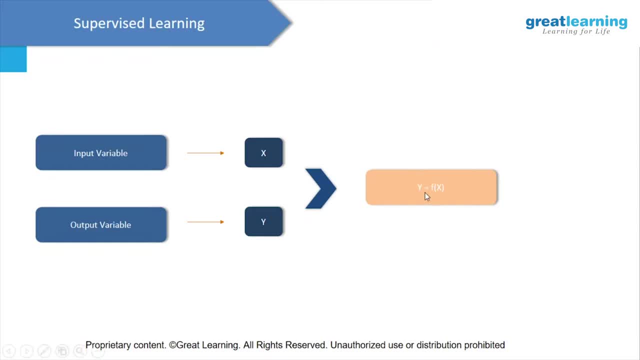 you're trying to understand the relationship between x and y. So here y would be your dependent variable and x is your independent variable. or in other words, you're trying to understand how does y change? So that is why, when you say how does y change with x over, here y is basically dependent on x. 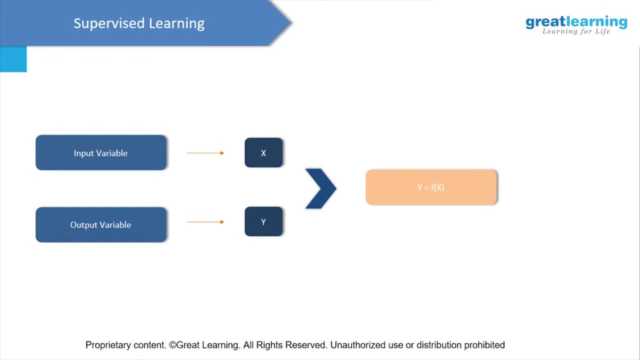 and that is why y is known as the dependent variable and x is known as the independent variable. and in supervised learning, you basically have data which is labeled. So, as in the previous example, we saw that we had image of a pen and we had a label with the tag pen. So over here. 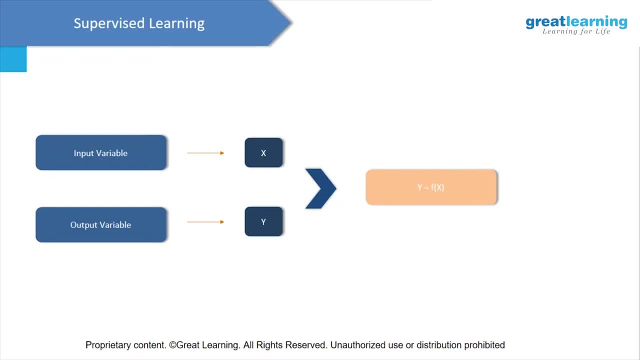 the image would be the image of a pen and the image of a pen would be the image of a pen. So over here the image would be the independent variable and the tag would be the dependent variable. So let's say, if I give you random images over here, So let's say if I have maybe an image. 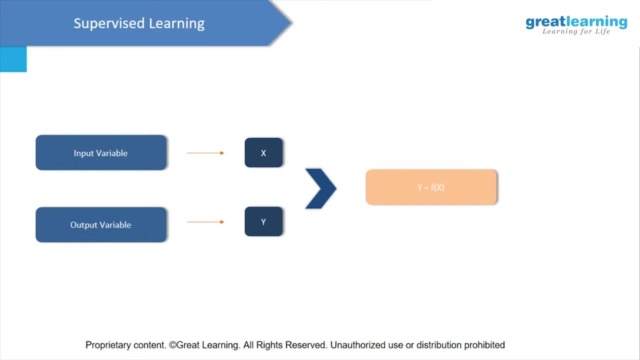 of a car, an image of a pen and an image of a laptop. and I have three different tags. and let's say I feed these three images randomly to the computer and then randomly I'll also feed the tags: car, laptop and pen. Now, if the machine has learned enough or it has been trained enough, 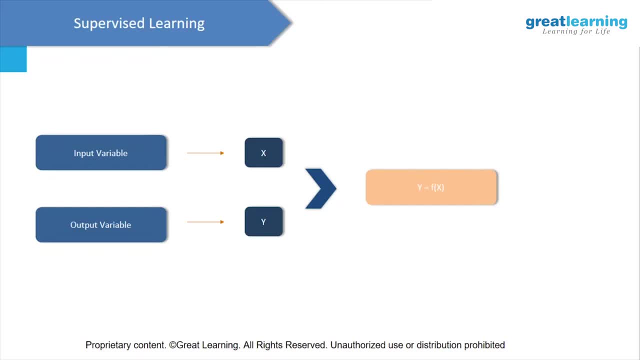 then it should be able to do the same thing. So let's say, I feed these three images to the computer and then, randomly, I'll also feed the tags car, laptop and pen. Now, then the machine is able to currently tag all of these images with the right labels. So this is how supervised learning works. 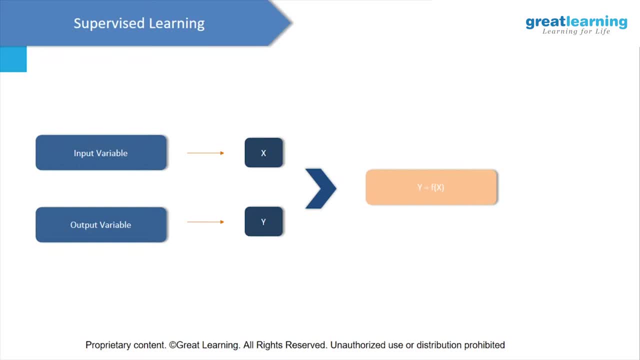 You have independent variables and you have dependent variables and you try to add the right label or you try to find out the relationship between the dependent variable and the independent variable. So that was supervised learning and then supervised learning. we have something around regression and classification. 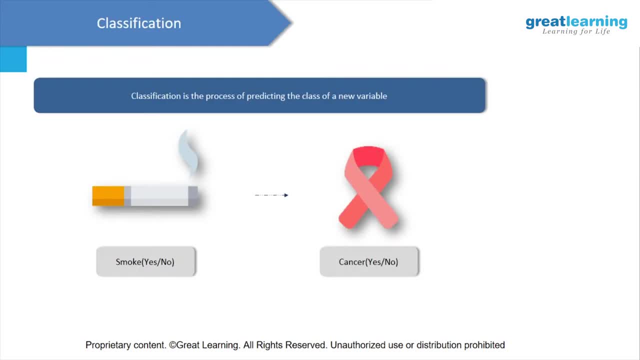 two, let's start off with classification. so classification is basically the process of predicting the class of a new variable. it's very simple. so again, let's take this example over here. so, as you see, we have an independent variable and dependent variable over here. so here the problem statement is: if a person smokes, 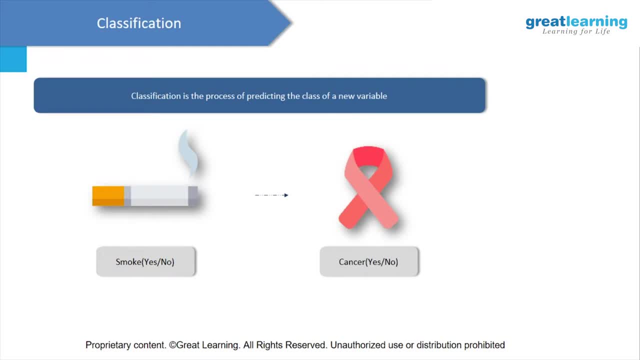 then what is the probability? or will the person have cancer? so this is the problem statement which you are trying to solve. so here our independent variable would become whether the person smokes or not. so this is our independent variable, and the dependent variable over here is whether the person has cancer or not. so, on the basis of whether the person 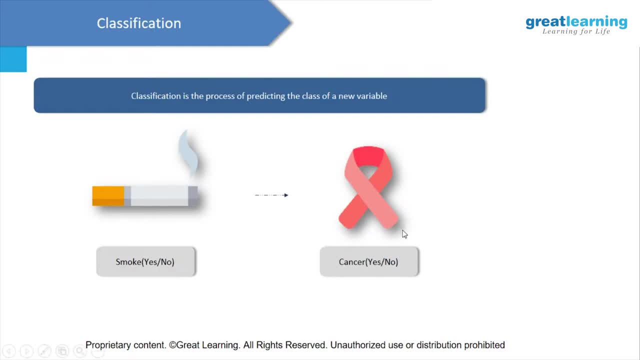 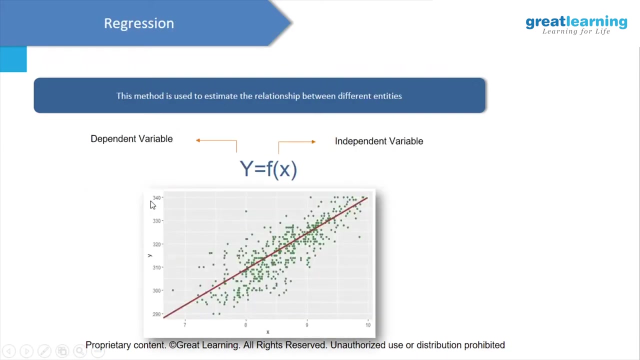 smokes or not. I am trying to provide the tag whether the person has cancer or not, and this is what is known as classification, or this is what happens under classification process. so, as you see, we have labels and we also have input data. that was classification and then we have something as regression. so also, I'd like to point out that 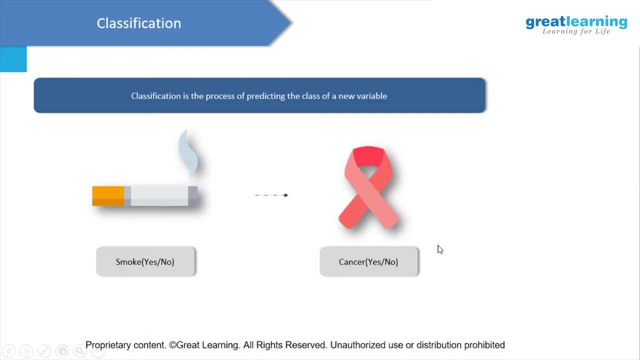 when it comes to classification, your dependent variable should be categorical in nature. so what do I mean when I say it has to be categorical in nature? so categorical is basically: you have different levels, you have different categories. so this was a dependent variable and, as you see, this is a categorical variable. so over here, the categories are yes or no. so yes, the patient has. 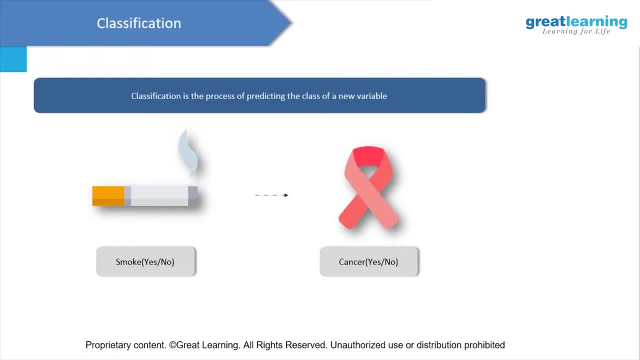 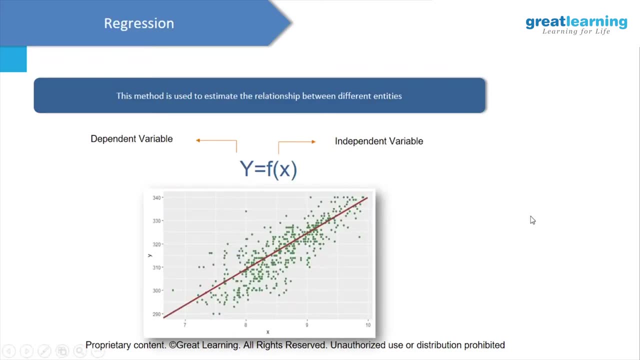 cancer or no, the patient does not have cancer, so this is where we'll go ahead and use classification machine learning algorithms. now, on the other hand, if our dependent variable is actually a continuous numerical, so that is where we will use regression methods instead of classification methods. so here, 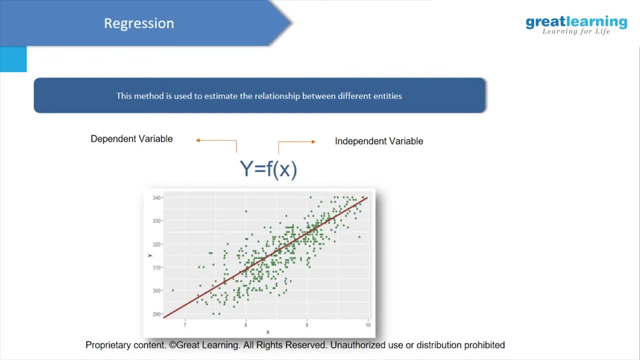 let's say, a perfect example could be: if you're trying to understand if there's a relationship between the age of a person and the salary of a person, so here the salary of a person would be the dependent variable. so let's say: over here y is the salary of the person and x over here is the. 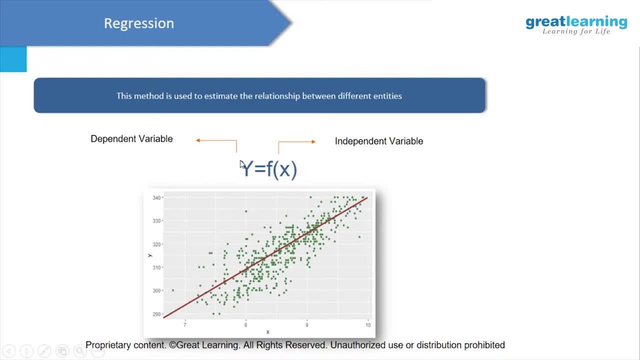 age of the person and we are trying to understand how is or how does the salary of the person vary with respect to the age of the person. so here let's say, if this is the result over here, then this tells us that there is sort of a linear relationship between the age and the salary. 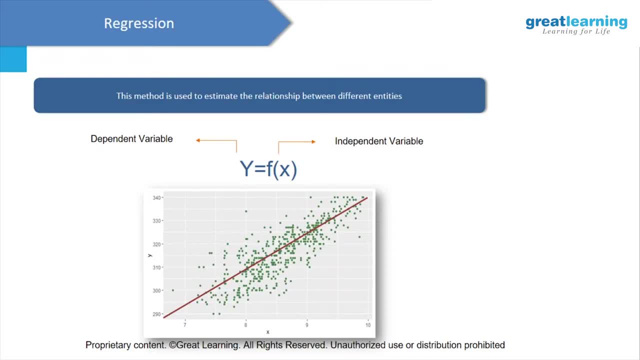 or in other words, if the age of the person increases, the salary of the person would also vary. so here, since the dependent variable salary salary is numerical in nature, that is why we'll use regression methods and for this particular problem statement, the regression method which we'll be 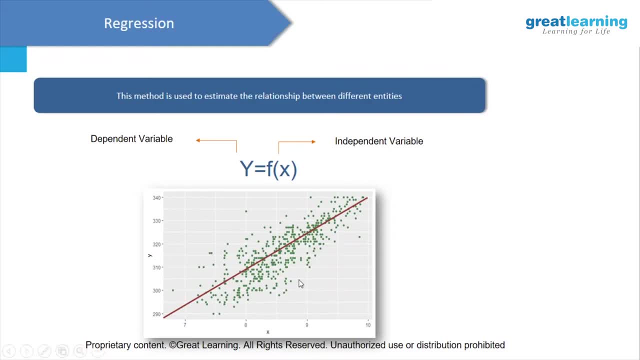 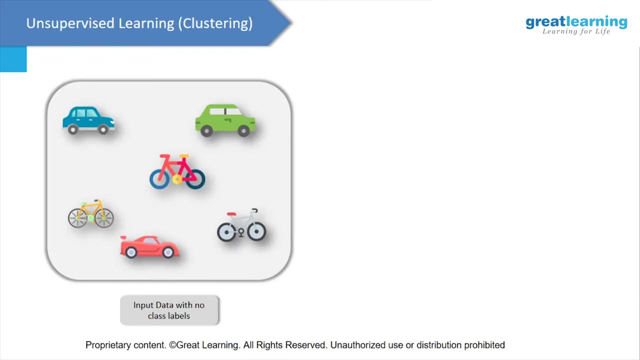 using is linear regression and, as you see, we have a linear line over here which gives us the relationship, or the linear relationship between salary and age. that was classification and regression. so now that we are done with this, let's go ahead and understand what exactly is unsupervised. 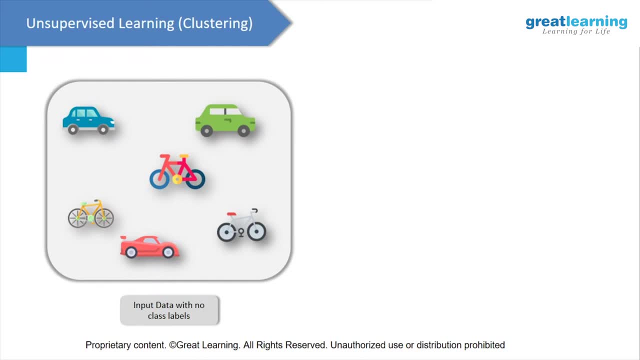 learning. so till now, the base of unsupervised learning is we had labels associated with the data, right? i hope everyone is clear with that. and now the base of unsupervised learning is you have data with no class labels. so let's say, if i have all of this data over here where i have images of different cars and images of different 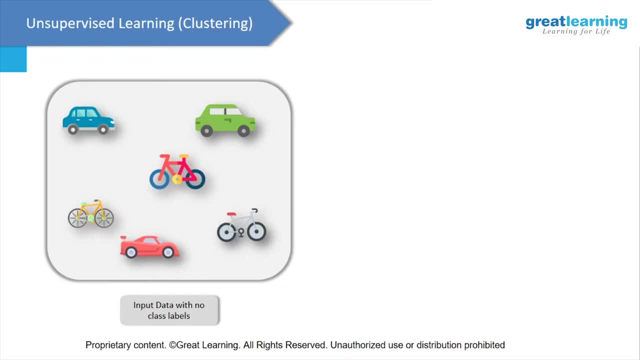 cycles. but if i feed this to a computer without labels, right, i'll not have any labels over there and i'll just randomly feed in the data. and i'll just randomly feed in the data and i'll just randomly feed in the images. so how can a computer understand which is actually what? so this is where 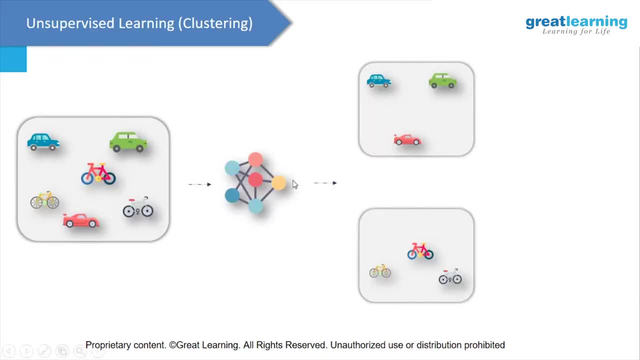 a clustering algorithm comes in. so here what we're doing is we are applying a clustering algorithm on top of this unlabeled data, and this clustering algorithm gives us two groups. now we have got these two groups even though there are no labels. we've got these groups because this has been done. 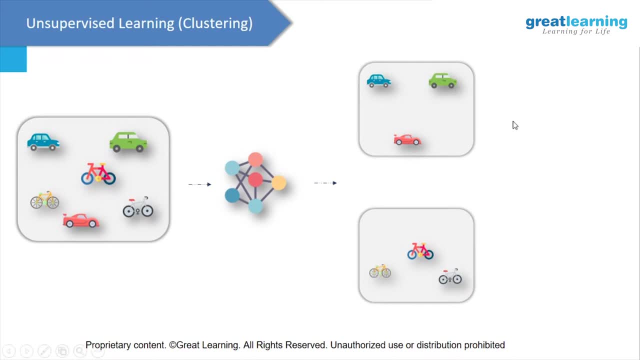 on the basis of similarity of the properties. so here you'd have to keep in mind two things. so the first part is high intra-cluster similarity and the second part is high inter-cluster dissimilarity. now let's understand the first thing where i'm talking about high intra-cluster similarity. so here, when you look at the data, 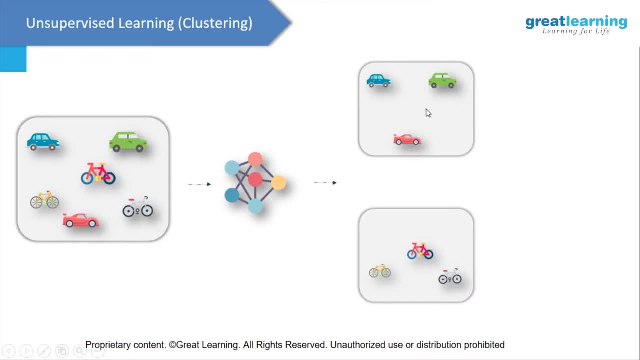 points which are present in this group, right. so all of these data points are very similar, aren't because all of them are cars. now, this is what is known as high intra-cluster similarity, because all of the data points are very same, but similarly, if you look at this particular group over here, 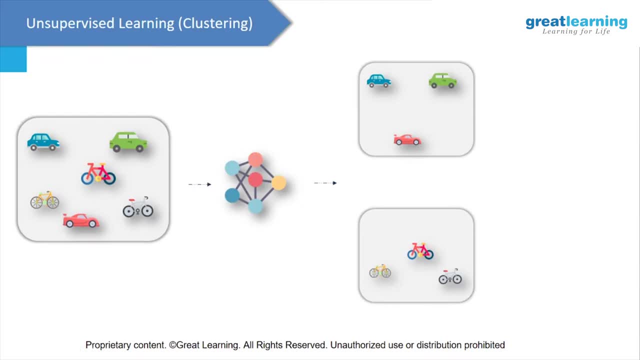 here again, all of the data points are very similar to each other because all of them are bicycles, and that is why there is high intra-cluster similarity over here as well. but when we compare these two groups- so let's say when i compare group one with group two- there is high inter-cluster. 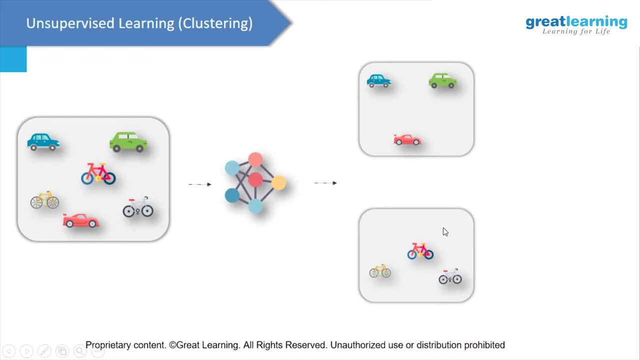 dissimilarity, isn't it because you have cars over there and you have bicycles over there and obviously both of them are very dissimilar when you compare them to each other. And this is the high inter-cluster dissimilarity which I'm talking about. 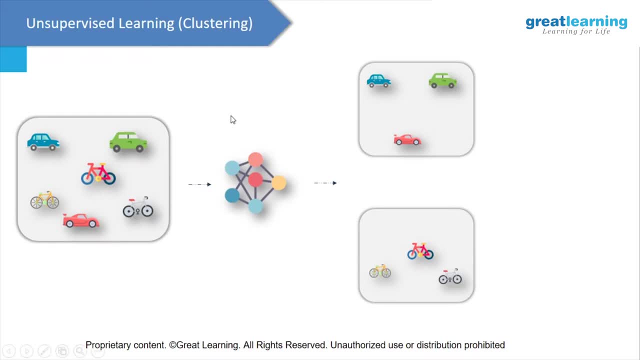 So when you apply a clustering algorithm, which is basically an unsupervised algorithm, on top of this unlabeled data, you are getting these two groups, because this data in the first group is very similar to each other and this data in the second group. 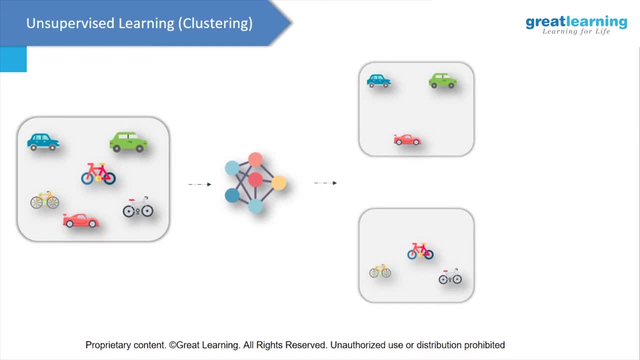 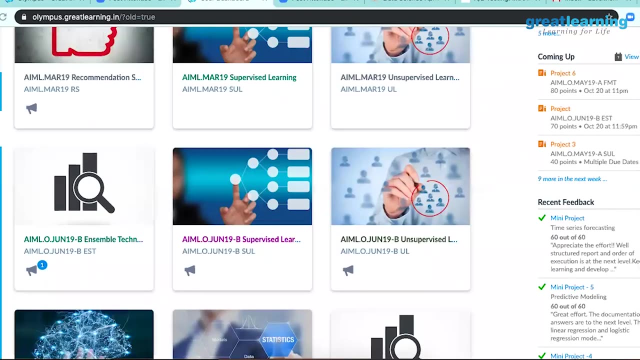 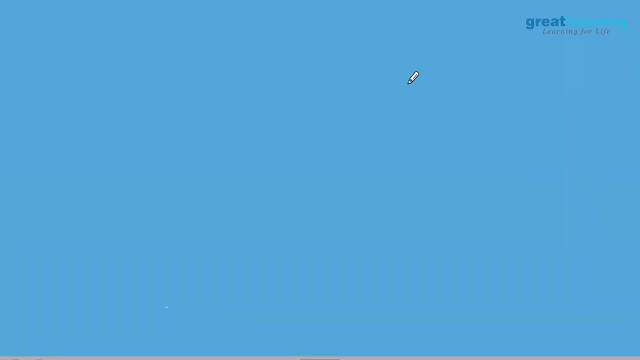 is very similar to each other, Right, I hope everyone is clear with this. So now moving on for our unsupervised learning. So last time I think I gave you guys an intro about what is unsupervised, what are different techniques we have in unsupervised. 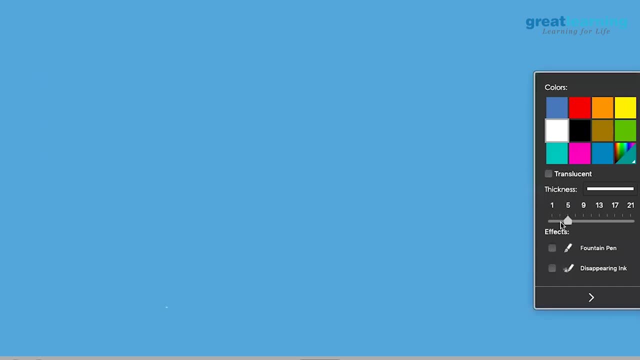 So just to brief it up what we did last time very quickly, I'll not take much time. So the only line of difference between supervised and unsupervised will be the target column. So once the target column goes missing or once in a data set, even if the target column is there, 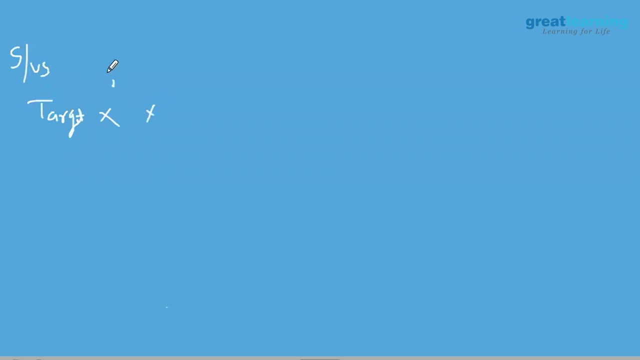 and you believe you don't want it. you can use unsupervised learning. I'll give you both the examples. So let us say in your banking data set that you have currently okay, Or it's okay fine, forget banking data set. 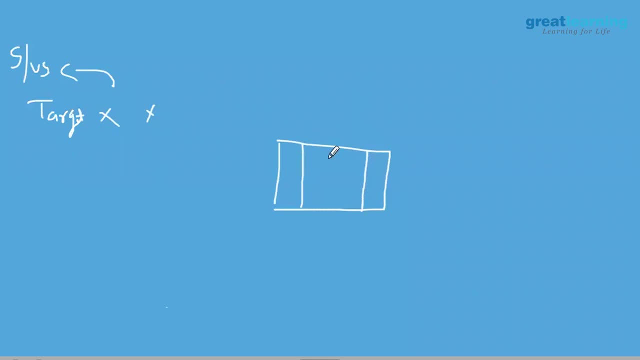 Let us say we are having a data set where there are some features given to us. So it's an animal data set And there are some features given to us saying that if the animal has got two, three, four, five, two ears, let us say one tail and he's furry. 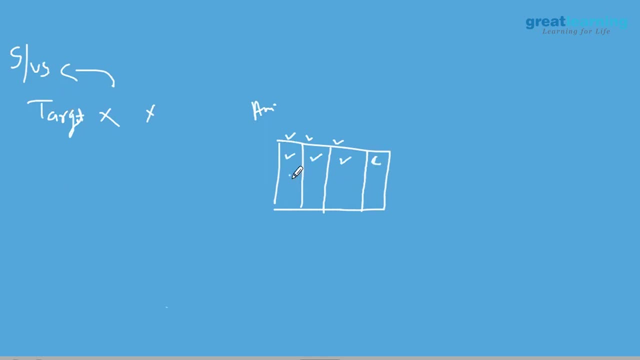 I can say it's a cat, for example, Or else, if the animal is having certain attributes, it's a dog, just an example In this. so this is your target variable In this particular data set. we are not sure. 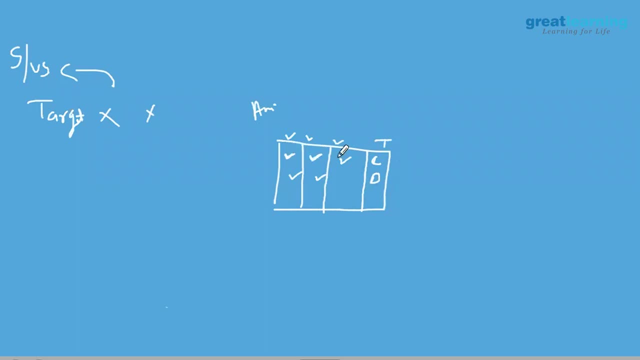 because, see, a dog can also have two ears, four legs, and they are furry and a tail. We are not sure about how authentic this data is, So if, in case, you are not trusting the target variable, you can ignore it And you can take this through unsupervised learning technique. 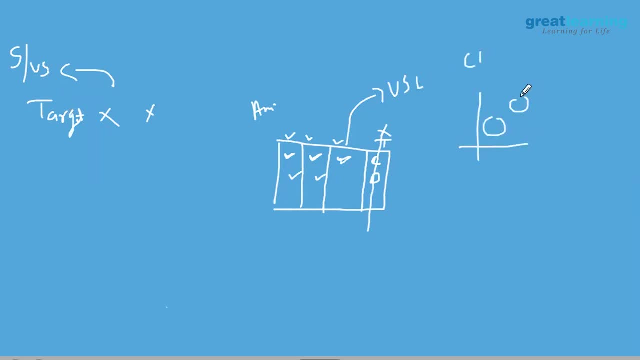 like clustering to build our own cluster. So once we have got our clusters, we can name the cluster: either zero, either one, either two. And we can understand on the backend, saying that zero will be dog, one will be cat, two will be, let us say, rabbit, for example. 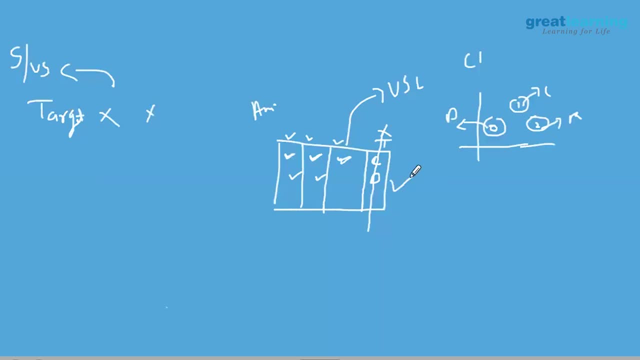 So this is one worst case where you can go ahead. Else, if your data originally does not have a target, you can create a target variable. yeah, What you can do is you can create a target variable using our clustering technique or some other techniques. 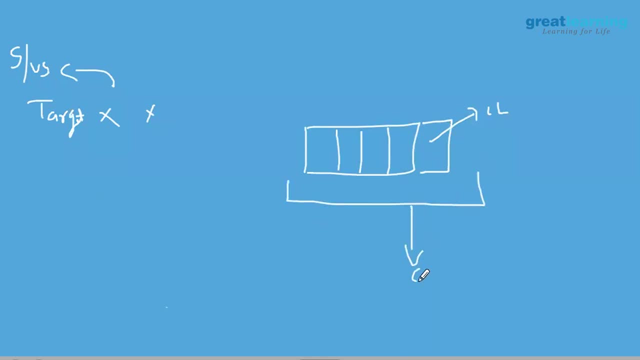 And once the target variable is created, you can push this data to supervised learning techniques. Okay, so you can do anything you want. Sometimes people stop at clustering. They create clusters and they stop Nothing. to do nothing, to worry, like it's a good thing. 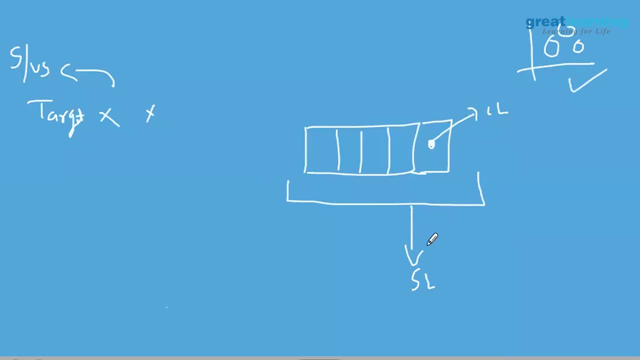 But if you want to do machine learning on that, do not stop, move on, push it onto ensemble techniques. Why? Because you already have no targets, So we can make a good prediction model. Sometimes I have seen people going on Google and reading blogs. 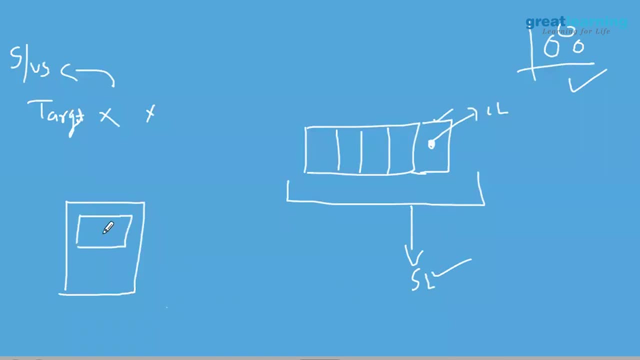 The blog, the people who's writing those blogs. they are very focused only on unsupervised learning, So sometimes this information is a little messy, So please try to think in this way, saying that you should not stop here. There are 100 possibilities, even beyond that. 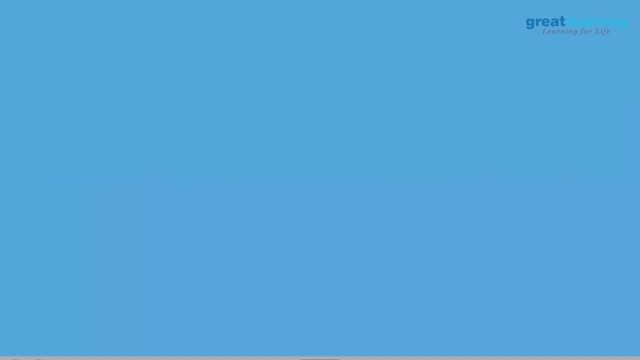 Okay, so this is one thing. Now, under unsupervised learning, there are many techniques. So the first and the most simplest technique that we are going to see is clustering, Post-clustering, a hybrid of clustering. we are going to see what is hierarchical clustering. 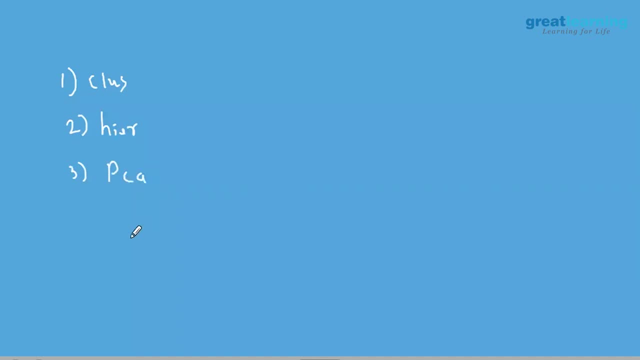 After that we are going to see a technique called principal component analysis. So this is, I think, what is covered in your course. Something extra from my side: I will show you guys factor analysis plus. I will show you another technique called SVD. 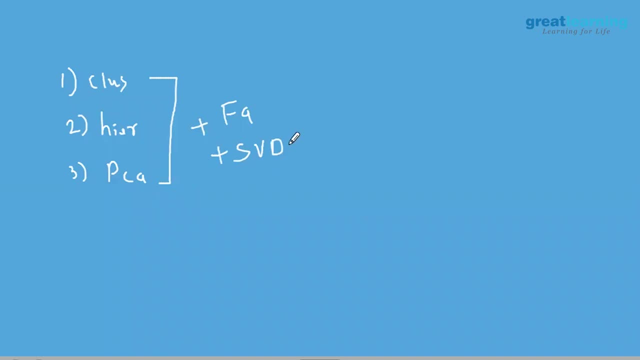 singular value decomposition. Yeah, so this one. anyway, it's going to come under recommendation system module after two or three modules. but it's okay, Why do wait? I will show you this also. So I'll show you all the case studies one by one. 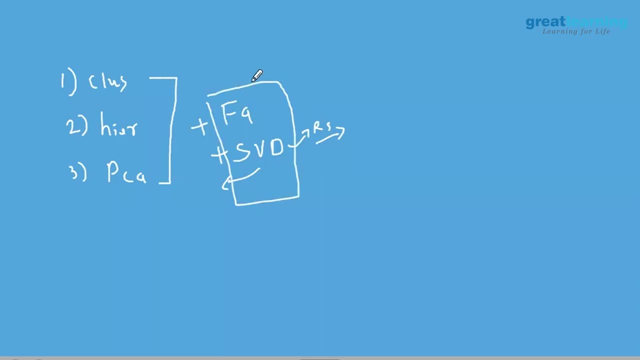 Okay, so I think we will do these two once our project week is on, so that we don't waste much time now, And these one we are going to cover one by one. So I think last time we did clustering, So everybody remembers clustering. 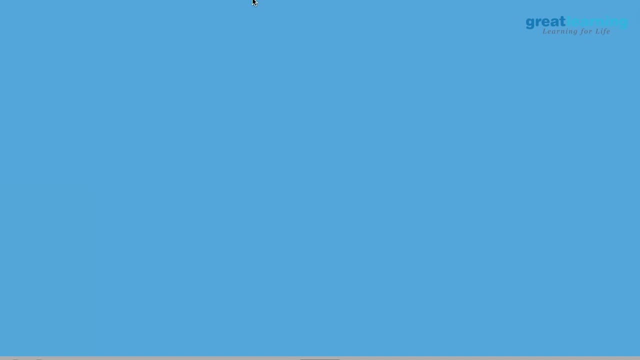 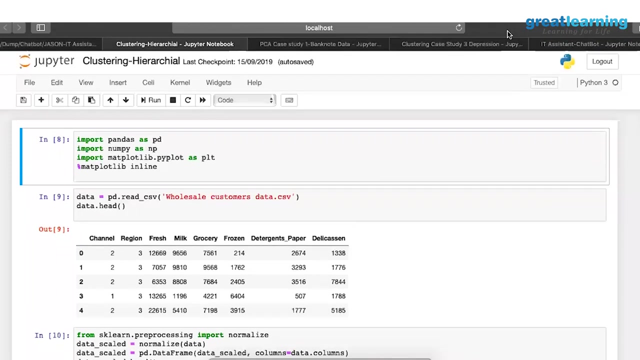 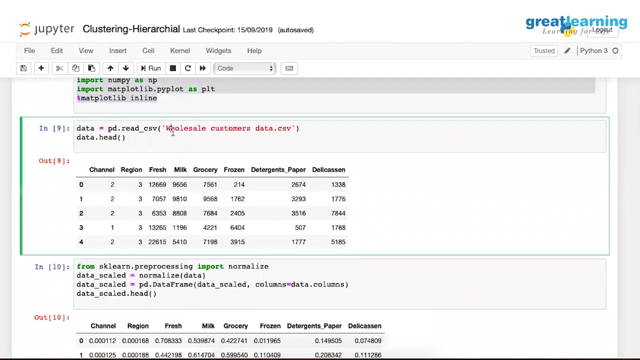 or do you want me to repeat once again quickly? We remember that, Remember, Okay, So let's move on directly to the data set now. So yeah, So as usual, these are our libraries that we are having, And what do we have here is we have got. 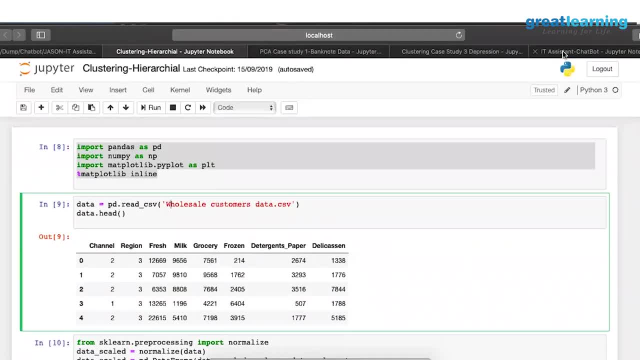 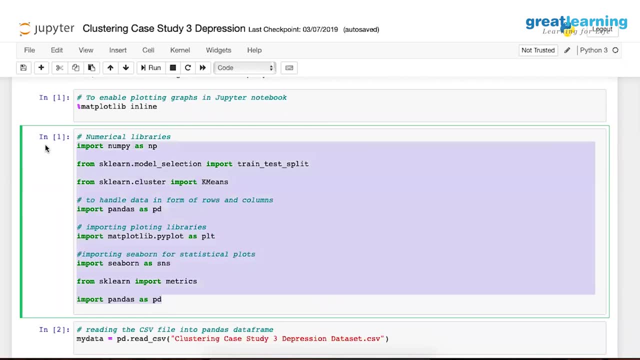 give me one minute, guys. This is hierarchical clustering. Yeah, this is what we're talking about. Okay, so this is my standard libraries that I'm going to import. One very frank question to all of you. We are comfortable with libraries and Python right now. 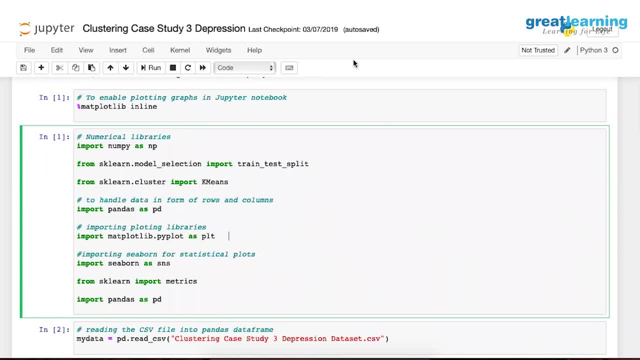 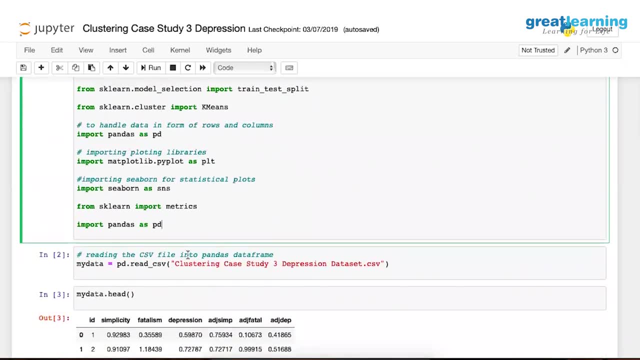 At least all of us. Yeah, Yeah, Okay, good, perfect, So if, in case, you want me to explain something, please stop me. nothing wrong with that. So these are my standard libraries. Next, what I'm doing is I have a data set with me today. 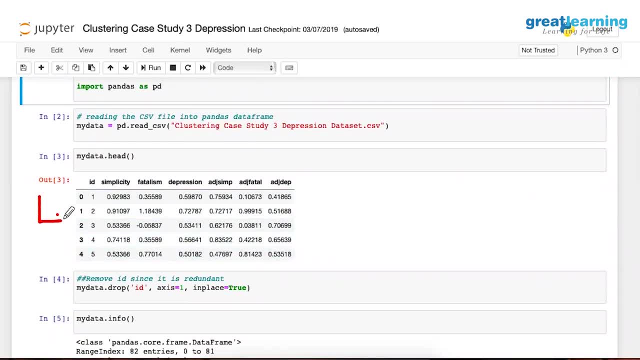 Where in This data set is coming from. I think one of the research is done on to some depression depressed patients or basically some patients, And then they are trying to, you know, trying to find out certain matrices within psychiatry on depression. 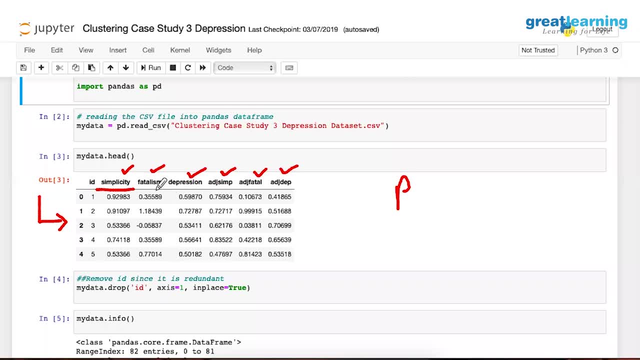 So let us say: this is a value called simplicity, fatalism, depression, adjusted, adjusted. So there are some values given to us and there is no target value. So now we want to classify whether the customer- sorry, the patients, they are into low depressions. 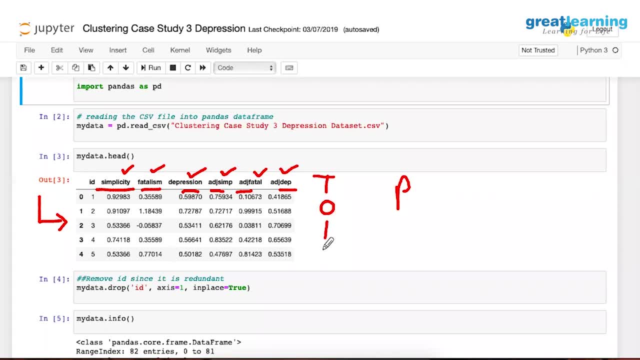 sorry, no depression state or high depression state, something like that. Or if you have one more, let us say we say K is equal to 0.. K is equal to three. That means you want three clusters. We can have extreme depression. 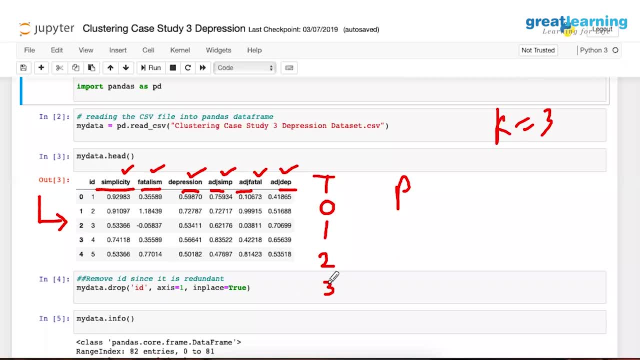 If you have one more, we can have no point of return depression or something else. If, in case, we have K is four, we can go ahead with a classification like this. Yeah, so the first thing which triggers that this is an unsupervised learning problem. 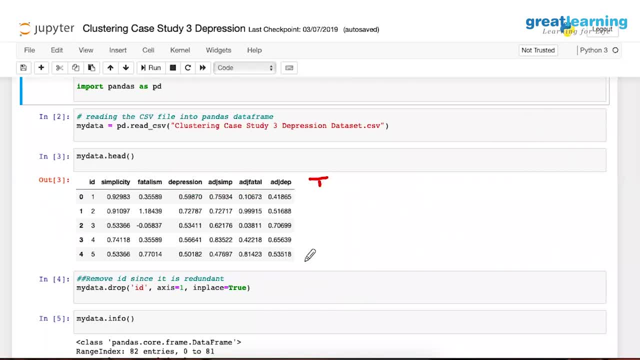 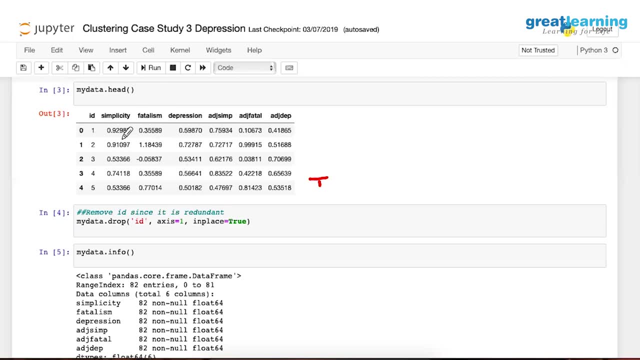 is because of absence of target variable. as simple as that. okay, Good, so this is my data set. This is my business problem. So these guys want to automate this particular report, saying that when the the computer generates this, along with this computer also should generate me a trigger. 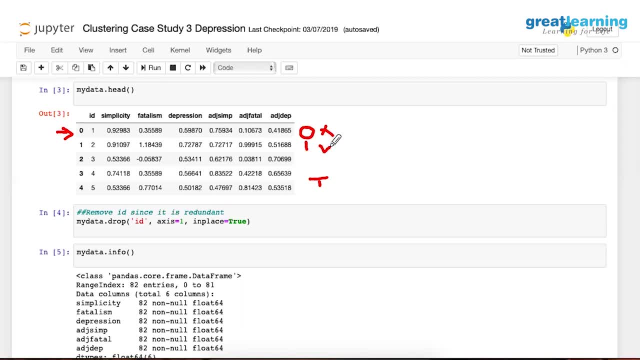 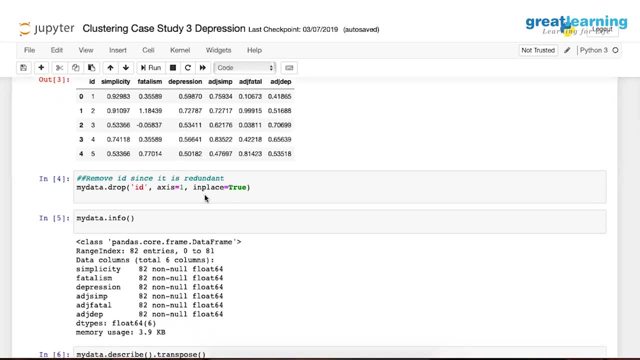 saying that this is no depression or this is yes depression, something like that. This is my total business problem. So what we'll do is we'll okay. So the first thing which we don't need here is our ID. It's of no use to me. 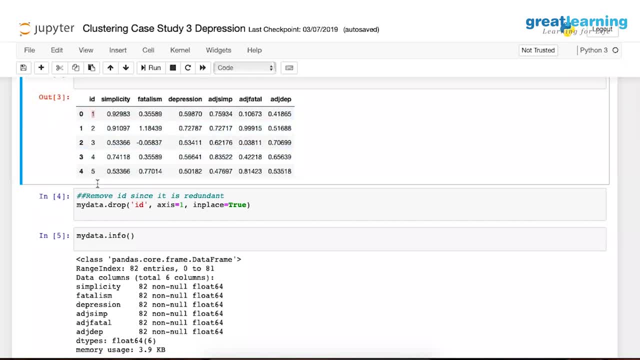 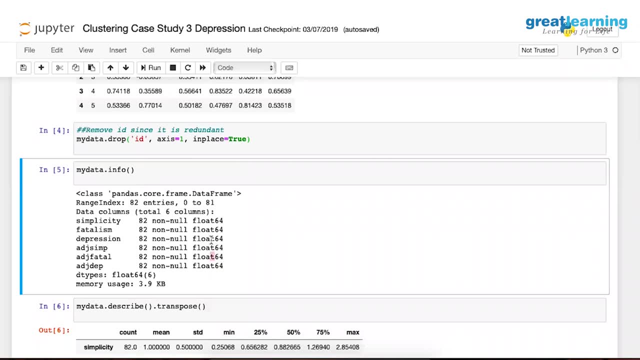 This has nothing to do with our output. So the first thing we are gonna remove is our IDs, So I'm just dropping it. Next, just have a look at the info. So everything should be in numbers. Please be careful. We do not need any non-number or non-numeric data. 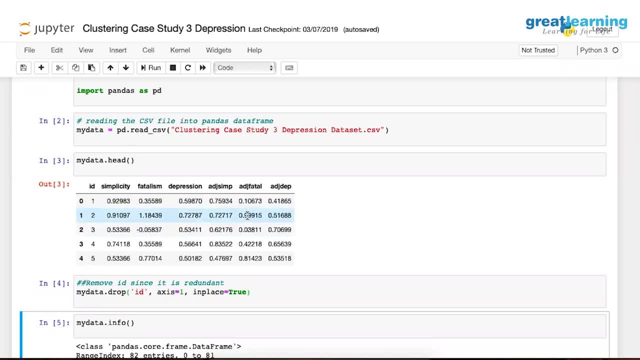 If you have a non-numeric data, you have multiple techniques to convert categories to what is in numbers. So we have dot dummies function or we have transfer transfer one hot encoding- or we have got transform function. anything you can use and do it. 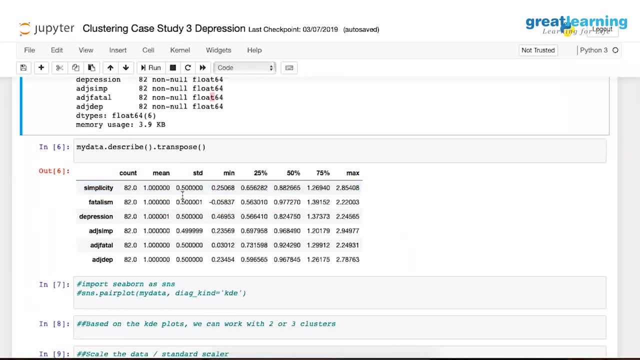 Post that. if you look at the means, so if you look at the standard deviation and mean again, the problem with clustering is if, in case, you have a data which is highly clustered, that means it is compact enough, like this. So if you want to create many clusters here, it is possible. 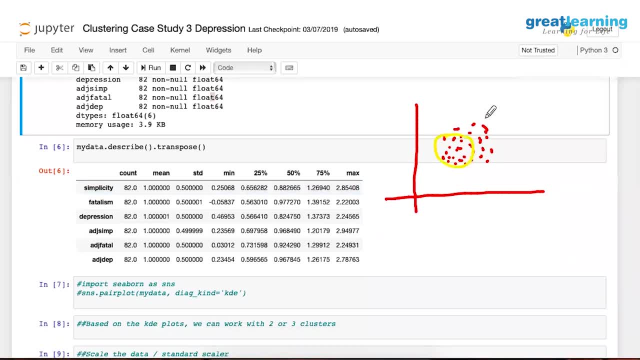 Definitely we'll get clusters out of this. nothing wrong, but please be careful. There will be a lot of points on the boundaries like this. Yeah, so our first job is to find out whether the data is tightly packed or sparsely packed. 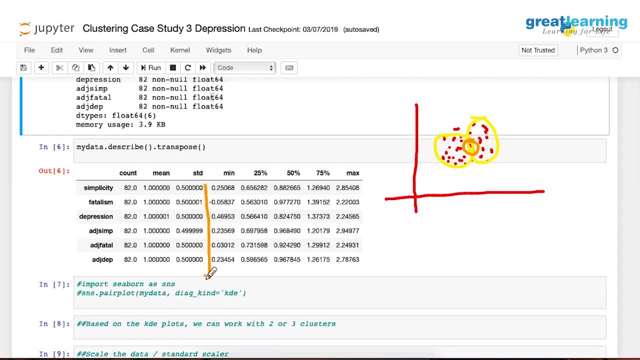 Okay. so the first thing: we can either check it from this or we can check it from the mean, So you can combine both. As per mean, this data will be tightly packed, just in case if I put everything together onto one platform. 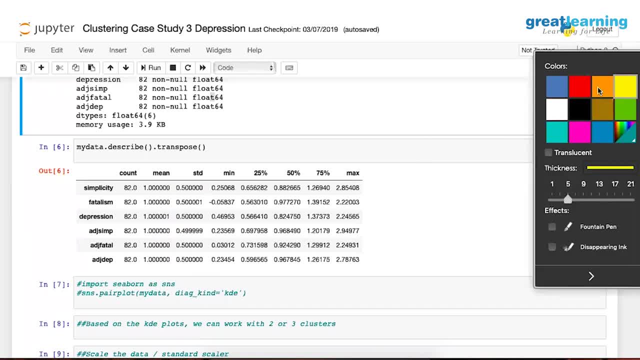 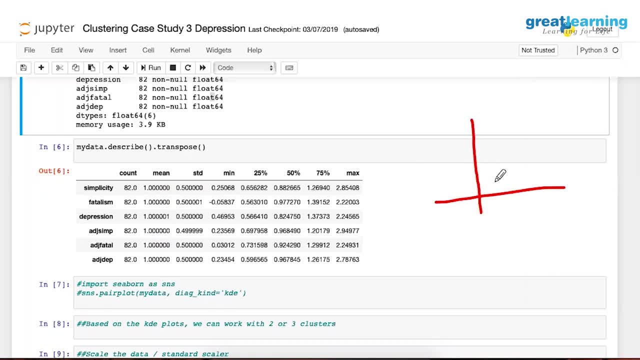 You guys can observe that. Why? Because if you look at the standard deviation, the standard deviation is almost similar, And if you look at the mean, the mean is also almost similar. Now, that does not mean that we'll not have extreme points. 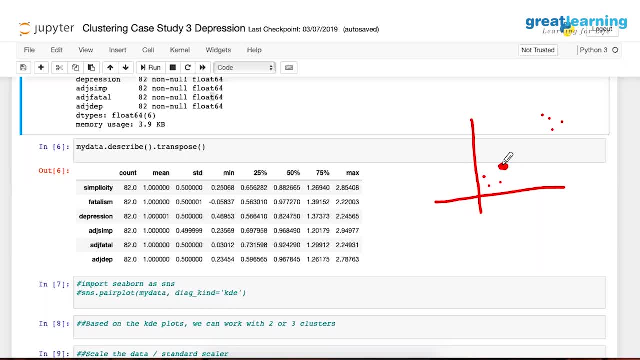 Definitely we'll have extreme points, But some of almost all the means are clustered here and almost all of their standard deviation, let us say, is this: So we might have extreme points this way, something like this: Yeah, So that is the reason. 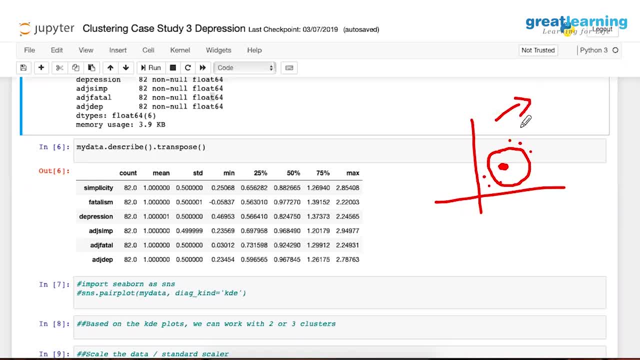 the first thing that we are supposed to do in any unsupervised learning technique- all the unsupervised learning techniques- is to normalize the data, or to scale the data, or to regularize the data. Any of the three means the same thing. 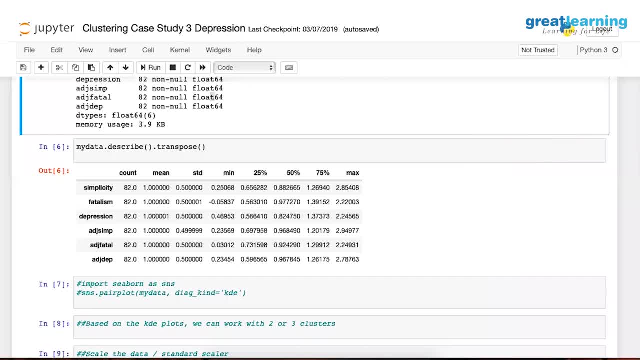 Okay, I hope everybody's good. We're the scaling part of it, the basics. Okay, Nice, we know the scaling right: Raju Jyoti, Nitesh Ramesh. What is normalization? and Yeah, maybe you can. 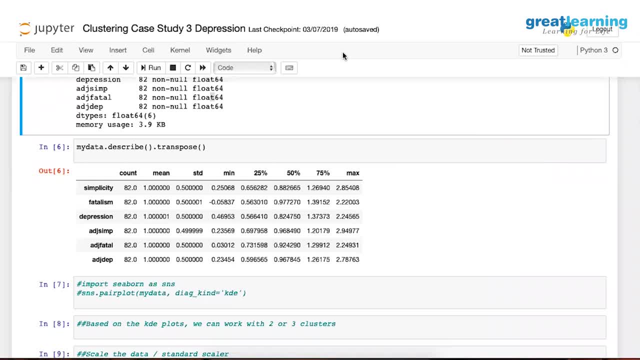 Yeah, yeah, that's a Z-score right, Putting the Z-score in, Exactly the Z-score, yes, Yeah. So on web you might find certain bloggers who are saying: we regularize the data. Some of them will say: we normalize the data. 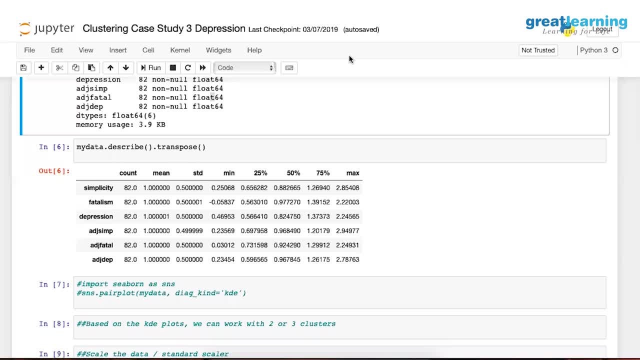 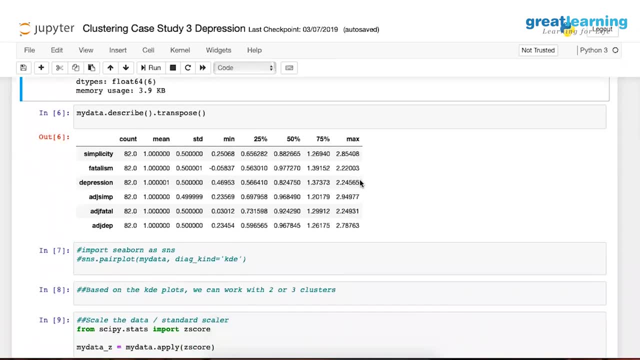 And some of them will be very down towards saying: we scale the data, So all three mean the same thing, okay, So I don't think we have not done like. we don't know what is regularization, So get a better result right. 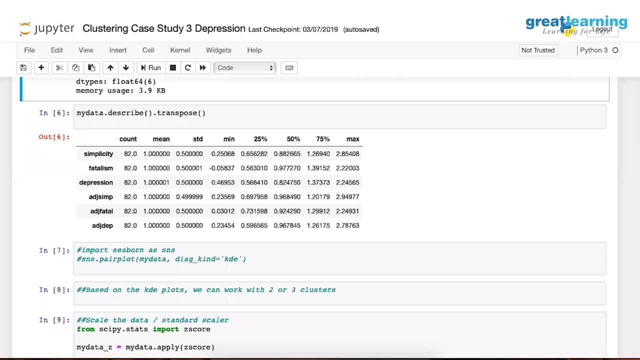 Sorry. So this scaling is to get a better result, Exactly So I will say: not get a better result, but I will say that. how do you say that? For example, let us say you have got, let us say you have got three kids, for example. 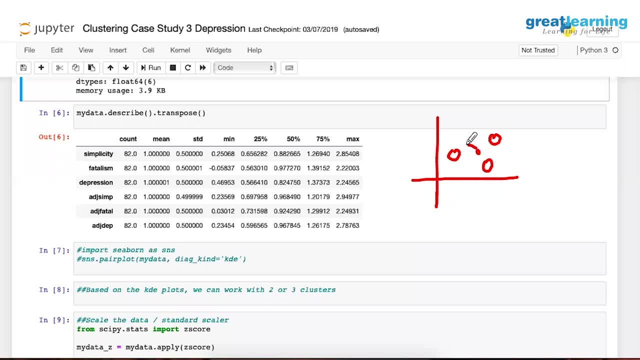 and you are babysitting these three kids. Now there are chances that when you're focusing on one of them, the other one might, you know, move out. When you focus on this one, this might move out, something like that. 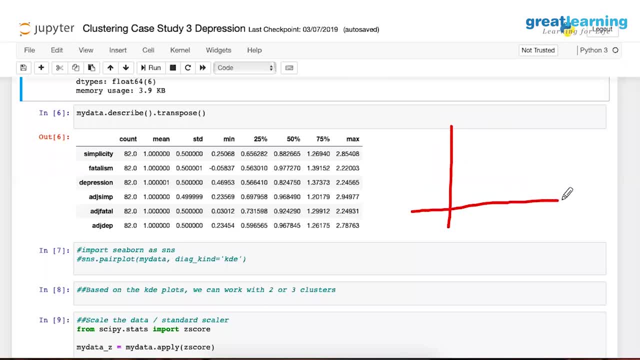 So here just to take care of the situation, what do we do? is we first of all put a center point? We say that our data point will come to center, So not all the data is a center oriented. If you plot this data set, it looks something like this: 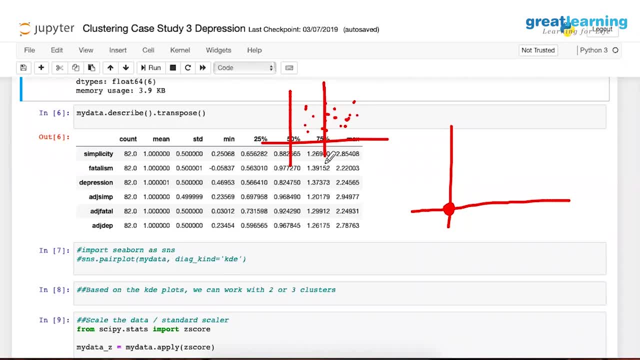 So when we do normalize the data, what we do is, first of all, we bring the scale here, We put the center here, so that we are sitting exactly on the center, And then what we do is we put a barrier against the points. 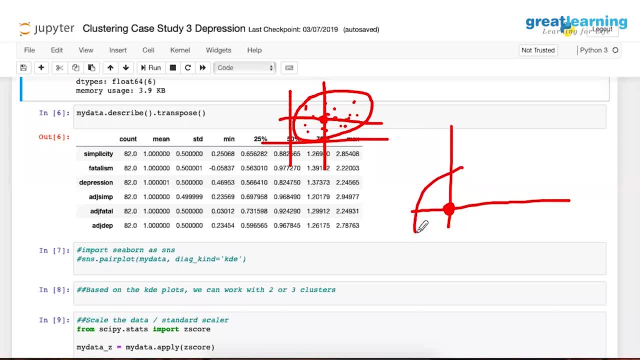 Saying that everybody, come closer, don't cross this barrier, basically. So this is what we do. So now we are assured that no data point is going beyond this. yeah, This is why we do our normalization. If you want more examples today, 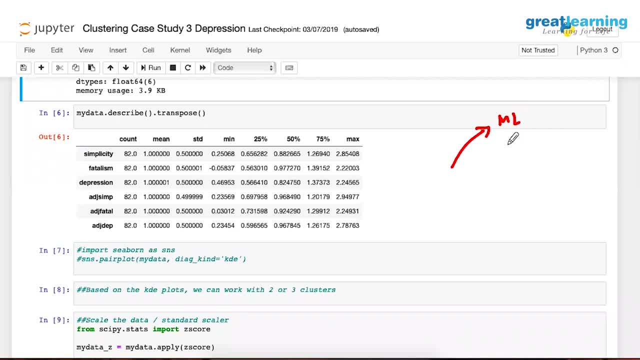 I will show you why we need normalization, Why we need normalization for ML, why we need normalization for AI, why we need normalization for image processing. We'll take it up at the end of the session. Yeah, We'll go deep into this. 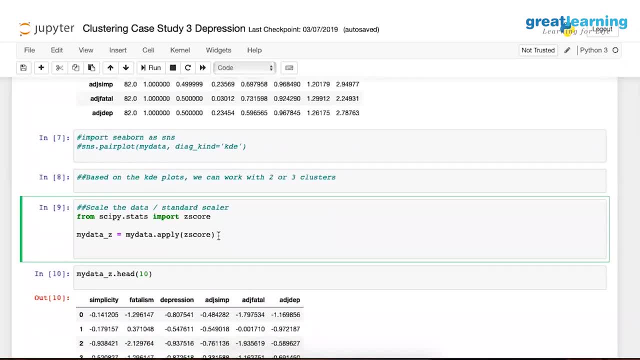 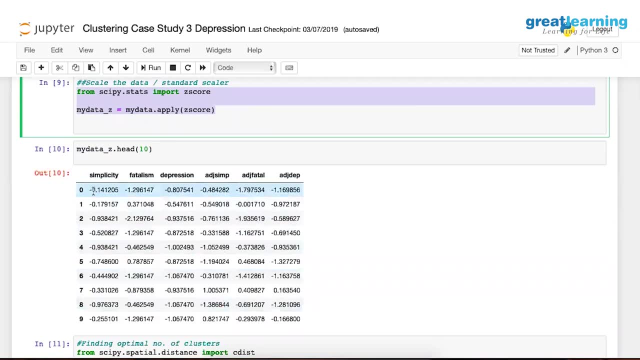 So next is: yeah, So the first thing that we are doing is the z-score, or scaling. So for scaling, the data will look like this. So some of them are not comfortable. Some of my batches get confused. Okay, why do we have negative numbers? 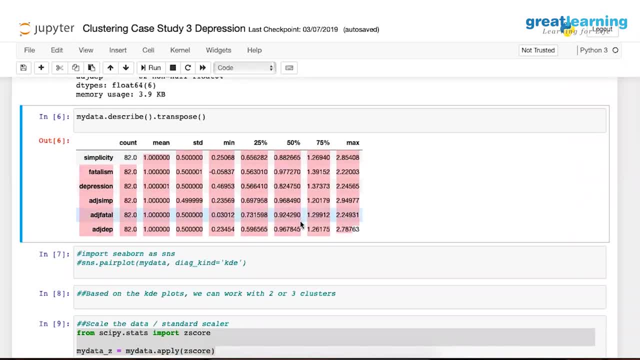 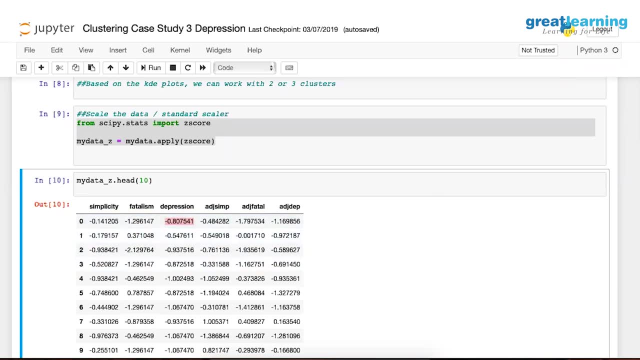 Please remember one thing: We are not changing the original values. The original values will remain same. How, if you look at the total standard, deviation and mean and all, it's not going to change much, except we are changing the axis. So originally it was here, now it is here. 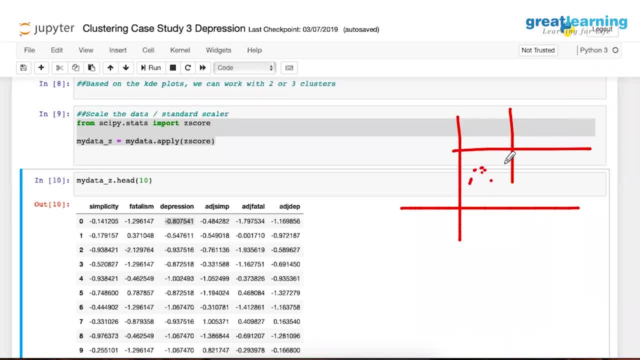 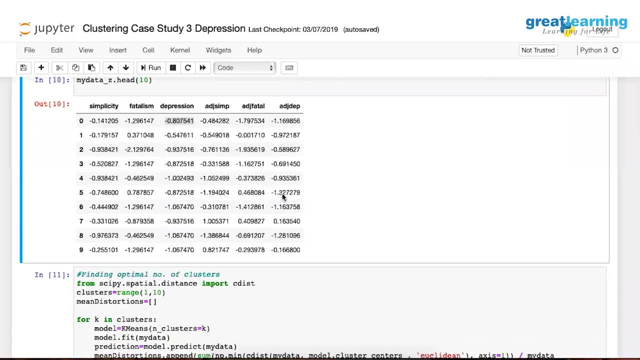 So imagine the points earlier which were here on positive axis. post-scaling, they will come on negative axis. That's the reason you will see some negative points, So don't worry about that much. yeah, Next is the way we find out number of clusters. 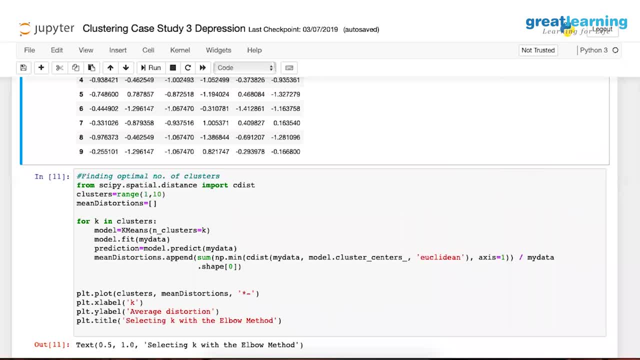 Now again, there are two ways to do this. The first way is when we come with a predetermined number. So let us say, we just saw an example here where we are trying to classify cats, dogs and rabbits. In this case, we already know that we need three. 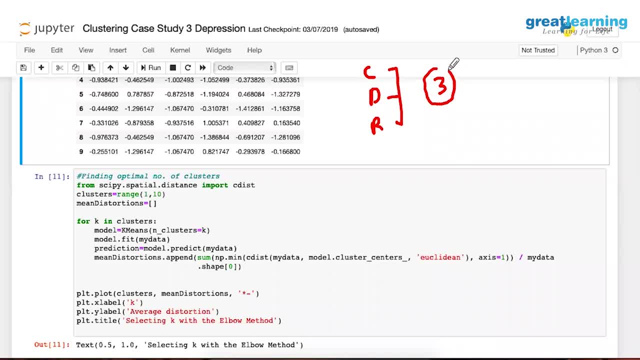 You don't have to go into any other technique. Directly put, k is equal to three. So when you already know it, nothing wrong. you can do it Else. if you want to know that as per the data set, let machine learning suggest us. 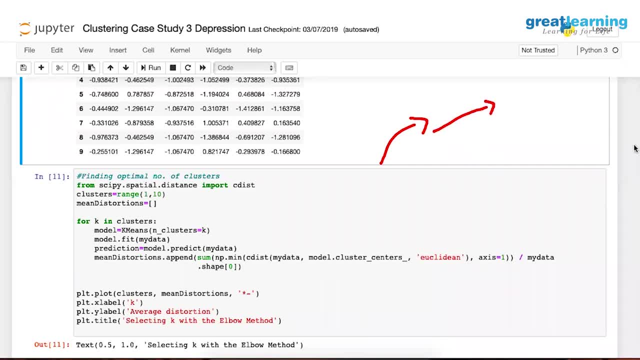 what is the total number of clusters? we can do best here, Yeah. So in this case, what are we doing is very simple. Python will try to put the points like this. Let us say: this is some points. like this, Python will start. 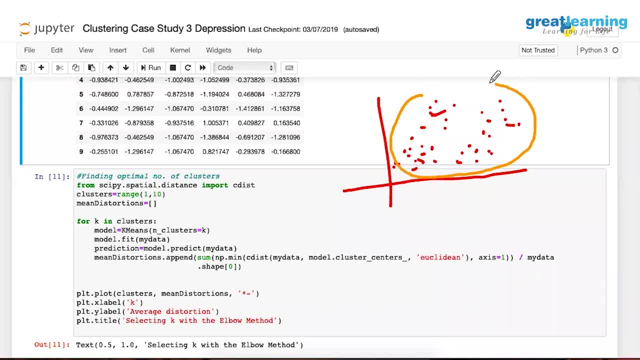 first of all it'll start with one cluster. It will say everything is in one cluster. Then it will say everything is in two clusters. It'll record certain data. After that it will say they are in three clusters or four clusters. 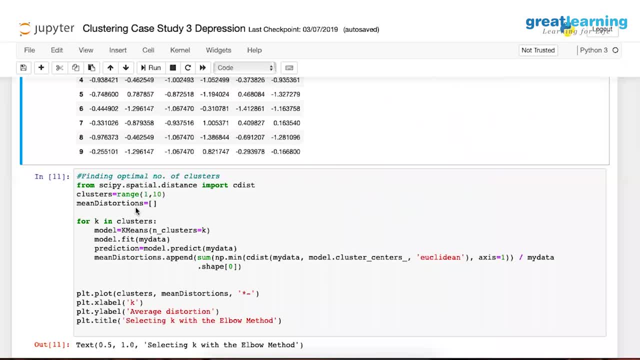 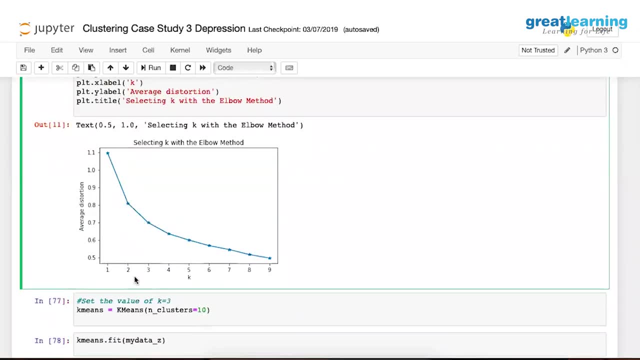 or five clusters. So, like that, Python is going to record all those values, starting from one going up to 10,, for example, if you look at this particular plot. So this is my number of clusters And this is my distortion. 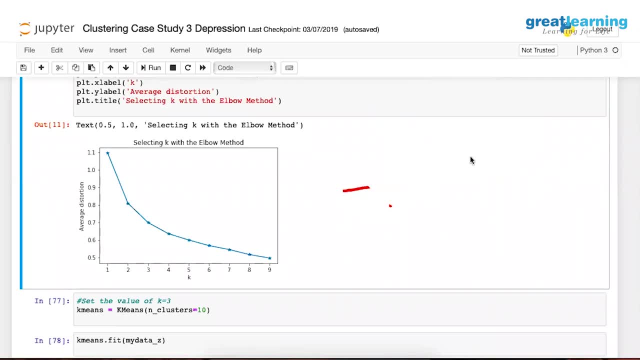 Now, what do we mean by distortion is whenever there are two points which are confused. So, if you remember, in the example that I gave last session, where there is a big area and there are some points which are equal to this is also an equal distance from this also. 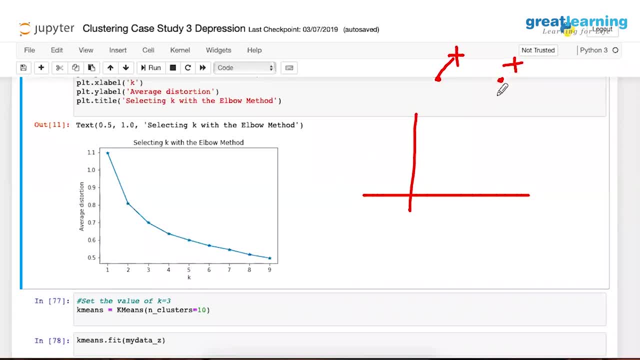 and equal distance from some other cluster also. In that case we call this as a distortion. Sometimes it go here, sometimes it go here. So keeping those distortions in mind when we plot. so when we start with one cluster we get certain distortion. 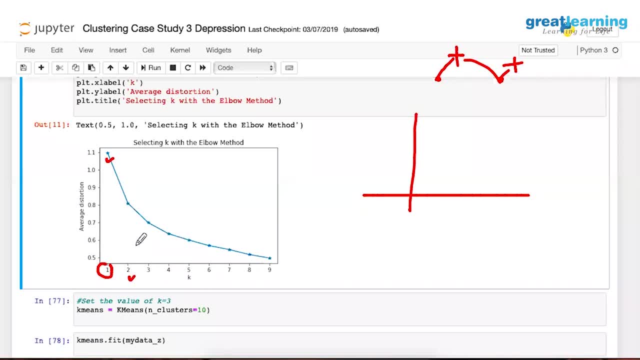 When we get go to this, so when we start increasing our cluster size, number of distortions might go lesser and lesser. But we cannot have nine clusters. It's not okay for me to have nine clusters. I'll tell you why. 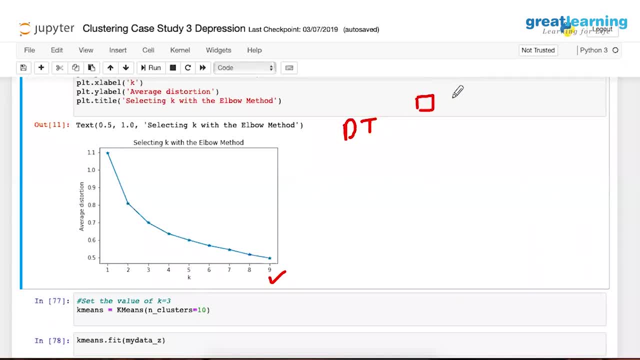 For decision tree. do you guys remember When we have decision tree, what is happening? Always there is an overfitting, for sure. why? Because the decision tree was made deep. You know, last time when we saw decision tree, we had around 11 levels of decision tree going around. 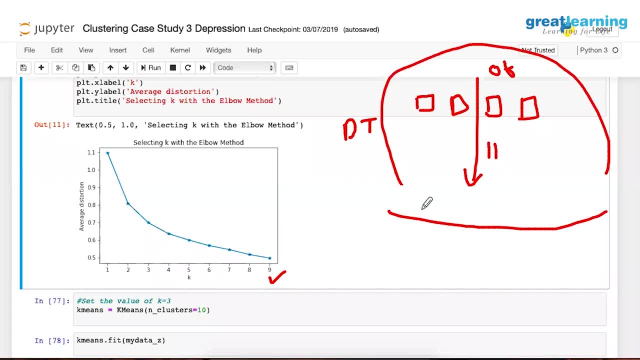 and multiple levels of nodes. So when we make, when we classify as per our convenience, there is a chance of overfitting. So when we over classify, also there's a chance of overfitting. So if you look at this curve, 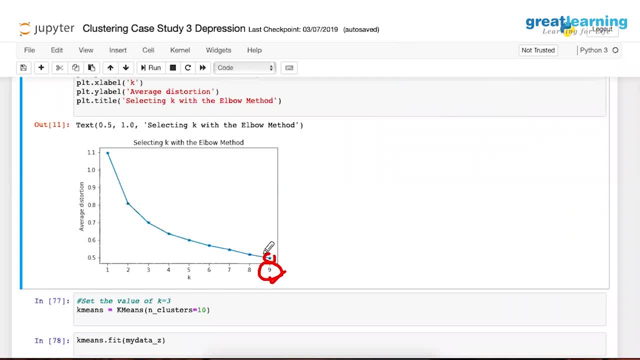 you will definitely feel that number of distortion is least for this. So my answer of K should be this: not at all. We are supposed to find out a particular point where the distortion abruptly goes down, So we call it as an elbow curve. 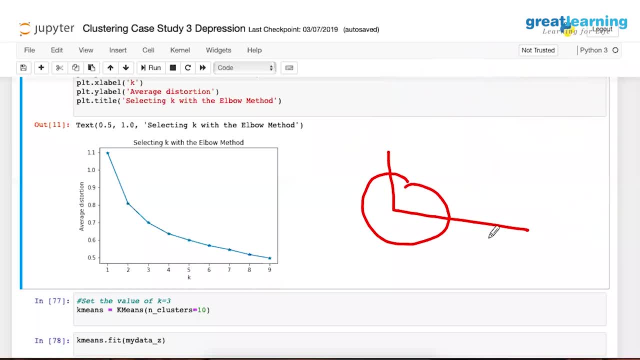 We will find a curve like this. that is our K value. So if you observe, here there is one elbow like this, there is one elbow like this and there might be one more elbow like this Remaining. all of them are kind of straight. 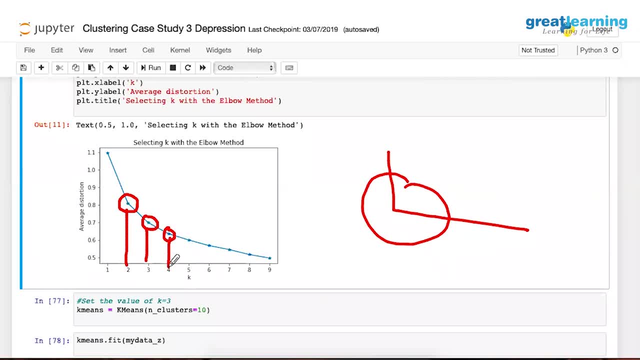 So one of these will be our optimal points. So what I do is I go, I check with this, also, I check with this. So now again, I say, it depends on our, our need. If you need four, do it four. 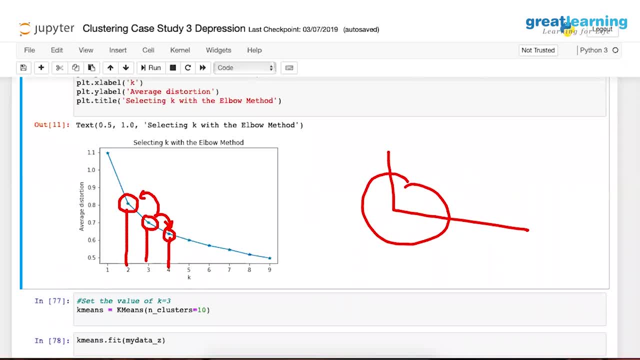 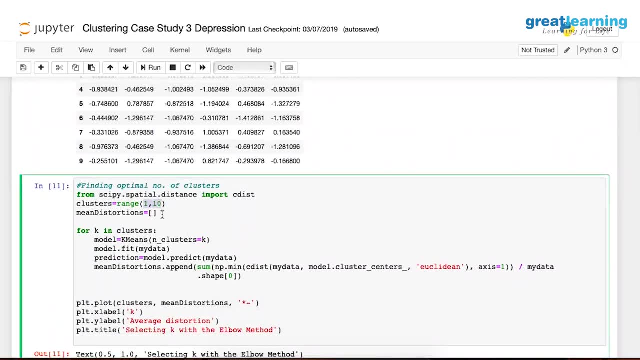 If you need three, do it three. do it two, do it two. Nothing wrong there. Now, how do we generate this plot? Very simple, It's like we are having a range defined from one to 10.. So, basically, from one to nine, 10 will not be calculated. 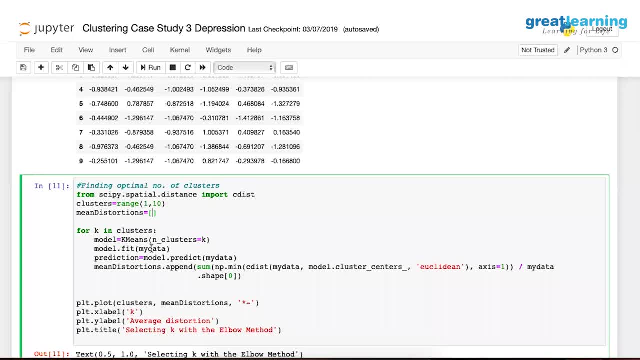 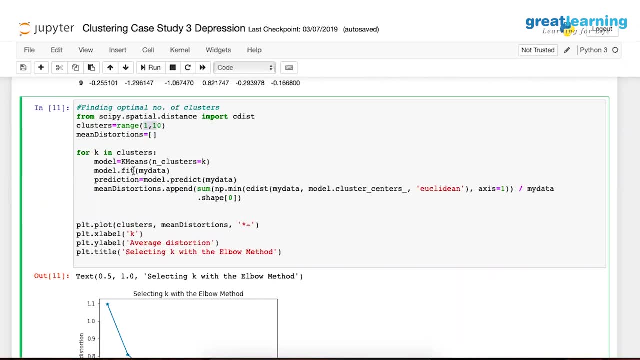 And we're keeping that number. 10 will not be calculated. Wait, mean distortion as an empty list. yeah, we'll store this mean distortion one by one. then we are running our for loop 10 number of times. okay, saying that start k-means or perform. 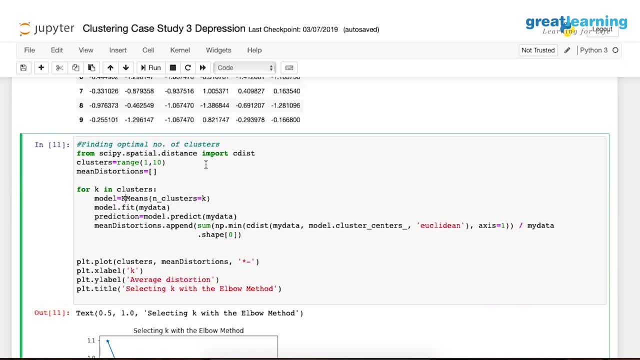 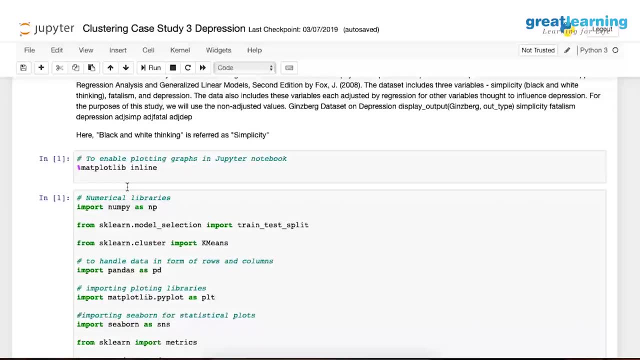 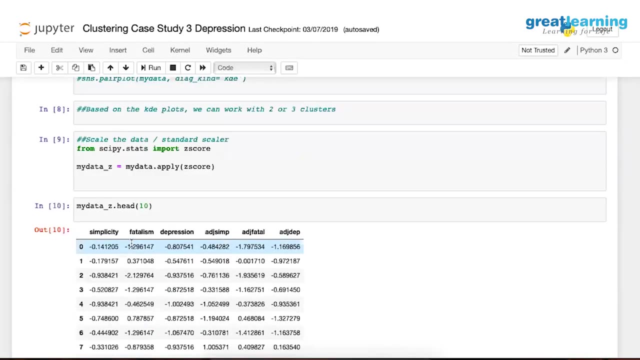 k-means clustering. how did we get k-means? k-means we have got from our where is our library, where is our k-means library gone? yeah, so from sklearn dot cluster we have got our k-means library, so from there we are saying run k-means on this data set with how. 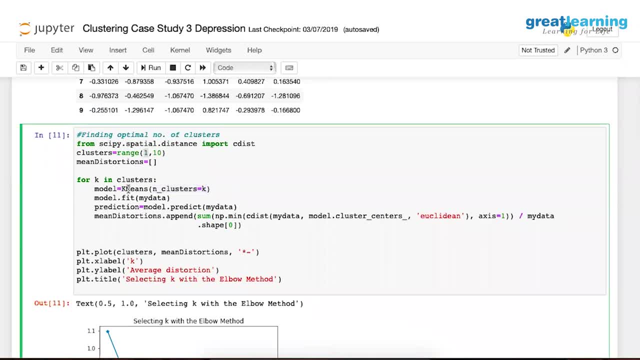 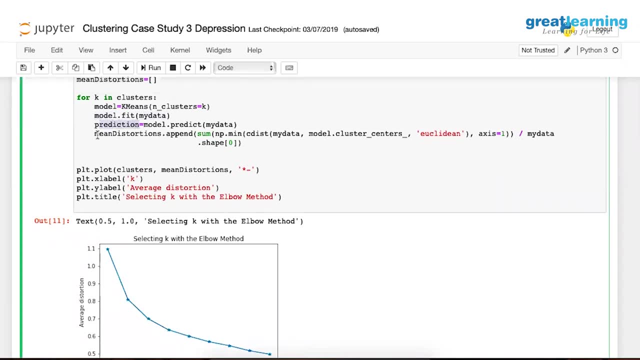 many clusters. clusters is equal to k, so the first value of k will be one. so that's how you will get the distortion point here. next you are fitting the model, you are doing the prediction and then you are calculating the mean distortion. now, what is mean distortion? 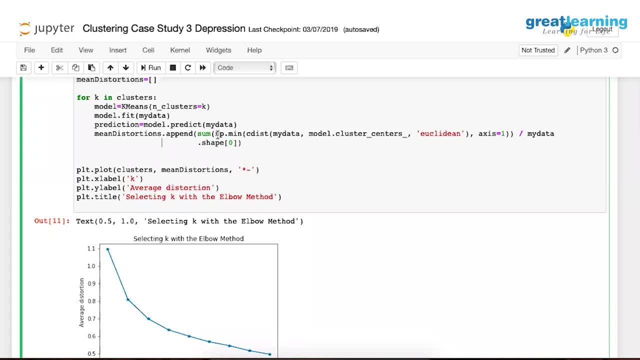 is. it's like: how do you say, find the minimum number of points with respect to the distance on your data with the model cluster center? so, if you remember, i said every time when modeling is done one center is found. okay, these are those centers, euclidean distance we are using onto that. 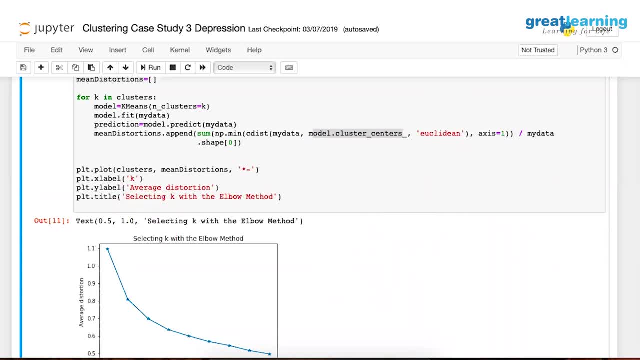 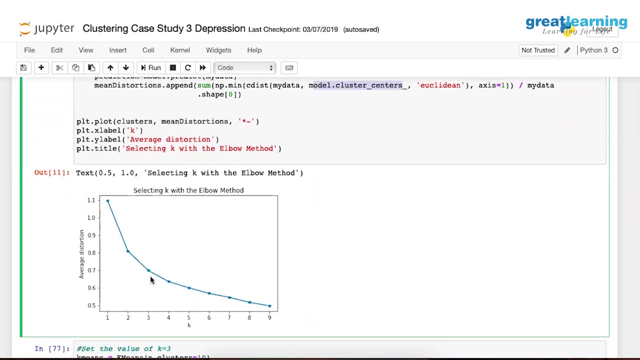 okay, so using this formula, you can find distortion. now some of them even do rmsc root mean square error. multiple ways you can do this. my method is using distortions. good, post that. what you do is you plot the curve. so when you plot the curve, obviously you can find the curve. 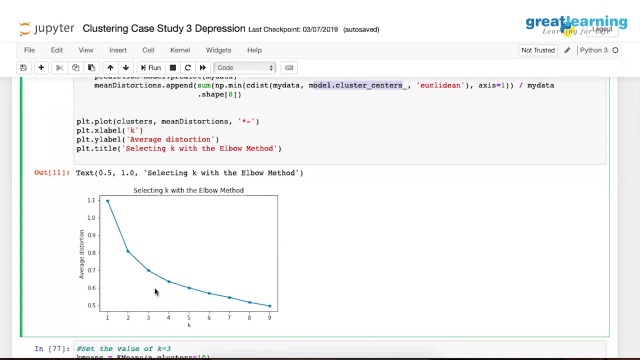 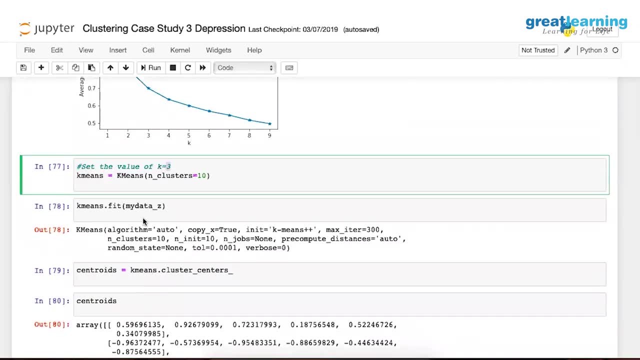 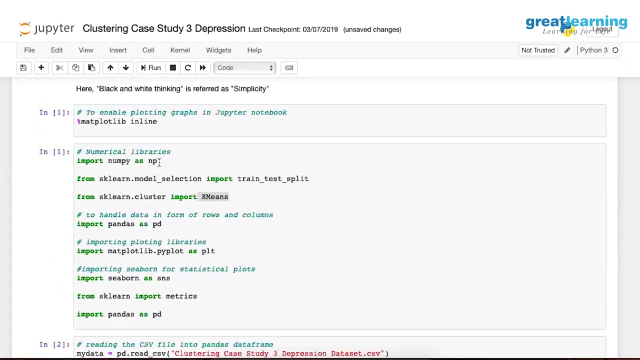 in the form of a, and every time you add a change to the curve you will get a negative value and you know that will be really annoying. it will be a big problem. you will just get each time 80 times it. in the end it will be maybe 3.5. this is a good question. we are going to go ahead and 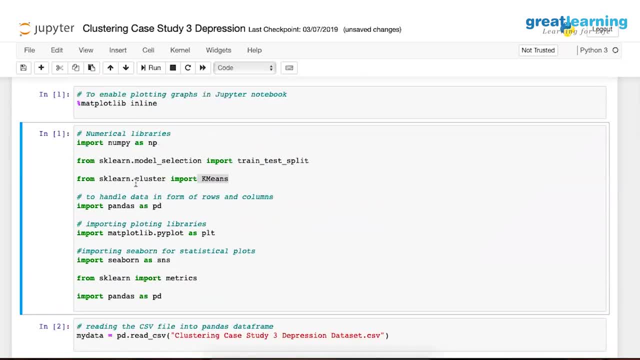 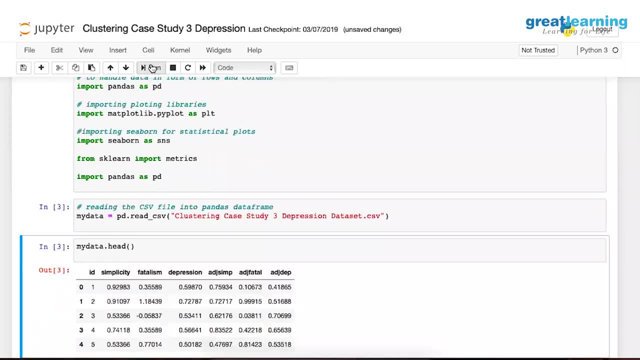 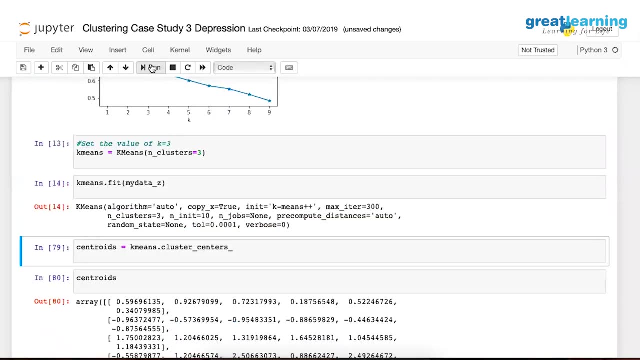 I think, when I might be showing earlier batches. no, I would have done that. Good, Okay, So now my key is equal to three. Now I'm fitting my data. Okay, Centroids- Okay, One minute, Yeah, So next. 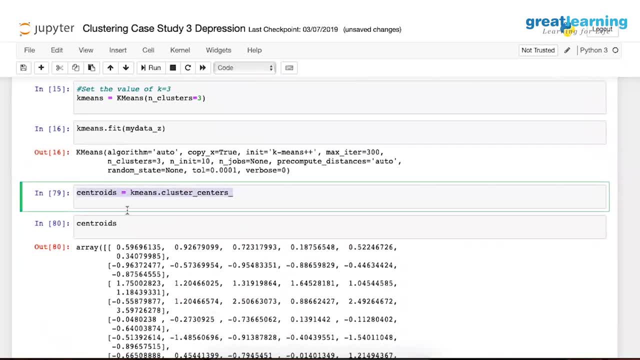 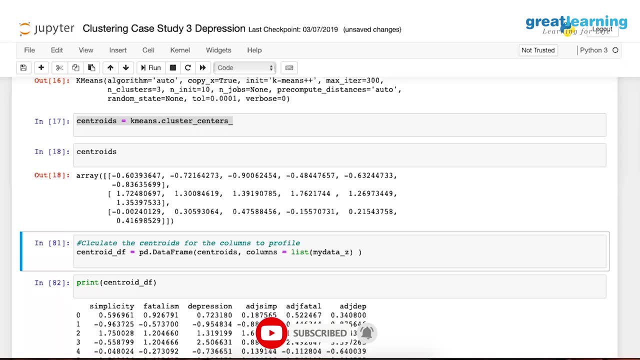 So it's not mandatory for us to check the centroids, but just for our understanding, what I've done is I've generated the centroids. Now, if you guys can visualize this, I say if there are three clusters, there should be three centroids. 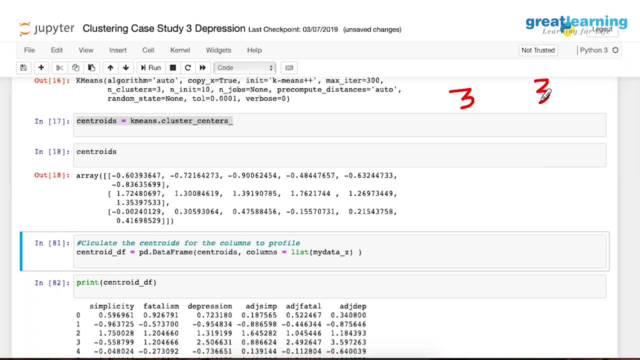 Correct. Yeah, It's a uh. what is? the cluster will have one centroid, But in this case, what I'm trying to show you is we have got these many features. If you observe our data set, these are the features that we have. 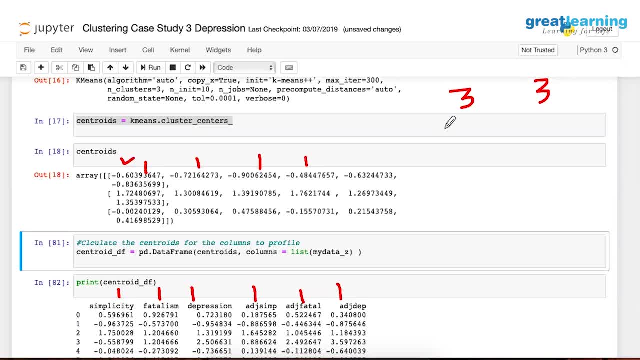 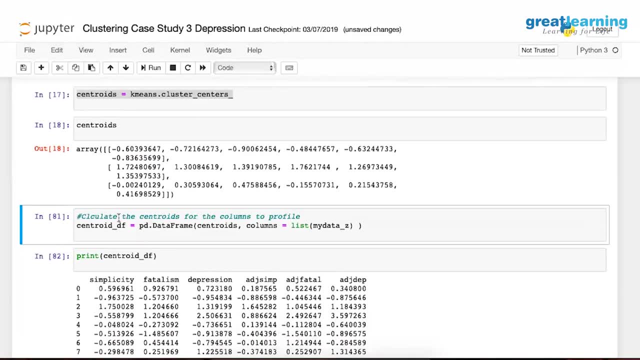 Yeah, Python is capable enough. You have to build one centroid for each feature. Yeah, So if, in case, you want to reframe this, what we can do is rather than visualizing this way. see, it's not necessary to visualize this. 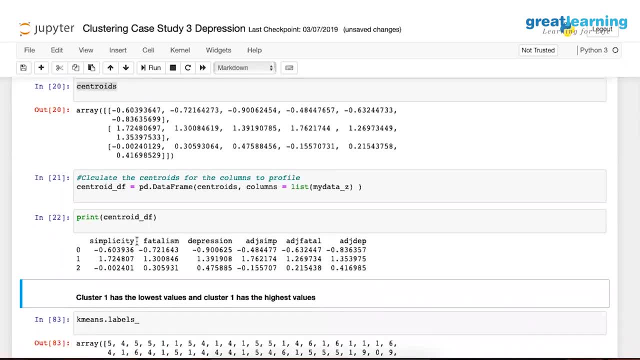 Okay, This is just for our understanding. I'm going, If you observe here simplicity, the centroid for zeroth cluster is this, for first cluster is this and for the this cluster is this: if you want to find a total centroid of zeroth, 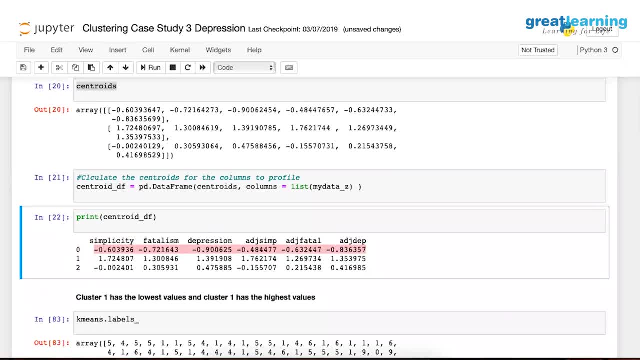 cluster what you're going to do. You find the average of this. You will get the center. Yeah, Now some of them. why did I do this? is just to show you guys that post. So this was my data before normalizing or before scaling post scaling. 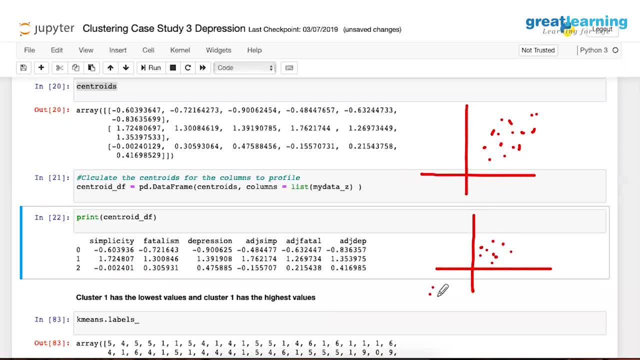 What happened was some of my data was up, Some of my data went into negative side and some of my data cluttered around the center. You can observe the same thing here. You can find out one cluster which is completely negative. You will find out one cluster which is completely positive. 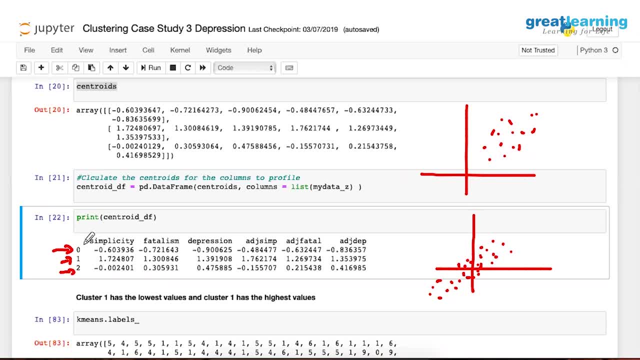 And you will find out one cluster which is a combination of positive and negative, So the one which I'm showing here in the zeroth one, this is your zeroth cluster, The one. the first cluster is this one And the second cluster is the one which is centered around the origin. 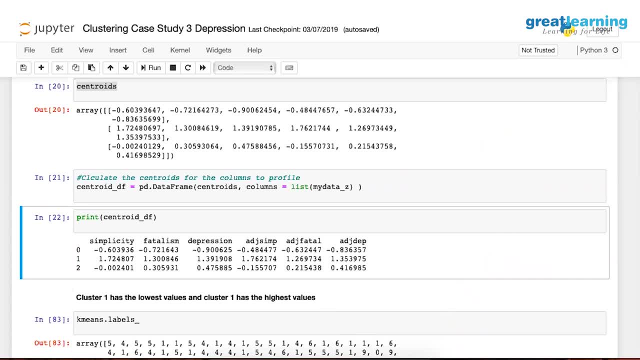 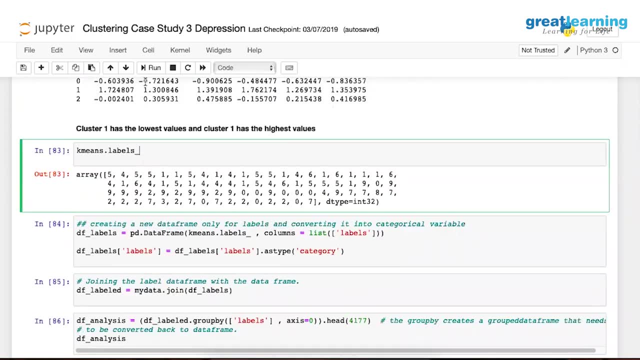 Okay, So this was just the reason to show you guys. otherwise we don't need to worry about this. You're just not making any impact on our answers anyway. Okay, So next, uh, let's generate our K means. So this is our target variable. 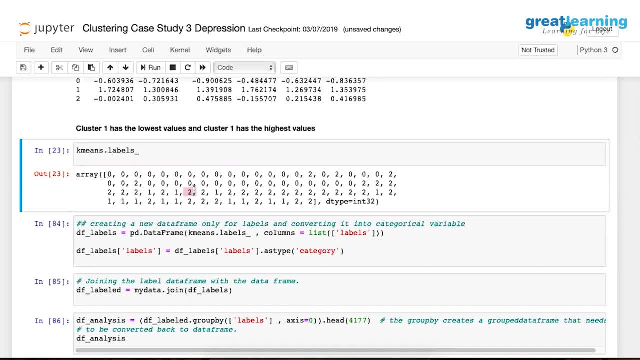 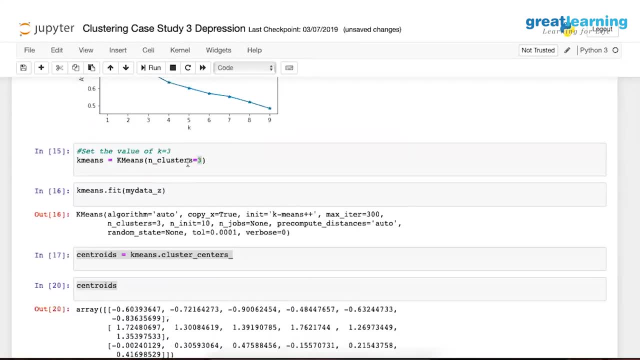 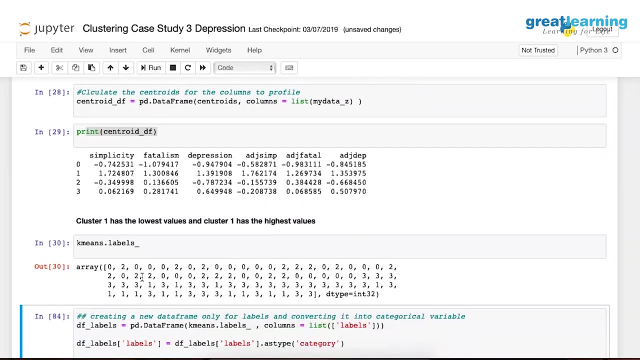 So these are our targets. zeros, ones and twos right, Because we have got K is equal to three. That's the reason we are having three targets. If my K was equal to say four, as I said above, you will find two, three, zero and one four. 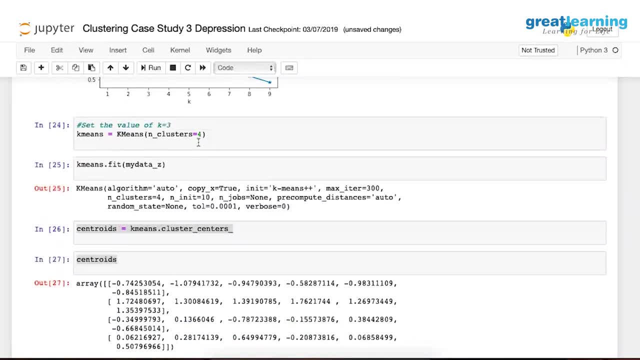 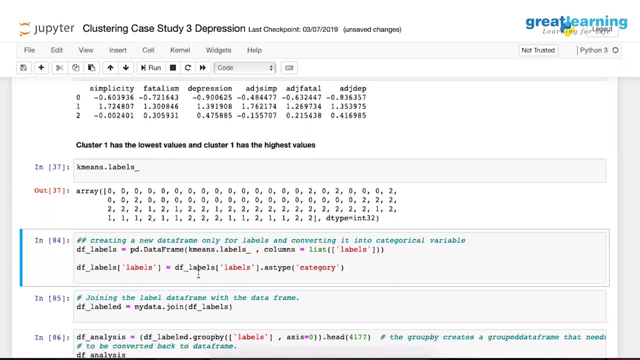 targets. Got it, guys. So this is how you do Clustering, So let me change it back to three. Now, next, what are we supposed to do? We are supposed to paste this as the last column. So what I'm doing now is I'm converting my labels as categories. 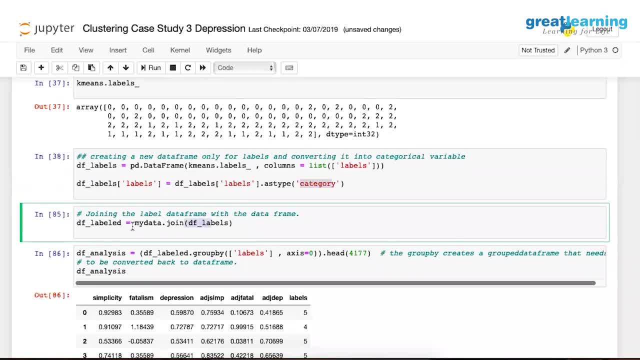 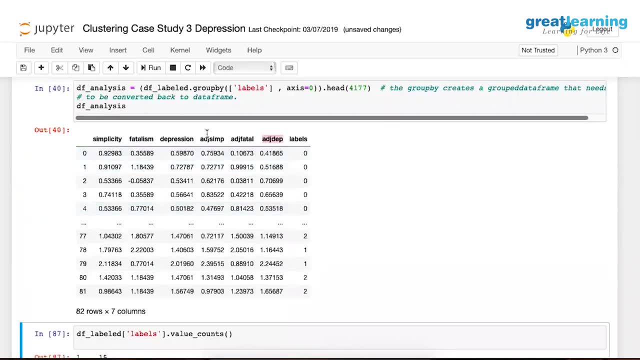 Okay, Then next, what I'm doing is I'm joining my older data with my new data And finally I'm displaying my data. So now, if you see, our older data set had only these columns. the labels were missing. Now we have appended some labels. 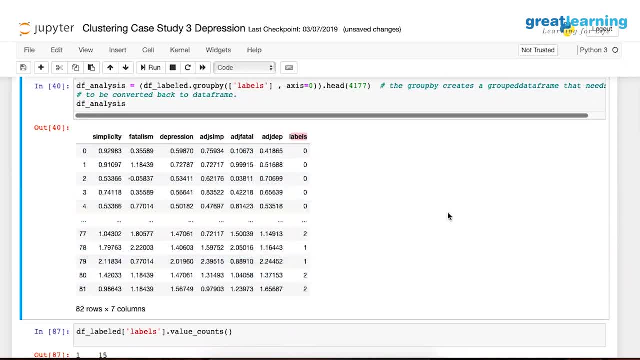 Now our data set is ready to be pushed onto some of the machine learning techniques so that they can build a predictable model out of this. If they don't want it, it's okay, if they want it, it's good. So our current business problem was what that? when the computer or when the person 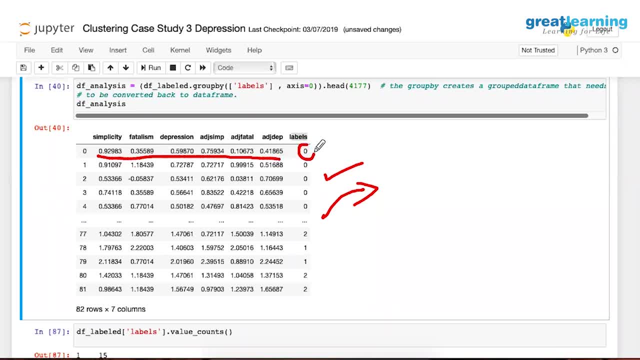 generates this report automatically, it should tell us what type of depression level it is. Either it's a very high level, mid level or low level. Again you are. it is not necessary that zero will be low level. No, You can name whatever you want. 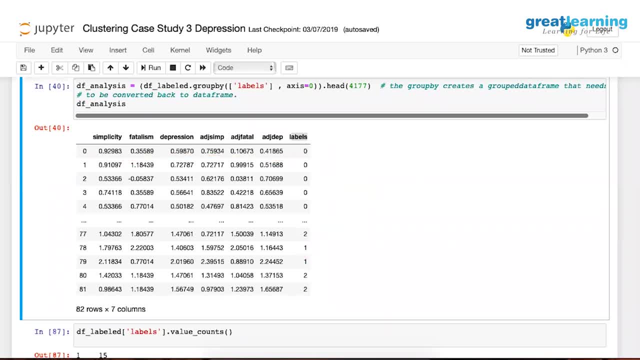 So post this. If you want to automate it more, you can write one more code saying that if label equal to zero, then change it to say depressed patient. else say not depressed patient, something like that. Whatever you want, you can label this zero once and twice. 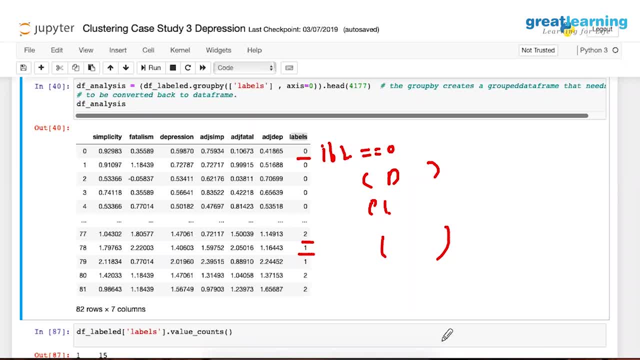 Okay, Any confusions guys? Yeah, Simple. If you ask me applications of clustering, so from the industry point of you know, since all of us are almost very high level or very high amount of experience, I will say: use clustering majorly when you are onto marketing or customer segmentation, or if you are, if 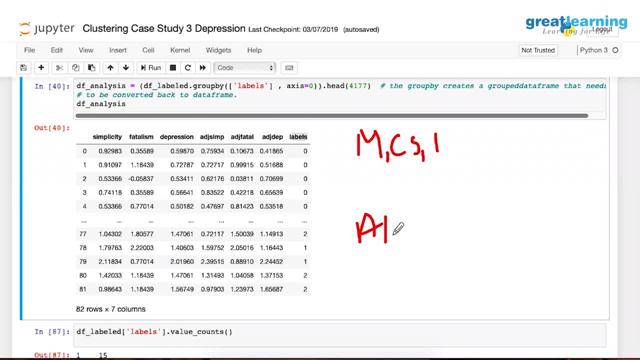 you have done an experiment, let us say. if you have done an A to B testing onto a marketing campaign, in that case you can use clustering to solve your problem. Okay, But some of us, let us say, who are a little innovative, and if you want to take a better 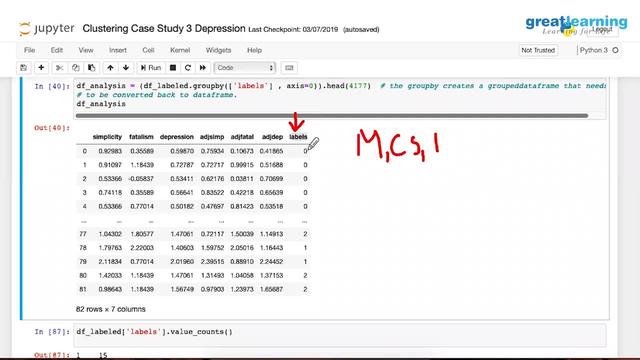 side of this. if you find a data set without labels, convert, put labels, push it onto machine. This is more popular. This one might not be explored that much. Yeah, So anybody here from marketing side? Yeah, Yeah So Nitesh. it's Nitesh, right or Raju. 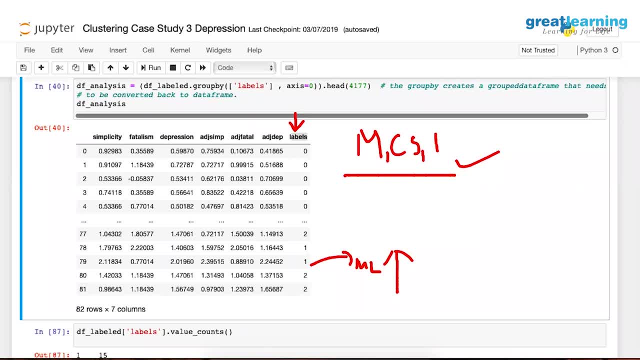 Yeah, Sorry, Yeah, Yeah. So this is: either you can use Tableau- Tableau has an inbuilt facility to do clustering- or you can use one of these to do cluster. Nothing wrong with that? Yeah, Perfect. So this was your unsupervised learning clustering. 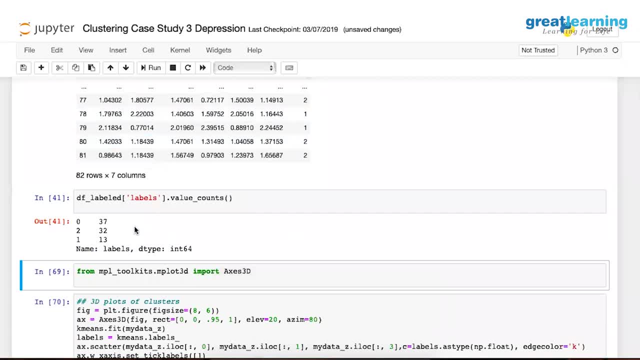 And if, in case still, you want to find out the imbalance or the balance between each of this thing. So number of zeros we found was 37, number of twos we found was 32 and number of ones we found was 30. So this is how you segment your customer. 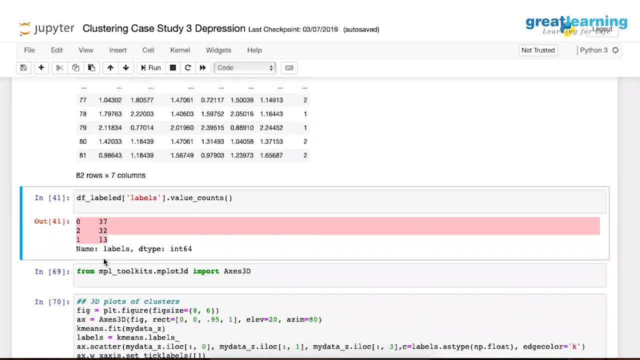 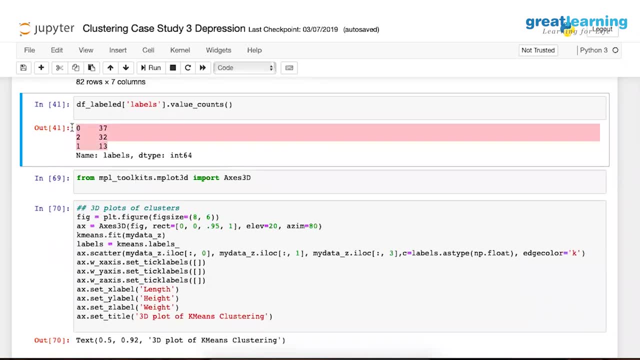 Okay, Perfect. Still, if in case, I will again recommend Python, I will not recommend Python for plotting them. Why? Because it's 3D data. So again, I will say Python is not the best solution, but if in case, you want to plot, 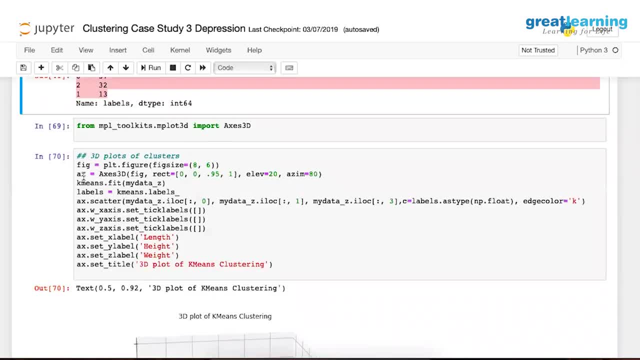 it, you can generate a plot like this. Now, what is this plot? This is a 3D access plot Standard code. You don't have to change anything here, except you just have to change the variable that you are inputting. For me, it is my kmeans labels. 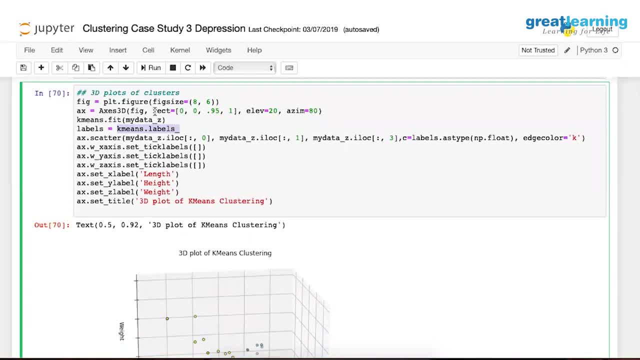 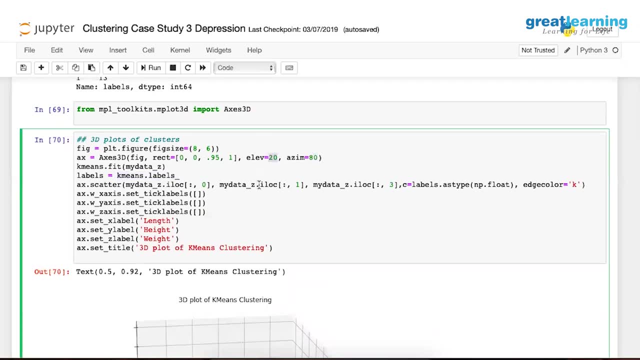 Yeah, The labels that we generated at the above, That's it, Suppose that if you want to rotate, you can change the elevation and asymptotes: it will rotate. Okay, So if, in case, you want to see this how it works, I will, let us say, change the elevation. 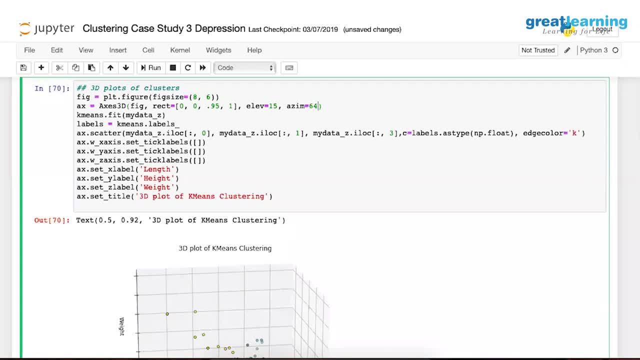 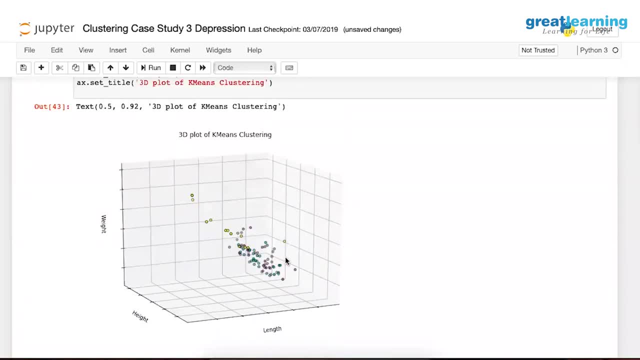 to 15 and the asymptote to 65.. So you can observe that the view changed. Yeah, Now why do we change this view? Sometimes the data is cluttered. So why do we change this view? Because the data is cluttered. 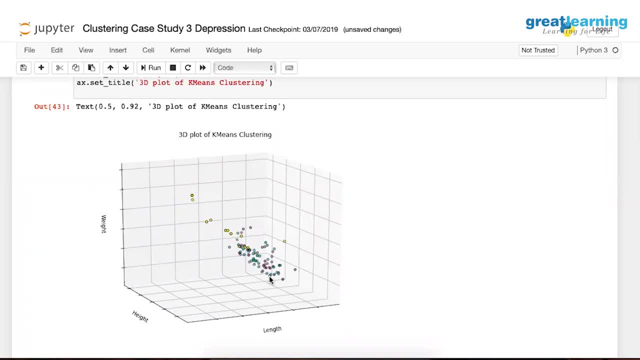 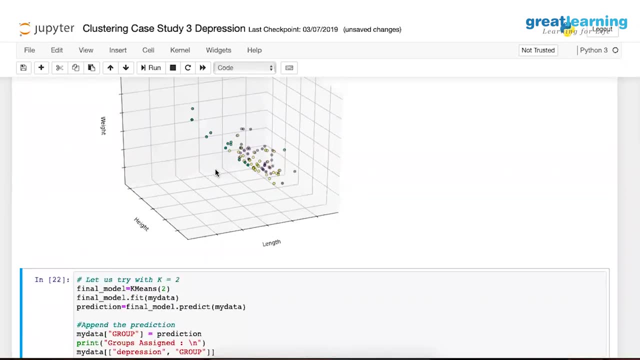 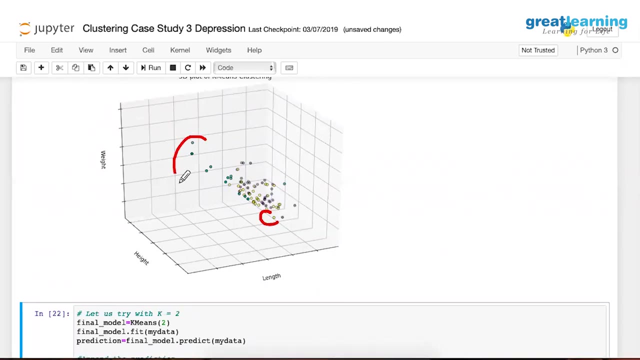 So we cannot differentiate between points. So if you see, here the data is pretty cluttered. So if I change, let us say, to 25, it will be more cluttered. Yeah, So if you can observe here one of these points, some one of this point might be group number. 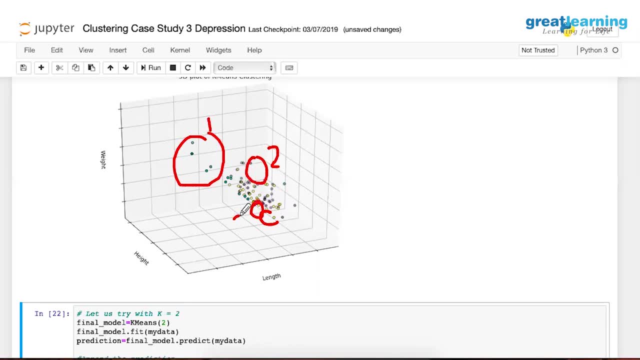 one. the one will be group number two and this will be group number three. Now, when I show this to my batch and ask my other batches that, okay, fine, can you find out if there are two pluses which are cluttered together? 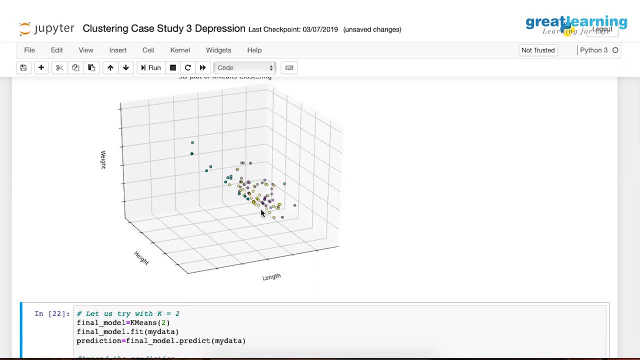 We cannot say: they say yes, Uh, uh yellow, and uh say purple, they are cluttered together. Okay, We cannot say that. Why? Because we are viewing this in a 3d way. So, for example, if I change it back to original value, 20, and uh, what was it? 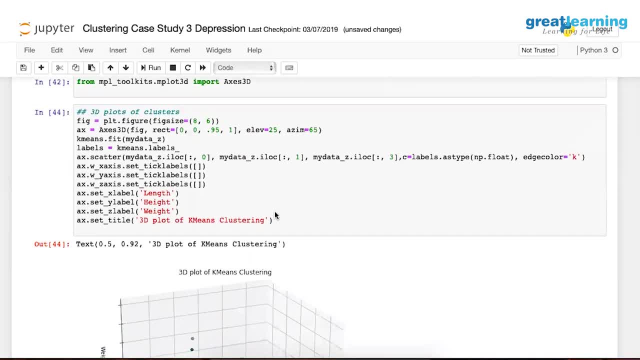 I don't know if you guys remember It was around 40.. Yeah, Now everything looks cluttered, So it all depends on finding the best location, but definitely it's not cluttered. Okay, Okay, Okay, Okay, Okay. 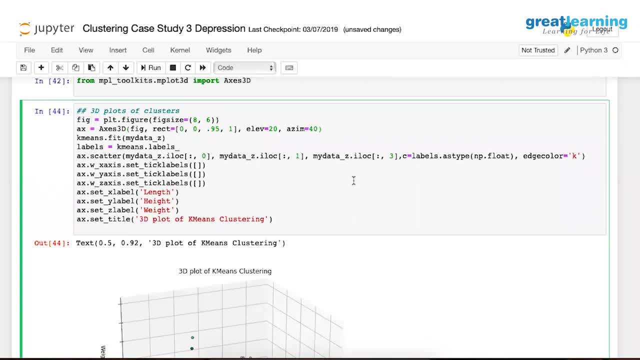 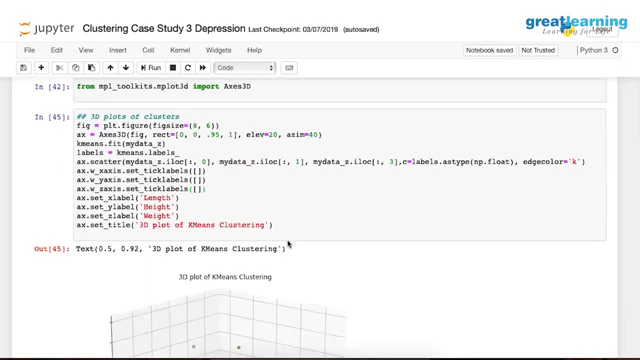 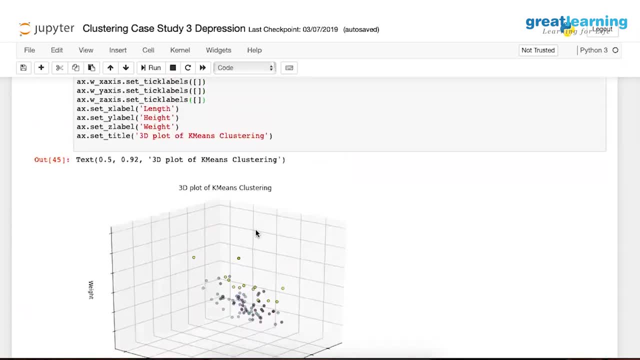 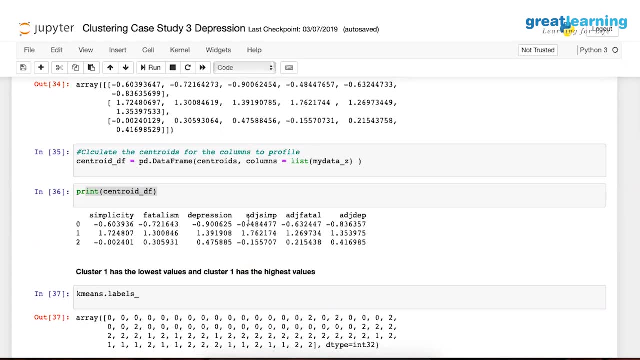 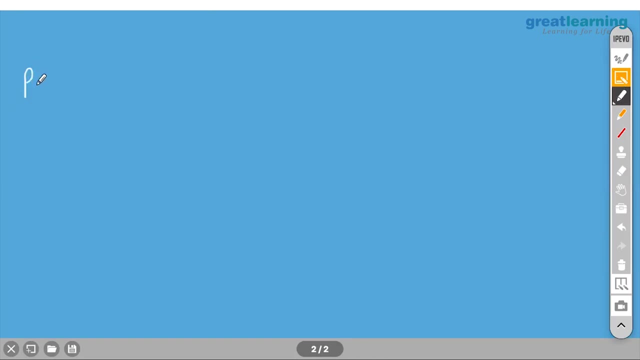 Yeah, So this is how we can plot. yeah, So that's, it is your clustering part. Any questions for me here? I hope it's pretty simple. Okay, Good, Perfect. So now we'll come to a little complicated topic called principle component analysis. 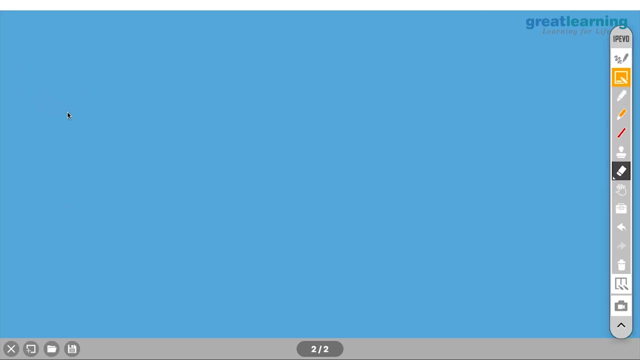 Okay. So any ideas about PC? Have you heard about this topic? Uh, okay, anything. yeah, it is. it is dimensionality reduction, exactly, yeah, so you know the basics of it or you just heard about it? no, I've just read some definitions, okay. 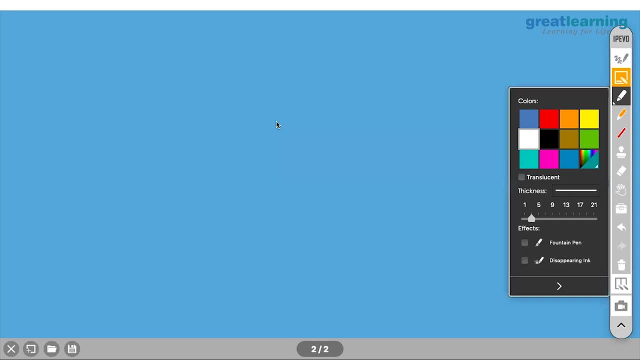 fine, again, I will say all of you this: once I complete my PC, do not refer anything else, because majority on the web people talk about high level things and they don't get it that if you are training or if you're writing a blog for a fresh person who is learning PCA, that is not the way to write it. so currently, 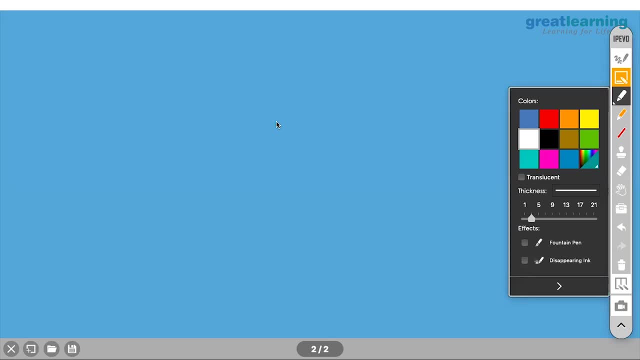 what I'm doing is I'm. I will write a simple article on to that and I'll share it with all of you, but for now you just remember what I'm showing you guys on to PCA, part of it: okay, make your problem solved, otherwise, when, when I take 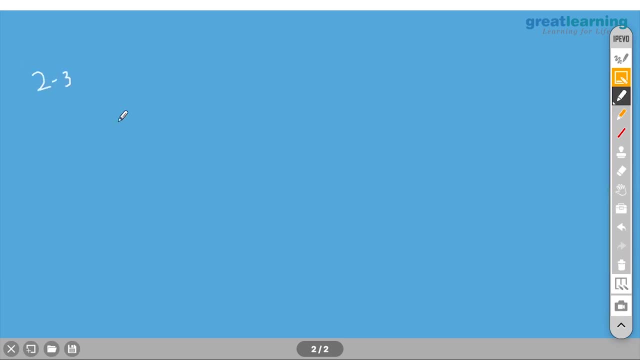 interviews, also for people who are two or three years of experience. what I do is I usually take this algorithm. why? because this is algorithm where you can catch whether the person is actually worked on analytics or data science or not. because this is one of the most widely misunderstood algorithm. okay, now, why do I say this? you people will. 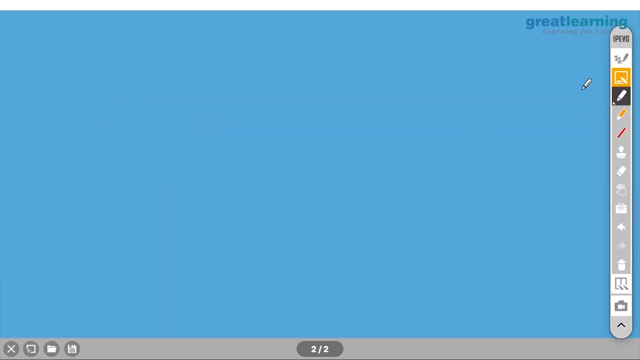 feel it now? and also, why am I running? one week ahead is when you watch PCA videos. I don't want you guys to be really confused. so when you have basics onto it, when you watch those theoretical videos, it'll be easy for you to pick it up. so sometimes people say, oh, I have to learn this algorithm. I don't want to. 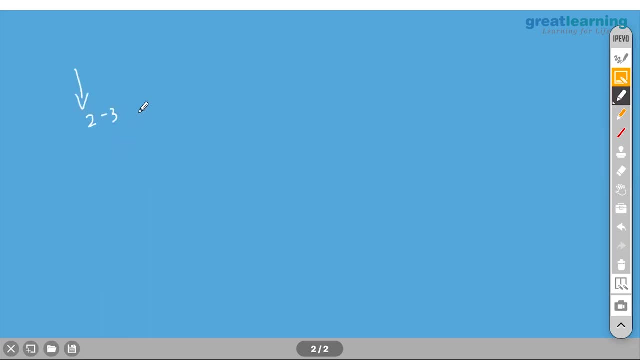 learn this algorithm. I don't want to learn this algorithm, I don't want to know. say that I have watched videos twice or thrice to understand. so in this case, you don't have to do that one shot. it should be good. now coming to PCA, so one question to all of you is: let us say: 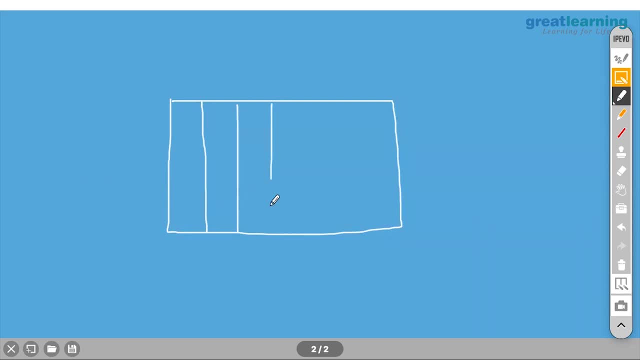 there are multiple columns, okay. so let us say: if we are talking about a marketing campaign, okay, and we do not have any target. so, since we are talking about PCA and unsupervised learning, let's ignore the target variable for now. but imagine, the target variable is there in front. 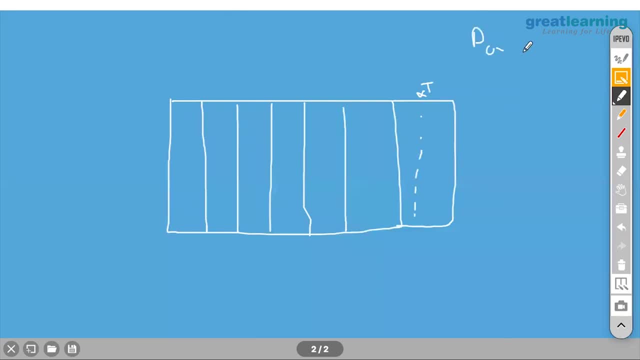 of you, or else we'll take the example of a Portuguese bank data set itself. so let us say: these are our attributes attached to it and this is the target variable. now what if I ask you, frankly speaking, do you feel all the attributes given to you in those data set? is it needed? 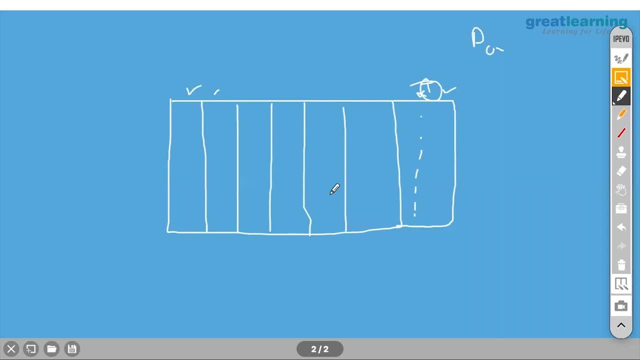 to predict this, like. I'll give you an example of profession. okay, I'll give you an example of age balance. previously participated in the thing: date, time. lot of attributes are there right? what if I do not? or what if I feel that not all of them are? 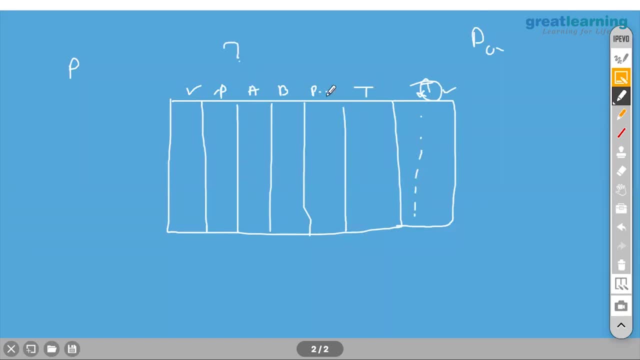 needed on to it. how do I find out that some of these attributes are of no use to me? so first question, okay, first question to all of you is: have you ever done like? have you ever done like? have you ever got a data? not, I'm not talking about analytics or data. have you ever gone, got a? 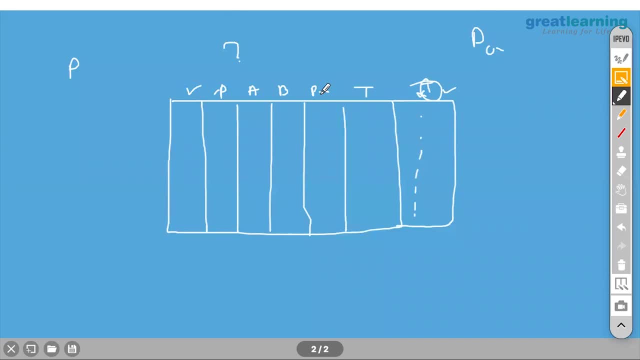 data from client C and when you're making a presentation, you have omitted certain columns by your own, keeping in mind that this is useless, it's of no use to me. we have done that right many times right because we have an intuition here that it's not needed. but what if I want to do? 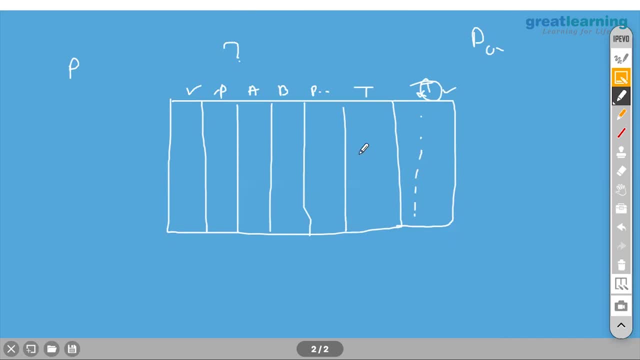 it on data science: is it fair for me to directly remove a column? no, no, right. why? because there is some data attached here and we are answerable. because if, in case, this data might impact, in our mind we will feel it's not impacting. but what if it impacts? we don't know? right, because 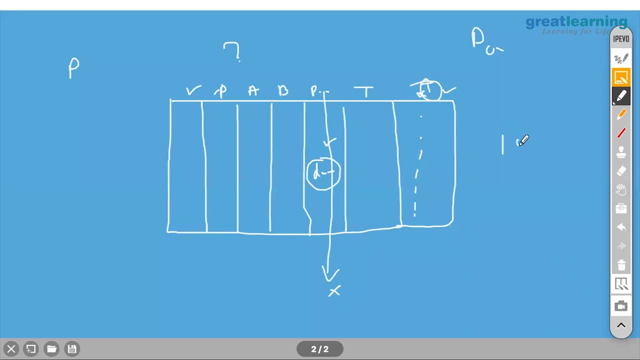 I have done one PCA. worst case I have done it on 150 columns. we had 150 columns so we were confused, like it's it's taking a lot of time onto. so we were making a machine- sorry, we are taking making a neural network here- and it was too much for the neural network to take it up. so next came the. 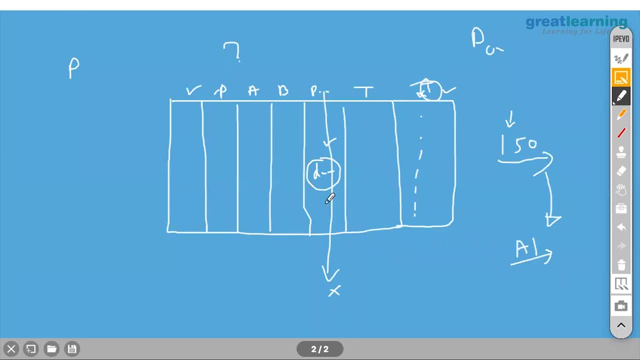 challenge was to how to reduce this. so what we can do is we can blindly remove this column. now, when we did, we did remove the column. definitely it solved some of our computation time, but also we felt that sometimes our accuracies and you know more learnings and all came down. why? because 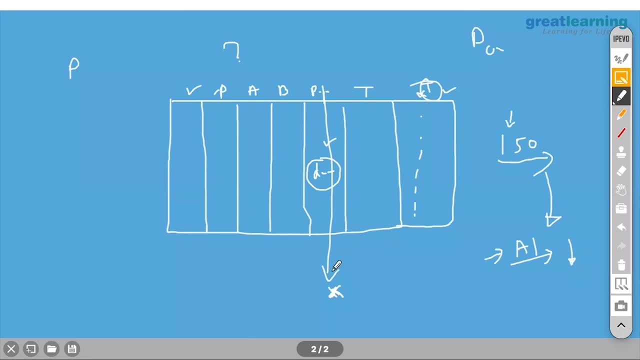 we lost the data here. yeah, so then what should be the solution in this case, what we should do? I'll give it two or three minutes, just think it out, what we can do here. I don't want to remove any column yet. I don't want 150 dimensions, or what if somebody from here from marketing right? 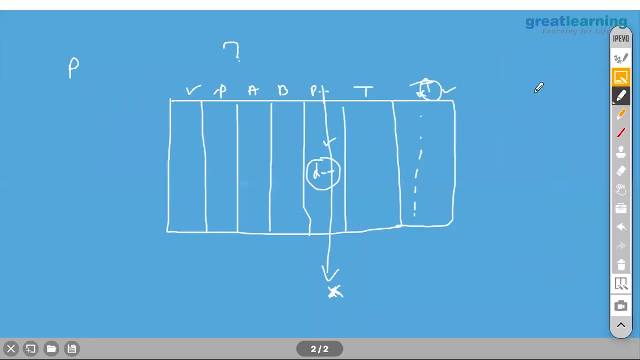 so what if I tell you that I will give you a clustering problem and there are four dimension onto that plot it? will you be able to put a 4d graph? it's not at all. so in this case, what we are supposed to do, max we can plot is 3d. yeah, so what we are supposed to do, max we can plot is 3d. 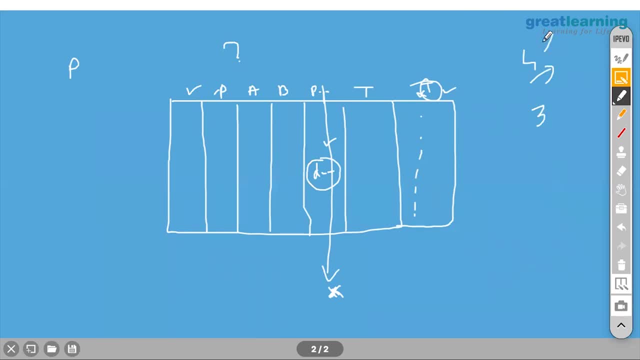 so we cannot tell the client: okay, since you're not able to plot it, we are removing one of our dimensions, we'll not need it. so what should be the solution then? this is implementable. I wanted this way. now my question is: what do you guys think how we can smartly reduce our dimension? 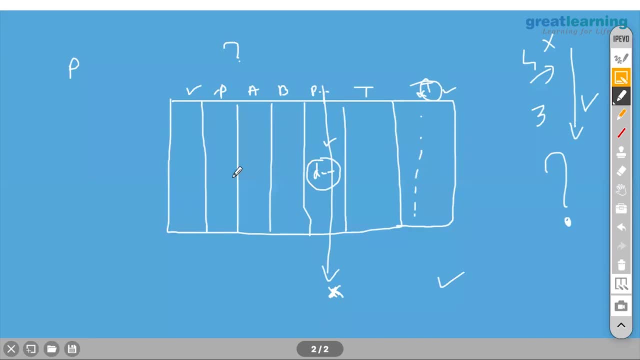 also and not lose data, and I'm talking about statistics. so just try to think that way. no idea, probably probably change the data type or something. I don't know, because that's what we're doing now. data type means, let us say, if it is numbers, yeah. if you're trying to say we should change it to object, or 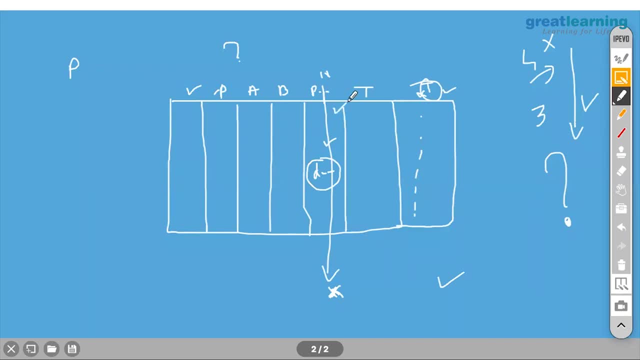 something okay, but still we are going to. we have to use it right. can we divide the data? divide in the sense, small parts. so divide in the form of columns or rows means aggregate. I am yeah. so we can, you know, take, make groups, and then we can make groups of these and plot smaller groups. yeah, 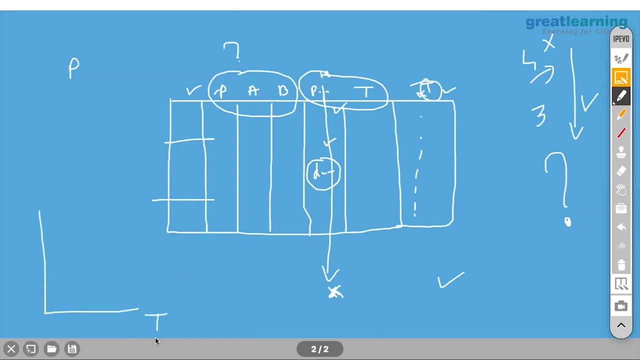 smaller groups. but what if I want to plot it against target variables? so out of this 4d, one of them should be my target and remaining three should be my behavior. what if I don't want to compromise on that? yeah, your idea is correct. we can do that. but what my client wants versus target? 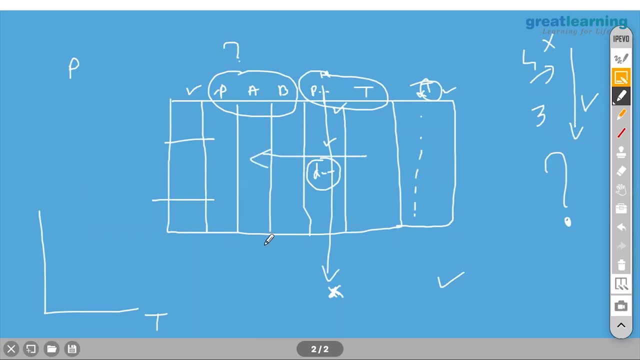 how all of them behave. I don't know random sample data. when we create the x and y right, just cut those right and still keep the data correct. so if you random sample it also, we will not be reducing the columns here. we are talking about reducing the. 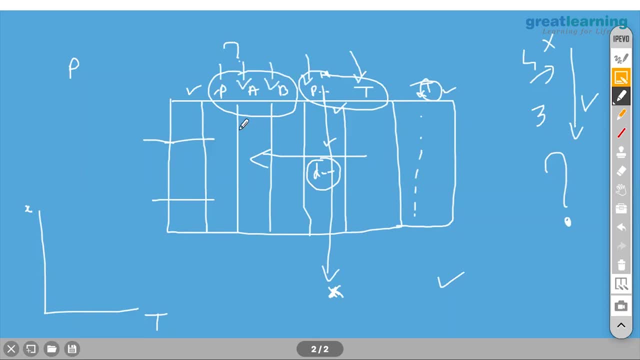 dimension. dimension is nothing but your column, okay. so have we heard about covariance anytime? yeah, yeah, so here we are going to use covariance to do this. now, let me show you how we can do that. So what, i will do this. let and say: i have got. 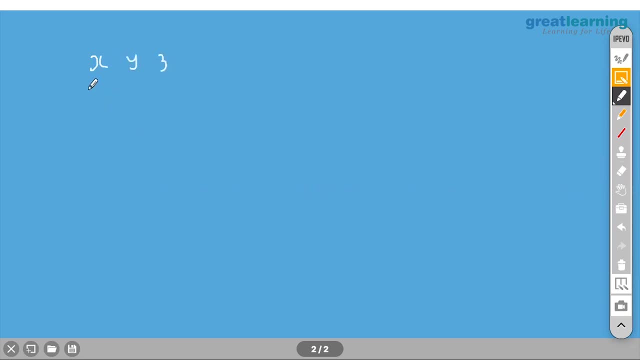 three dimensions: X, Y and Z, for example. and let us say i have got points like 1, 2 and four background: 0, 4.. 0, 2, 3, 2 and let me change this to 4, and here I have got 0, 1 and 3. 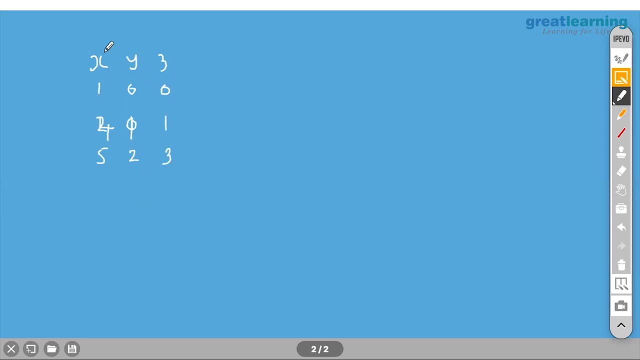 So let us say, I've got some plot like that. now my intention is: I don't want 3d plot, I want a 2d plot, but yet I do not want to lose any of the dimensions. So please remember two things. first thing is we are going to do dimensionality reduction. 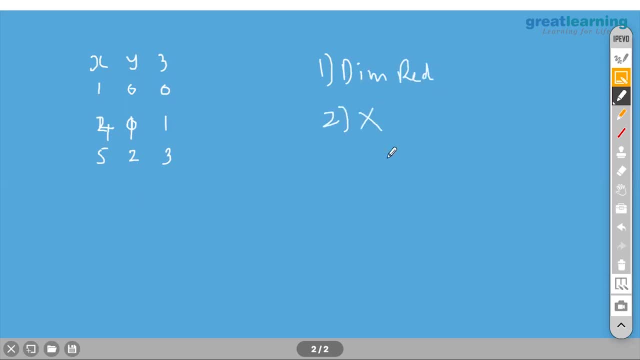 Okay, Paradox. we are not going to delete any dimension. Okay, so it's like a paradox. Please remember that. now how I will show. Let us try to plot this, for example. Or else, let us not confuse with Z, for now Let us like to plot X and Y, because if I plot Z it will be a little weird plot. 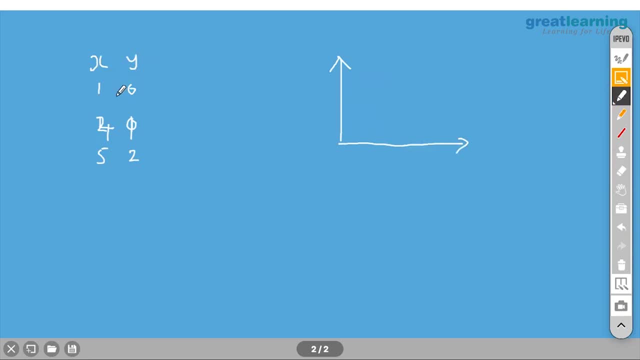 Let us say I want to reduce this from X and Y to only one language. So what if I plot this for 1 comma 0? so I'll have 1 comma 0 here, or else I will change the color. You will have 1 comma. 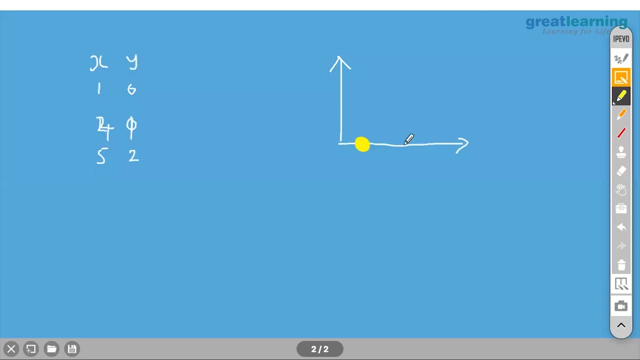 0 here. let us say: next is 4 comma 0, so 4 comma 0 here, Next is 5 comma 2, 5 comma. Okay. so this is our plot. now, if I ask you, We have two axes, were two dimensions here, dimension X and dimension Y. 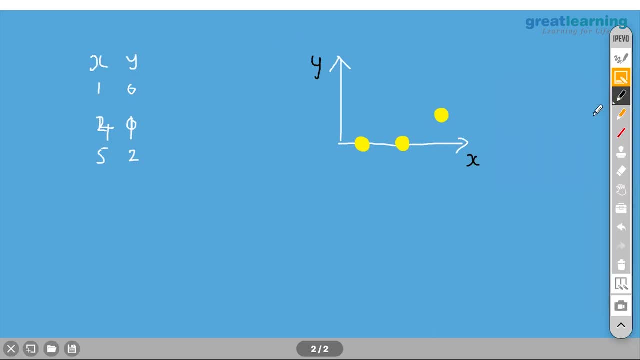 Which of the dimension retains the majority of variance, or majority of numbers? What do you guys think? which dimension here retains majority of numbers? X, because Y has got couple of zeros. okay, so now, keeping this concept in mind, Tell me which dimension has more variance, which Dimension has less variance? 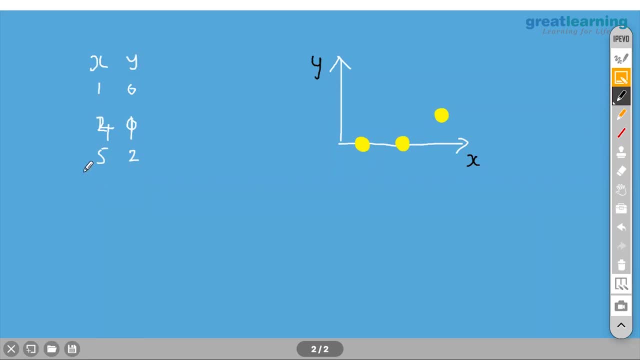 X because y has got couple zeros. Okay, So now, keeping this concept in mind, Tell me which dimension has more variance, which dimension has less variance? Which dimension has less variance? You remember variance in structure. Yeah, X has got more variance and y has got more variance. 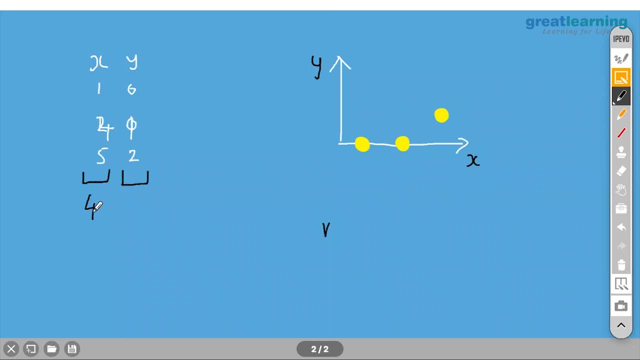 did you ever think of four variants? four here, five minus minus four. two minus zero is two, correct. now can i say: the two is nothing but a subset of four. if i say variance two, if i say variance four, can i say this is a larger curve. 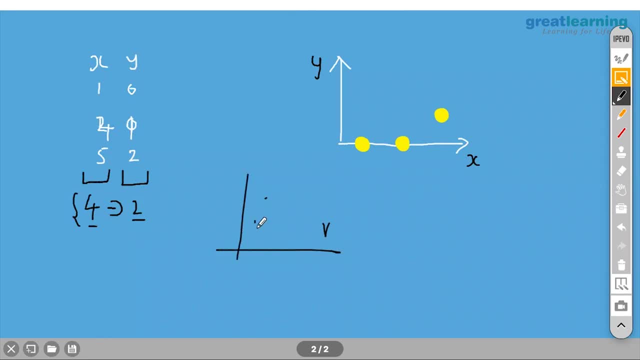 this is a smaller curve, or this might be a more scattered data, and this might be a less scattered data, this one. so it's going to lie anyway inside the larger data. if we talk about variance plot, don't confuse it with this plot. i'm talking about, currently, the variance plot. 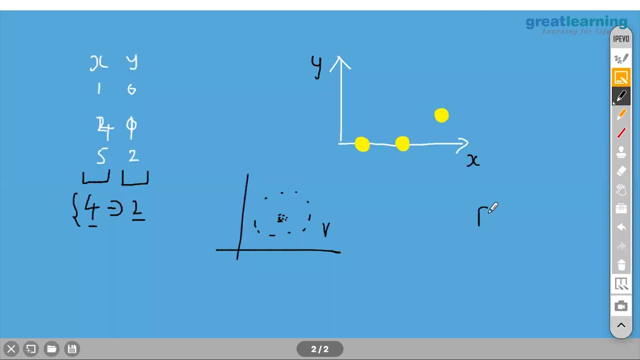 yeah, okay. so it's like a data scientist and a data analyst and a data visualization guy. can i say: data scientist is a subset, so basically data analyst and data visualization guy will be a subset of ds anything. so the scope of the data visualization guy is a subset of ds anything. so the scope of the data visualization. 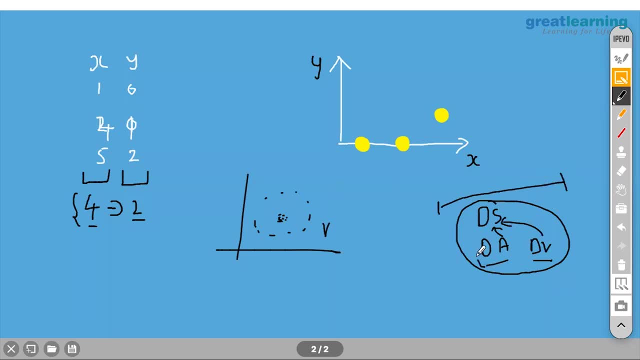 of knowledge, what data scientist has has more as compared to these two. so now can i say: if i have three people in my team, it's okay to release one of them, just in case. okay. in a similar manner, what i will do is i will plot a covariance matrix. now, what is a covariance matrix? is very simple. 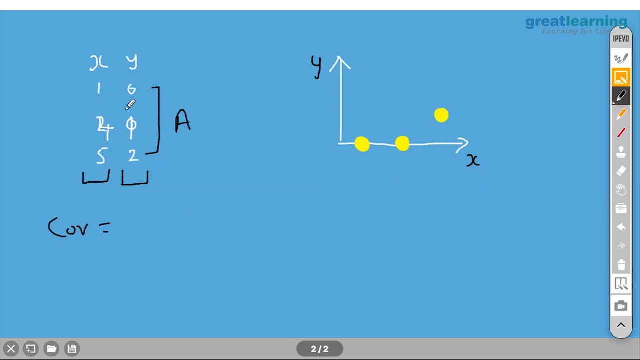 let us say we call this matrix as matrix a. it's a three cross two matrix, okay. a covariance matrix is a multiplication of a matrix with its own transpose, yeah, so what are we going to get? we are going to get a matrix. what should be the size of it? three cross three, okay, and any idea. 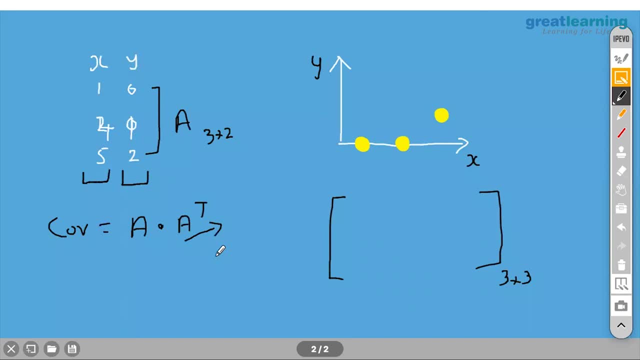 why did we transpose it, guys? i want you guys to understand covariance. that's why i'm going little deep into that. what is the dimension of this? yeah, three into one. yeah, if i multiply the same one, will it get multiplied? no, no, i need two here. so for that reason, i'm 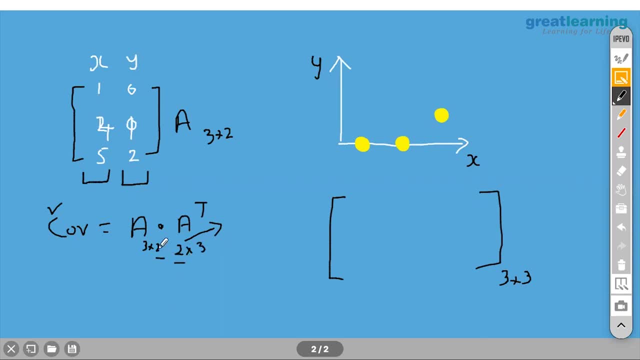 transposing as simple as that. sometimes even we ask this as a question: why? why we transfer the covariance matrix? why we transfer the original matrix in covariance. okay, so this is the only reason. now, when i do that, the answer will be: we are going to get a matrix. okay, so let us say this: 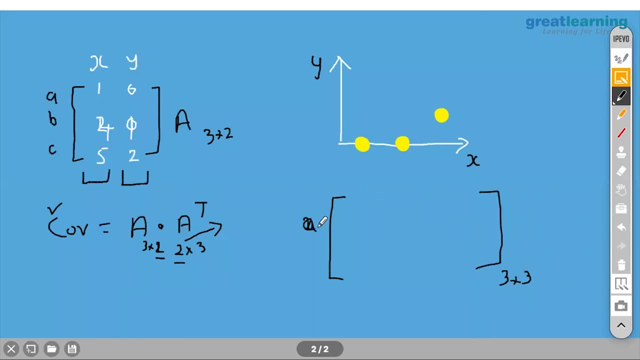 is feature number a, feature number b, feature number c. so we are going to understand a, b and a, c, a, b and c. we are going to get a relation: how a behaves with a, for example, how a behaves with b, how a behaves with c. like that we are going to get a whole matrix. and if you look at the diagonal, 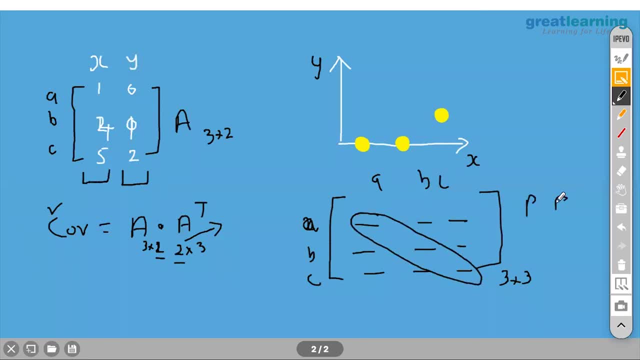 elements. it is similar to a pair plot. if you remember your pair plot or heat map, the diagonals always will be represent because they are 100 similar. so there will not be any change here. the triangle will be the same. so we are going to get a whole matrix and if you look at the diagonal, 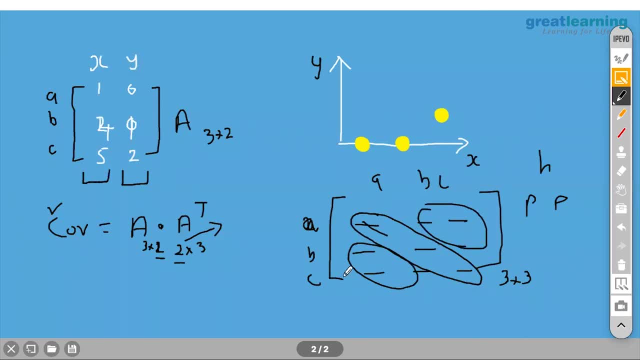 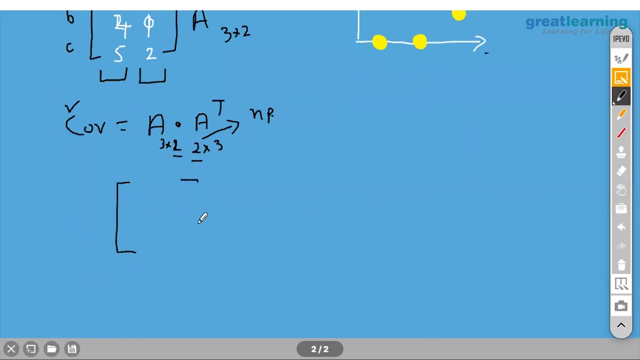 on both the sides will be your original matrices. now this is your covariance matrix. so this is how we generate it. now python, or numpy, basically has a capability of dividing this covariance matrices into two more matrices. what are those matrices? the first matrix and the second matrix? the first one that we get is called eigen values. again, remember, guys, this eigen eigen thing. what? 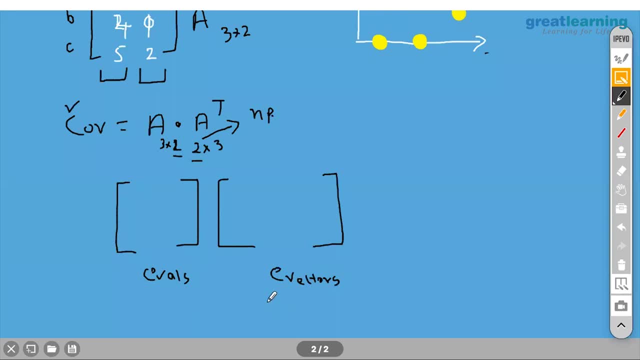 i'm talking about now. this is also too much misinterpreted on web, so please do not follow anything else except this concept: eigen values, eigen vectors. what are eigen values? eigen values is the variance captured by the dimensions. okay, so in this case i will write four into. we will modify this, just for understanding. we are doing this. later we'll come. 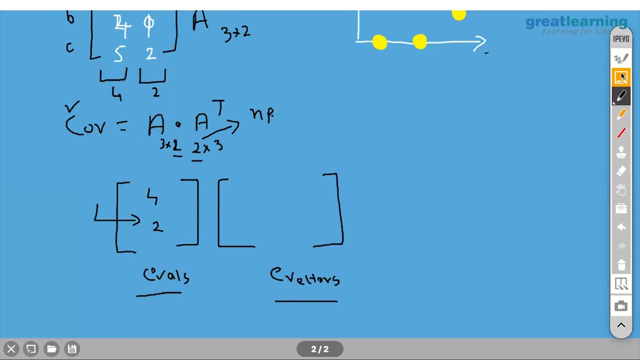 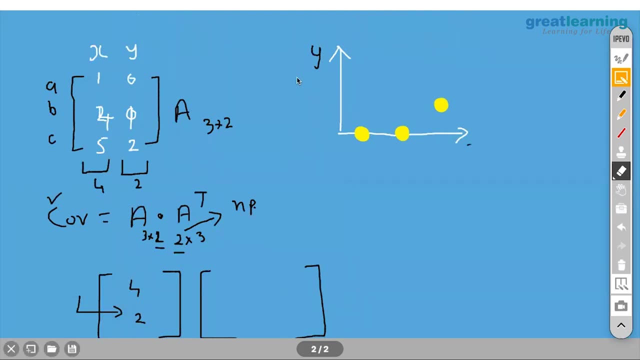 and modify this also. next, what are eigen vectors? eigen vectors are some matrix. it's like: what if i remove y, for example? if i have removed y, what will be my points? my points will come and sit on the axis. what if i remove x? what's going to happen? my points will come and sit on the axis. so what are we? 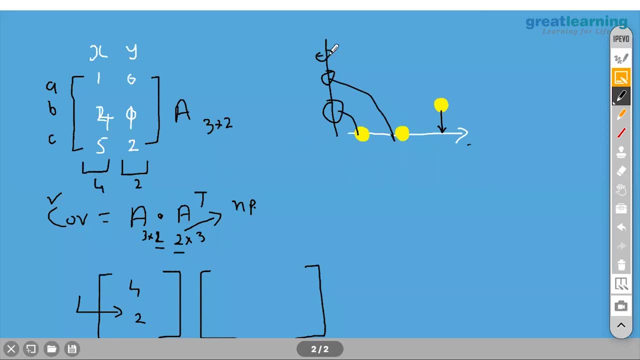 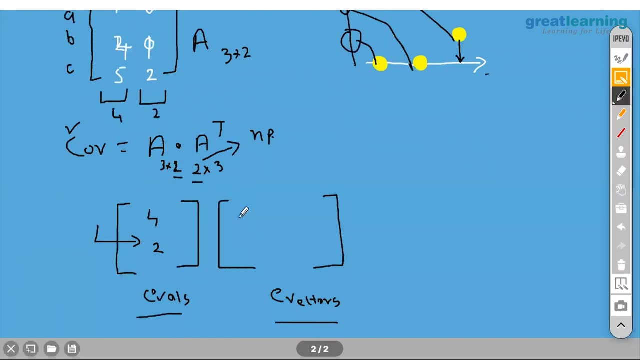 doing now is we are trying to understand the correlations between the points from the covariance matrix. so eigen vectors will be the lone points which are left out. if one of the dimensions was deleted, guys got it. values is nothing but your variance or standard deviation vectors is nothing but the 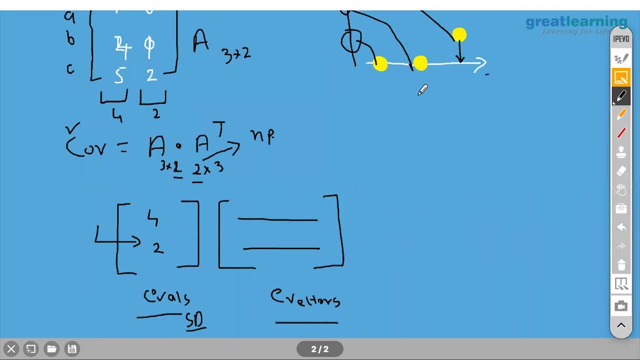 points. if, in case one of the dimension was gone, what is the remaining points? if, in case another dimension was gone, what were the remaining points here? we have got two dimensions, so we have got two rows. okay, simple, right? so covariance matrix can be splitted into two rows. so we have got two rows. so we have got two rows, so we have got two rows. 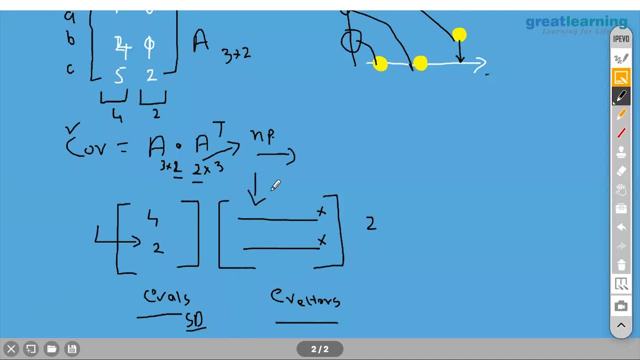 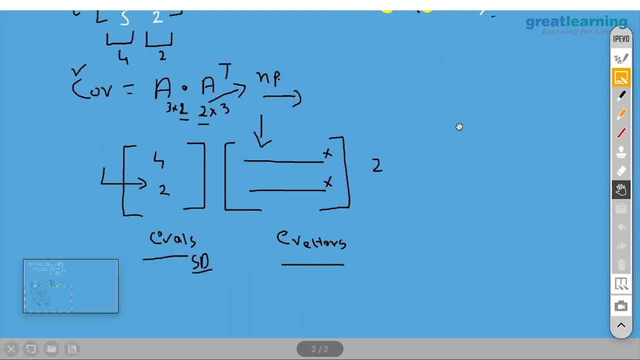 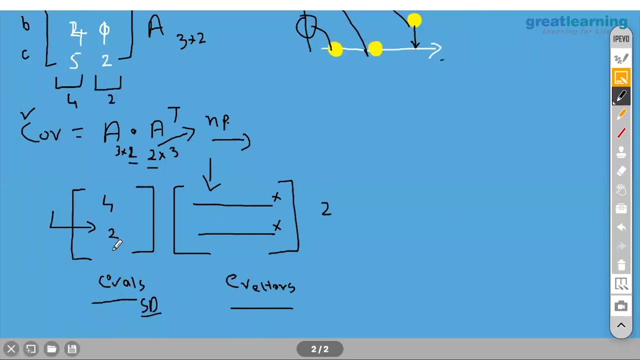 these two. how numpy takes care of it. we don't have to take a headache of it. okay, now. next, why did, why do we do this now? now somebody can ask me: okay, why do we need values and vectors now? first thing is, i have written here four and two here just for your understanding, but actually, if you have two, 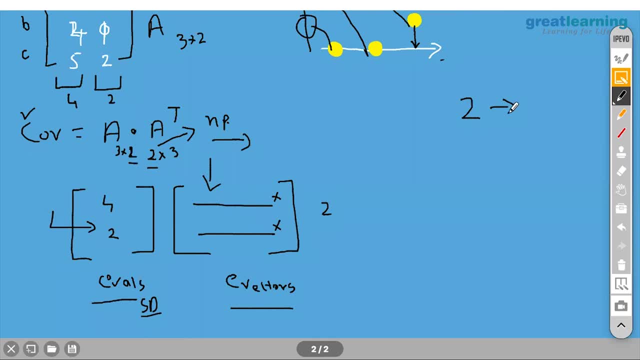 dimensions. the total standard deviation or variance captured by your data set will be two units. if you have three dimensions, it will be three units. if you have four dimension, it will be four units. please remember that in this case it will be two units. so if you have two units, i cannot write four and two here. it makes no logic. 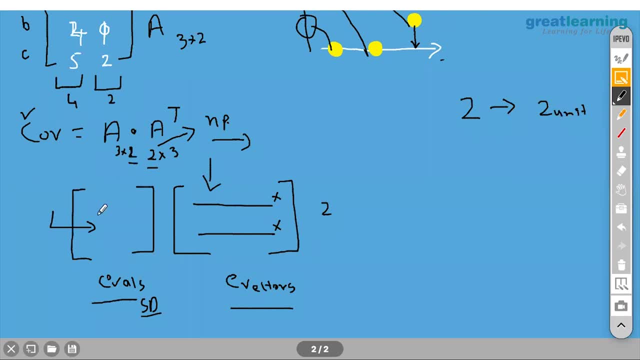 so what i will do is i will write in terms of units. i will say the first dimension. so out of the total variance captured is six. four out of six is the variance captured by the first one. two out of six is captured by the second one. so let us say four out of six is around 0.8. 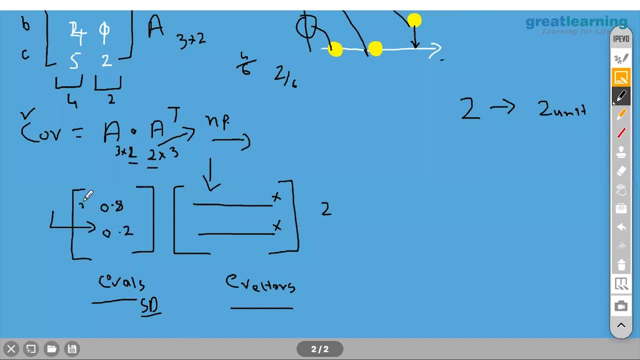 and this is 0.2. so this is refers to x-axis, this is refers to y-axis. now can somebody tell me which axis is. okay, sorry, this is 1.8 and this is 0.2. now can somebody tell me out of two units. 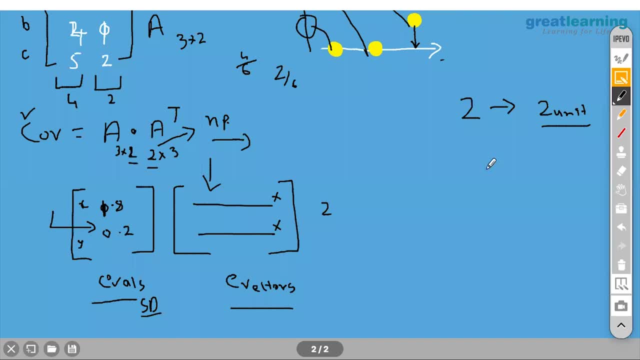 which axis gives me the maximum variance. i will say x-axis. so we can say we will remove y-axis. we can say it's okay to remove y-axis. yeah, i'm not deleting it. why? this is just to take a decision that which of these axes are not important. so in 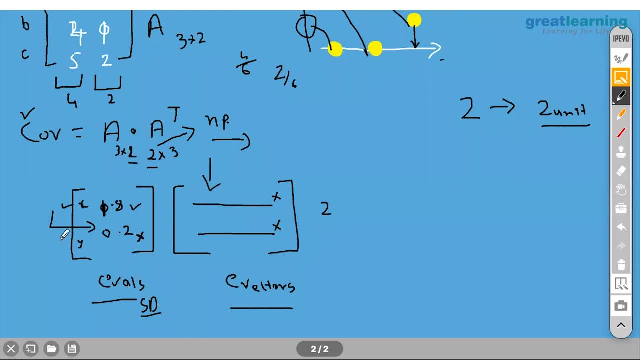 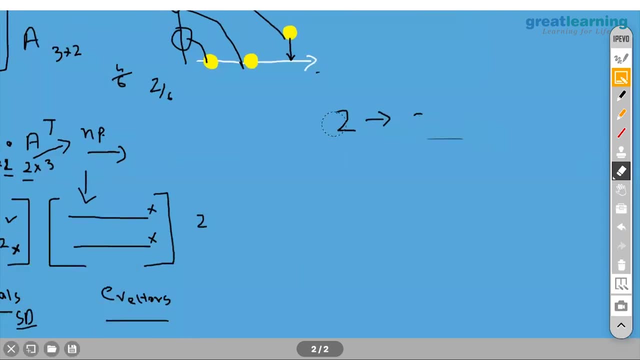 this case i will say: this is the axis which is important. this is not that important. now coming to eigen vectors. now, what is the use of this one? so what if i plot my covariance matrix? so let us say, this is my covariance matrix axis and i'm trying to plot them. so let us say my plot goes. 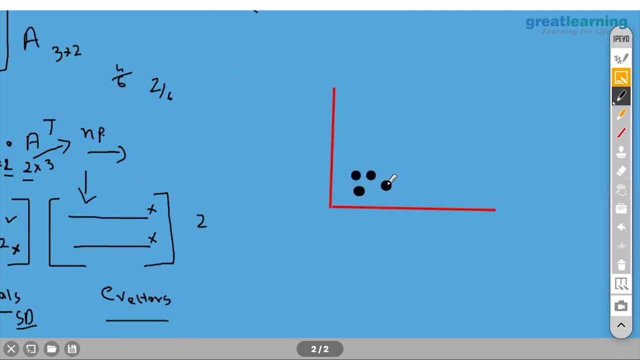 something like this: okay, let us say: this is my covariance matrix. now we are supposed to create new dimensions here, so let me make it together. let us say this is one dimension, and let us say this is one more dimension. is there any other dimension possible? no, why? because 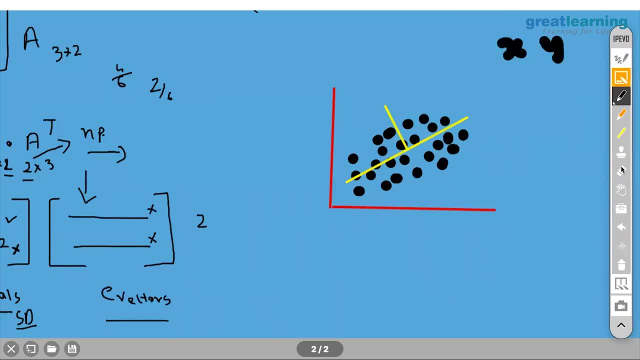 we have only two dimensions: x and y. yeah, now can somebody tell me- let us say i will call the horizontal dimension as principal component one and this dimension is principal component two. yeah, can somebody tell me which dimension captures majority of variance? guys, simple, look at this dimension and look at this dimension which captures more variance. 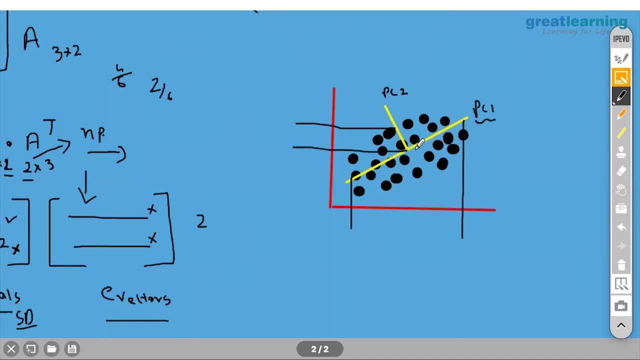 can i say: yeah, so like we'll not say x and y, because this is excellent. now we are transforming our dimensions, we are visualizing it in a different way. so now can i say my new dimensions are pc1 and pc2, for example. okay, so can i say pc1 captures majority of variance, pc2 captures minority of variance. do 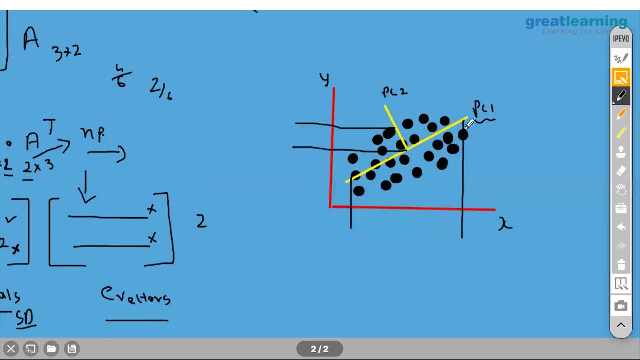 you agree? yeah, yeah. now, in this case, you people know this is x and this is y, so that's why we are doing it. but from now, when we transform the dimension as per covariance matrix, we will not call it x and y, we'll call it pc1 and pc2. okay, pc1 captures around 1.8 units. 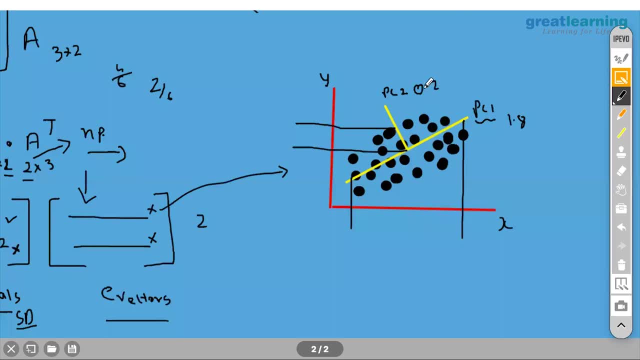 pc2 captures around 0.2 years. so now i can say that it is okay if i reduce this dimension. okay, i will ignore this dimension. and what are this dimension? this dimension are these points? i will say: in future i will ignore these points. second value: i will consider only my first. 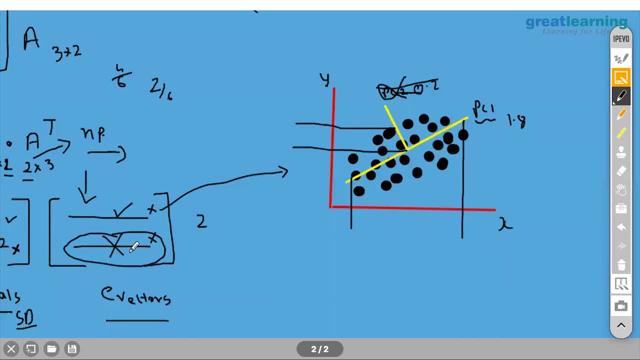 set of vectors. yeah, now, what are these vectors, guys, combination of x and y. agreed, yeah, they are covariance matrix. they are not a single dimension. this is a hybrid dimension. so, logically, i am not removing y yet i am removing y. got the point? yeah, or please tell me frankly. if no, if you are still. 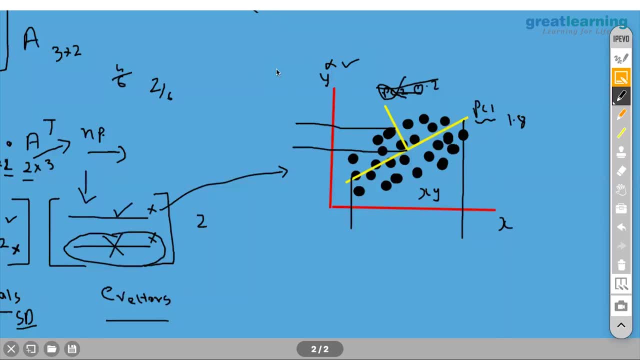 confused. it's very. yeah, verify this one. yeah, if you can just explain it quickly over again. yeah, yeah, see, we are comfortable plotting x and y. so when we plotted it, you guys were okay with it. nobody like asked the question in that side. we know how to do a 2d plot, but now what i'm plotting is i'm not plotting our x and y, i'm plotting our. 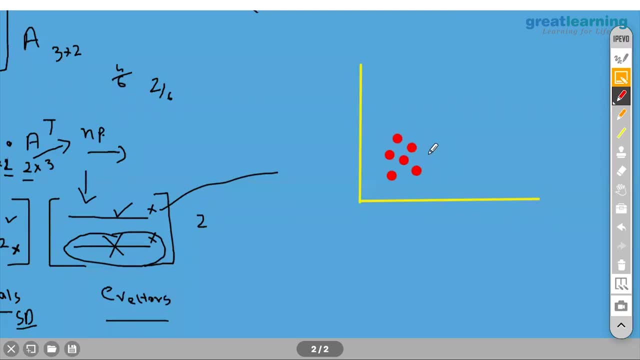 covariance matrix. okay, so let us say my covariance matrix. when i did it, i got a curve like this or scatter plot like this. sorry, not a curve, scatter plot. okay. now ignore these dimensions, delete these dimensions visually and say that i will put my own dimensions here, which i will call some dimension this side and some dimension this. 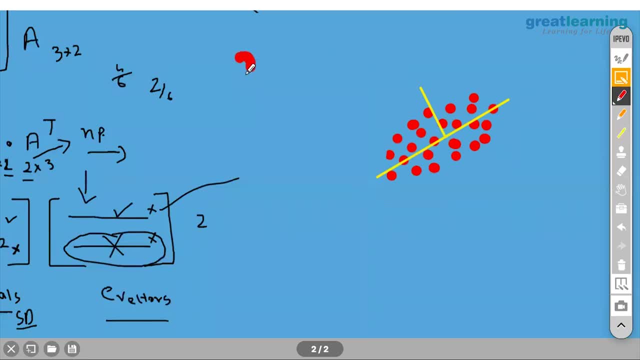 i will have only two dimensions. why? because, logically, we have only two covariance matrix points, which is x and y. clear so far till now. yeah, yeah, see the way we transformed our dimensions in and it's way more close to ourselves. so actually, i am going to put my origin data later in the 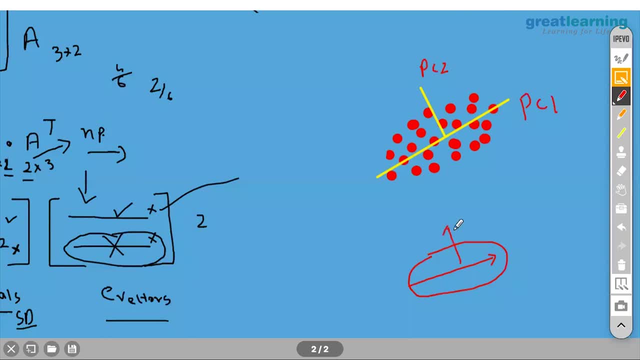 session. okay, okay, way which is giving you more information? can i say the one which i have put it on a horizontal way or kind of horizontal way gives you more information. yes, or it's okay. let's forget that example. what is the dimension pc1 or pc2 which gives you? 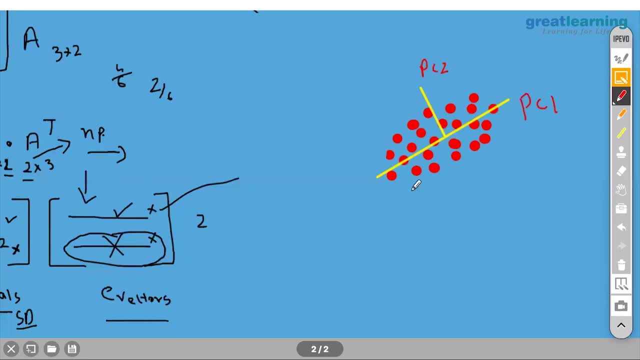 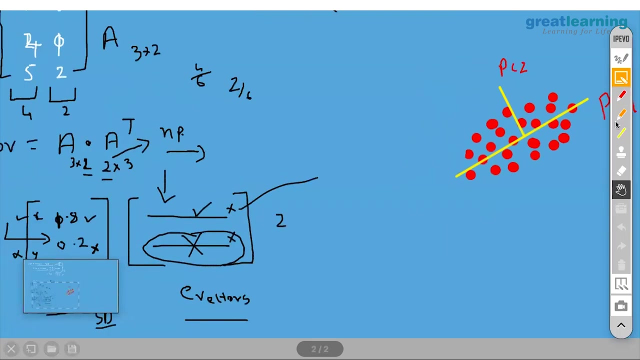 a variety of data. who is having more thickness? pc1 is having more thickness or pc2 is having more thickness? guys, pc1 exactly. so pc1 is a new dimension. okay, pc1 is a new dimension which is capturing majority of the variance, and pc2 is again a new dimension which is capturing minority. 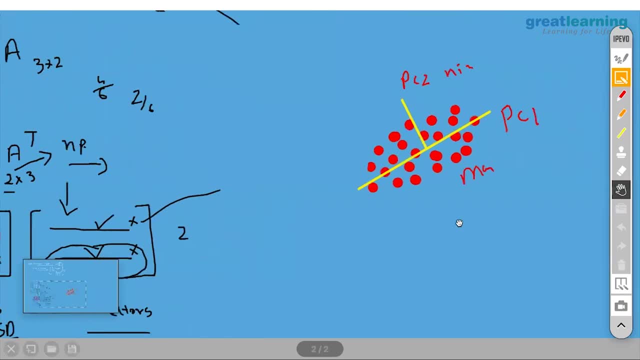 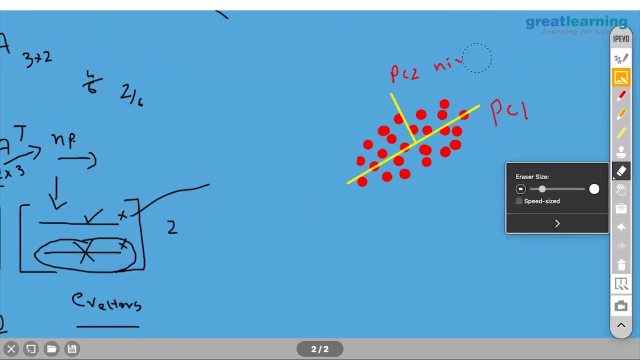 of variance. okay, so now, if i ask you guys, if you are given a chance to remove one of these dimensions, which one you will remove? obviously pc2, pc2, so exactly, so, virtually, i will delete this. okay, now, when i delete this, what is going to happen? if a point is here and if you remove one of the dimension, what's going to happen? 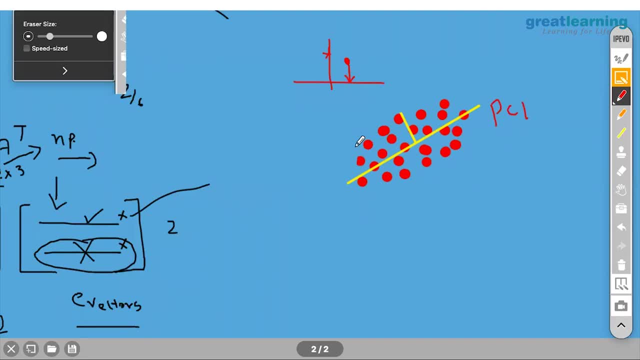 the point will come and fall on your original axis. so this fallen points: when you delete pc2, the fallen points are the points which we have given as eigenvectors. so if i would have deleted pc2, this is my eigenvector. if i would have deleted pc1, these are my eigenvectors. got it okay? so these are okay. yeah. 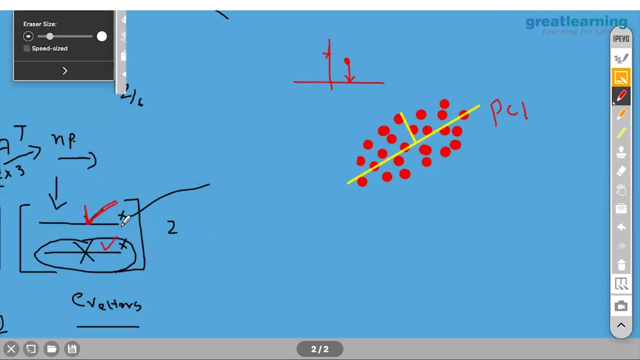 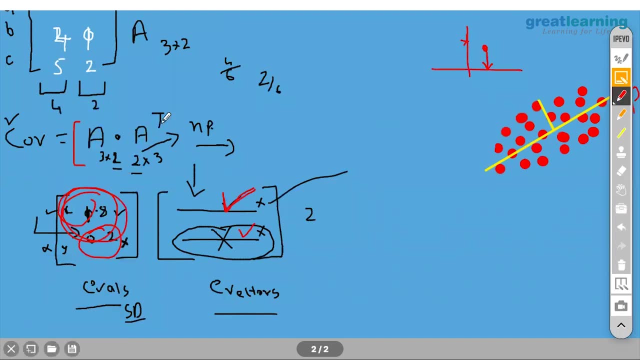 okay, but how did you compute this? the covariance bit right? the? how did you do that bit? yeah, the covariance matrix. yeah, the covariance matrix. and the, uh, the left eigenvalues, right. so how did you get that? so that, yeah, the statistically numpy will help us to do that mathematically or manually, we can. 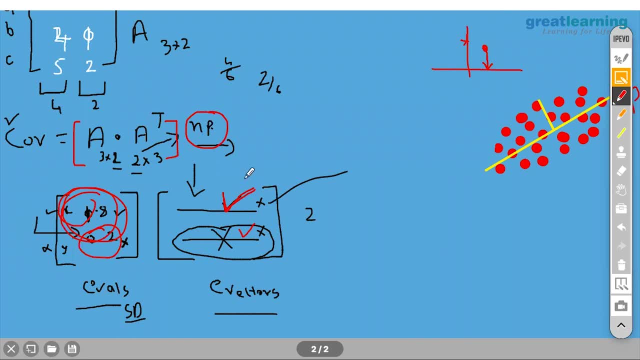 not, we do not have that much power, okay, okay, very frank. so we have got a ready-made library in numpy which divides our eigenvalues and eigenvectors. so are the a and a transpose right? so a is the a. is both x and y put together, is it? yes, so that's the okay. 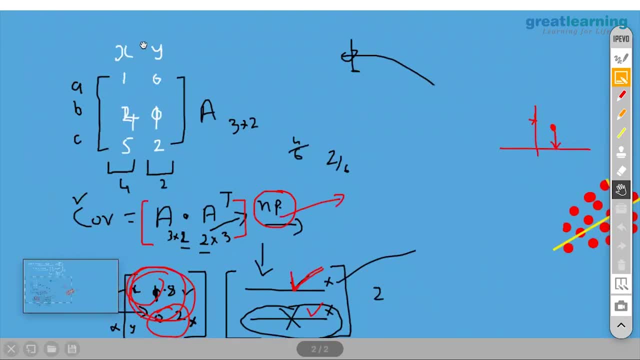 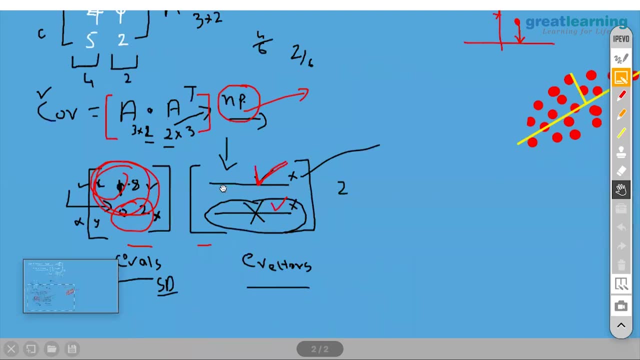 okay, so i have shown you two dimensions so it looks simple. but imagine if you have 150 dimensions here. what will be the size of covariance? so so 150 dimension would be what uh, a in the a transpose plus b into b transpose, or just one, one matrix, only one matrix, one matrix. 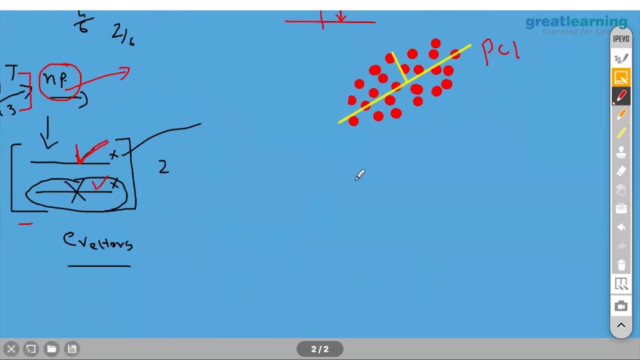 some, uh, 50 by 10 000, something like that, exactly. so imagine, this is your data set. you have 150 dimensions here. that means 150 columns. here each column is a dimension. so in that your new matrix will be a square matrix, 150 cross, 150 covariance matrix. so here you are going to get 150 different. 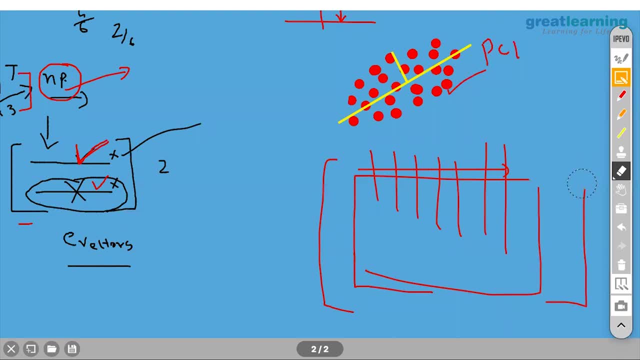 dimensions, okay, yeah, good, so guys give yourself so. so, so this, all these uh dimensions, the new dimensions that comes by, they're all hybrid dimensions, hybrid, exactly, virtual ones. we cannot see them or even we cannot plot them, to be very frank, okay, okay, and we do not know which one, what? 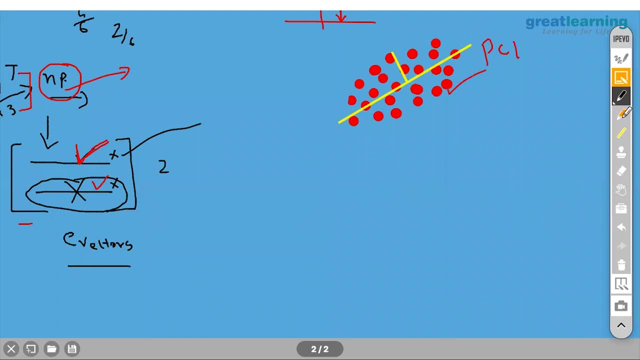 is the importance? what is the ratio? it's just takes all the 150 dimensions, create hybrid uh dimension, and we also specify how many um uh dimensions we need to bring in the matrix. so we're going to do that, we have to do it, we have to take a decision depending on these numbers here. 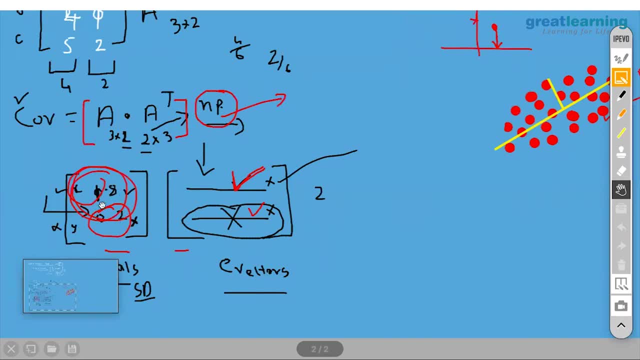 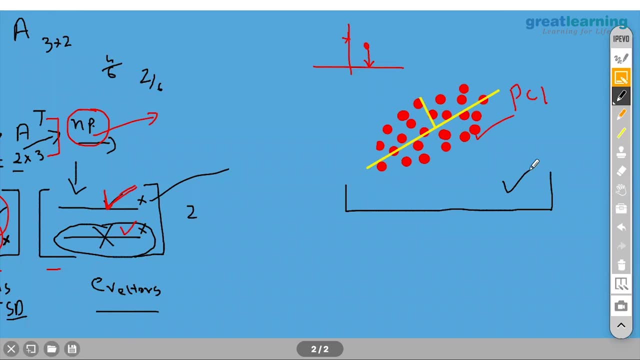 so i'm going to come to that anyway. the next point is this one: yeah, so whenever i showcase these dimensions, no people get a little confused. so now are we okay with this virtual dimension? okay, so the covariance that we saw is a bivariate, is a multivariate covariance. 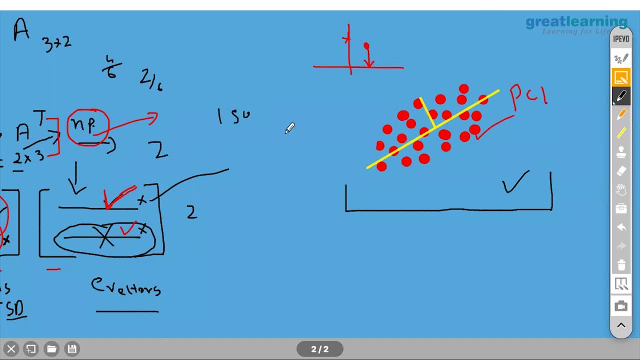 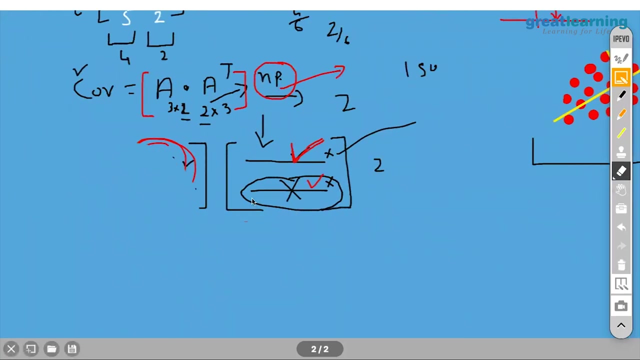 in this case it is bivariate. in 150 case it will be multivariate. okay, yeah, okay, okay, yeah. so we'll add to this again. um, my last bit, the last trick is on this. so now, let's okay, two eigenvalues. now how do we choose which dimension to take and which we wanted? so let us say, rather than saying, we have 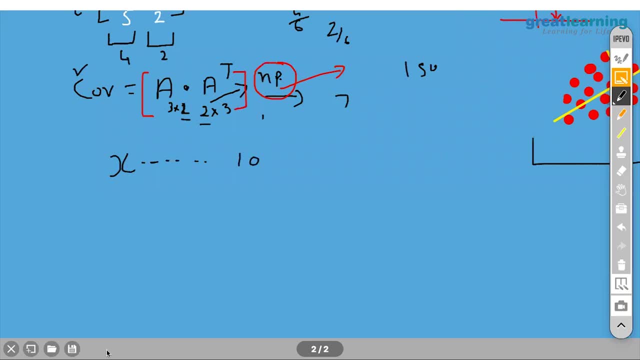 x and y. now let us say we have got 10 dimensions, for example. so if we have 10 dimensions, what will be your total variance? 10 units. okay. what does that mean is, when you generate a eigenvalue vector, your answer will be 10 total. as you saw in the previous example, i did 1.8 and 0.2. when you add it, 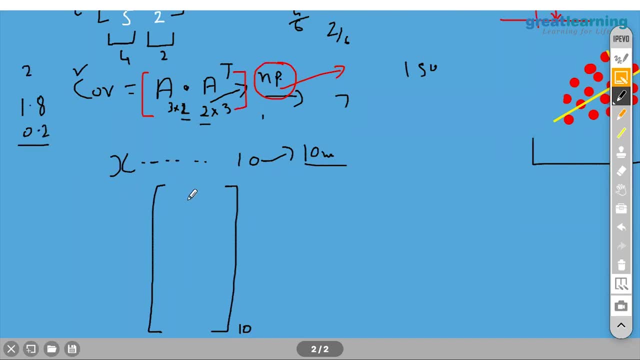 up, you will get 2.. okay, so let us say the first pc. so i will say: rather than 10, let's not complicate, make it 5.. yeah so, pc 1, principal component. 2, principal component. 3, principal component, 4, principal component: 5.. let us say principal component: out of 5 units generates 3.4 units of. 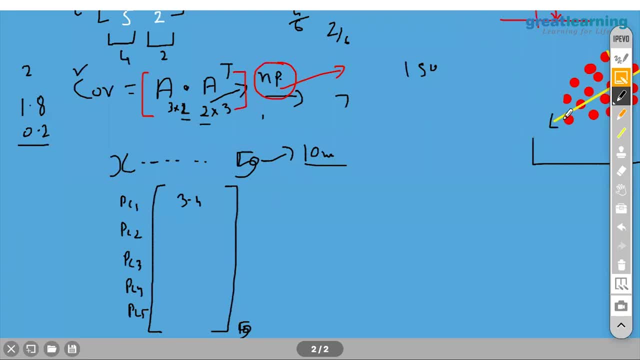 that means this one, the first one, okay, principal component 2 might be 1.2. so the total is how much? 4.6 and 0.2, that is 4.8. 0.15, that is 0.95 and 0.05. so when you add this up, the total should be 5 yeah. 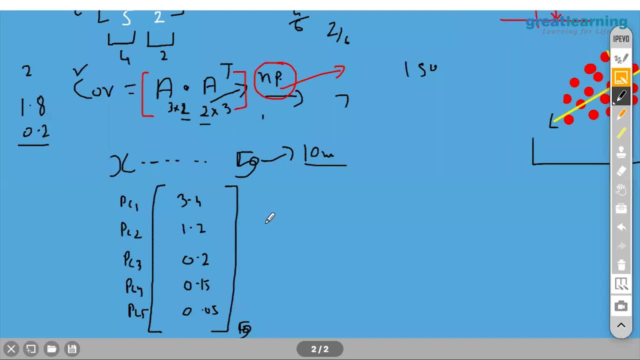 so that numpy will take care of it. we don't have to worry about it. now, what if your project says out of 5, if we can remove three dimensions at least? what if there is a request onto that? so how to validate this? you can go and add the first three principal components. so what you will get. 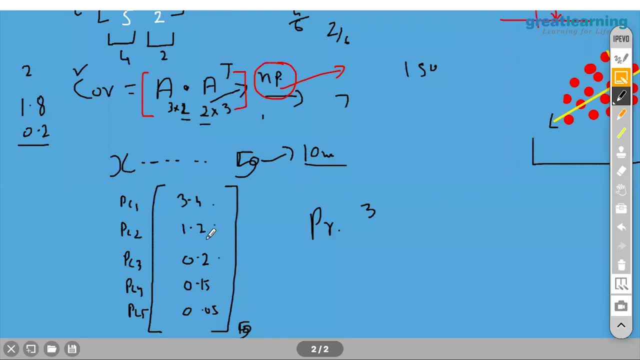 3.4 plus 1.2 is how much? 4.6 plus 0.2, 4.8, you have captured 4.8 units of variance out of 5. how much? it should be 86 or 87 percent, if i'm not wrong. right, yeah? 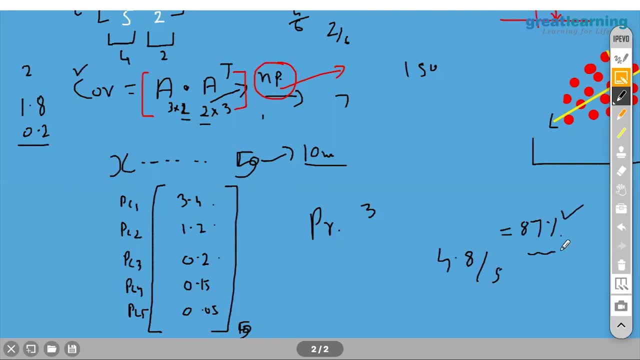 yeah, 86. yeah, if we are happy with this, if we are happy with this percentage, we can say that i am okay to retain first three and i'm okay to remove last two. how to remove and all i'll show you, don't worry about it. first we have to take a decision on. 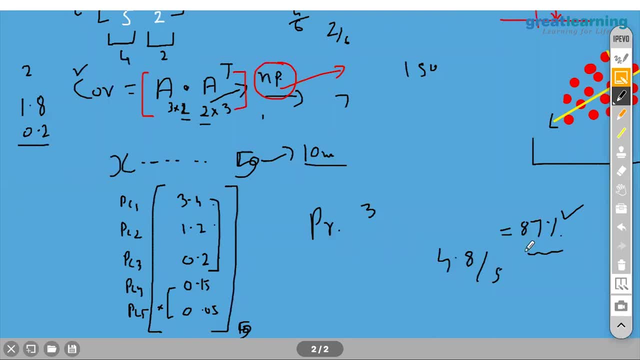 how many we need. so 87 for me is a good. so again, my suggestion is: anything about 75 should be good. what if you keep first two? first two is how much 4.6 by 5? this will also be above 80 percent for sure. so either you can retain first two or you can. 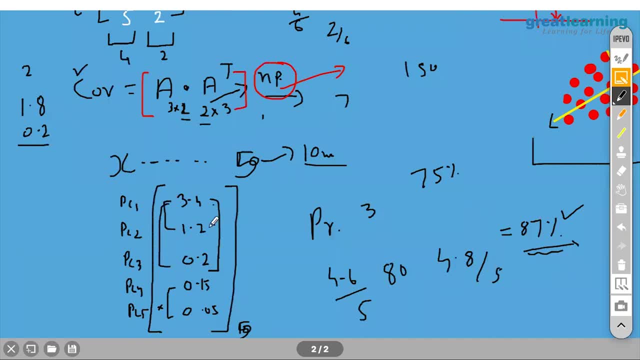 retain first three. the third one is not making much difference here if you compare these two numbers agreed. so this is how you take a decision. python will not, or no way numpy will give you suggestions. numpy will just give you eigenvalue chart. it is you who has to take a decision. 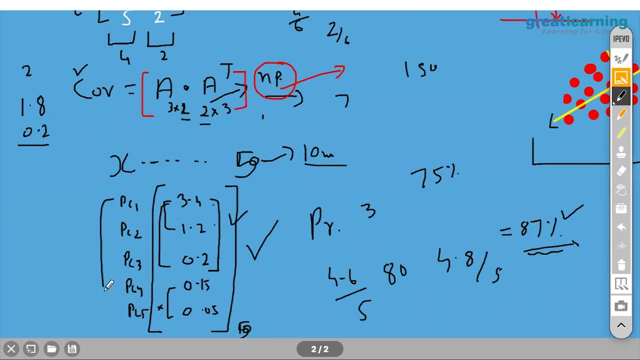 some people. what they do is, when they do this, they retain first four. now, logically, if you think these two are very low, so it's like doing all five together, there is no need to remove one. so it's like you're taking a bucket out of an ocean. so there is no meaning of doing. 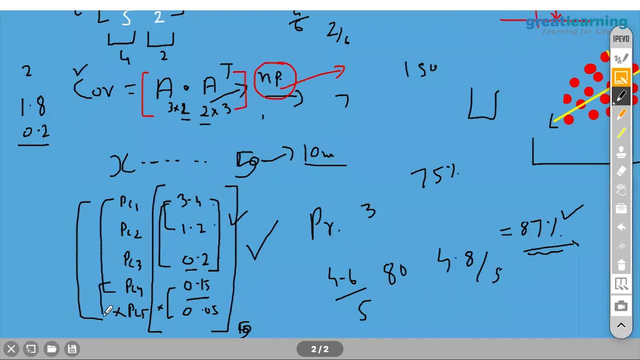 dimensionality reduction. at least try to reduce two or three dimensions, then it will make more impact on your computation time and complexity. okay guys, got it. so are we clear on how to choose how many dimensions to remove? yeah, yeah, yeah, it's a manual. we will get the matrices, so numpy is kind enough to give us the matrices from. 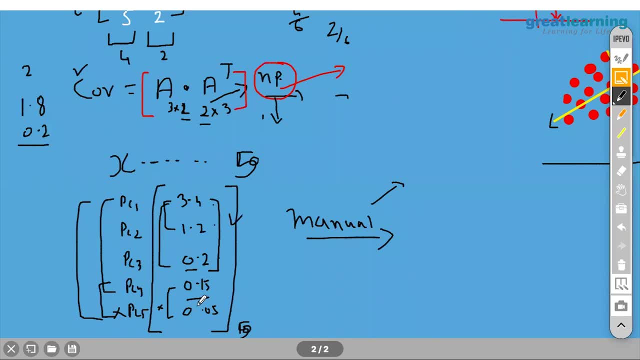 matrices. try to find out the values. okay, okay, primarily the eigenvalues, right vectors, vectors and value complex. yeah, okay, but vectors will make no sense to us because there will be some like our scaled data. if i give you a scale data like matrices in front of us, you can't visualize. 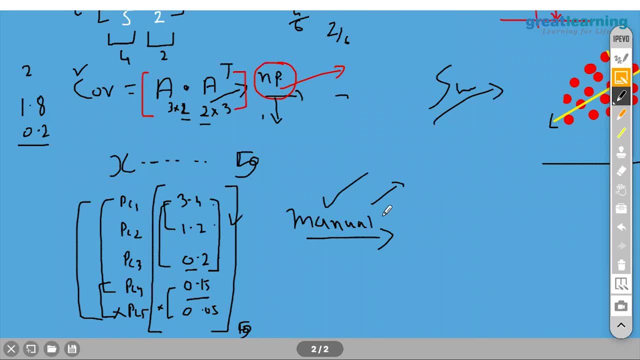 okay, yes, it's a manual task, i agree, but we can automate this. yeah, it's possible to select and automate, but again, why to do that? we can do it manually, like we can just add it up and select it. so this is the process of how to identify number of dimensions. now next question is how to reduce. 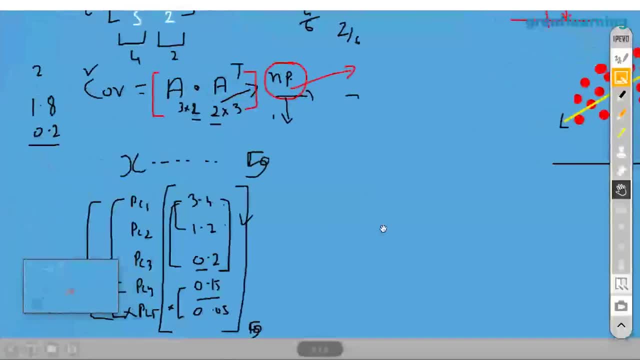 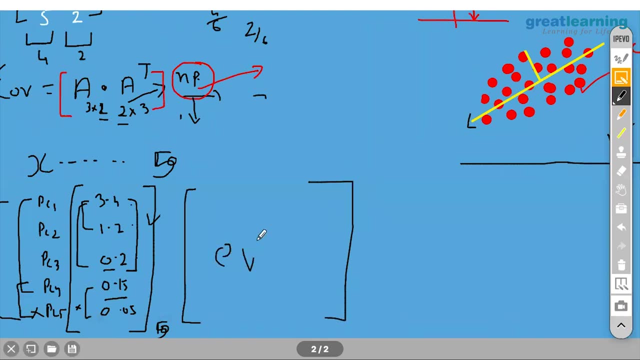 this now. we talked good, good things, fine theory, so basically it sounds very nice. now how do we reduce this? so let us say: we have got, this is our eigenvectors, this is our eigenvalues. now, from eigenvalues, we found out that we just need top three. 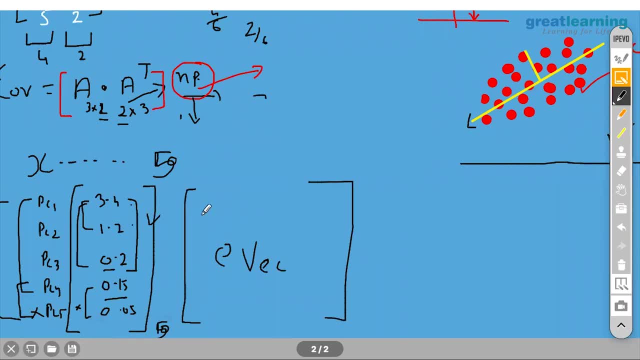 uh, features okay. so, as i said, pc1 eigenvectors, pc2 eigenvectors, pc3 eigenvectors four and five. so what are we supposed to do? we are supposed to ignore these two. so when you ignore these two, what will be your dimension here? three cross something. we don't know how many of them we have. 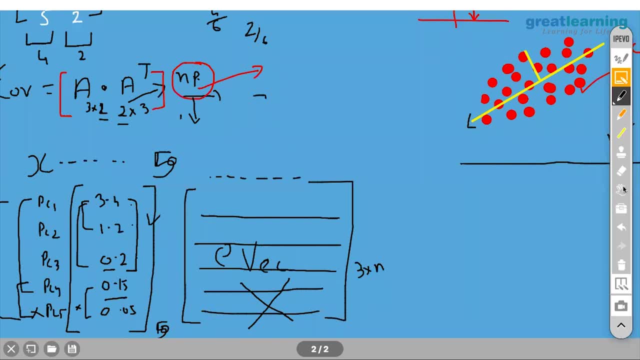 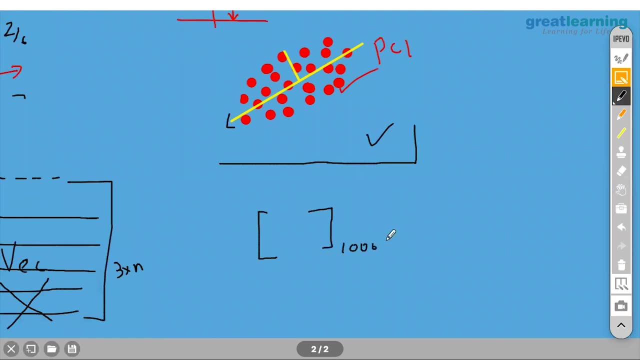 here, correct, okay, so now let us try to reduce a data set. so let us say your original data set is one thousand cross, five features, one thousand rows, five columns or five dimensions or five variables, whatever you say my answer. so i'm going to multiply something to it. 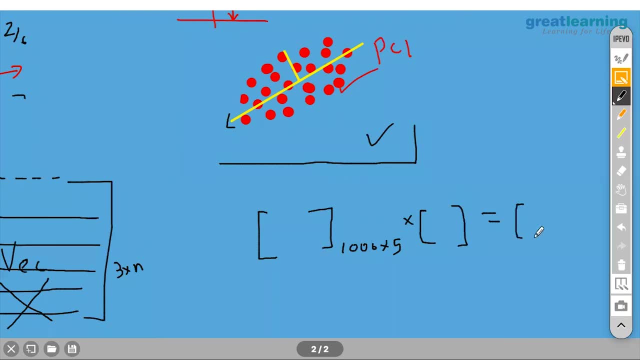 we will see what we will multiply, but my answer should be one thousand cross three, correct? that means i have reduced two dimensions, agreed. now i have only three dimensions, correct? now this is my eigenvector, basically. so what should i put here? what should be the size of my matrix? 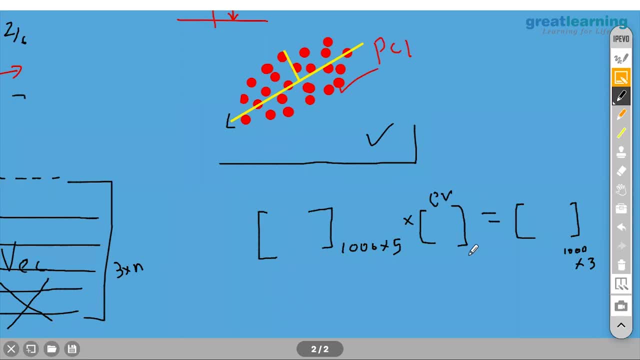 uh, it should be: uh, three, five cross three, five cross three. uh, this and this should match for multiplication, correct? so now this is my original data set, this is my eigenvector data set. so here, if you see this was five and this was three, what i could have done, i could have done transpose of it. if i transpose this, 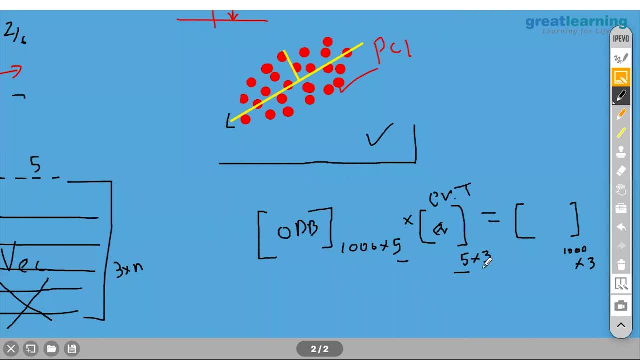 matrix, please, it is going to come now somehow. and my final answer. so this is how. finally, we can do it manually. we have to first find out this manually, multiply and annually we'll get a new data. and now you can use this data for your future analysis. it can be machine learning or it can go. 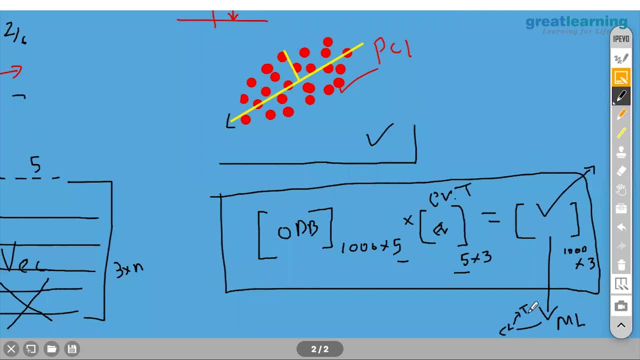 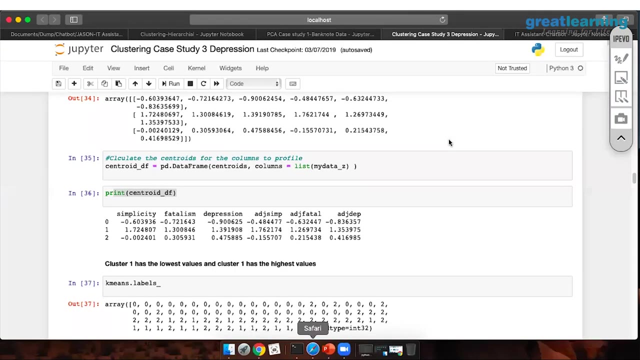 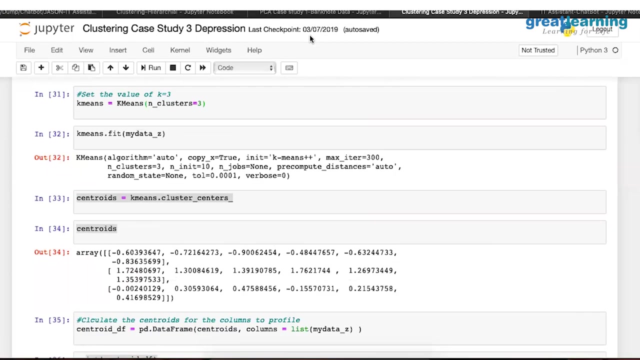 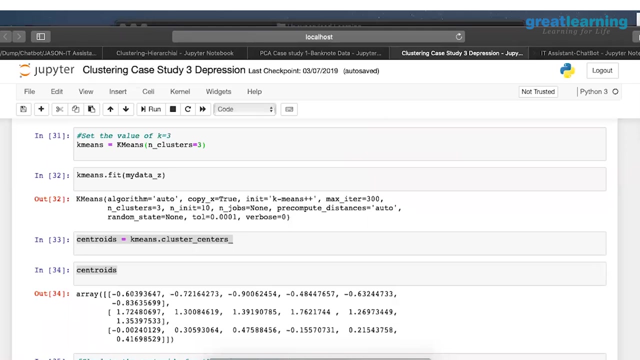 to clustering, to put target values- most target values. you can send it to supervised learning- anything you can do, okay, good, yeah, so now i will show you. anybody want to take a break? we might see this break and come back. okay, we want to continue. we continue, okay, so let me take up a pca data set. so now again, uh, before. 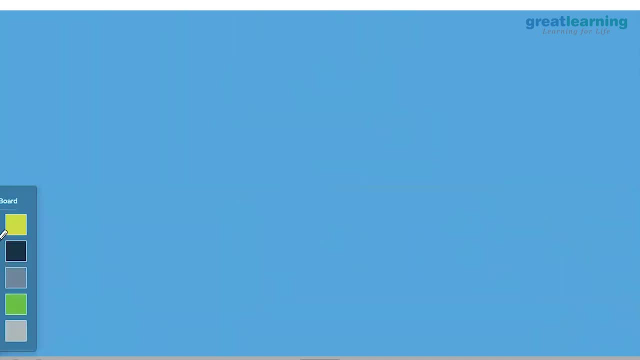 moving on. so just uh, pca. so one of the applications of pca is to do dimensionality reduction. okay, there are more applications to pc, so one of my personal application, or one of where i use personally pca, will be to generate some scores. so i will show you, probably this session or next. 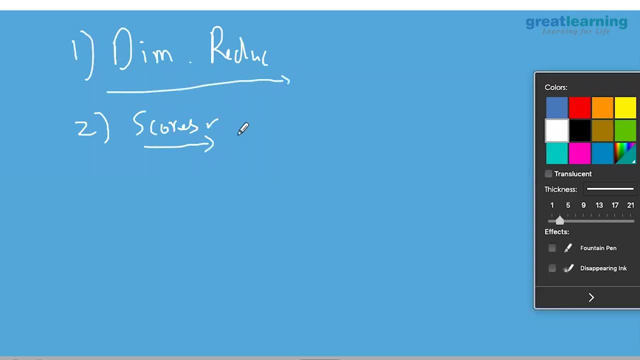 session. probably i think i'll show you next session- only become comfortable pca, then we'll go on to this. so please don't think that pca is only used for dimensional production. there is one more way we can generate some scores out of it. so it's like, if you remember, i said in clustering we 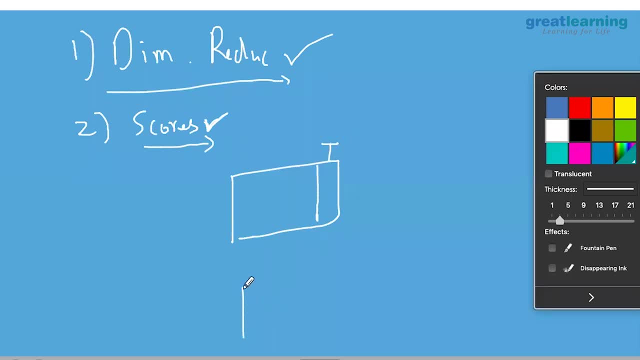 are appending a target with. that is that it a revolving Em Signal relay in the data set parties are target variable In PCA. did we append any target variable guys? No right, There is a possibility that we can give a score to each and every. Yeah, I'll show you how this. 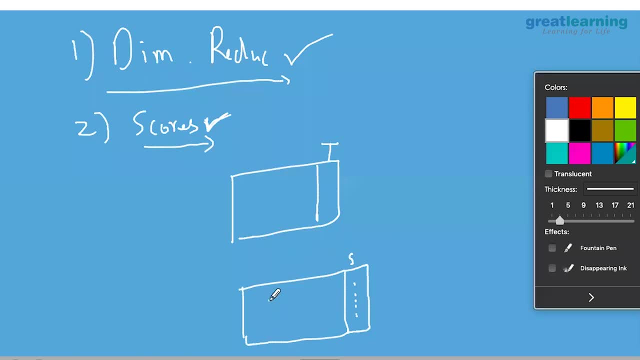 technique also, So I usually use this to rate my employees. So at the year end- now it's almost- we are down the road. When you want to, you have a bigger team and you want to equally rate your employees depending, covering all the important features and penalizing. 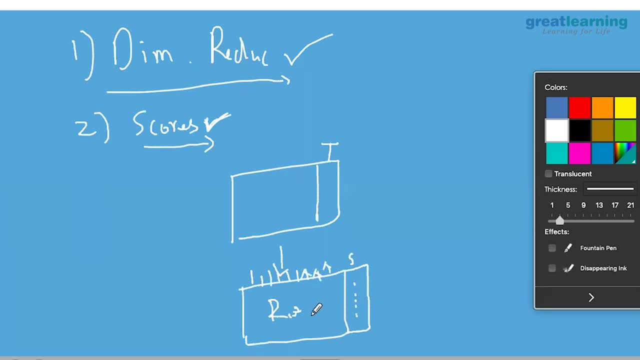 them on all not, or highly important, or non-important. In that case, we can generate a unique score out of this PCA technique. I'll show you down the line So and also I'll share it with you. Some of you want to use it for your teams. You can easily do that so that tomorrow they 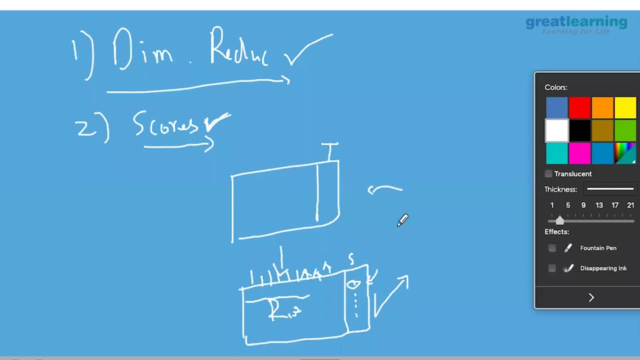 will not come crying saying that, okay, my neighbor has got rating. I've also worked the same. I have not got a good rating, Why You can directly pull out The stuff and show it to them. Yeah, Again, I will show it to you. So don't think that. 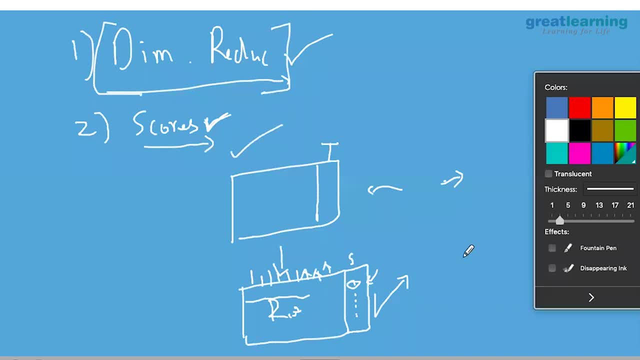 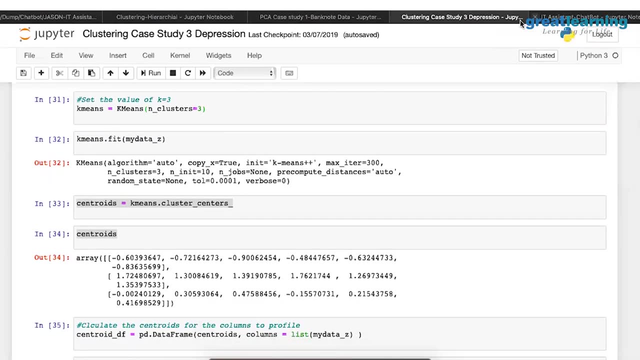 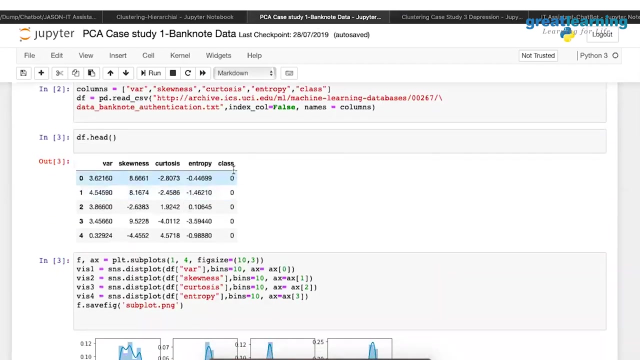 we have to do only dimension reduction. We can even do this. Now, moving on to the first example is how to do dimension reduction using PCA. Let us say I have gotten examples set here. Say I have got a data set where I have got a target variable. So definitely it's. 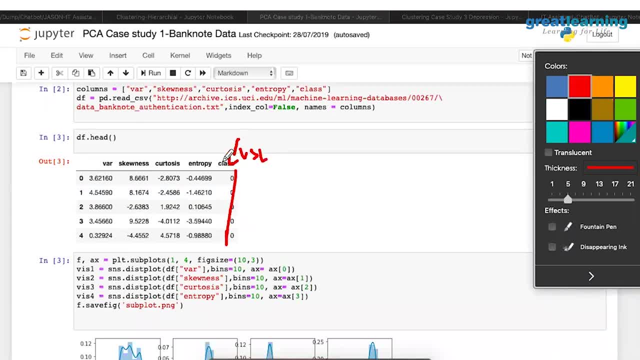 not a part of unsupervised learning? yet I am not. I want to ignore it for now. Not always necessary to keep it. I'll ignore this. I have got some attributes of a note, of a bank note, For example. these are some attributes that they have captured. might be the dimensions. 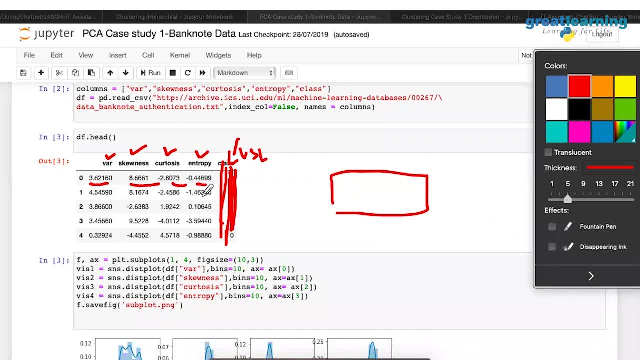 or might be some other chemical properties, or we don't know what it is. Let us say, these are some attributes And now the bank comes and tells me that we are not able to process all four of them. I want to plot it. What if you can give me a data reduction of two? 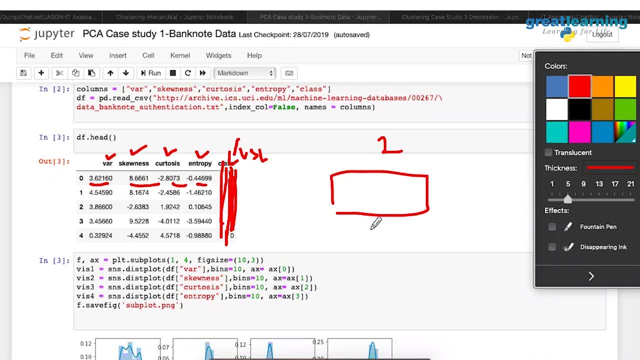 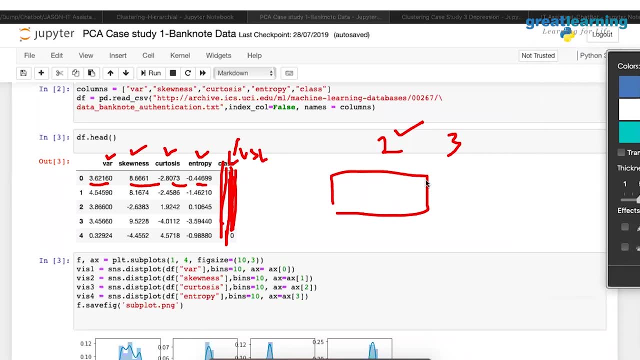 You can reduce my dimensions to two and show me how to plot it, or give us the best possibility. Even three should be okay, but try to do it for two, Okay. In this kind of case, what you can do is you can directly start with the PCA. Now, before you start with PCA, please, 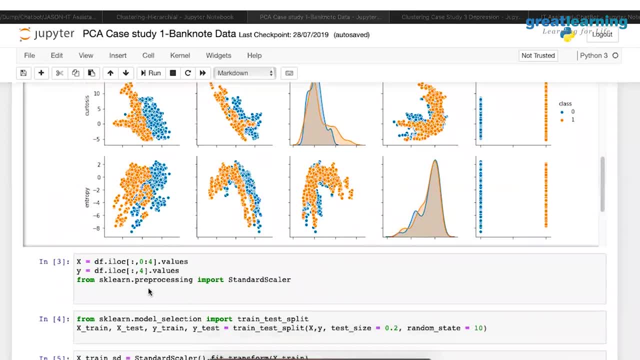 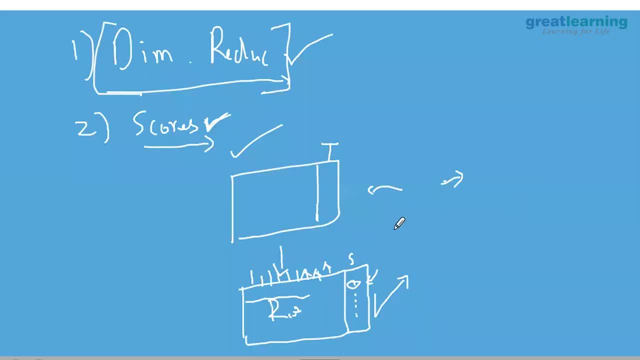 remember, we need to scale the data. So ignore the pair plot right now. We don't need it. The first thing we are going to do is data scaling Now. my question to all of you is now. this is again a debatable topic. 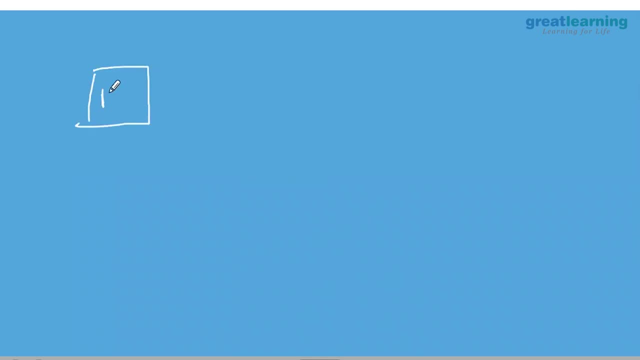 What we do is we have a data set. Okay, We split our data set into training, validation and testing. Now you guys are not exposed to validation yet, So for now you ignore it. We do the step on all the machine learning techniques we have done so far. Should I do? 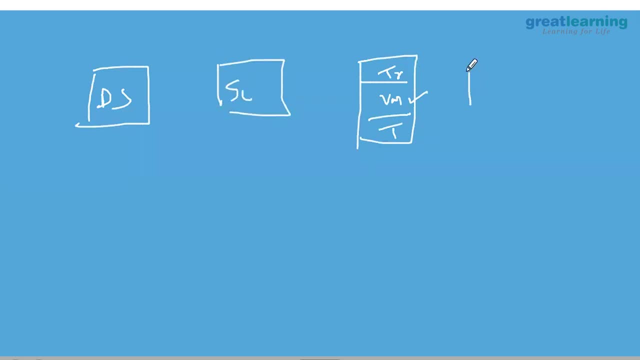 scaling here or should I do scaling here? Which is a better option, Before splitting or after splitting? is it Exactly So? what is it? What do you think is a better option? The first one, Okay. One vote on this. Okay. Anybody says here: See, try to think, Try to think what. 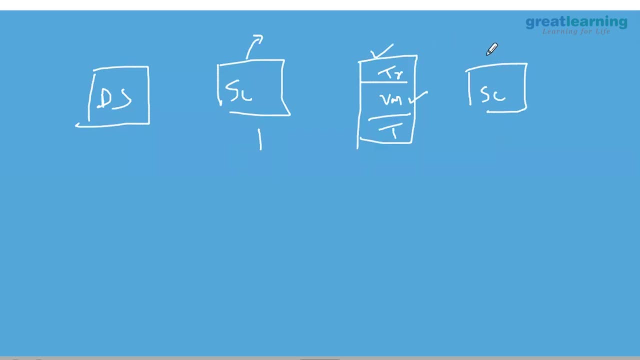 we do here. Yeah, What we do here And what we could do here. Just just give yourself a minute of time. See here. what we do is here. there are chances that we will have a scattered plot line When you split. 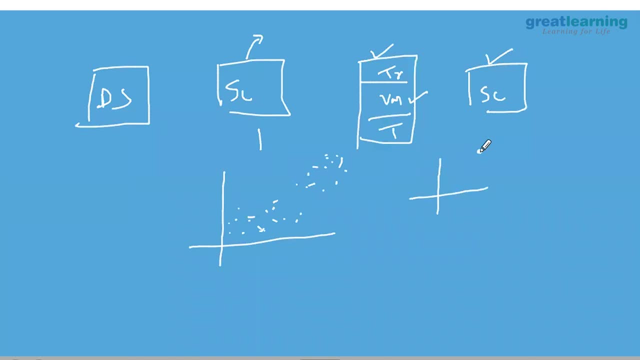 what happens? We might. it's possible that you will get this value in the data set. Even you will get this value. So we have no control over this, So we have no control over this. Okay, So we have no control over this. So we have no control over this, So we have no. 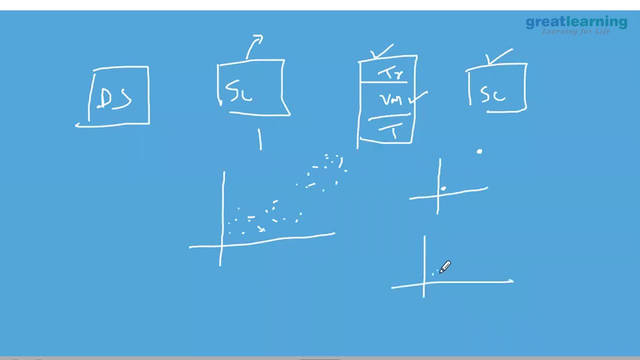 control over this, And sometimes there are chances that we may. we will get a cluttered data, But there are chances that we'll get a sparse data also. right, Correct, Yeah, So what are we doing, unknowingly, when we scale the data first itself? what are we doing? 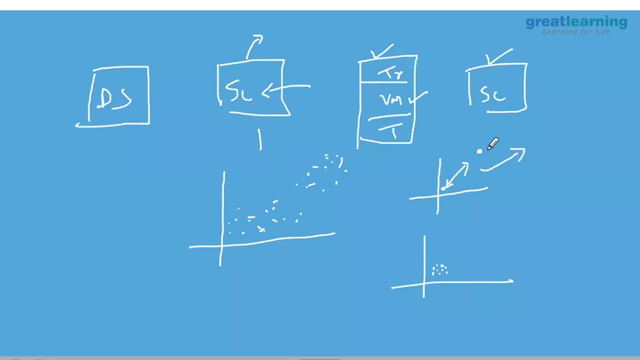 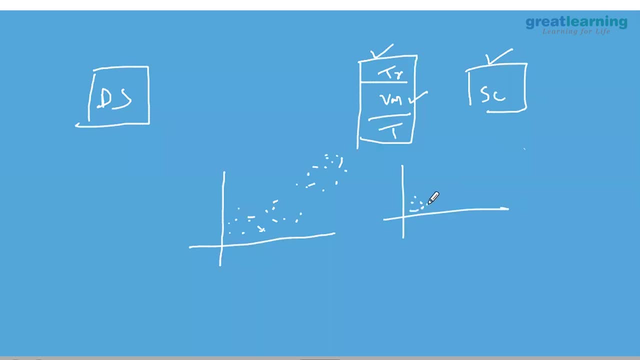 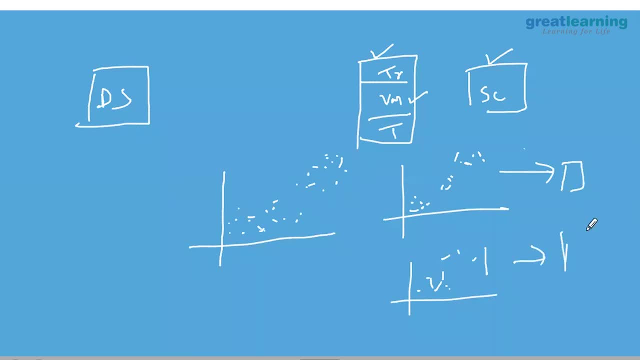 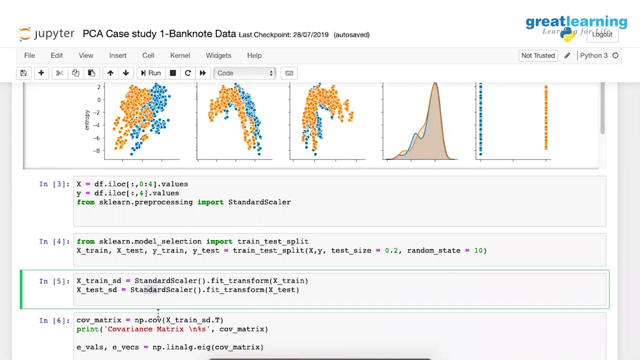 Put them through skin. What is going to happen? Yeah, Yeah, We can do this sometimes. If you are confident, data is not that you can do this technique- or if you ask me, which I like I am, I will recommend post test and train. split you individually, scale your test and train. 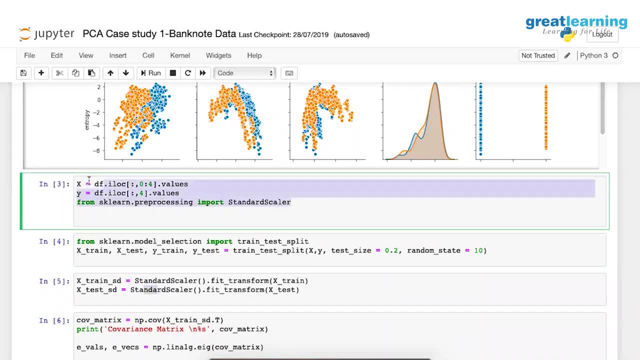 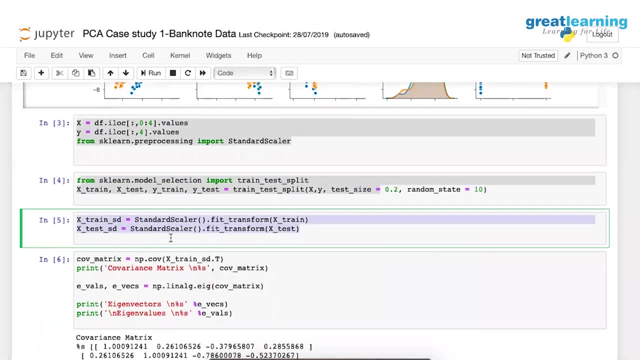 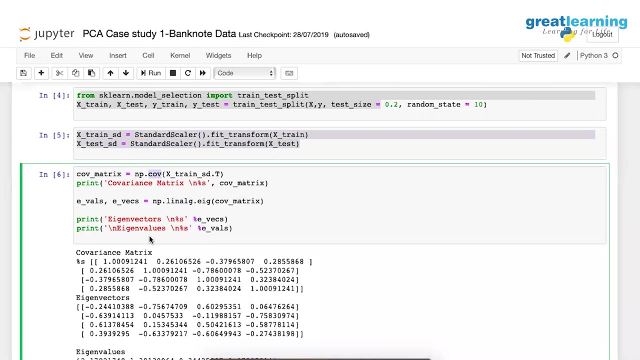 data. So this is my x and y, this is my splitting and this is my co-variance matrix. Post that very simple. directly generate a co-variance matrix. How do we do the NP co-variance On to what? On to your training data multiplied by, transpose Next numpy linear algebra dot. 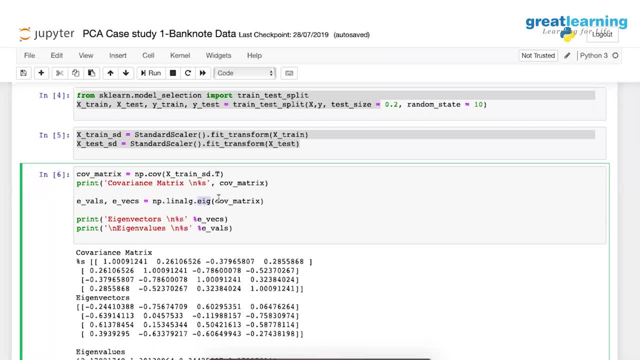 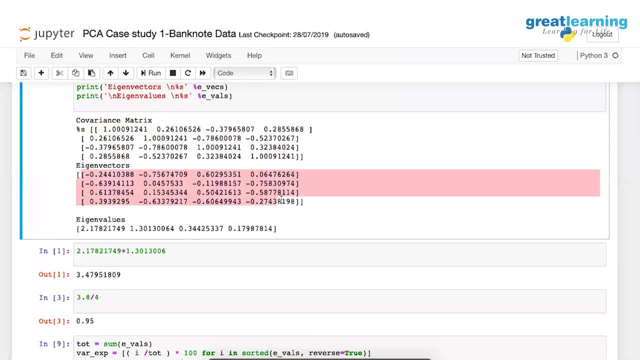 So this: when we apply this function on co-variance matrix, it is going to give us two different matrices called values and vectors separately. So if you display this, this is your co-variance matrix, this is your eigenvectors And these are your eigenvalues. Now, if you look at these eigenvalues- very simple this- 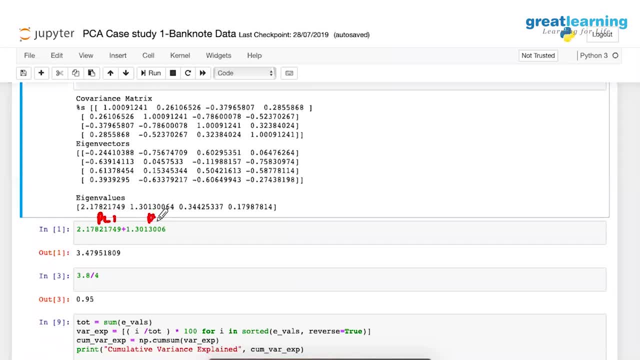 is your principal component. one. principal component. two principal component three principal component four. Now can somebody tell me what could be the optimal dimensions we can reduce to? And if you add all of them, the total variance you are going to get is: 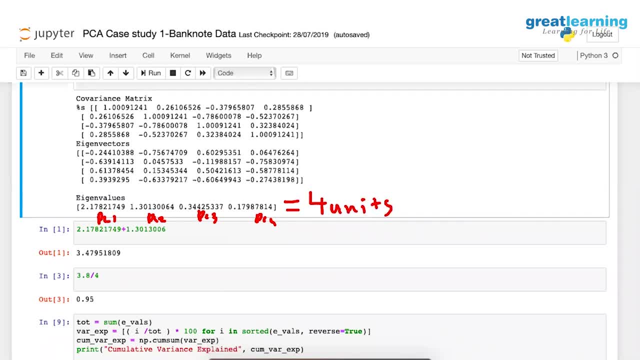 four units. You can confirm that. you can check it out Now, can somebody tell me which three or which two? you can even retain One, two or one, two and three, Perfect. So if you see one and two together, we are getting around. let me try, if we have. 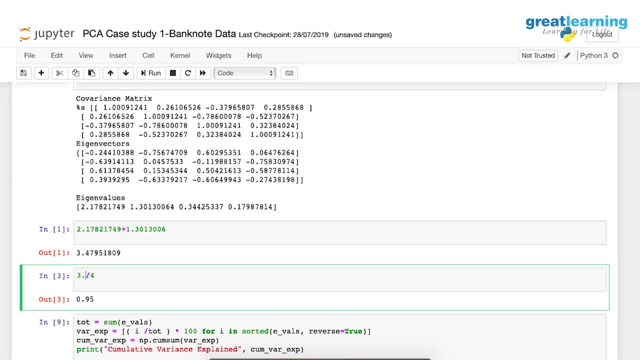 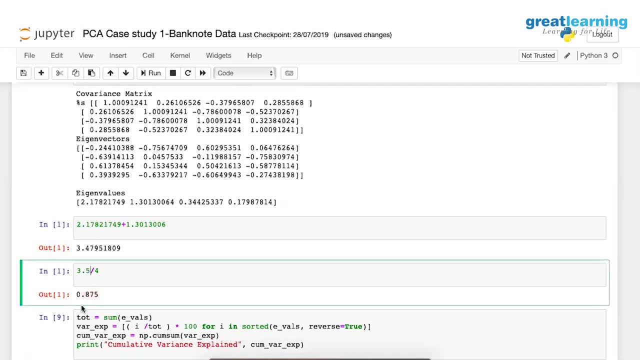 one and two, so two 2.4 out of, yeah, 2.4.. So when I run this, 87 or 88% of variance, we are getting Okay Good, And if we add first three together we are getting 95% of variance Since the. 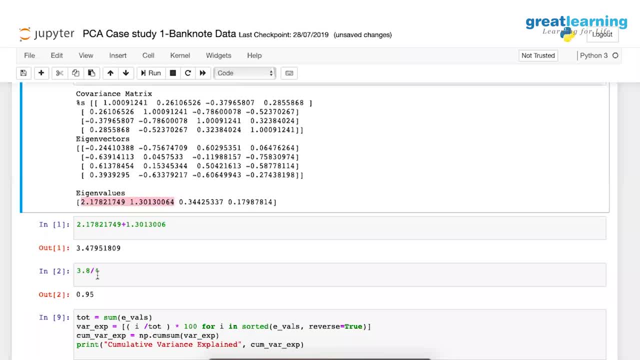 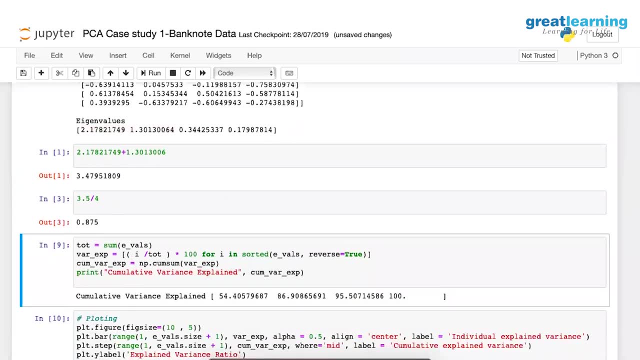 bank has requested us just to retain two of them. we will say 88% is a very good number. Nothing bad into it, It's a majority number. Yeah, Sometimes you won't believe I even go ahead with 55%. also, When I'm in desperate needs, I go ahead with 55, also nothing wrong. 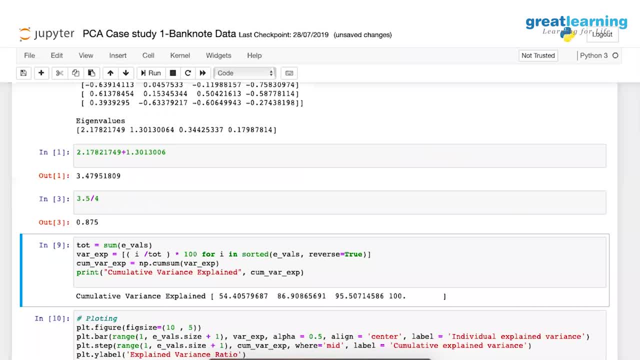 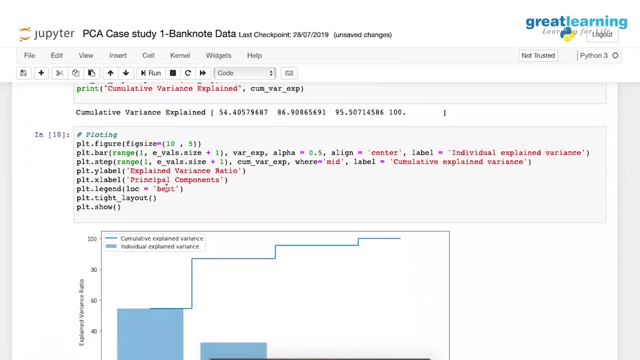 Since we are in majority. 55 is a majority. it's nothing wrong. Now we can do this. So now we have chosen first two. If you want to plot and check it out, this is the way you can plot it out. So what is this? This is your individual contribution. 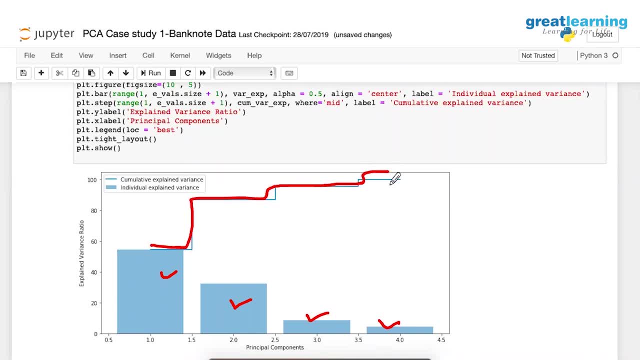 Or if you want cumulative, this is your cumulative contribution, whichever way we like it. So if you look at cumulative, we can say: this is 88%, giving us a good value. Yeah, So you want it an automatic way, you can do this. Or if you want a manual way, manually you. 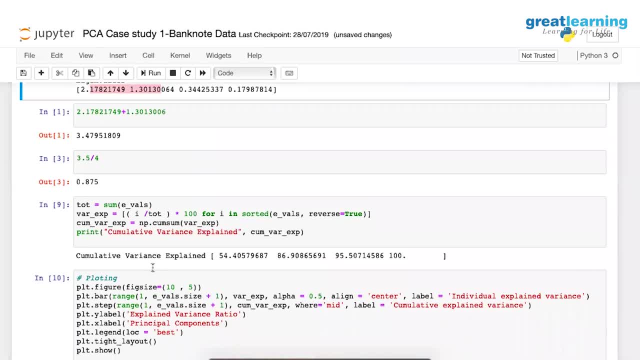 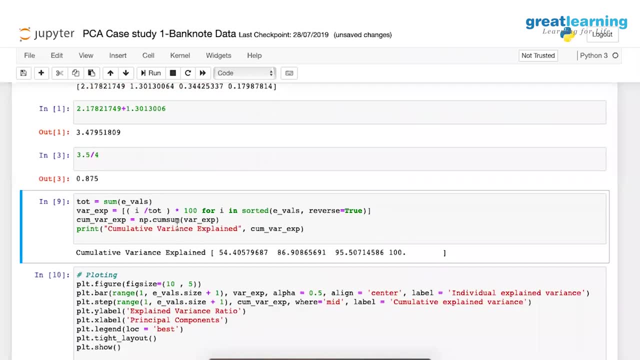 can calculate Perfect. Why do I say manual? Automatic is sometimes you have 100, 150 dimensions, In that you cannot keep adding this. So in that case you do the cumulative one, Cum sum, is the formula that we use. If you observe here, the first principal component gives me 54%. 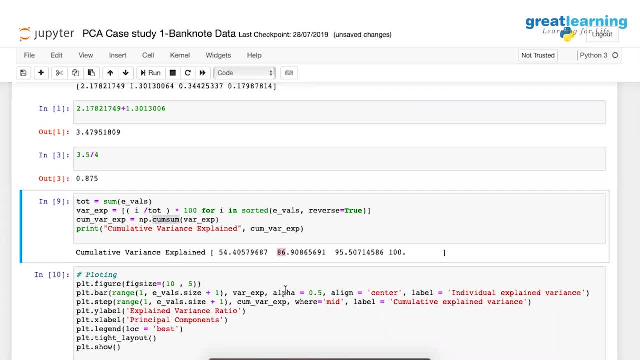 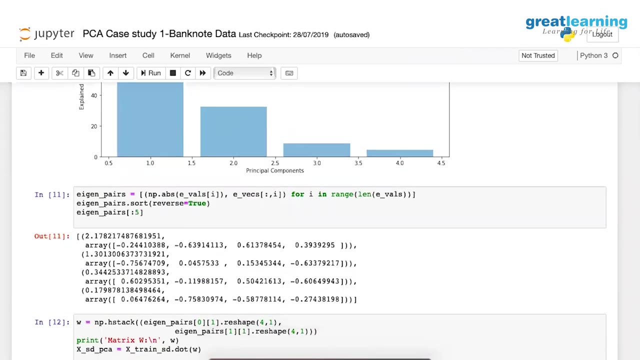 The first two together, cumulative way, gives me 86.9.. First three is 97. So if you add, if you see this, you can directly visualize it. Okay, First two are good enough for me to move- Perfect. Next is the challenge of creating the middle matrix. Now, what do I mean by? 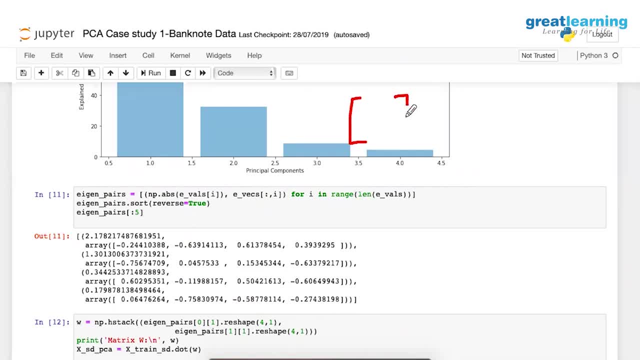 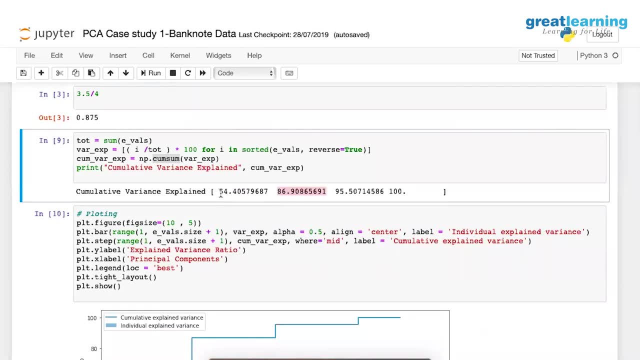 middle matrix is, if you observe, Sorry, sorry, sorry. What does the percentage imply? What does it mean? 55,, 85. Okay, Right, We selected that, But what is it? Is it accuracy, Is it? 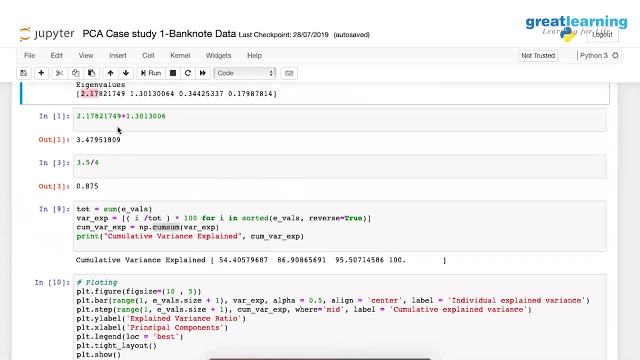 No, no, it's not accuracy. It is 2.17 divided by 4.. Yeah, Agreed, Agreed. So what does the number imply? So if I choose, say, 55,, like what you said, 286, right, Is my model going to be better Or I will have a better confidence? 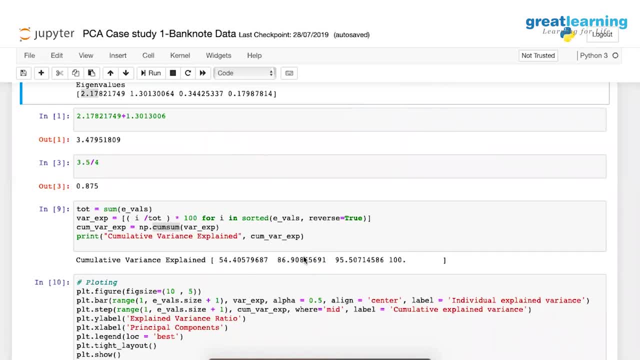 though I remove a few attributes. What is the No? How do you? Okay? So it's like saying that we have five dimensions, Okay, And out of this five dimensions, we are generating a covariance matrix. So now our matrix is a mixture of all five dimensions. 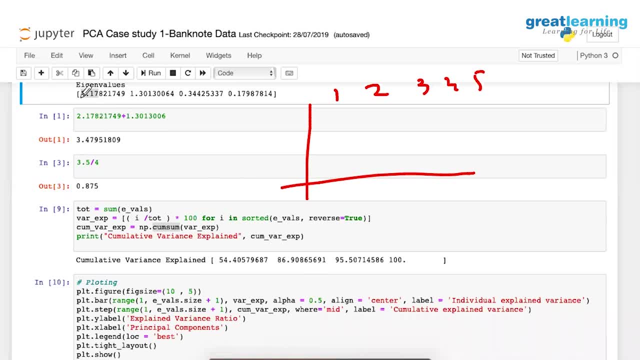 Yeah, So now I'm saying that first two principal components, we are generating a covariance matrix. First two principal components are giving me 87% of variance. Remaining 13% of variance is coming from the last two dimensions. Or say, here we have four dimensions. Yeah, 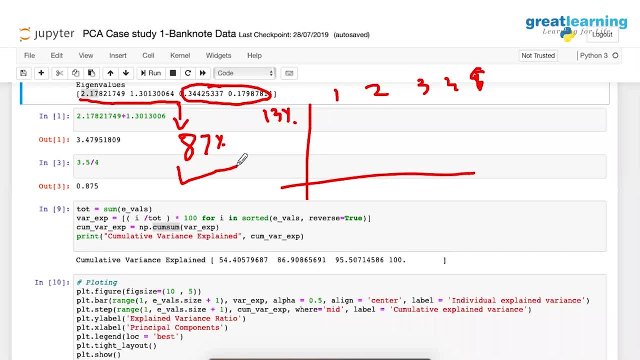 So we can say that since we are capturing majority of variance, it is okay for me to lose some variance. Got it. That's a variance measure. Exactly, It's not Because here we do not See, we don't have a target variable here. 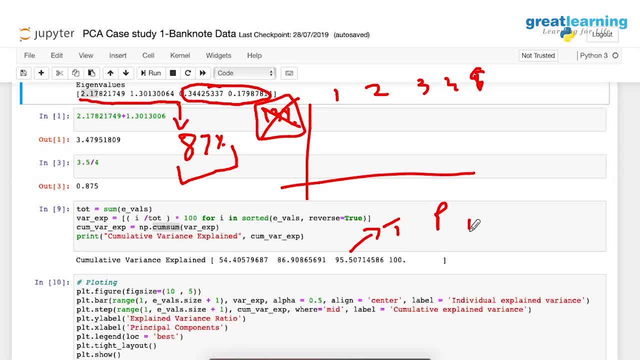 right, Yeah, So we cannot do our performance measure or accuracy rate or recall factor. We cannot do this because target variable itself is not. It's an unsupervised learning technique. So in unsupervised learning technique we play around with. variance is captured Got. 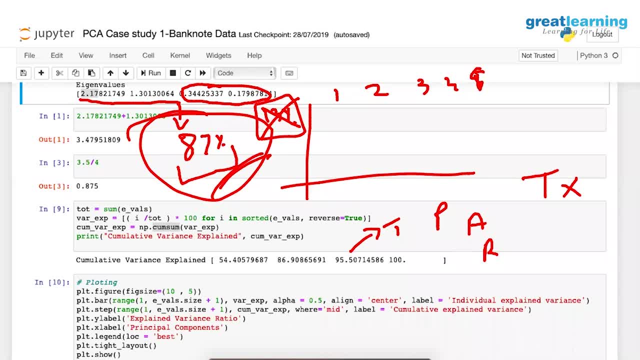 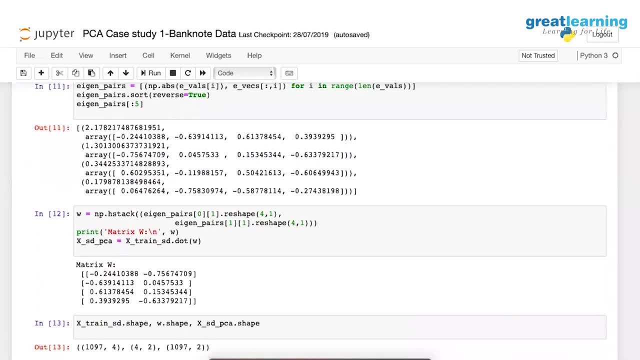 it. Okay, Sure, Perfect. So now the game here is to find the final answer. Now, why do I say it's a little bit tricky? here is let us try to understand our matrix dimensions. Initially, our matrix is of 1097 cross four dimensions. Okay, Yeah, We have got four features. 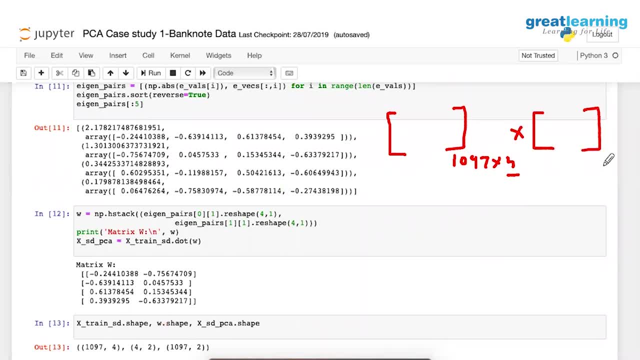 Now we are supposed to multiply a matrix to it with four cross. So now our final answer. as we saw, as we chose from eigenvalues, our answer should be 1097 cross two. Everybody agrees We have chosen the first two dimensions. Okay, Now what should come here? We should. 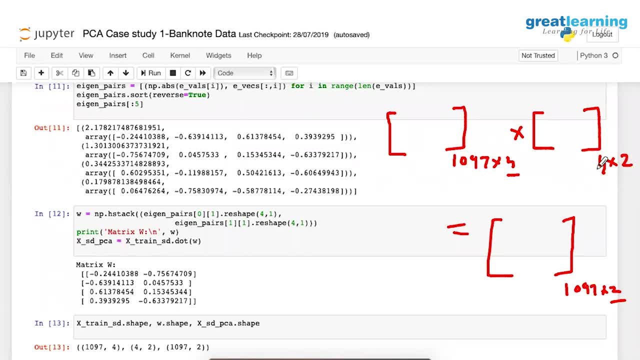 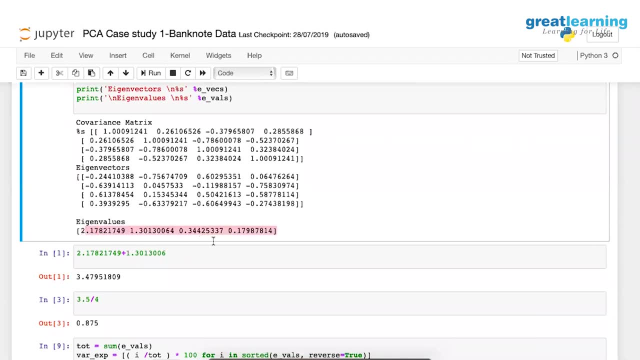 have a four cross two matrix. Now how to generate this four cross two matrix is very simple, as what we have here is: we have got our eigenvalues and eigenvectors. Now the job of eigenvalues is over. As soon as we choose dimensions, this is over. You don't have to. 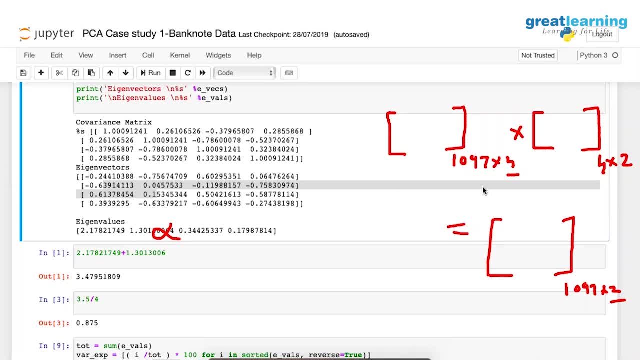 play around with this. Now, as I said, if you can see, here, this is my eigenvectors from PC1, PC2, PC3, PC4.. PC3 and PC4, we are not seeing anyway, Correct. What are we left with? We are left with PC1,. 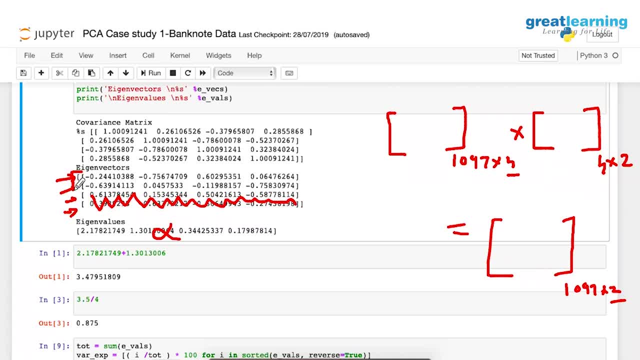 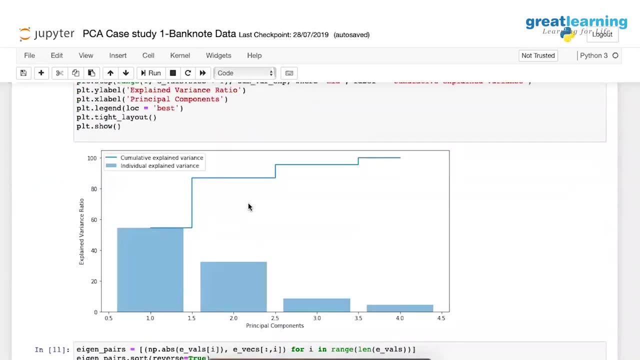 PC2 eigenvectors Correct. Can somebody tell me the dimension of this? If this was a matrix, Two cross four, Two cross four- What are we need for Four cross two? What to do here? To transpose Exactly. Pick this up first to transpose it. So when you transpose it you will get a new. 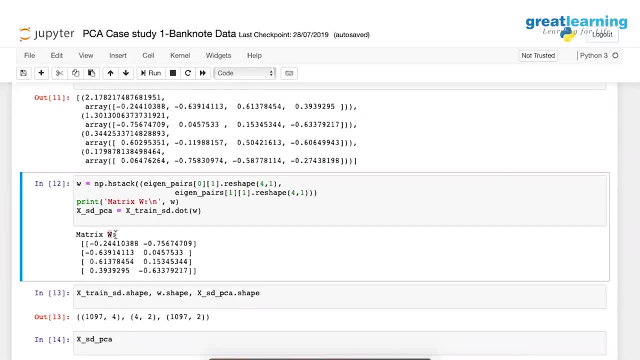 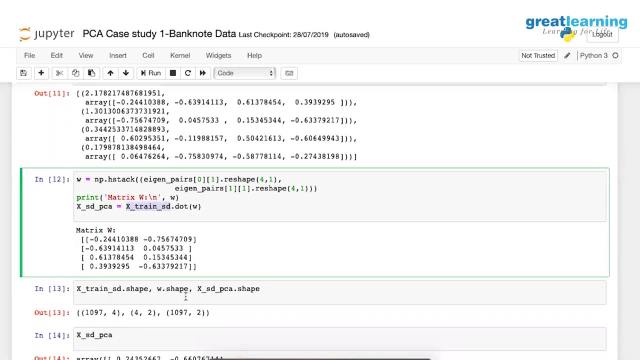 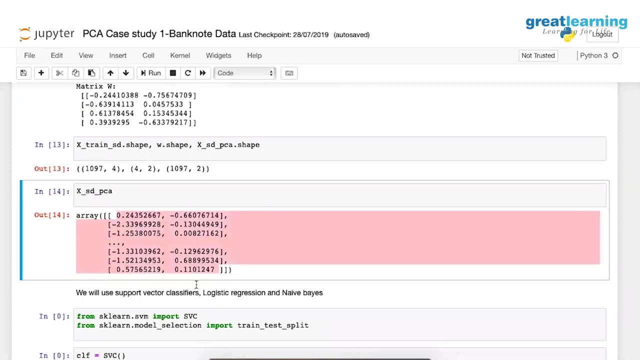 vector called W. Yeah Yeah, When you get the vector W, do a dot multiplication with your original matrix. You are going to get the final matrix as your PCA matrix. If you look at this, if you look at this one, this is your PCA matrix. Okay, So there are a lot of values missing here, So don't think. 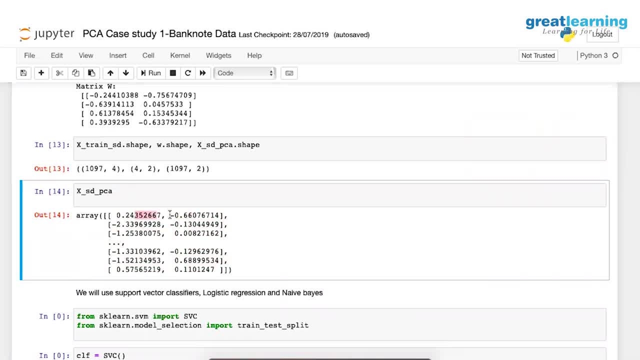 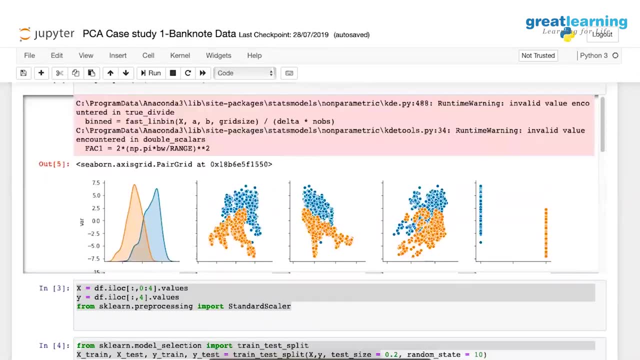 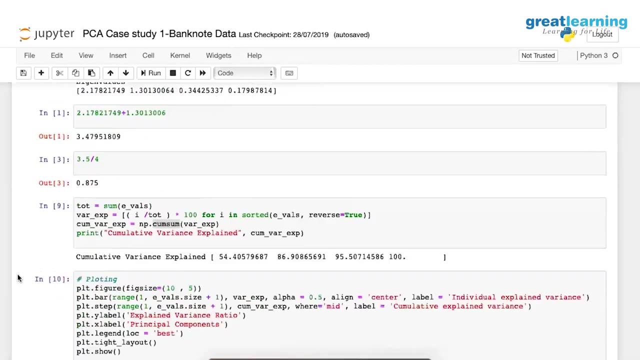 this is the only thing. Just look at the dimensions. You are having only two dimensions, But look at the numbers: Point two, four minus point six, six, And look at the original matrix: Three point two, eight point six, Eight point six. Yeah, So we'll come back to that, Why it has happened, But for now, 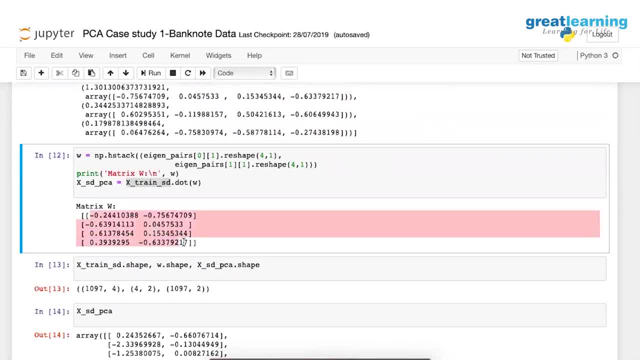 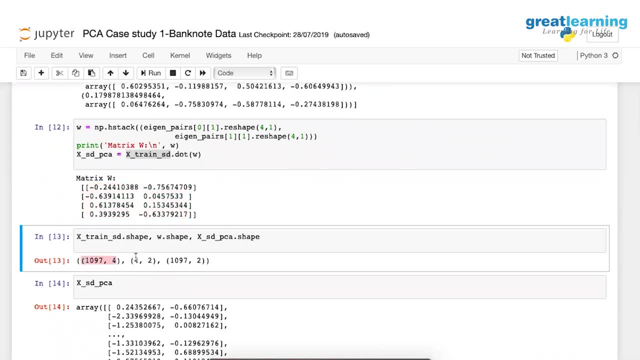 did we get it? What happened? This is our dummy matrix. We multiplied with our original matrix, So it's the dimensions are here: One zero nine, seven cross four into four cross two. The result was one zero nine seven cross two, Simple. 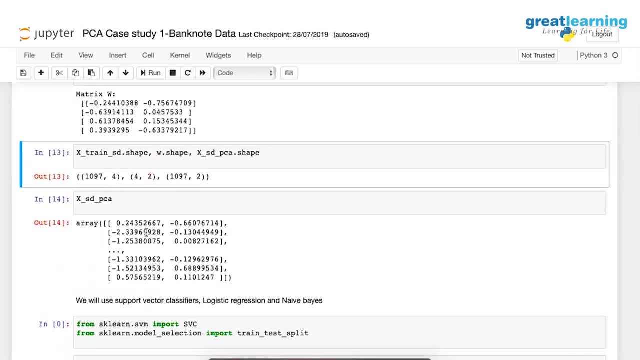 Yeah, So this is the new data that we will use for all our modeling. Is it Perfectly identified? Perfectly identified? Now, my question now is: which dimensions got reduced? So, if I go back here, which dimensions got reduced? Can somebody tell me? 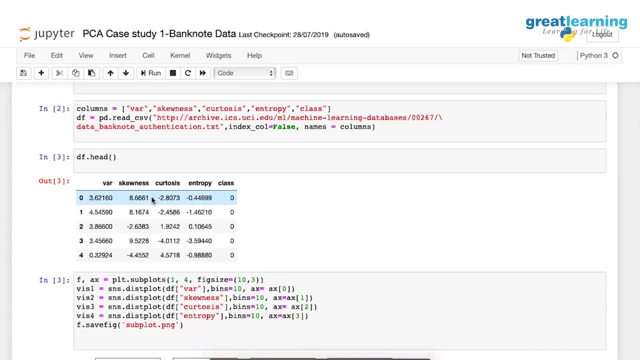 We don't know. No idea. No idea Correct. Even I have no idea. You know why? Because we did our dimensionality reduction on covariance matrix. What is covariance matrix? It is a Khitri or mixture of all of these, So it was a virtual dimension. 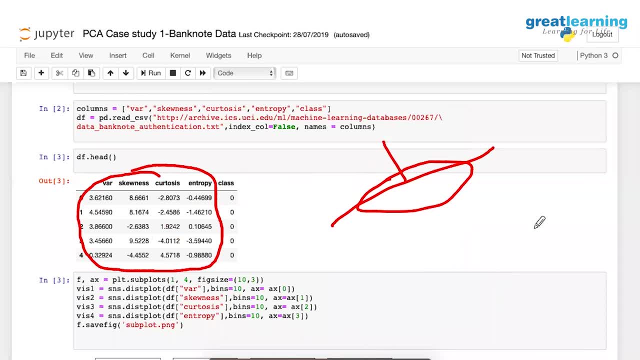 If you people remember Correct. So what have we done? We have reduced the dimensions, Yes, But did we delete any of these dimensions? No, Got it. This is the paradox, Krishna. what do you suggest for this coding, Like you know? because how to, how to, how? 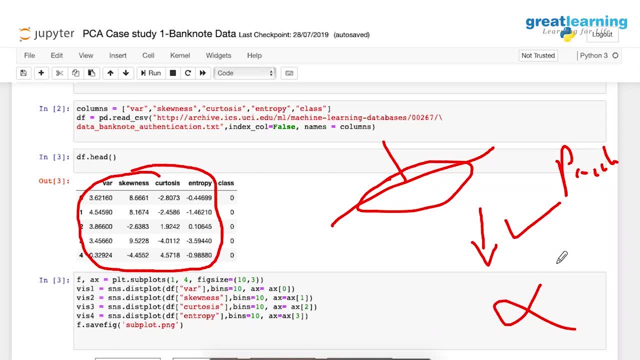 to be perfect in that. Yeah, Which one Coding part? Coding part Again, I'll say you have to actually sit onto it. It's like practice. So I will say, see, I will tell you personally, as don't take it in a positive or a negative. 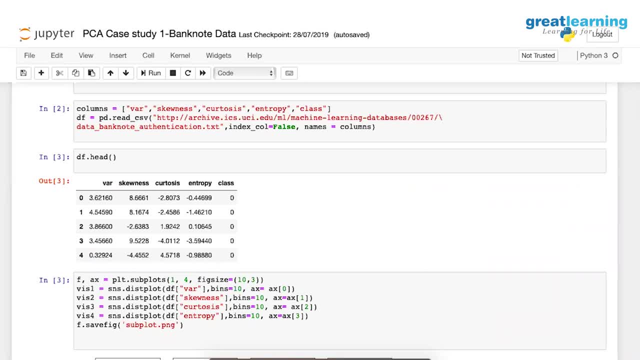 We'll just be very neutral here. You don't need to be exported Python to be a data scientist. You know why Google is there. Your own database will be there. So let us say, today you made a PCA code. Okay, You can restore this code. 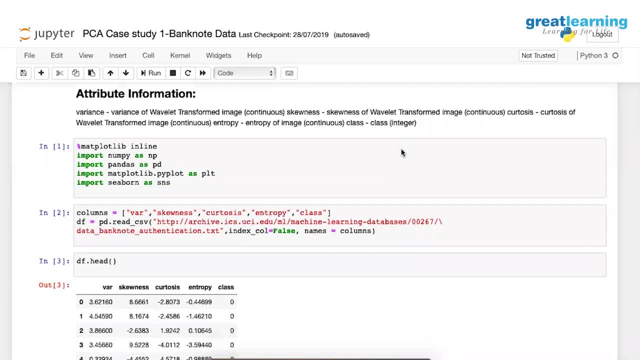 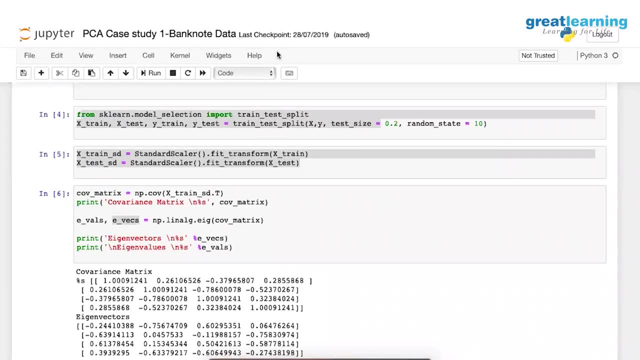 Tomorrow, whenever you want to do a PCA, retrieve this code, change the data here and there you will get your answers ready. But okay, May I know the average experience you have, just in case? 14 years, 14 years. You don't need to know Python for that, because, as at this experience level, 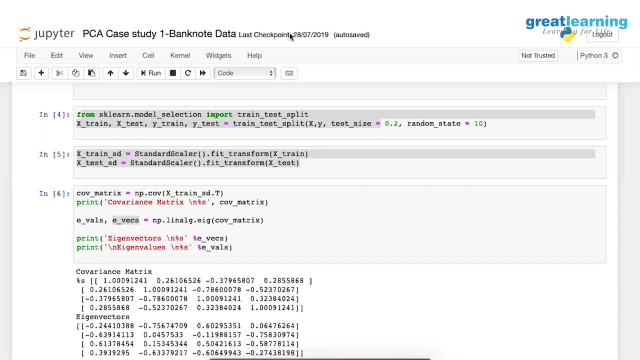 you will be going as a transformation leader, basically, So you don't have to code through this. You have to suggest to a data analyst or a Python programmer That this is my model, This is my design, You do it And if in case, you are going as 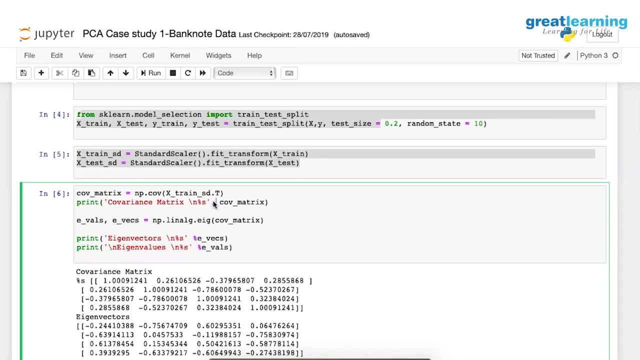 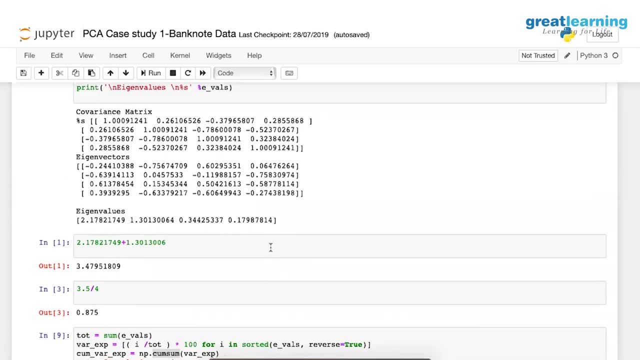 a data scientist. these things are ready with us. When I deliver my codes to you, you know my codes are universal codes. Nowhere you will find references to this particular dataset. if you observe it, What you can do is you can directly take it up and I'll be very happy. 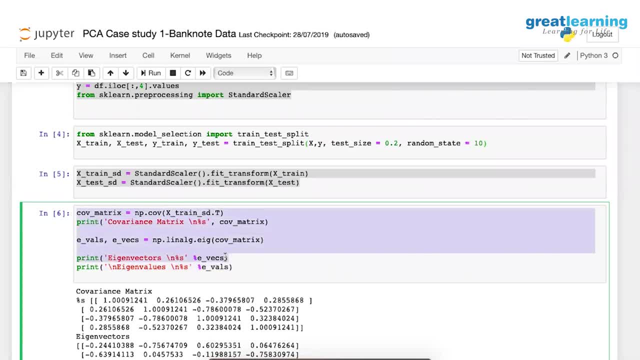 You can take it up, paste it, do some changes, It'll work. So again, I will say: we cannot have, we cannot be a Python expert in two, three months. to be very frank, See, I am coming from an R background, So I started with Java, Then I moved on to say Python in middle, Then 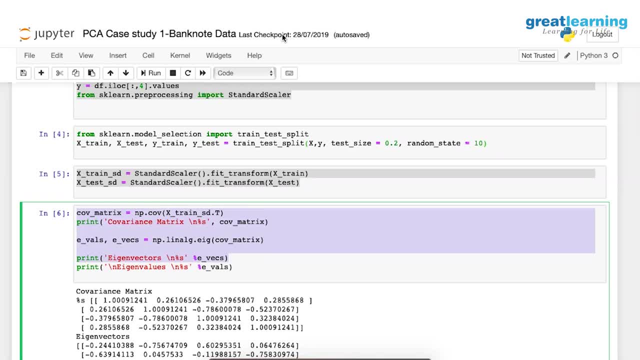 as a data scientist. then I moved on to VB and all this because I want to do automation, testing and all. Then I moved on directly to R. So R was a little difficult for me. So this is what I felt when I started with R: It took me around two years to have a command. 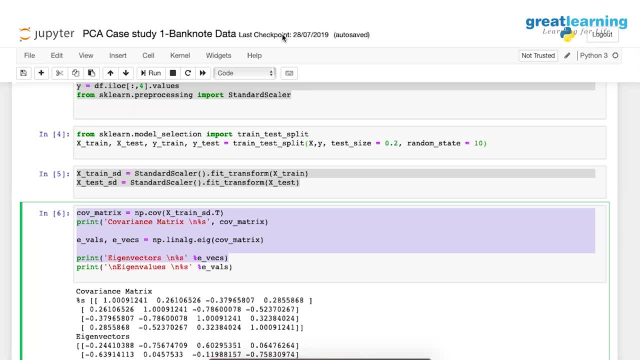 on, But unless and until I did that, then I got the idea that, okay, why do? why do I need to? How do I completely expertise the coding when I have my dataset ready? Why not to be expert on how to implement it? Okay, From R I shifted to Python. It was a very easy. 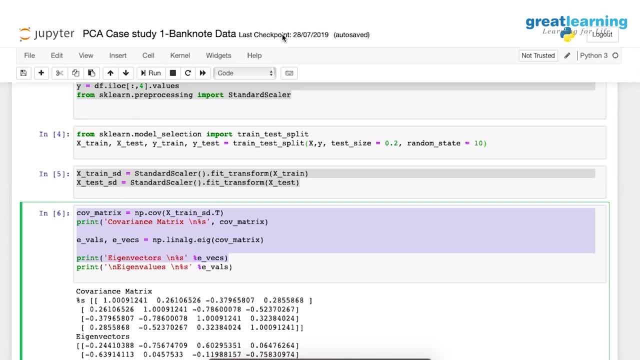 curve for me, because if you know R, R is little weird, It's a actual data scientist language and Python curve is very easy. So again, the overview of this- why I summarize this- is it's not necessary that you should know all these syntaxes and all property, but you should. 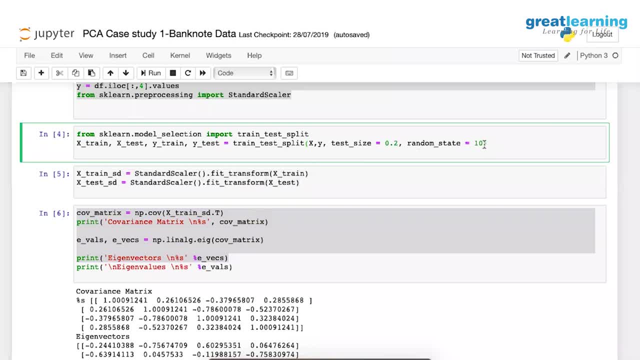 know where to change what. So if I ask you to change the random state, you should exactly know what do we mean by random state. There is nobody in this world. if I give him a dataset, he will start coding. He will code this without any reference. I will tell you openly this. 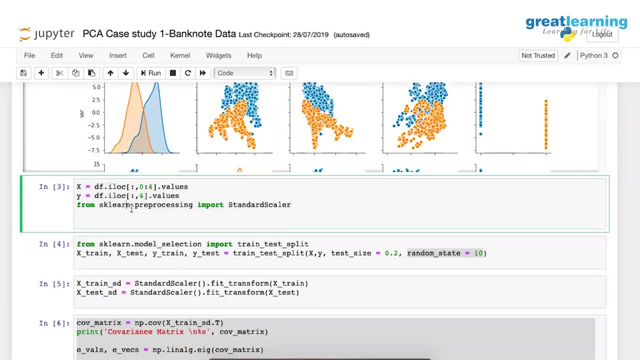 thing. There's nobody in this world who will. so what we see? you know what we imagine about a dataset. it's not like that, because we have thousand opportunities here. Nobody knows all the stuff We have got. so many libraries. 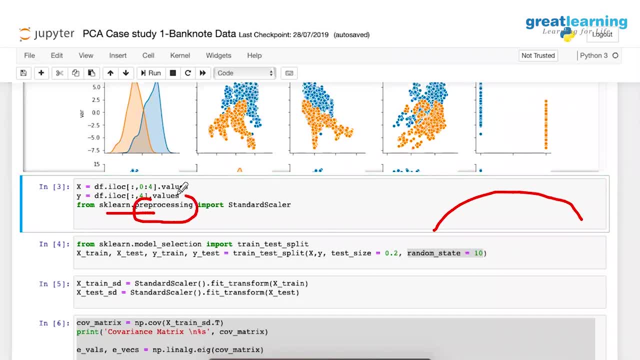 See, every day this library is getting updated. It's an open source. Somebody else is updating it. It's not necessary that I know all the functions of this game, but definitely I know where to go and hit on. So this is where I want you guys to be expert, rather than taking 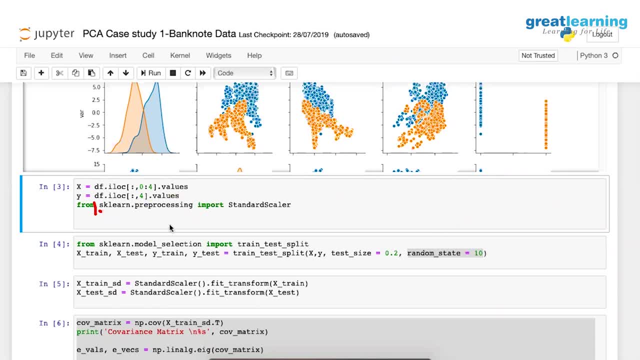 pain off. you know, becoming expert at Python Tomorrow, after two, three years, even this might be replaced, We don't know. Yeah, Correct, Yeah, So these work with notebooks, right, So do they get uploaded? I mean the one that I 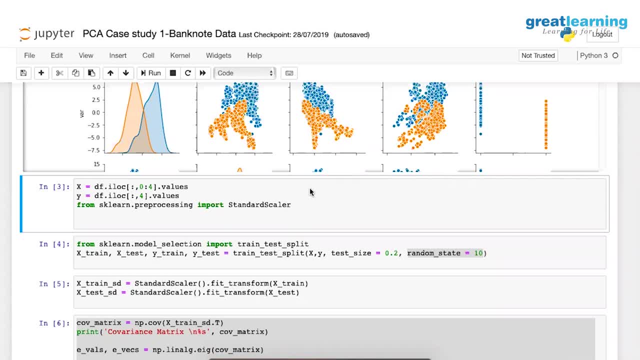 see is that the video recordings that come as part of our weekly training. there is a notebook that comes for the for that, But this is there a separate folder. I don't know, I'm new to this group also, So so is there a separate folder. 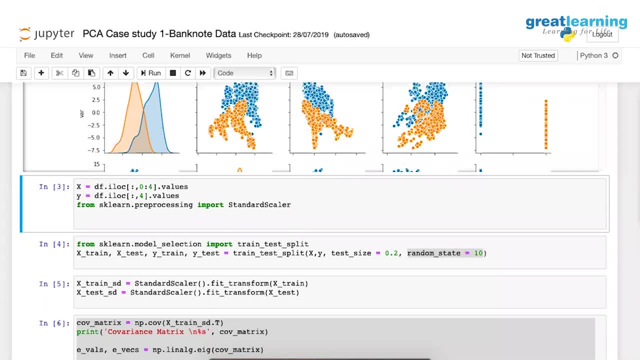 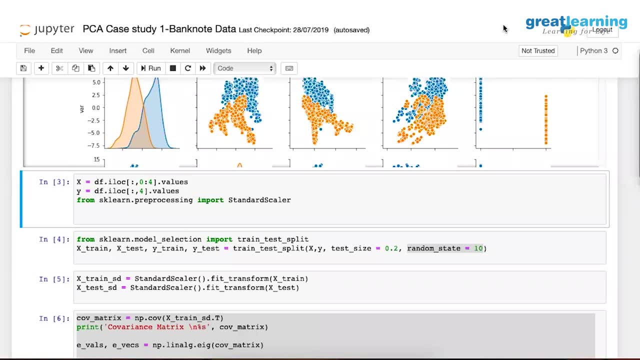 I send it to my group As an email. Yeah, as an email. Oh, I'm not in the email list, So I just joined for four minutes. Okay, I just joined for four weeks back, So I will, I'll request, probably. I don't know how to. 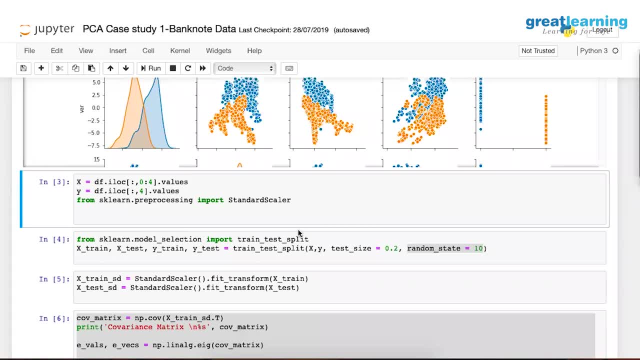 send No. no, you just drop a mail to me. I'll take care of it. Okay, Perfect, You can copy my mail ID on the common chat, Okay, Okay, Is anybody else not receiving my emails? Anybody else here? 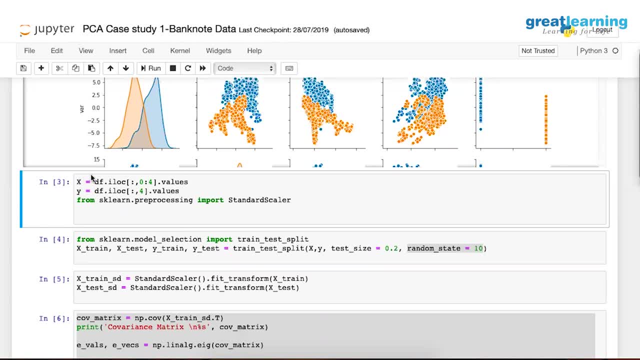 And is that a repository that I can go and pick it up? because the older ones? how do I get it? Actually, I tried. I tried proposing that A Google folder or something. Would you have a? can I share my Google folder or can we? 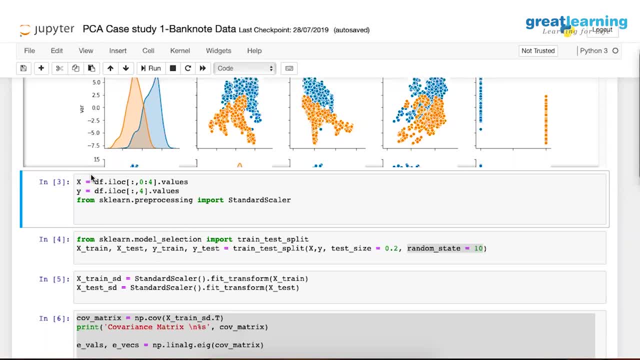 create a Google folder for this group. Let me check with great learning onto this part of it, because I'm okay to share with an email, but I don't know. I've never asked them about a repository. Actually, it's a good idea. We can do this, So let me confirm with on this and, if possible, it's a very 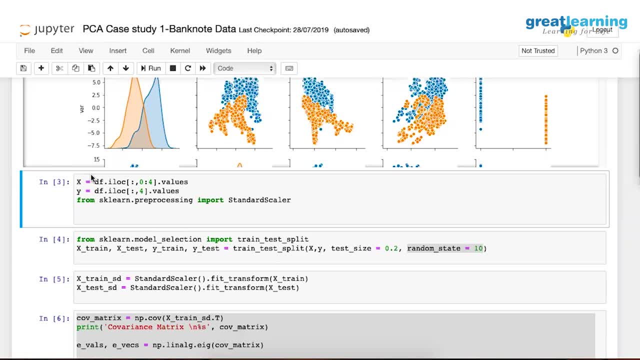 good idea. I can directly go and drop it. You guys can pick it up from there. Yeah, I'll. I'll probably see. if I have all the email IDs, I can create a Google folder and share it with everybody. Group level if you can share. yeah, group level if you. 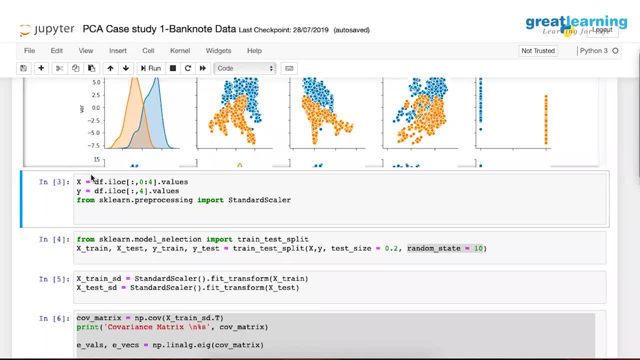 can share your email address. I'll just pick it up. Yeah, no, I just shared yours so that everybody. so one thing, Krishna, see all these examples and the the machine learning exercise that we do know very trivial, that we have to this. 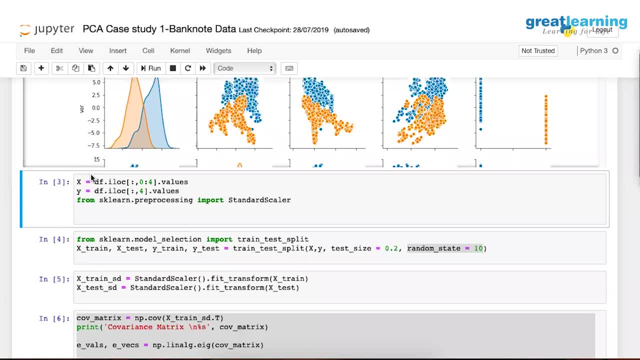 this new exercise that we did. today's project is the biggest that we've done. It's got about 45,000 rows Okay, And I mean of course, my computer MacBook crawls If I do any swamp art or says some sizable peplot or something like that, Right, So I'm hoping that a a 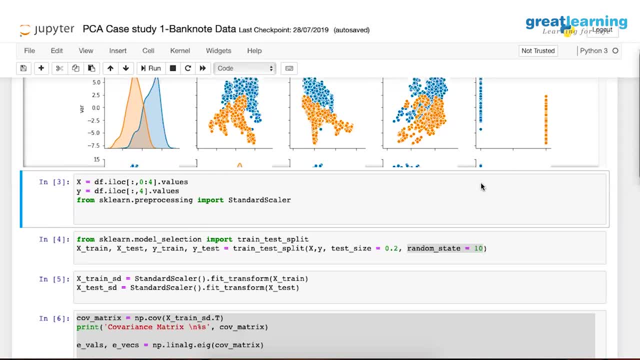 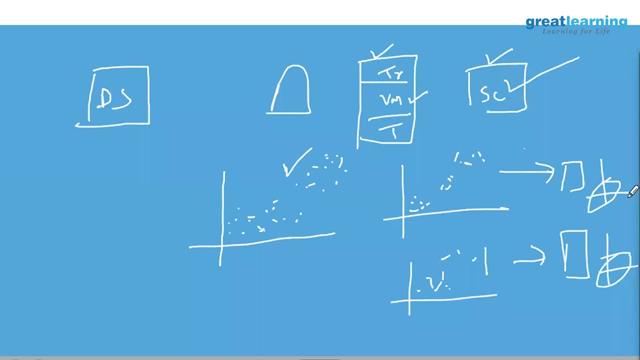 serious project which has got hundreds of millions of record, So does that also do the same? You go to a Jupiter notebook and type No, no, no, no, no, no, no, Yeah, Yeah, Okay, See, okay, fine, Let me, I think I got it. See what I'm. what is my method is for first, 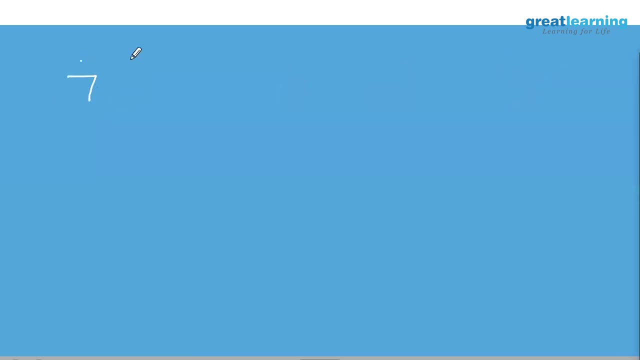 eight or six or seven modules. I will be showing you this stuff on Jupiter. Why? Because we have to understand line by line. So once we complete. so I think we are in what model? right now we are in unsupervised line. This is an AI ML batch, right? Yeah, that's correct. The post unsupervised running. 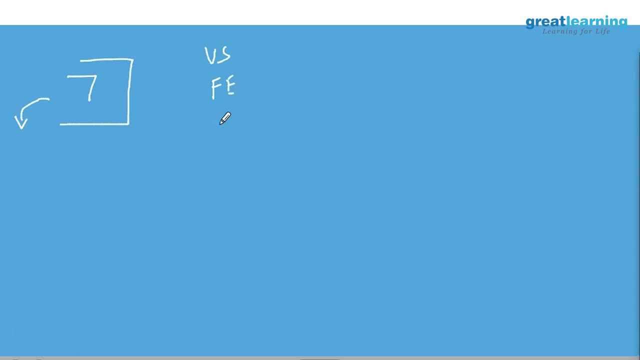 we are going to do feature engineering. post feature engineering. We are going to do a recommendation system. was that we are going to do neural networks or deep learning? Okay, Right That it is a computer vision. Again, I will say both are same. on the thing You 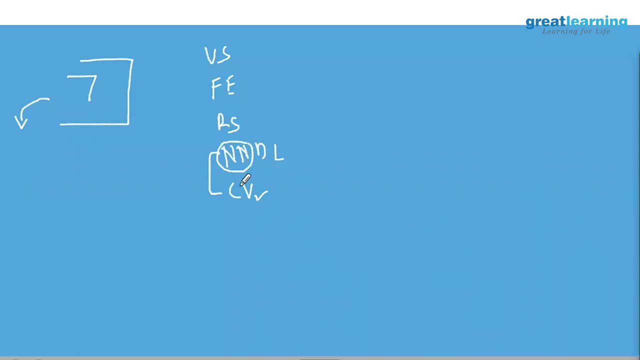 can see, here we are processing pictures. here We are processing text, speech and everything Whatever. Finally, we are going to end up with NLP- natural language processing. So once we have entered this phase, I will shift you guys directly to production environment. on. 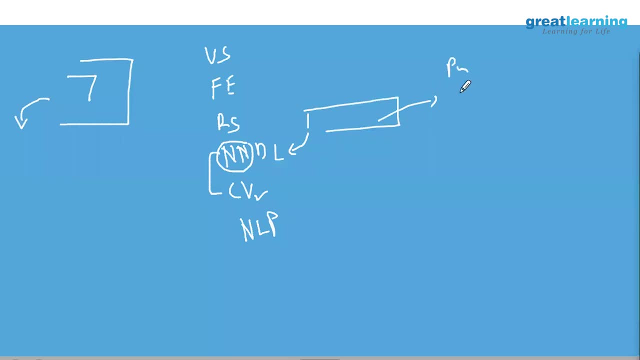 industry, So where I think we will use by charm or use by torch, or we'll use Eclipse If, in case, you guys are okay with it, we can use these IDs to do our computation. So this will be a phase where I will 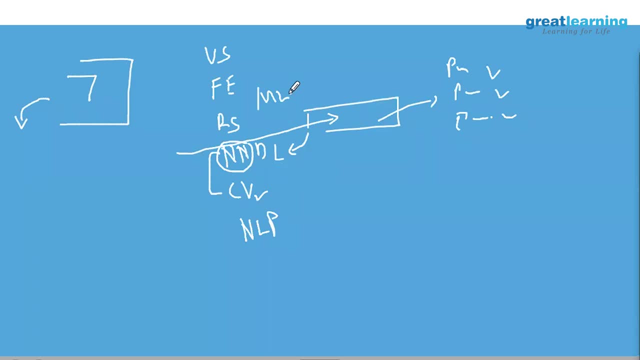 Okay, I can say that you guys are machine learning experts at after recommendation systems. So there I will directly shift you guys to the production So, where we will bring in the concepts of. I'll bring some extra concepts of Hadoop. So, as you told, 45,000 rows your. 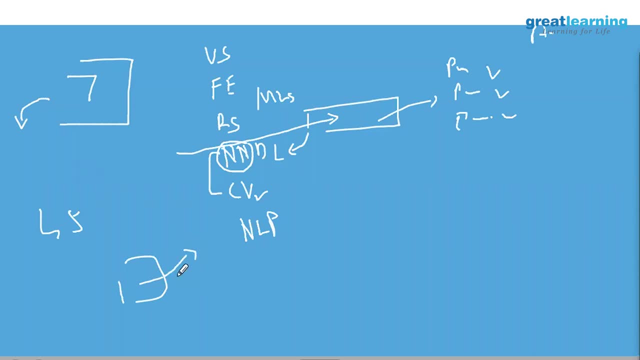 Mac book is getting cluttered, So for this also, we have got multiple solutions. So usually what we do is we run these stuff onto our VMs- Okay, And these VMs are high powered machines, Yeah, Okay, So we will do a little bit of a demo on this next step before we even start. So I don't 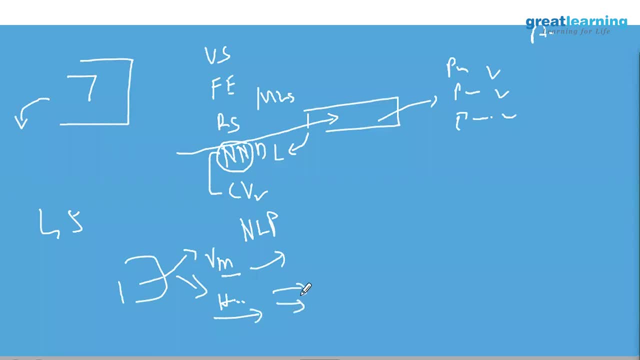 have the time to show all the documentation here. But once you have done that, I will start the first step and we will go over to the Editor and let us go through that. So first of all, we have actually got a bit of an experience on how to do this, but in 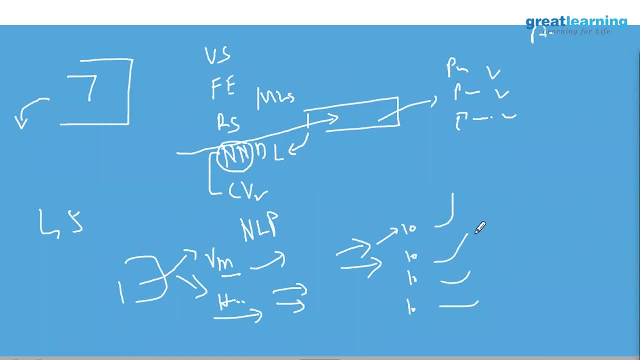 the last couple of days we will be doing a little bit of work on How to Do This. So before we will get into the demo, I will just show you what sort of method that we will use on how to do this. Yeah, sure. 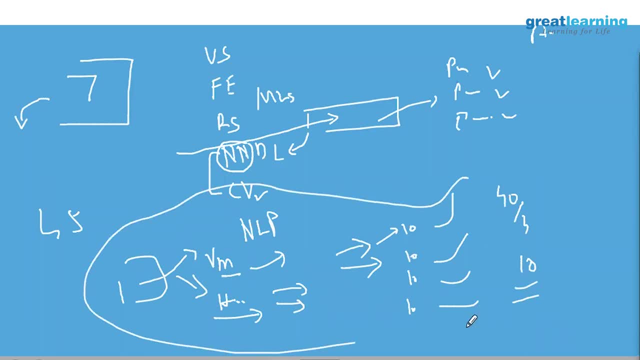 So I'll just give you guys a bit of a overview on how to do it. I'm going to start off with this, all these things, but for that we need to wait some more time, because I want you to be very good with stats. right here we are. 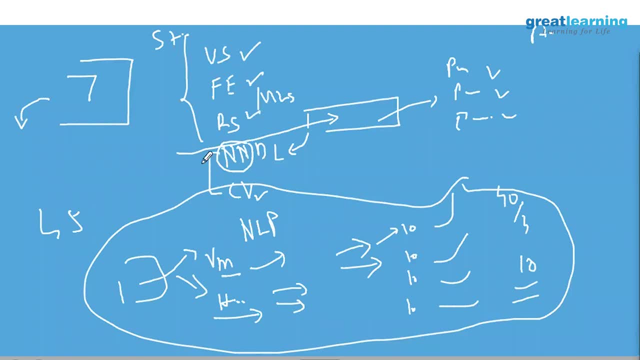 having a lot of time to talk about extra things once we enter neural networks, and this will be very hectic module for you guys. so here we can go back and revisit what is variant, what is PCA and all. so that's the reason till here we will hold on. 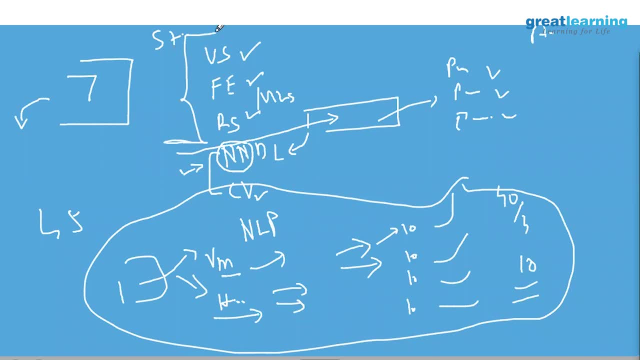 to little bit on, to theoretical part, where I will request you guys, because you might not get these all stuff readily on web, to be very frank. so if you see PCA today, whatever I showed you, you can try searching on web. not all the blogs will explain you what is covariance. 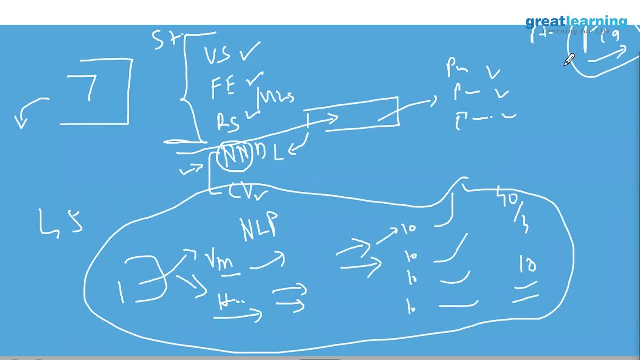 matrix. they will just write covariance matrix, but at the back of our mind we won't get it. how can we reduce dimensions? even when I started some six years back, it was like very difficult for me to get it. yeah, so that's the reason I'm going a little slow and I'm going more on to the 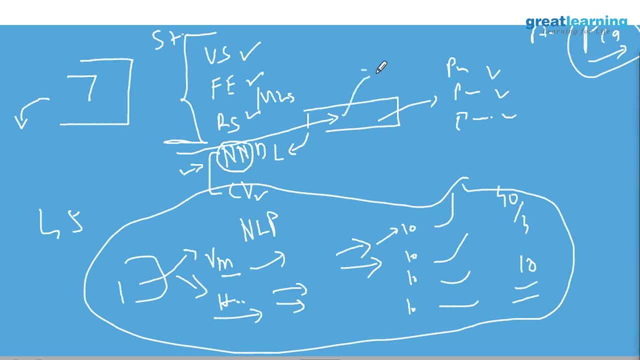 theory part of it, but at the end of this I will directly shift you guys to live production environment, so where I will show you how you can use AI versus ML. we will directly compare AI. we will implement a data set onto AI. we will implement a data set onto ML. 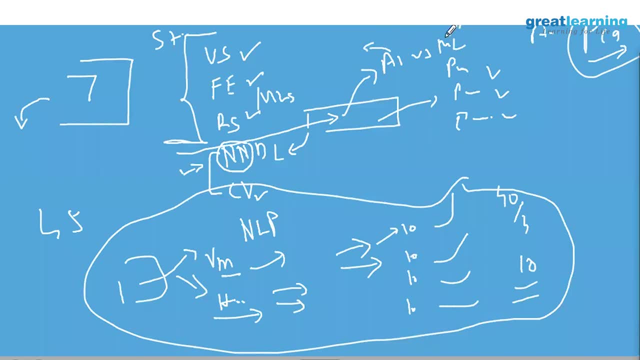 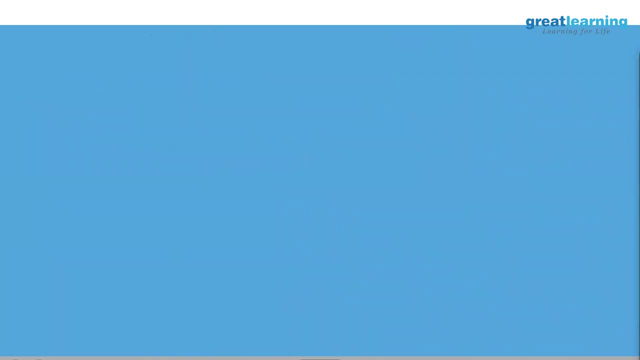 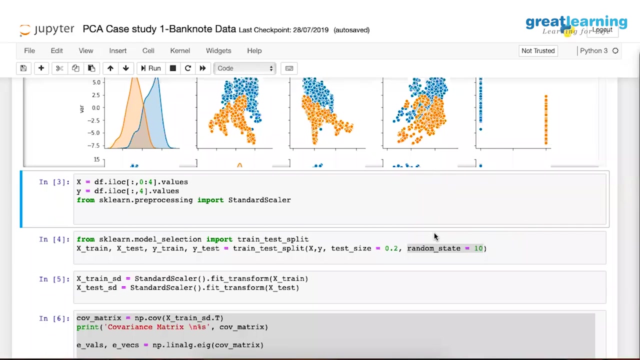 and then we will directly compare which is better. I have got n number of stuff. sometimes I feel these two words is also not enough awesome. so you tell that these things are not really blogging material, which we totally agree and understand. is there a book that you could recommend that we 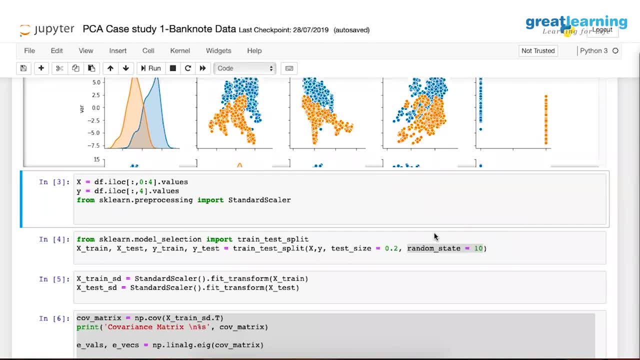 could keep it by the side, because see the the way this whole great learning is structured. the team here will will agree. if there is a quick reference that I have to do right, even for the quizzes I have to quickly check. there's no way I could do it. I have to go through videos. 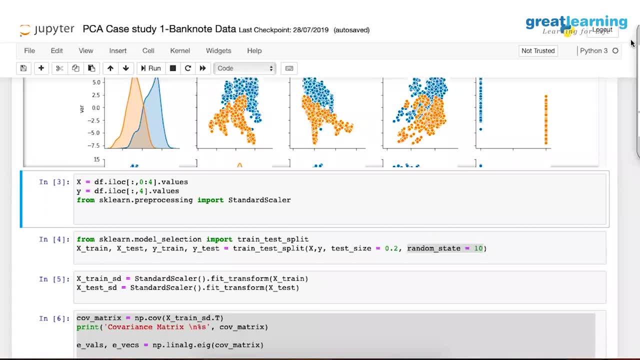 I have to go through. there's no reference at all. the PPDs are also pretty malformed, but it's any good book that you can recommend. yes, I can. I can, so probably give me two days of time. I will connect with dr PKV or dr Mukesh. I will connect with Dr PKV or Dr Mukesh. 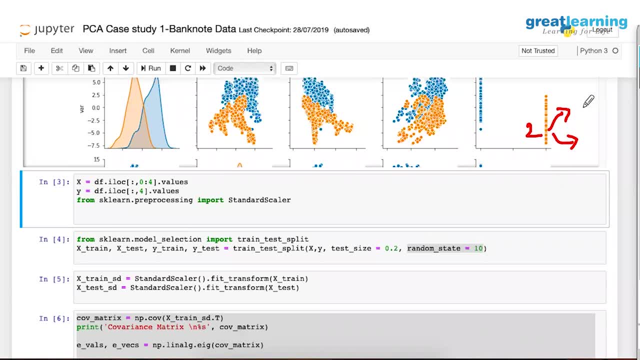 both of them. they are like my gurus, so let me okay. Mukesh Mukesh is our Mukesh right, the one who takes classes for us. Mukesh Rao, highly knowledgeable guy. the only thing the problem is he will refer us multiple books from both of them and 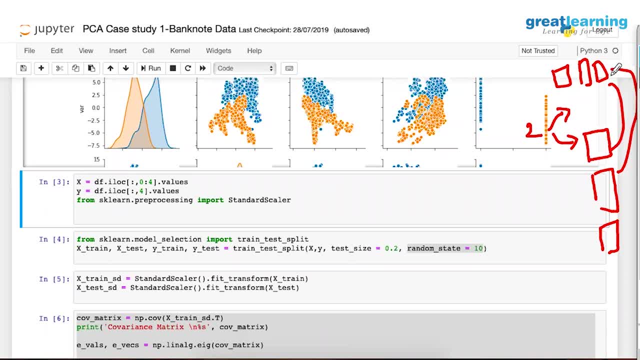 then we'll try to find the relation between them and we'll propose one or two. okay, because if I, if I talk about dr PKV- I think I don't know whether you know this person or not- he's a one of the most senior, most person in. 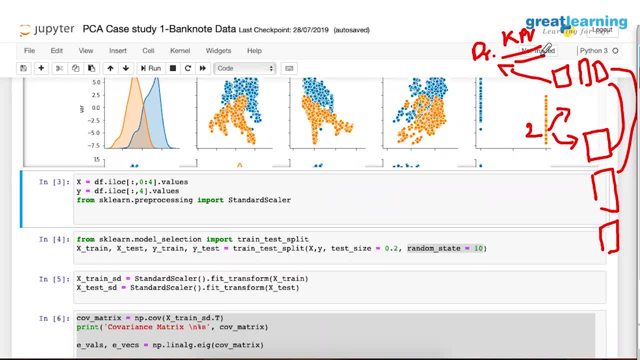 great learning, yeah, just to add. just to add: who is PKV guys? yeah, so go on, go on, go on. PKV has taken any lesson lesson for us? it's Kumar. oh, okay, Kumar Muthuraman. is that the one? yeah, from Austin, the same one, right, Christian? no, no, no, this is. 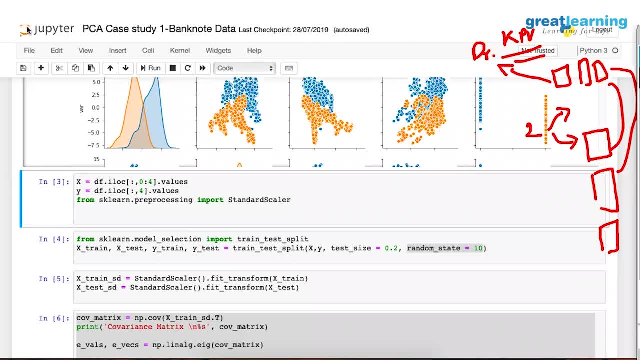 dr PK Vishwanath. oh, okay, so and so this this person is is not just tax, so he's like one of the best statisticians in India, one of the best, actually. I can say, oh really, oh, we had the class with Abhinandan Sarkar. oh, he's amazing, he's. 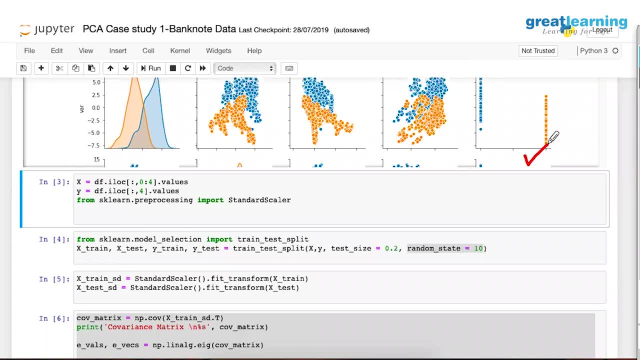 amazing. yeah, yeah, yeah, I know him also. yes, yeah, he's, yeah. so I think dr PKV and Dr Sarkar were named as one of the top statisticians. yeah, yeah, yeah recently. that came out right. so I try to connect with them and I'll try to ask, because I know. 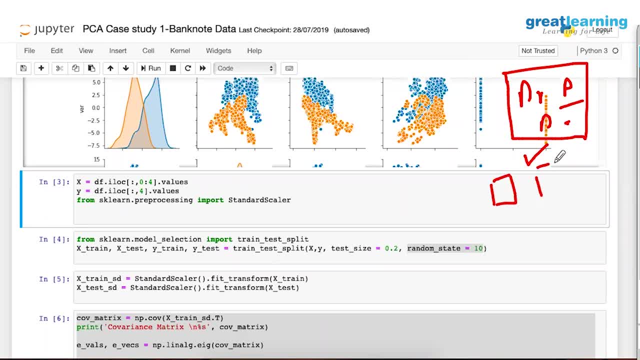 PKV very well, And he will not refer me one book. That's the problem with academician. but because you're in the industry, right, I'm sure you must be having your go-to book. Do you have anything off your head? 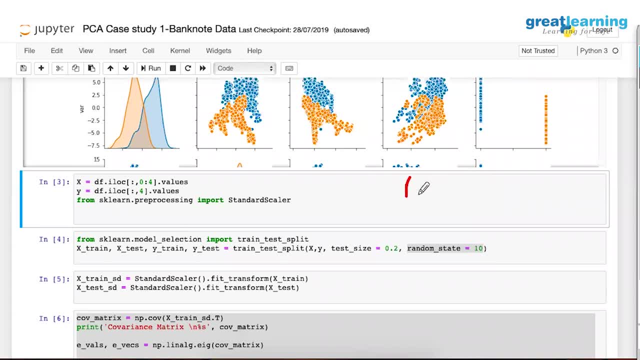 Two websites. One of them- I've seen one- is called data cam. I will ping you in the email today. I will send this data cam and analytics with you. There's one more called Geeks for Geeks. So Geeks for Geeks is more onto Python. So if you want to understand, let us say what. 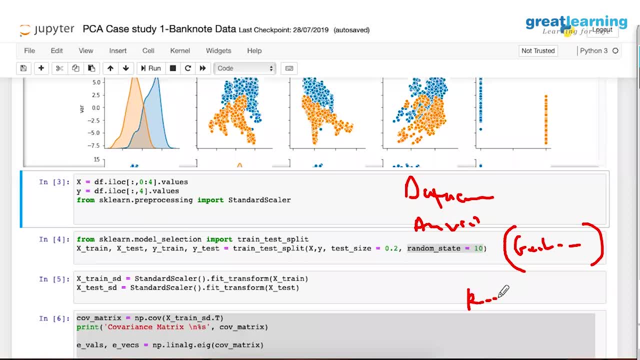 what does K-means clustering do? So from the Python point of view, I will say Geeks for Geeks is a better one. So this will be our last talk, So you can start with analytics with. yeah, it is our Indian website. They teach basics. 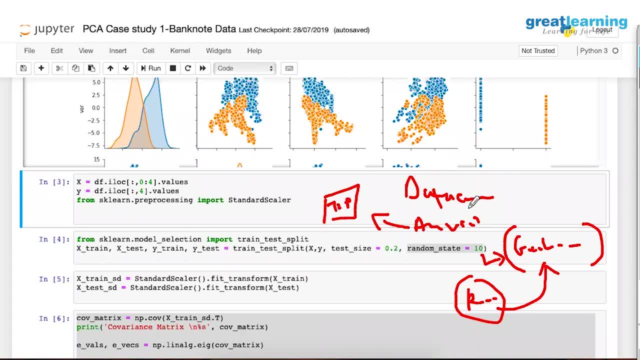 Theory, that's Python. So once we got the concept- let us say today we did PCA from analytics with you- We've got the concept post that you can go to pay data, that data can be a little bit more on statistics, They will show you exactly what it means. And finally, when you have got both the 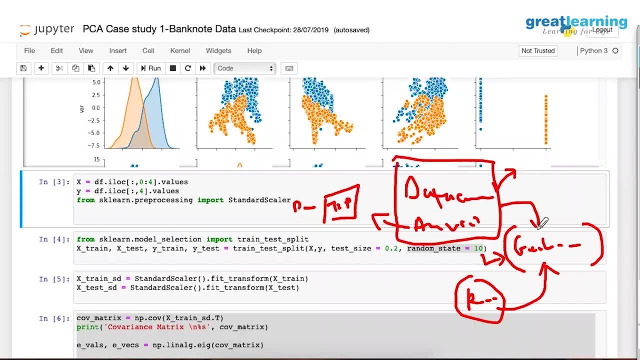 concepts together. you can move on to the same topic, on Geeks for Geeks. I like this, this person's examples. Now, it's not a one person, basically, but I particularly like Geeks for Geeks because they would explain you five, six, seven, eight, nine, 10,, 20,, 11,, 12,, 13,, 14,, 15,, 16,, 17,, 18,, 19,, 20,. 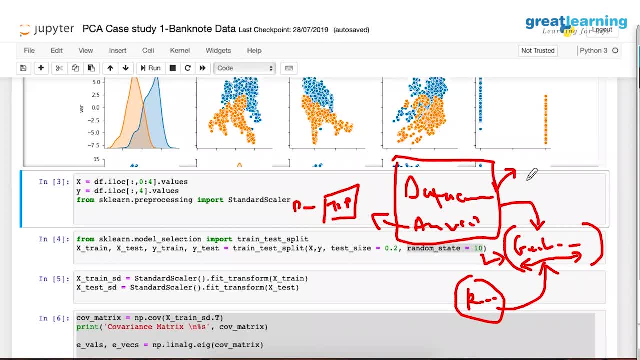 you tighten line by line, okay, so you can have a mesh up like this is how i have learned to be very frank. if, in case, you are referring to one book, just give me two days time. i'll definitely get back to you. uh, so i will say again: um, it's like checking our patience, basically. 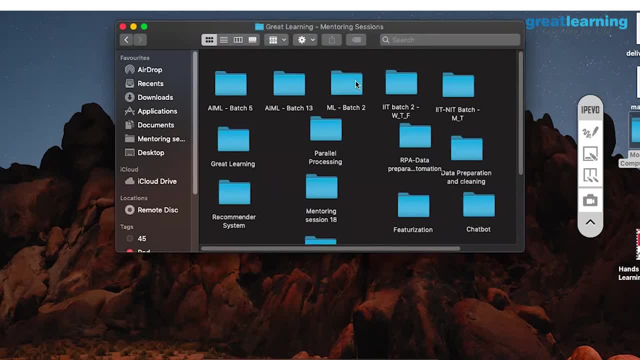 so, um, in that case i will say you can follow my format the way i have learned it. else, if you want a book format, yes, it's a good idea to take a book up and then put the topic and then go on to the part of it else. if you like one more way, i'm not sure that you. 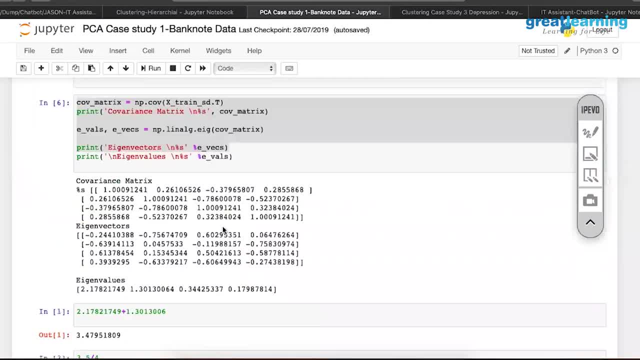 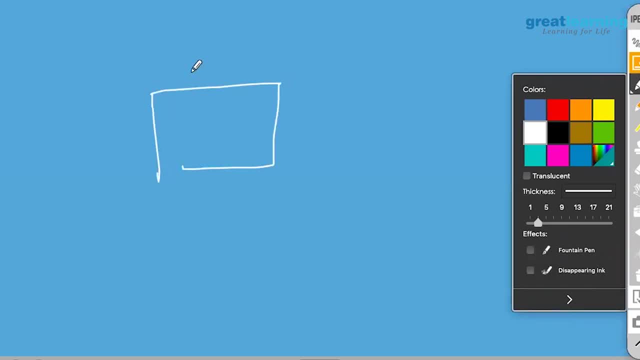 come and give it again, guys. uh, quick, two minutes from my side is uh. i agree with you. there are n number of techniques, there are n number of tools onto that and there are n numbers in which you can apply them. yeah, so it's not possible to know everything in five to six months. 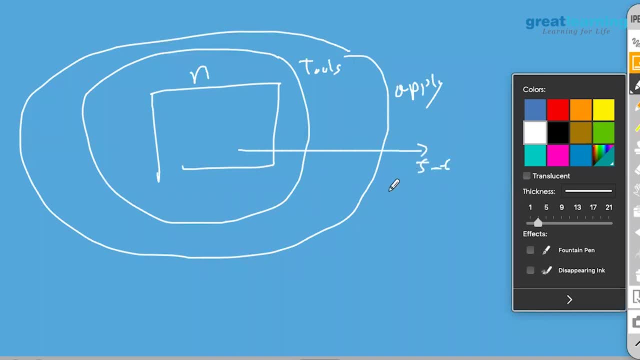 to be very frank. so i have around seven years of experience into that. still, i feel i am still learning on this, to be very frank. okay, because every application is different, every tool is different and every concept is a little different and worst part is every day this thing evolves. to be very frank, 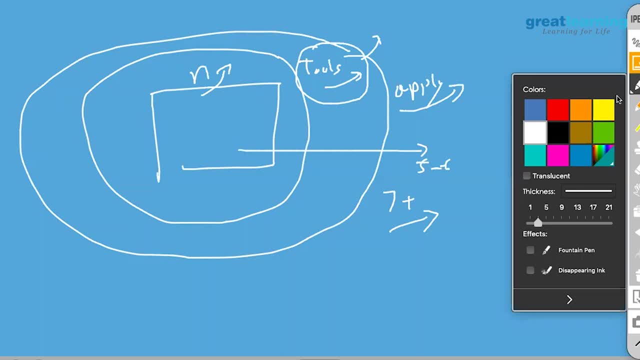 so all i would say is start applying these techniques directly onto your project. whatever data you have as a poc, i started like that. take out any data, put some machine learning, let's try to find a value out of it and propose it to your client or project, whatever you can. 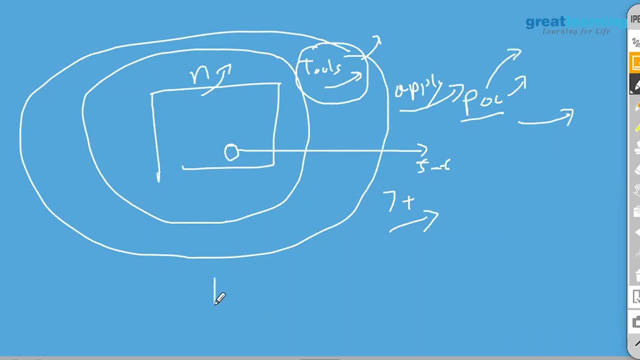 this is how i feel you will learn faster, as compared to if you wait till end of the certification and then you start applying. you know the certification is going to add end, let us say, in January. so whatever you have done in july, may, august and all, it's not necessary that you can recolect everything. yeah. so this is my daily stuff. that's why i know SVM and all on heart. but let us say i don't touch svm. i when i say i don't touch it раз. everything that you do, please take change can be done. it's just you've shown everything you're familiar with. yeah, so this is my daily stuff. that's why i know svm and all on heart, but let us say i don't touch it ever. you may try and give me that few things, nothing to learn, or you can read this while and then try to answer it. 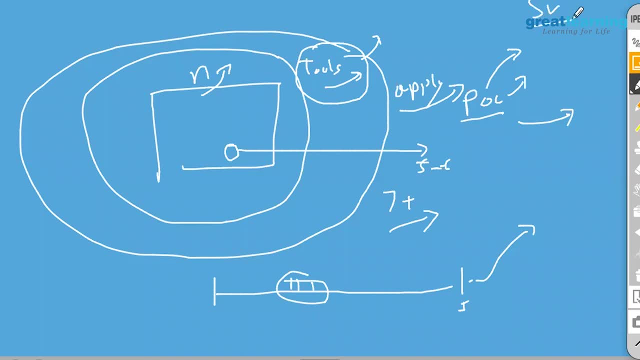 stuff. That's why I know SVM and all on hard. But let us say I don't touch SVM for one year and then I visit back. It's impossible for me to recollect, Okay. So that's the reason I say don't wait. 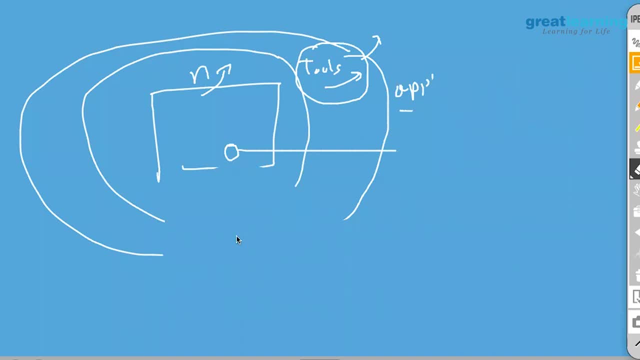 Start something, If, in case, you want some work. if in case you want some real work, do contact me. I will give you some live data sets to work on, Okay, So if in case I have one right away, I'll give it to you. 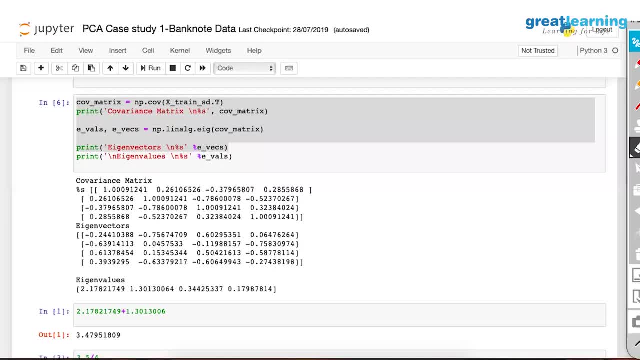 That'll be awesome. So they are into recommendation model and AI part of it, So hence I'm giving them. But if you guys really want it, then I will show you those work today. You can take your time. This is an industry. 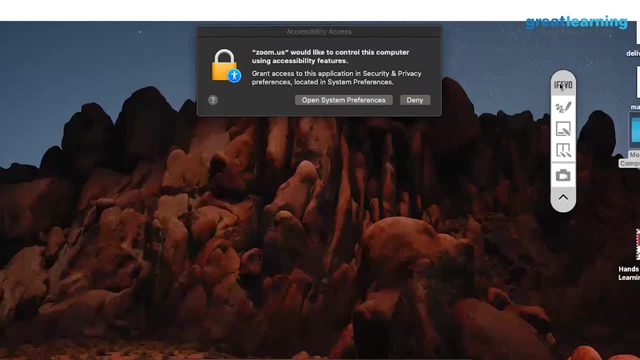 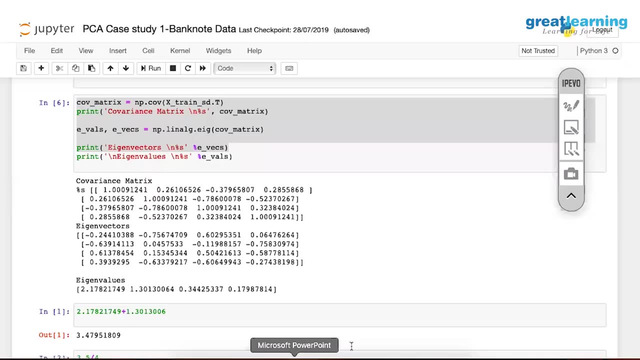 work. You can take your time and get back to me. I'll be very happy to share. Nothing wrong, Yeah, So you want to do that, or should I show some of my extra implement? What do you want? You want to take? 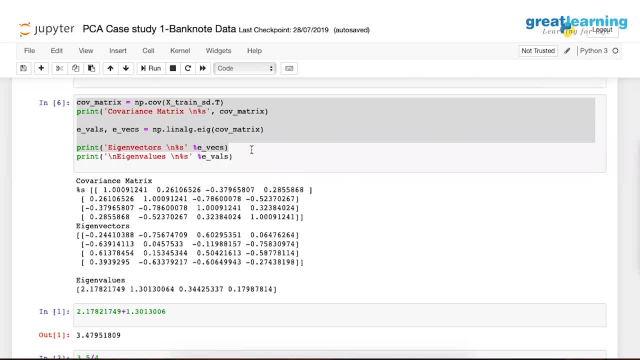 up an extra work, kind of the real time work, or we will do it post VM insurance, So whatever you like. Yeah, You were saying that you have some model that you've built for employee assessment model And stuff like that, Using PCI. 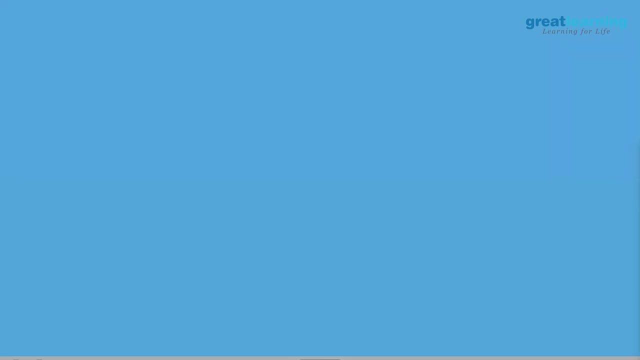 Yeah, Okay, So let's do that. So first I will do one thing. I'll give you guys the concept of it, What exactly and how I use it. So I do not use PCA here as dimensionality reduction. The normal silo for PCA is dimensionality reduction. 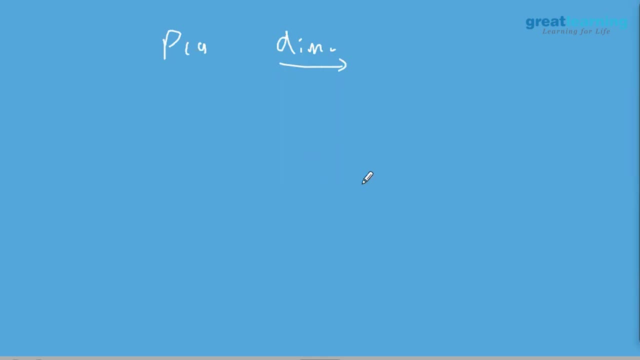 I don't use it for this particular application as that Why? I'll tell you. See, what I've seen here is in my org. we have got KPI And each level there is a different KPI. So let us say, if we are talking about 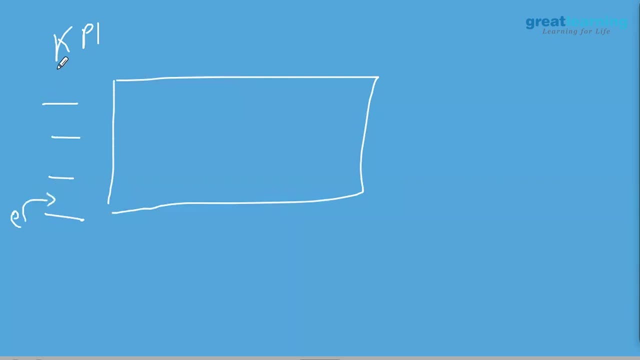 an entry level, the person who is in KPI, is a little bit different. The person who is in mid level, his KPI is a little bit different. The person who is on managerial level, his KPI is a little bit different. So what happens is every. 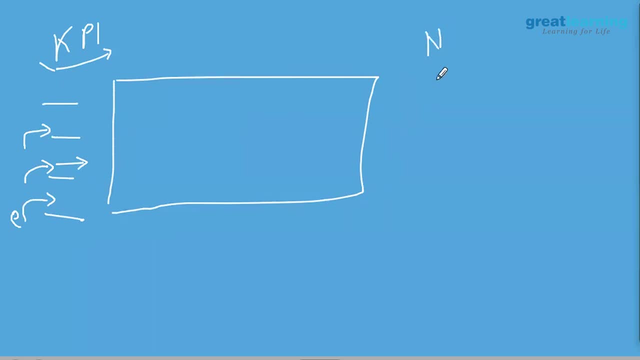 year. twice a year I have to assess- my sorry- the people who are reporting to me Now. there might be some mid-level managers reporting to me. There might be some freshers reporting to me. There might be some different level of people reporting. 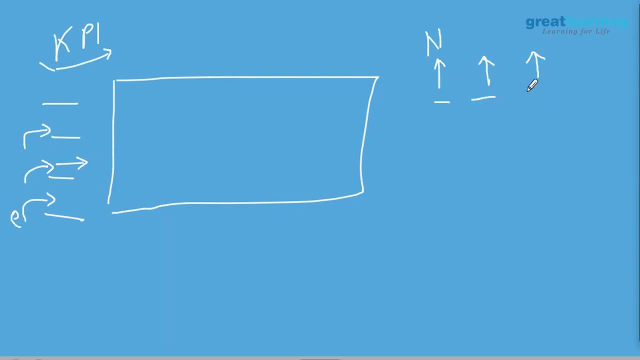 to me. Let us say So. it's not like sometimes it becomes. how we do traditionally is on impression point of view. First of all because as they report to me and work with me, I clearly know who does what, So depending on that, I can rate. 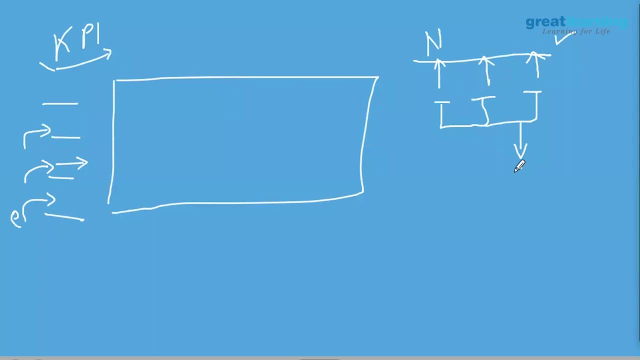 them Nothing wrong. But what happens is at the end, when the ratings are published, and, as a human nature, what they do is they try to communicate with each other how much they got and what they want. Okay, In the worst case, even it goes up. 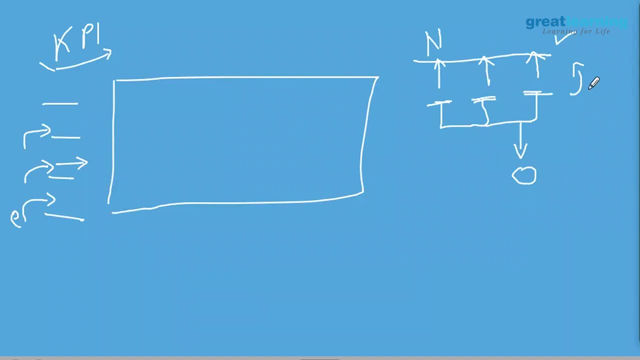 to other numbers and all which I don't want to talk about. So what happens is at the end they raise an what do you say? change request, and then it comes to me And then I have to somehow fight and negotiate and try to. 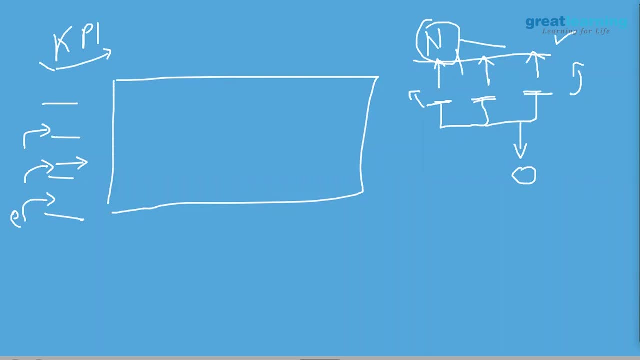 pacify them and close it. Okay. Now why do I feel we can apply this concept here? is PCA is the only algorithm or technique that I know which has covariance matrix so far. Have you seen this anytime in any other algorithm where we are comparing the same? 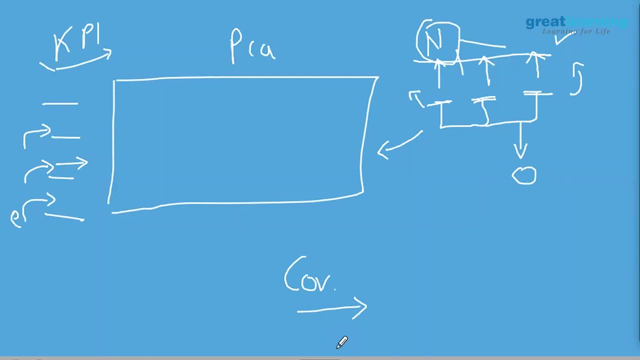 variables within themselves. You know we are trying to create a matrix, a dependency kind of matrix, how each variable is dependent on other variables. Correct, Right Now. why do I use this? So now, keeping this covariance in mind, let us say you have got an. 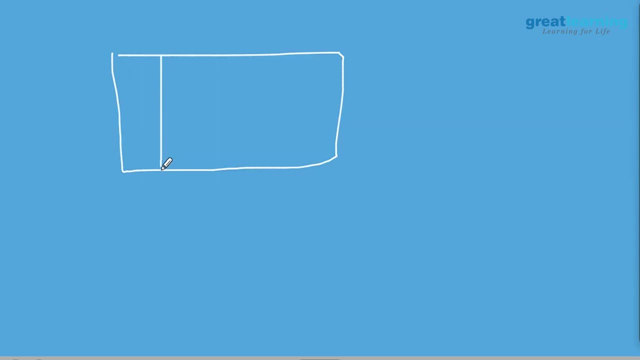 employee data. Okay, This employee data has what? let us say it has, what level that employee is on. Let us say how many. what is his average working hours, for example, What is his total leaves taken so far? How many modules he has developed? So let us. 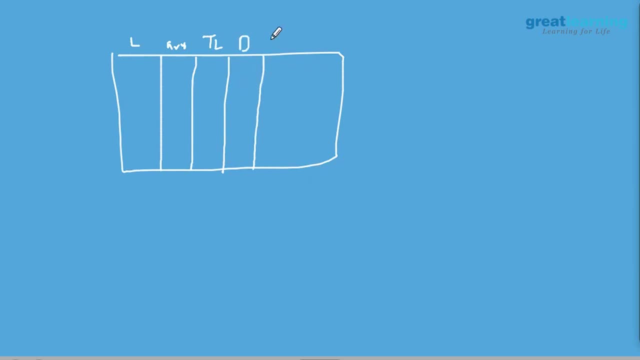 say I'm coming from a DevOps environment, basically. So I'm talking about how many releases or modules he's developing, for example, If, in case, he's in testing, how much he's testing If, in case, he's putting both the roles. 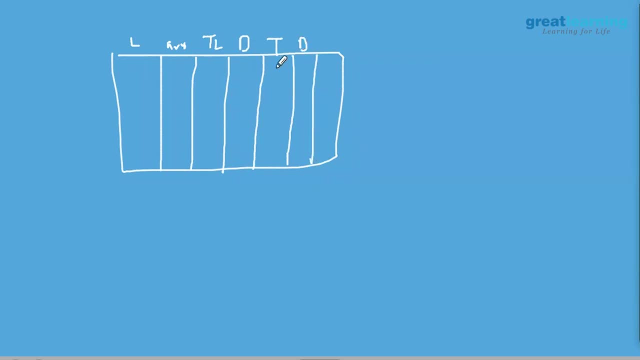 how many defects are getting produced because of his coding or because of his testing? How many escalations the person has? Is he cross-trained himself this year? Okay, For example, if an employee leaves, can I use him for other purpose or not? 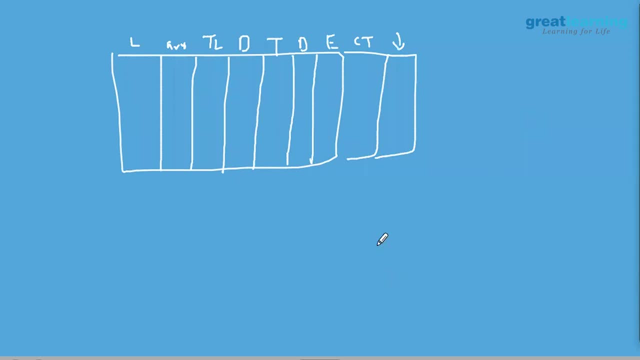 Else, how much business is bringing in. Let us say, if you guys have heard about what we say as like, once the SOW is signed, we can, you know, give some enhanced, enhancement to the client and we can update the SOWs correct. How much of these? 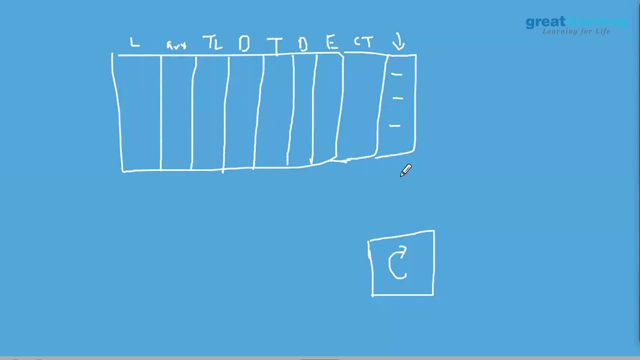 automation enhancement that employee has brought in. We just brought in more money for us. We can have multiple areas in which we can build a common KPI. See, I'm not talking about single KPIs. KPIs in sense, key performance indexes. 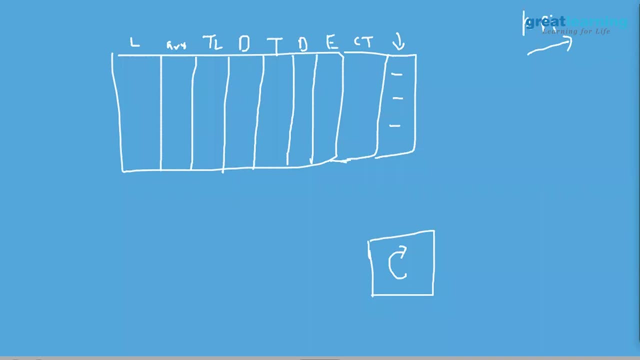 And every level has a different KPI. Yeah, So what I'm trying to do is I'm trying to find certain similar KPI which I can rate all of them together. Why? Because, at the end of the day, when I'm 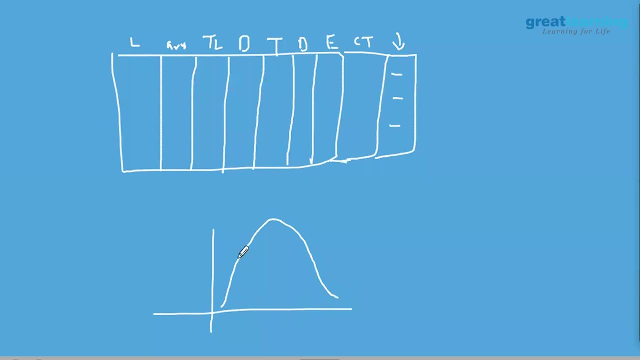 rating them. I have to follow a bell curve. Agreed guys, Correct. I hope you guys are doing the same in your org, Where 20% will be rated least, 20% highest and remaining whatever we have will be a mid-level rating. But we are putting. 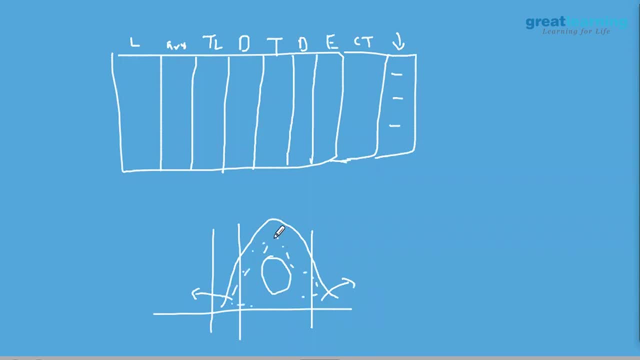 all the levels of employees in the similar bell curve. This is my bell curve, My boss will have my and his report is bell curve. His boss, a VP, will have a different. So we are not talking, We are not basically trying to segregate this. 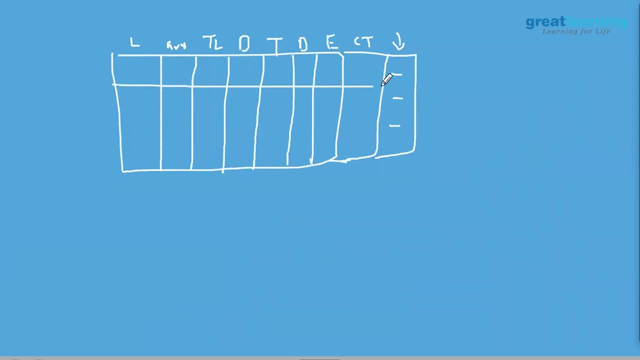 So what I did was I did this model where we have got a lot of employees. Now what I'm doing is I'm generating a covariance matrix out of it. Now, the covariance matrix that I get now and eigenvalues that I get- I built up a formula called 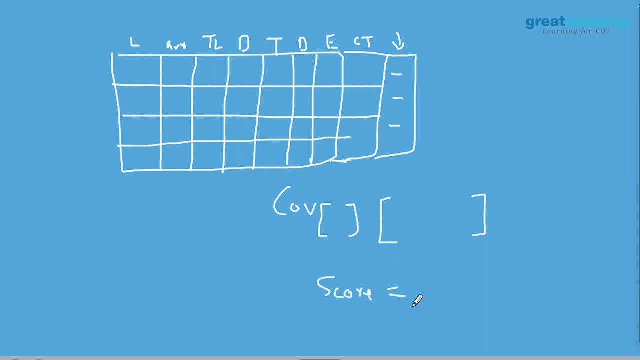 score, Score. as per my formula, a score is nothing but an eigenvector. Okay, Into square root of eigenvalues: Yeah. So when I did this particular formula onto each employee, I was able to give a target variable to each and every employee. 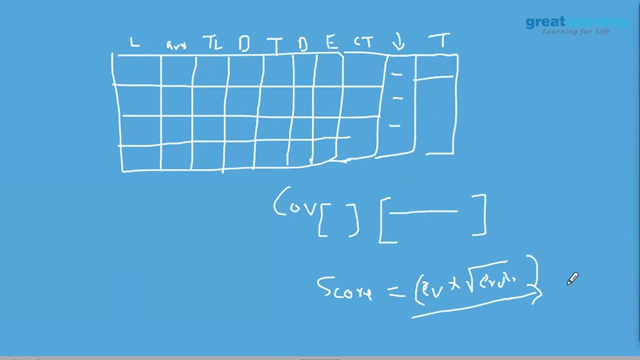 That target variable was, if you see the dimension of this. dimension of this will be one cross one. That means it's a single digit, continuous number. This will be a score between 0 and 1.. Yeah, So now what will happen is depending on good things. 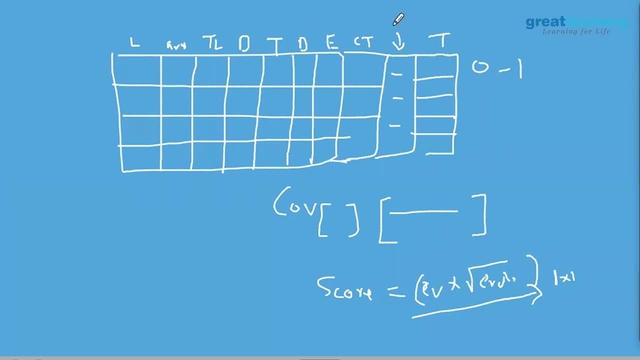 So let us say good things are what. total number of enhancement proposed? It's a positive. Think total number of leaves taker is what a negative thing. So what I will do is I will try to adjust this column. Let us say my an employee has taken 23 leaves and my organization 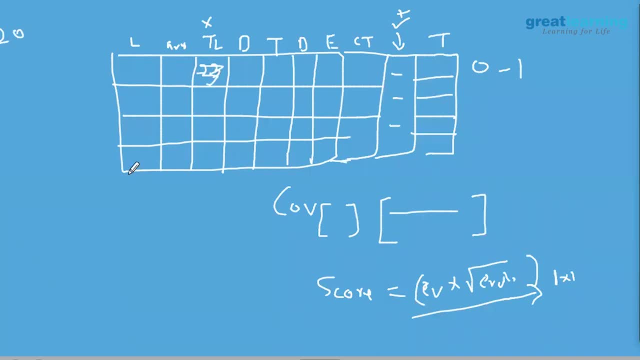 allows 20 leaves. So what I will do is I will make it negative three for correct total number of escalations got. if, let us say, 10 escalations, I can say I allow only two escalations. more than that, I will negate it. 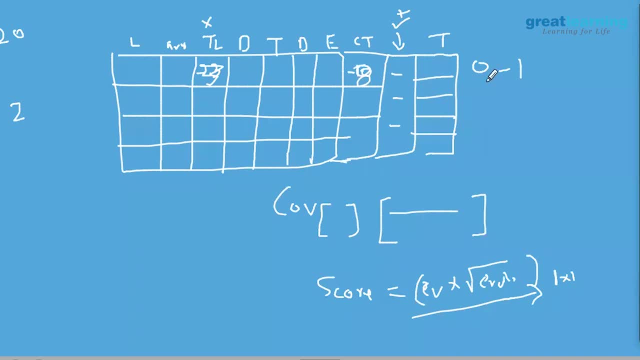 I will negate this values and I will correct it. I'll make it minus. So what will happen is covariance matrix. It's will penalize employees for having negative value here and give good score to an employee for having a good value. That means I'm trying to find a correlation between all the variables. 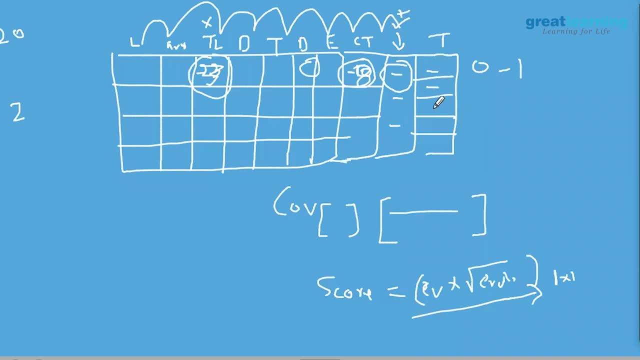 Got it, guys. So this is how I found out a way to score them up, And now, when I, you know, put in a descending order, I can put my weights, or else, if I generate a curve out of it and want to get a curve something, 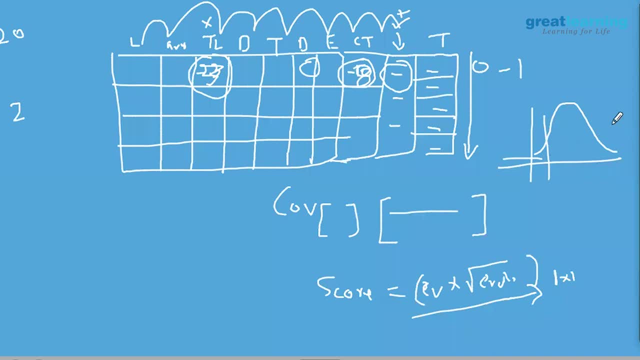 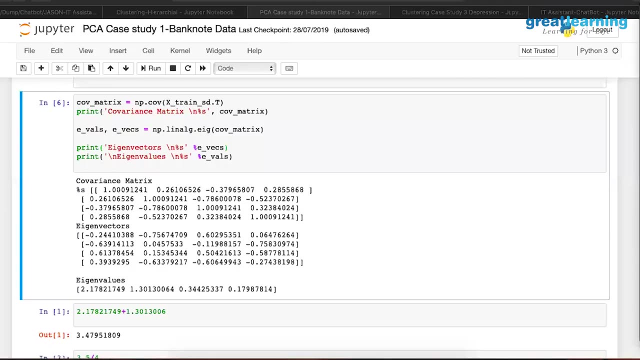 like this, agreed. So for the people who lie here, I'm going to give this. for the people who lie here. I'm going to give this for people who lie here, and very simple. Okay, Now, if you want to see it, give me a minute. 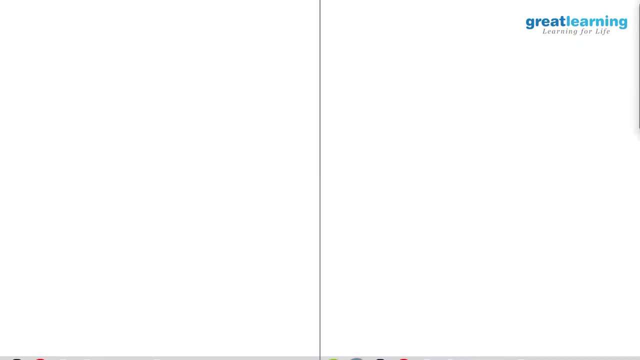 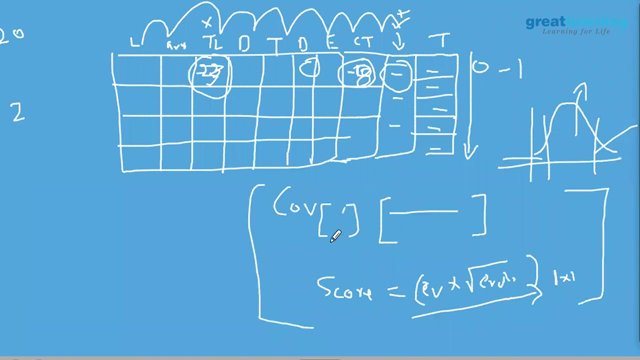 I have to pull up that code. Okay, any confusions here? First of all, theoretically, did we get it? Are we able to correlate? I am not going to the reduction here, I'm not using that. So the the formula that you put, the score formula, is a standard formula. 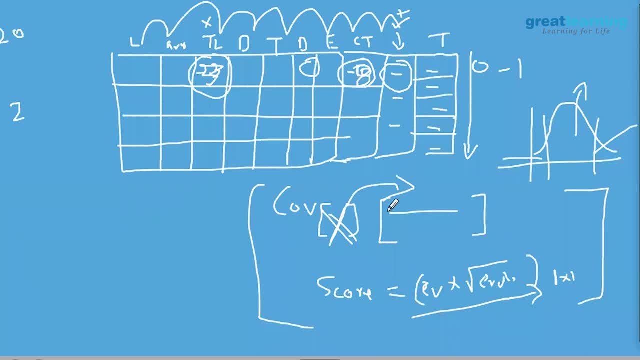 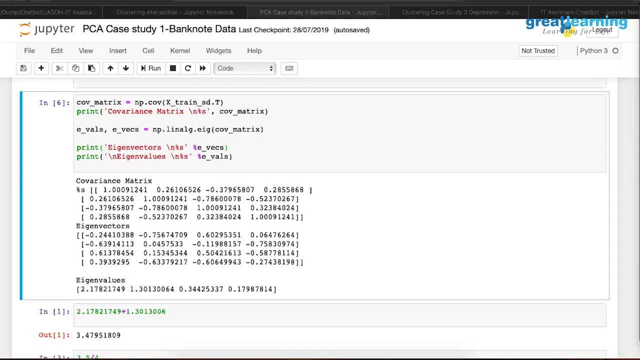 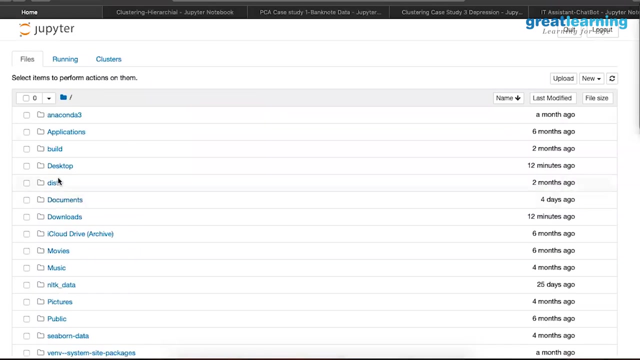 Is something that? no, it's my own formula, research. So you can play around with this formula: Yeah, Okay, Okay. And in this you know, now that you said this, for example, the same example that you said- a value that someone brings in should be weighed. 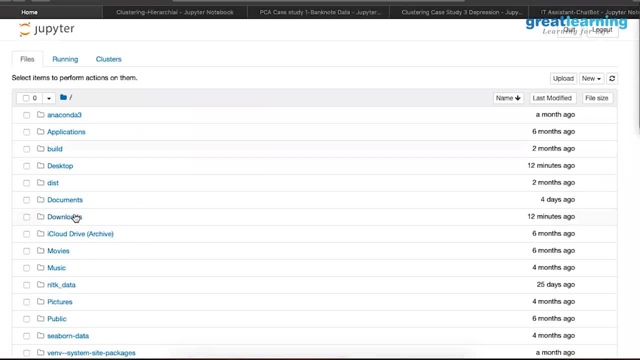 lot higher than, say, a sick leave that is taken because that's you know. so so is there a weightage that you give? can you? can you give to a column? We can do that. Yes, We can put a filter on to that. 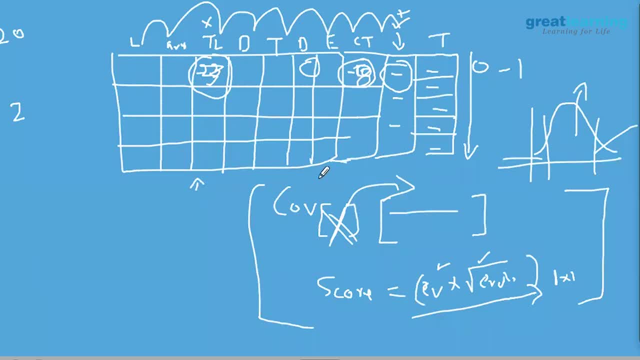 Yes, We can put a filter on to each column If, in case, you feel you need it, Okay. Okay, There's a field we can do a lot of things, see, as a part of data cleaning. I'm here to do with you guys. 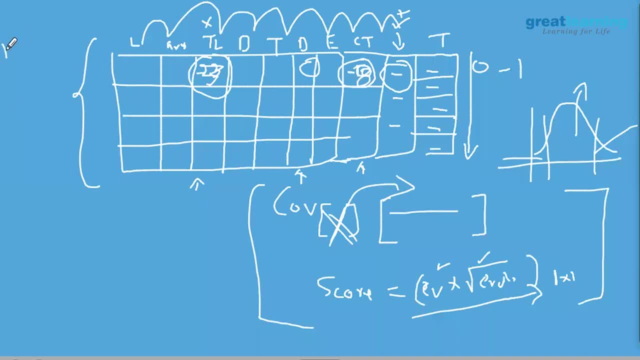 I'm not finding time on to that. as a part of data preparation, data validation and data cleaning, We can put a lot of things on to this. We can put threshold values. You can put filters on to that. We can even replace values depending on them. 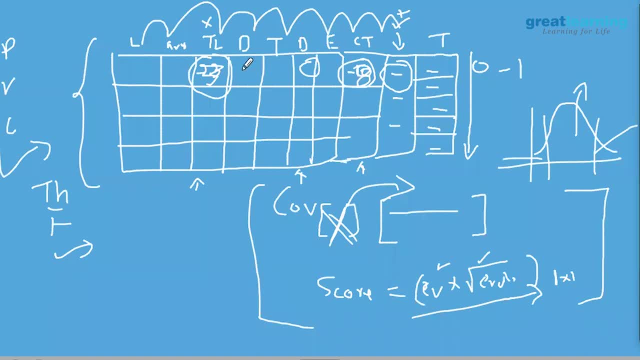 So let us say number of. let us say if you're talking about, you know the deployments. this person can deploy letters, 500 deployments at near, but if you look at the number of enhancement done, it will be only one or two. look at the mismatch. to avoid that, even we can scale them up a lot of. 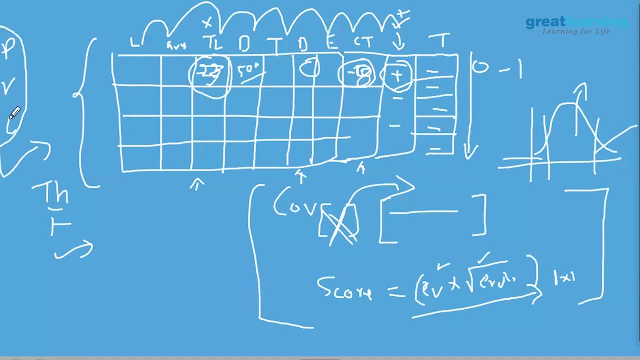 things you can do. So I'm yet to do this with you guys. in this particular session I'm trying to find one empty slot, So there will be one. last week I don't know why I missed it, but I could have taken that slot. 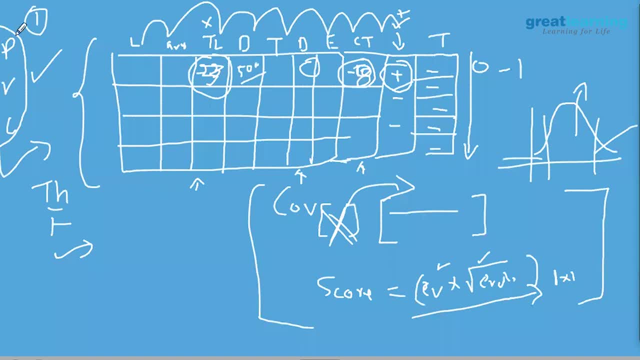 So now in next session, when you are having an empty slot, no, I will definitely take one session on these three techniques at least. Yeah, So I think in that session you will have a lot of how we can set up values. 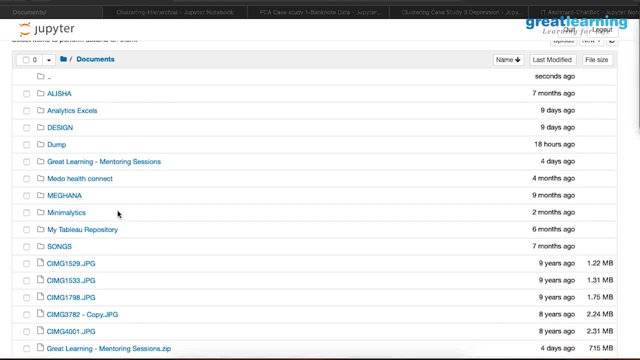 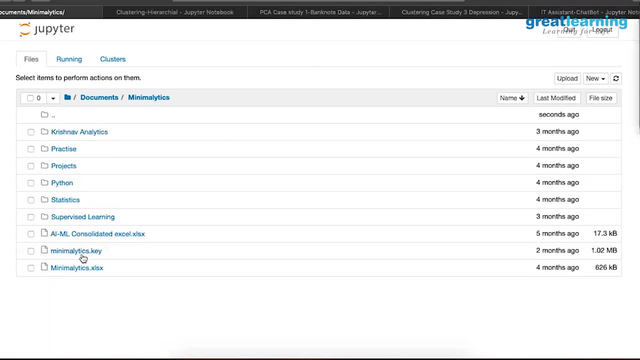 Awesome, Yeah, Okay, The idea as you pull it right. one question that we have- I think we had been discussing the group also: When do you create dummies? Is there a thumb rule to create? Is, if it's a text column, that's when you do that, or any any rule on? 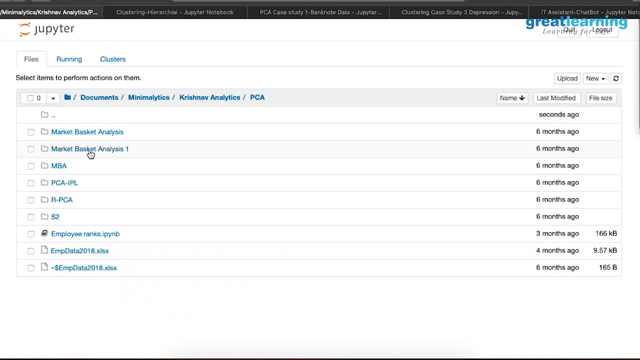 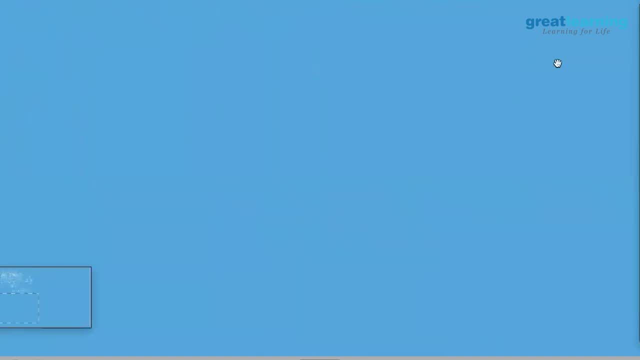 that dummies? Is that function you're talking about? Yeah, the get dummies. you know the, the classical, sorry, the classification variable, column, column, right. So when you get the, okay. when to do dummies is very simple, is sometimes. 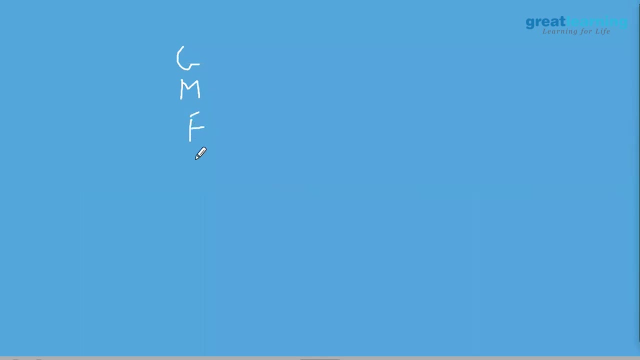 what happens? and let us say you have a gender column, Okay, and let us say you have marital status, called, for example, married and unmarried, for example. So one way you can create this. basically, let us say you are doing linear regression on to this. or let us say you are doing classification. 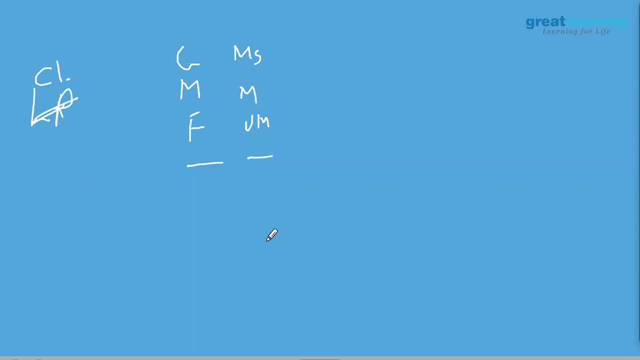 on this. What's going to happen? You cannot use this values. So what you will do as a normal person, What I can do, is I can convert this into two separate columns. correct, Correct, guys? So if this is one, this will be zero. 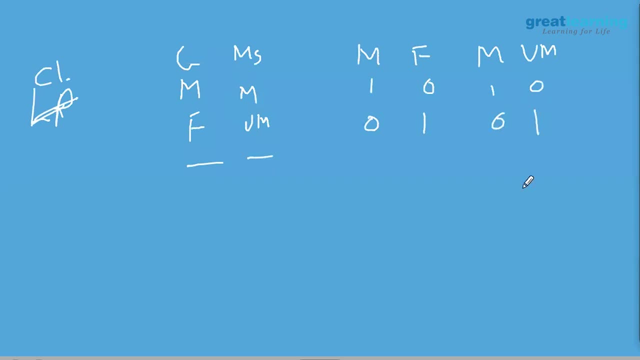 If this is zero, this will be one similar. is the case here, Correct or not? Yeah, You can do this. You don't need to do. dummies function, It's okay, But what's going to happen? Can I say these are highly correlated to each other. 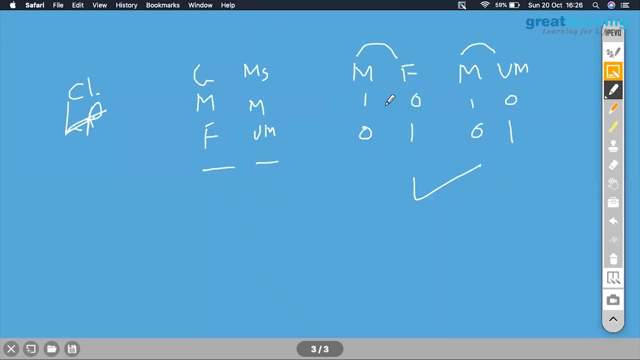 Yeah, they are there. later They will Mitchell exclusive right, Exactly. So in this case, what to do is using dummies function. It's easy for us to remove one of them and keep only one. Yeah, So again, I will say: there is no specific rule that you should use only. 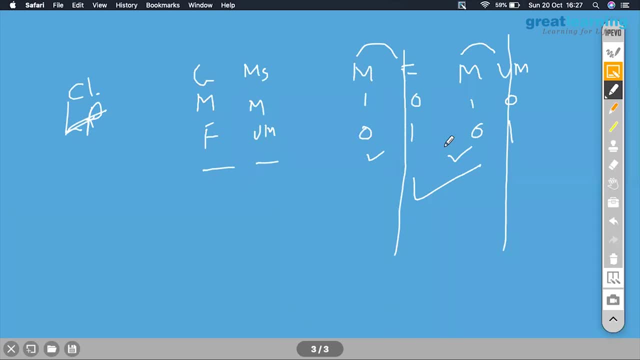 dummies, or you should use only dot replace function, Or you should do one hot encoding. There are three techniques. Okay, you can do one of them. There is no rule that. okay, you should use only dummies. Yeah, That's the third you said. 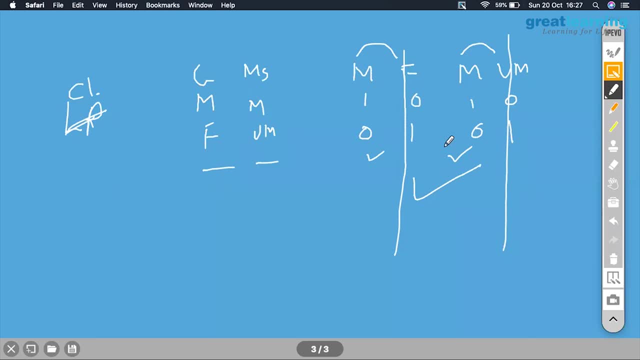 So one is dummies. The second one is we kind of encode it, as you know, one form. if you have heard about, sorry, dot transform function, Okay, Okay, I will show it. Yeah, that is changing male to one and female to zero, something like. 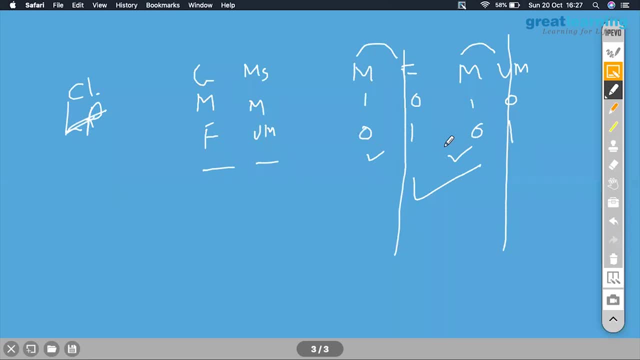 that right, Yes, Yes, Yeah, that is the second third. one is third one. It's called dot replace function, So you can write your own dictionary. So let us say, I put my own dictionary. If you find M, replace it by zero. 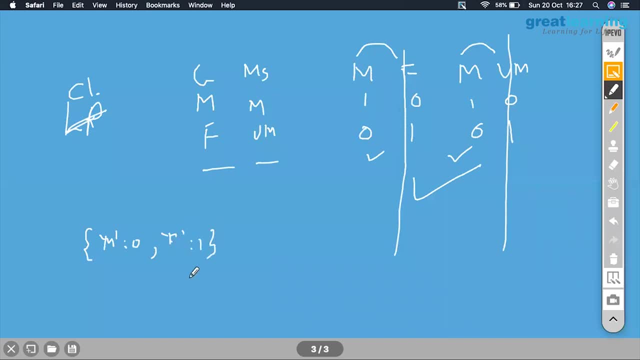 If you find F, replace it by one. It's a. it's an old-school technique. See, if you do dot transform technique, or if you do dummies function, right, Okay, dummies function will leave it. if you do dot transform, What is going to happen is on alphabetical order. 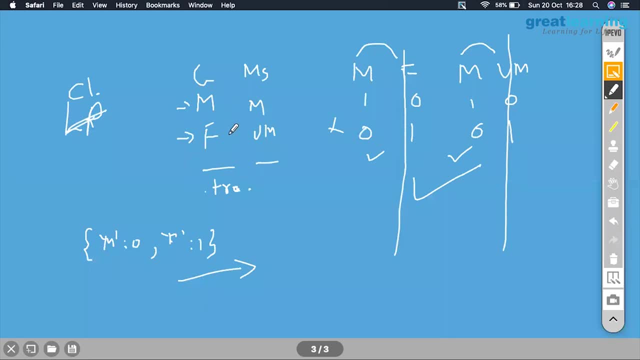 It is going to pick it up. So F comes before M. That means it will be zero. This will be one. If you don't want to do that, if you want a specific one to be replaced, you can use a dictionary to replace, or you can do dot, transform, or you. 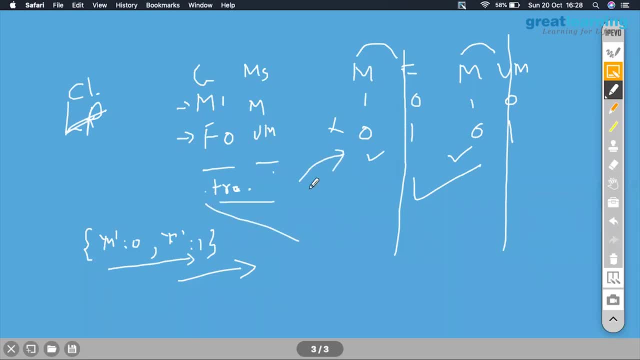 can do dummies. If you want a clear difference between all three of them, I will show it to you. next session We'll take up one data set and we'll use all three of them and then we'll see what how it's different each one. 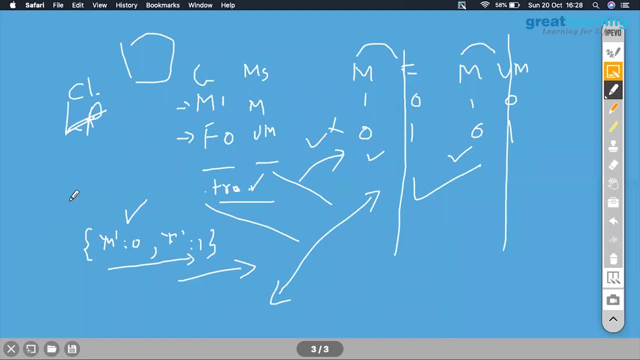 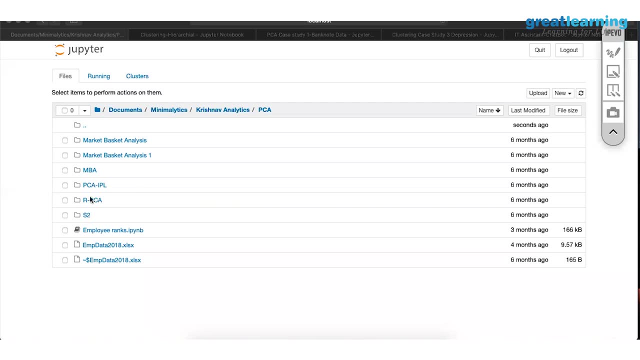 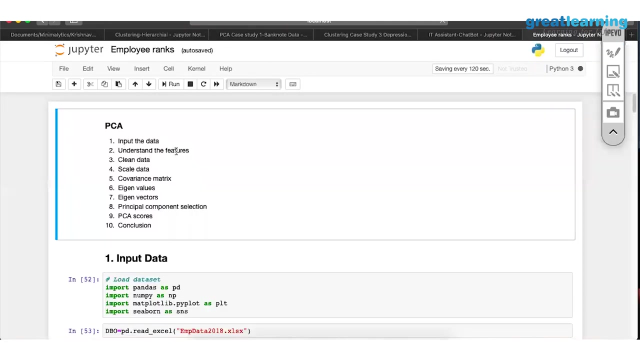 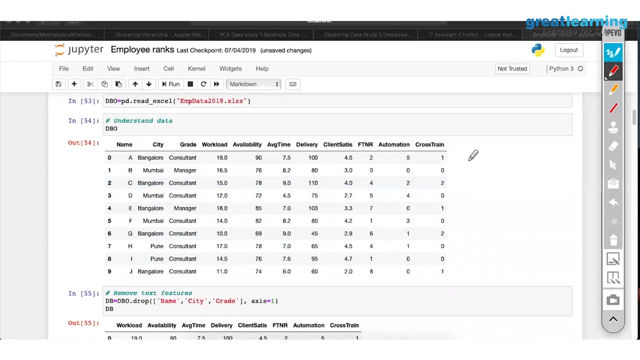 Okay, Perfect, So was I. I was finding that PCA. where is my PCA market employee ranks here? Here it is. Let me check whether it's the same one, because I made some modifications here. So let us say this is my dummy set data set that I have, and as I 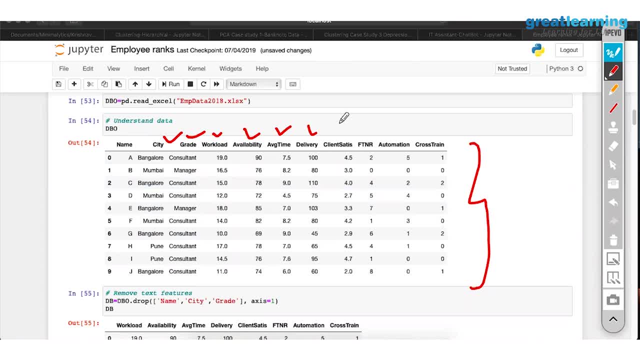 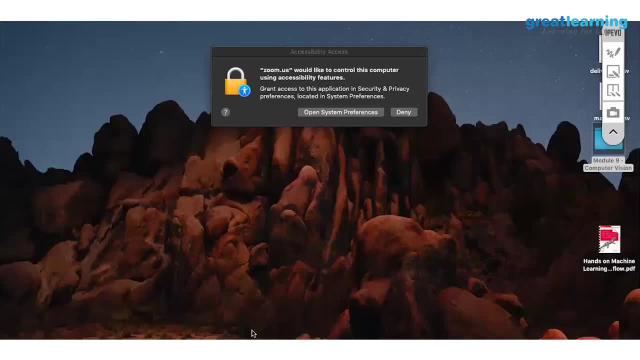 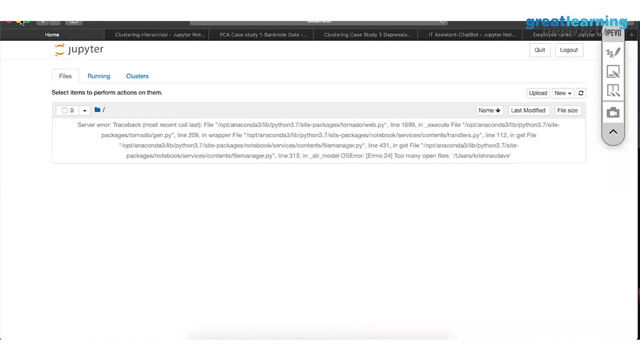 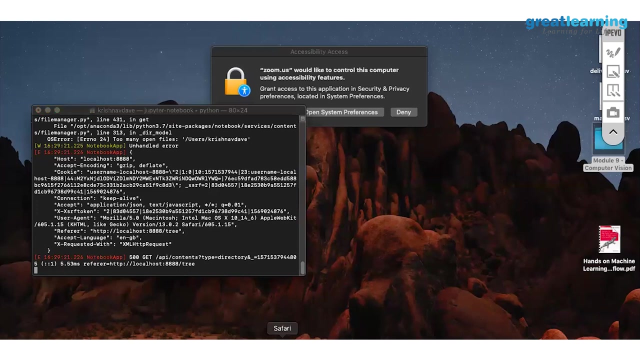 said, some of these attributes might be similar for almost all the persons. Yeah, I think. still, this is an older version of it. Give me one minute. This is an older version for sure. My net, What happened? My python died. Okay, give me one minute, guys. 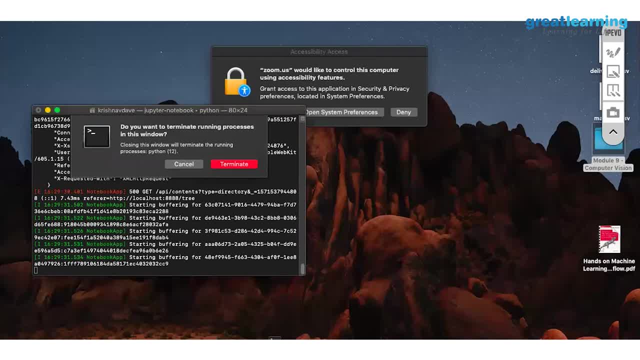 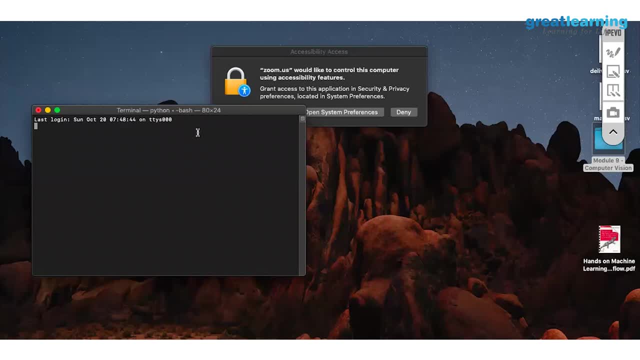 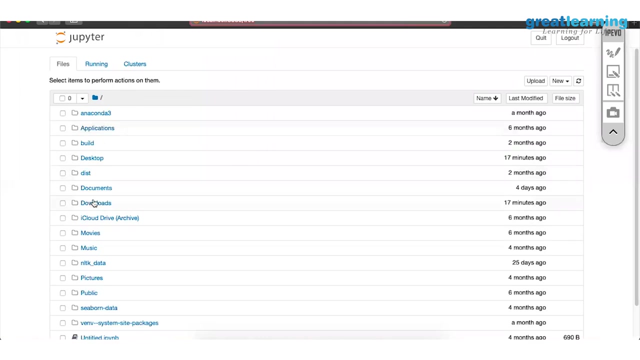 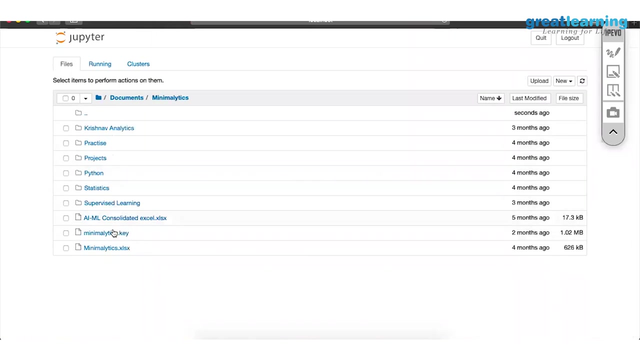 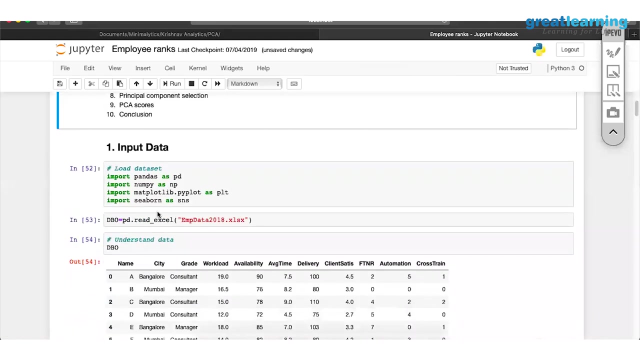 My python died. Yeah, Good, It's working with the documents. PCA. Okay, Okay, I think this, This is an old one still. I'll explain you this, but for actual implementation I'll pull it out. I think I have stored it somewhere else. 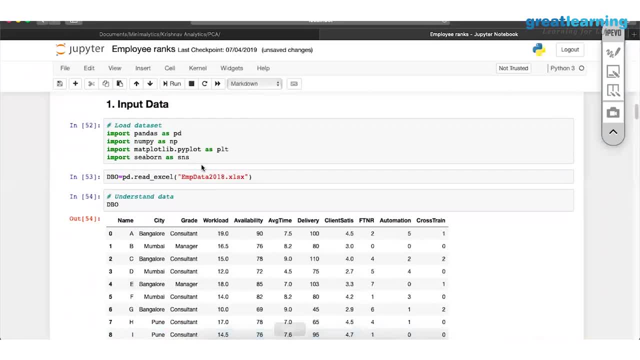 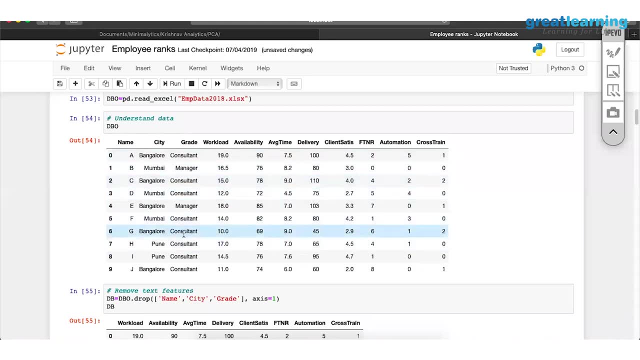 Python is working or not, So we show it my python. Okay, fine, So look at this data set that I have. there might be various fields onto which you can do it. Yeah, Again, I am not considered these two, Yeah. 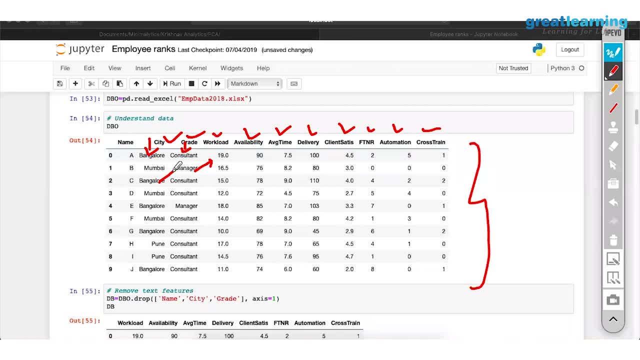 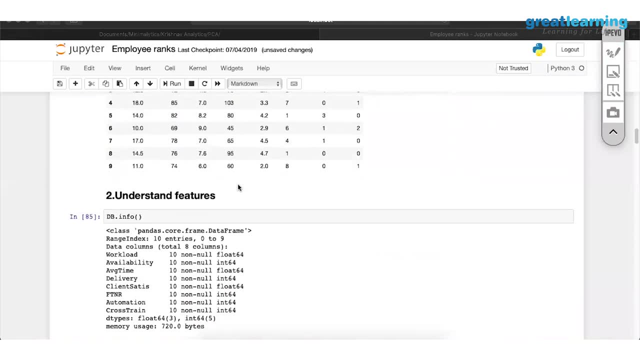 So what you can do is you can do one hot encoding, or you can do dot transform or whatever extra things you know You can convert into numbers. for now I'm ignoring these two parts. Okay, next, what I'm doing is I'm directly generating the covariance. 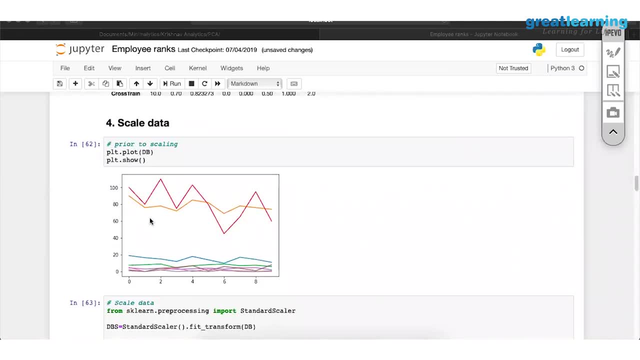 matrix. So first of all we should check how the data looks like. So when you plot the data simply, the data looks like this: That means some of the variables are having high values. We cannot blame them. Why? because the nature is that way. the units are that some of them. 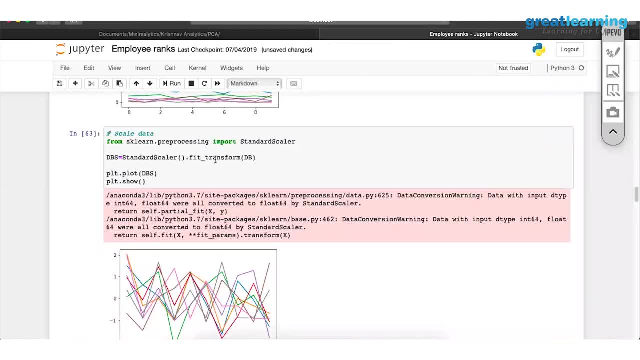 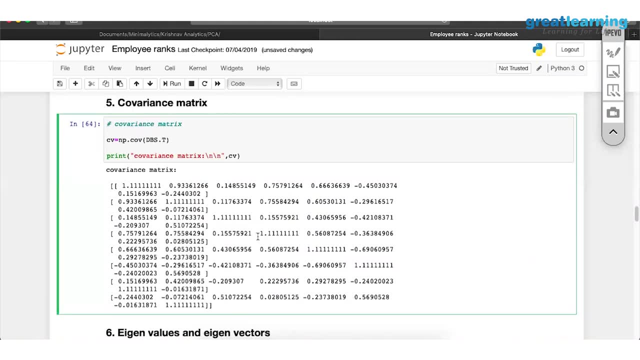 are on a very low level. So the first thing I understand is to scale them. So when I scale them, you can see that we are somehow bringing everything together. Yeah, post that. you generate your covariance matrix. This is my covariance matrix. next to that, eigenvectors and values. 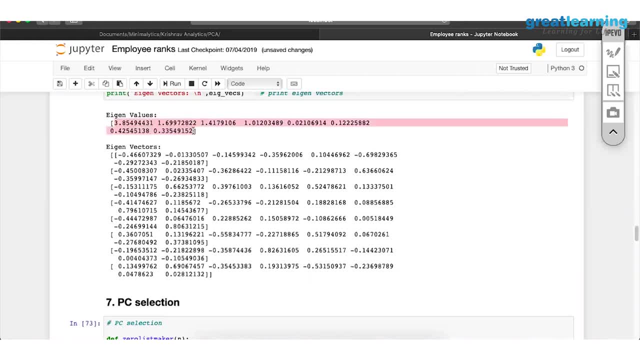 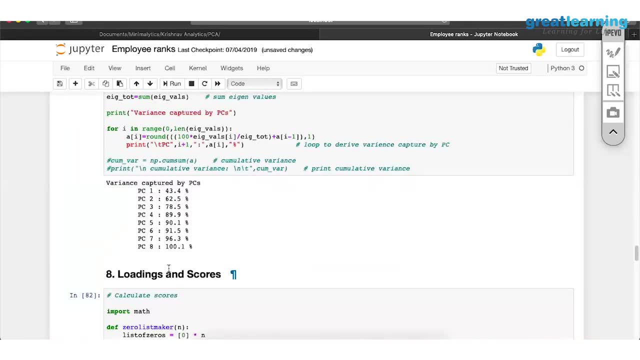 So here we are doing it, But, if you observe, I'm not using them anyway. I'm not using the variance dimensional reduction, and I'm just using both of them. Yeah, next, just to show how each PC behaves If you look at it. if I say 96% accuracy, I want I have all the 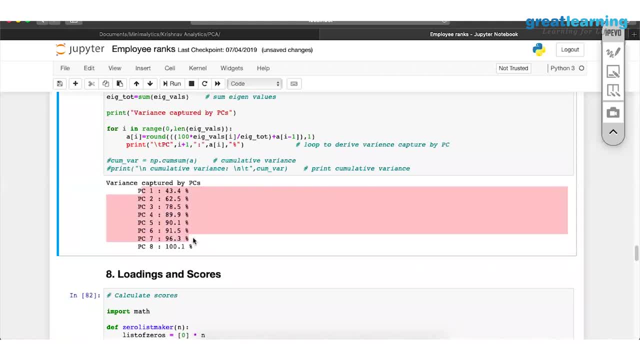 pieces working. That means all of my features are highly important. That's what it shows. So I have a. I have a little odd habit of, you know, catching the ear in a wrong way. So if you, if you see, a PCA is for reducing the dimensions, my take. 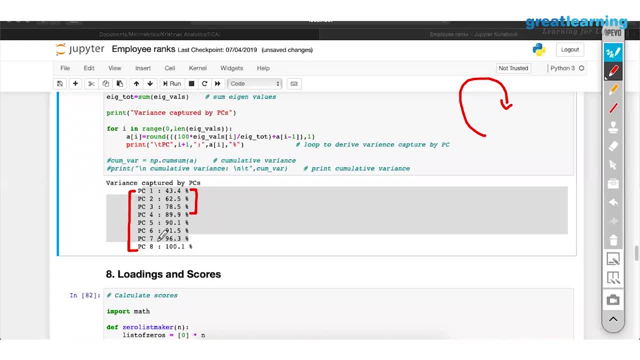 is. I'm trying to identify which are important dimensions In this case. you can see, to reach 96. We have to go up to almost seven out of eight, So that means almost everything is important. We will not reduce anything for now. 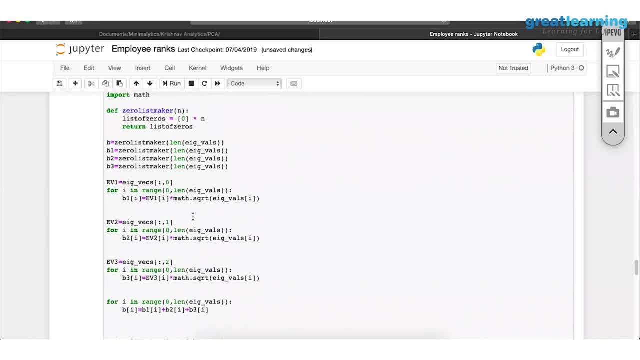 Next is my scores. So for the scores thing, what I'm doing is I have done a very simple formula: eigenvalues into square root of your eigenvectors, into square root of your eigenvalues. So when I do that, if you observe, here I've got a score. 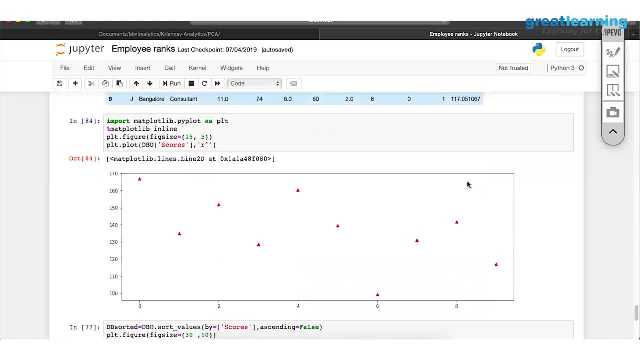 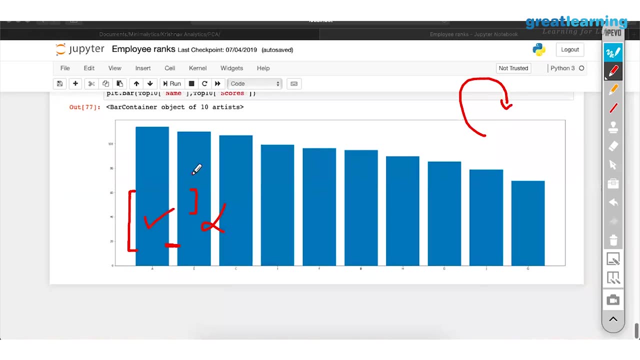 And when I, you know, format the score or when I plot it. for example, if you see, here I can easily say that employee number a should be rated the best least, next, next, next, next, next, next, next, something like that. It's a very simple implementation, but it solves a real-time problem. 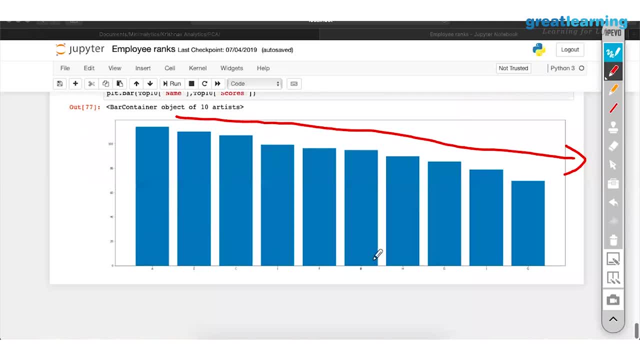 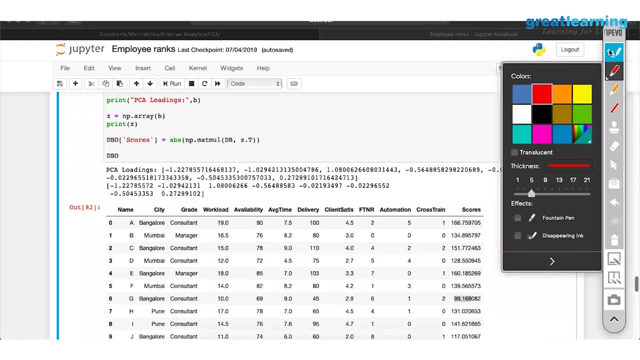 Now some of some of, let us say, your superiors might come in chat. You can vary. You can easily say that this core is a mixture of relationship between this particular employee. Okay, with respect to all the available Numbers here, Got it. 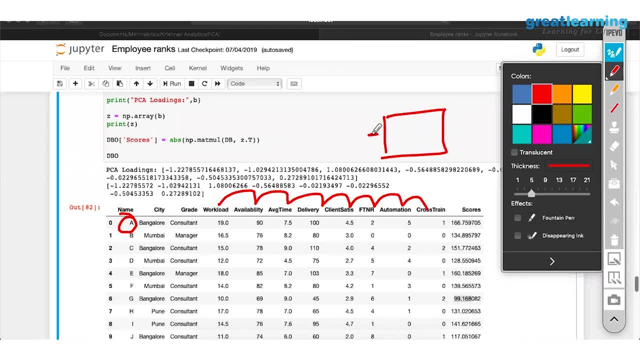 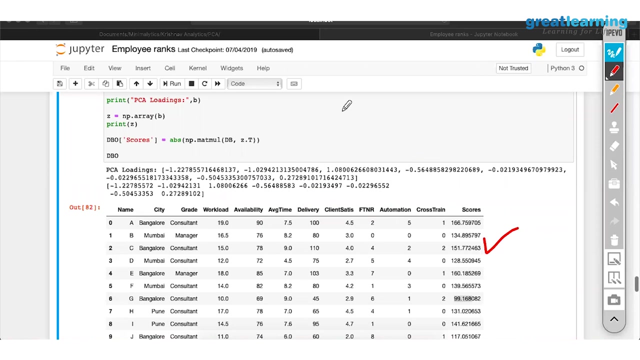 It's like a square matrix which tells me how my employee a is behaving with workload, availability, average time, delivery client, blah, blah, blah, blah, and in turn, we are having all of them plotted onto one graph. Okay, so you can do this on to your employee ranks, even if you remember. 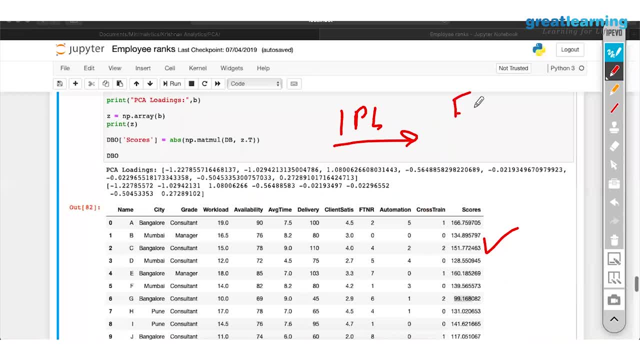 these IPL, or if you talk about FIFA, These clubs know, if you remember, guys, these clubs are attached to this data science companies. If you have heard about recently, nowadays, the person, yeah, so if you have seen that movie- Brad Pitt movie- I forgot the name of something. 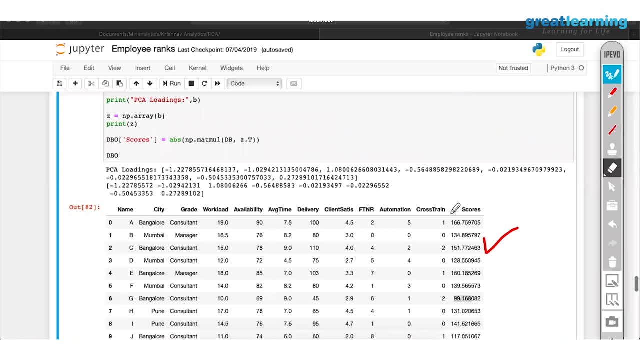 like that. nowadays, There's a trend whenever these sports thing is going on. So if you see IPL ranks, I feel That they are somehow using a hybrid of this to do this. I'm not saying they're using my formula, but they are somehow using a covariance. 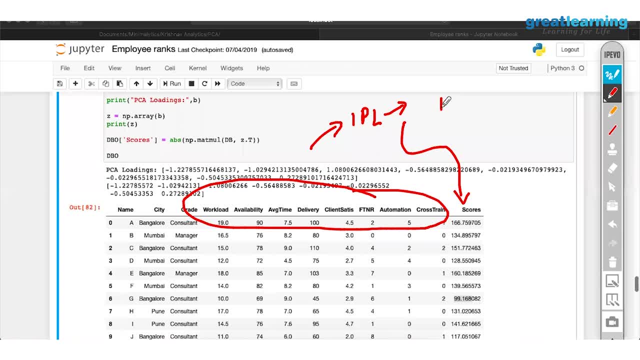 matrix. Why? because nowadays there are a lot of this, what you say, all around us. So nowadays you cannot see only batsman and bowlers, Yeah, So in that case, what they are doing is they're trying to cover everything So related to that. 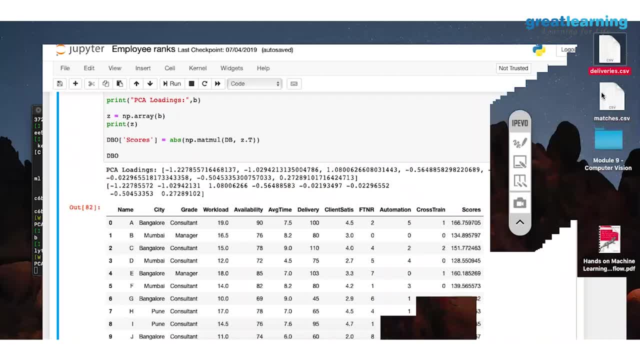 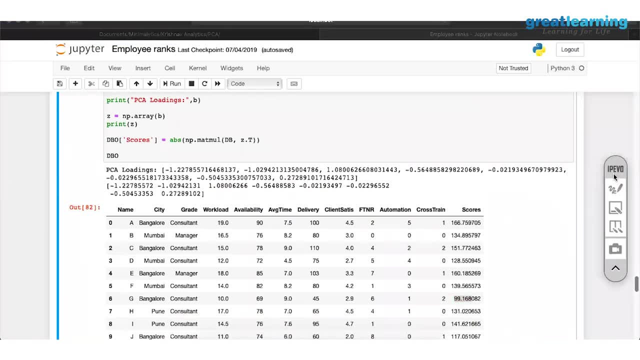 I have what a simple project here with me. It's a similar IPL project, only It's a live data from IPL website Where I think I will show you guys next week. You guys can kick start on that and start working on some business. 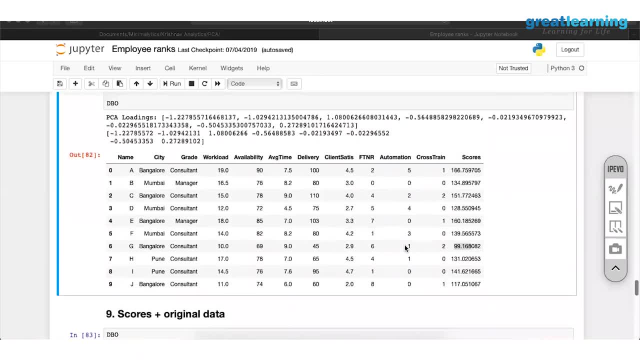 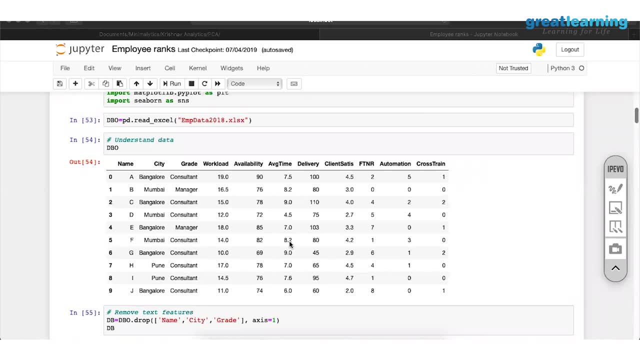 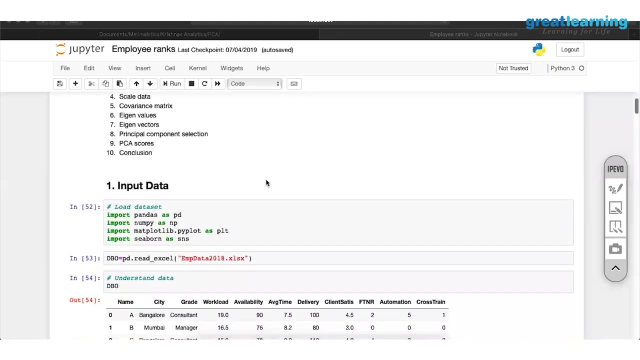 problem: How you can use a non-targeted data. So this is a non-target data: how you can make use of a data like this ones. Okay, I share this implementation with you. You guys can try it out yourself here, Okay. 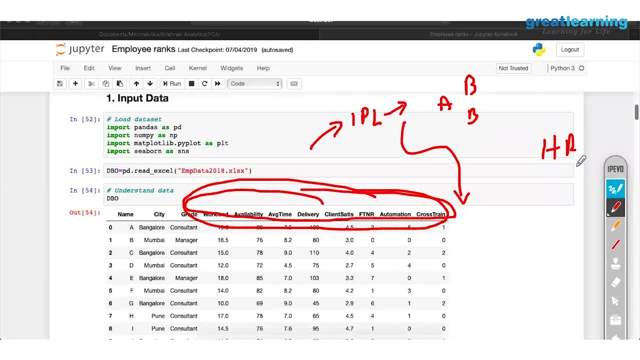 I will say it's a part of it. Super, Yeah. So the only the only challenge, Krishna, just to let you know. So we, I've tried this a couple of times, but manually, not in Michigan, but the only challenge, biggest challenge, is collecting data. 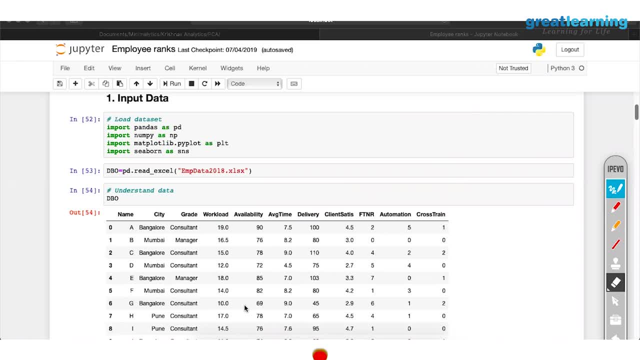 Yeah, You know that because I've done all these magic. Yeah, nothing. Nothing gets into the excels. in this case, The manager has to be proactive. So what exactly exactly I proactively do this? My HR does not give me this data. to be very fun. 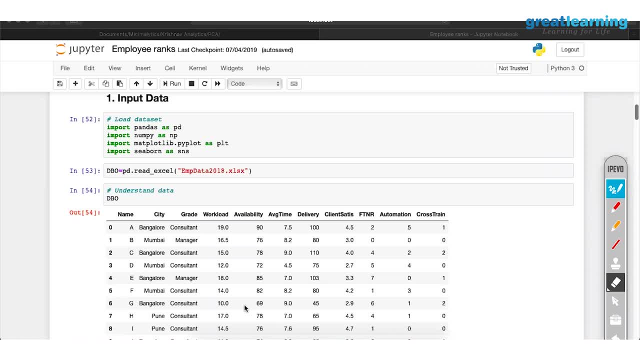 Yes, you're right. Okay, perfect, Okay. anything else, guys, you want to know, Everything's good. So we are running one week ahead now to be very funny. Yeah, you're right, Because last week's this decision was supposed to be clustering, clustering. 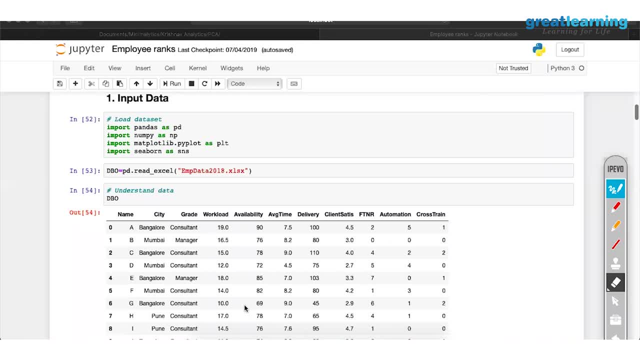 Yeah, So please be clustered Habitually. This is my pattern. See, what happens is when you see something for the first time as a video theory- This is my personal- you have to see those videos two to three times to be very fine, to get it right. 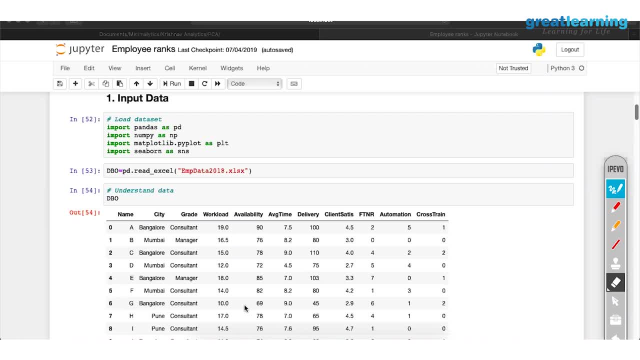 So what is my pattern is? I will walk you guys through one week ahead. It's so that when you watch the videos it is flawless for you, and yet I will not compromise on to any of the extra topics that we cover. So if you see, today we have taken two industry sessions. 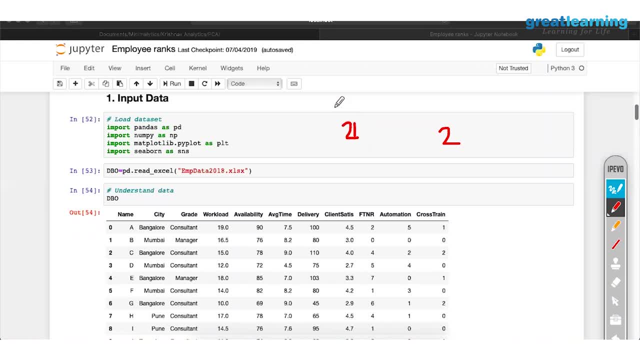 And one- sorry to once- one on clustering, one on PCA and two separate modules on some extra stuff. So I'll make sure I show you this also. plus, I keep you guys one week ahead. This is what my pattern is. If you guys are okay with it, I'll follow it, or else we can run parallel to it. 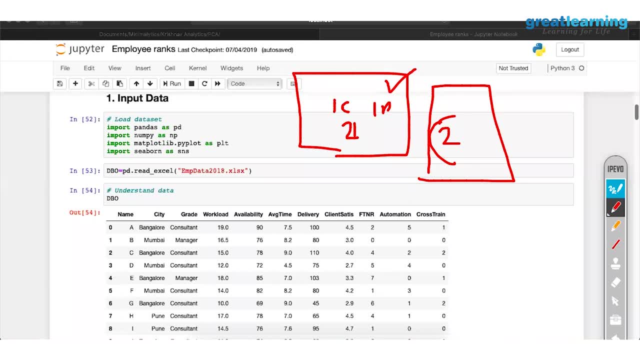 Nothing, Nothing wrong. One thing I would like to ask, like more, that we were telling that you don't concentrate more on coding part, because with your experience You have to get into the different transformation. Yeah, Yeah, what do you suggest to how our preparation should be for that? 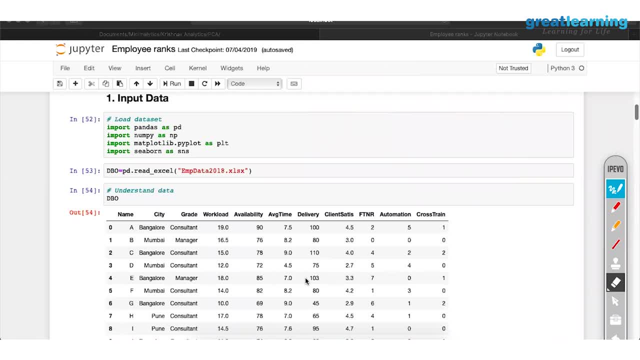 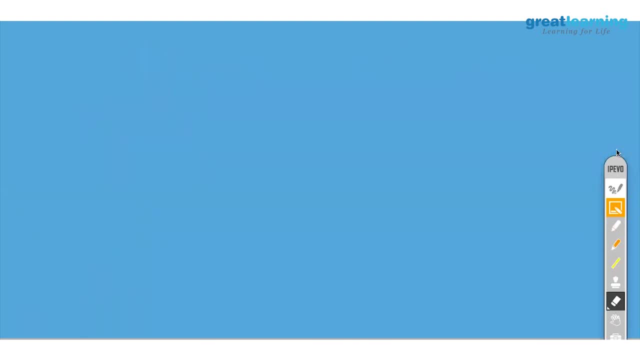 For for transformation leader. Yeah, see, I'll give you a very simple example of my org. Okay, see, what are we currently doing? this? So I am currently heading the transformation teams. Yeah, so I'm not of that level, So I have around eight years of experience as of now. 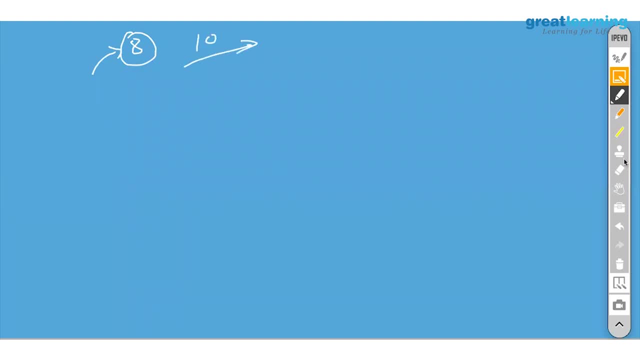 So you guys are more than 10, I can say. So coding is, I will say, we way out of your box to be very fun. So what you guys can do is we pick up a problem. So in my org currently, let us say, there is a problem. 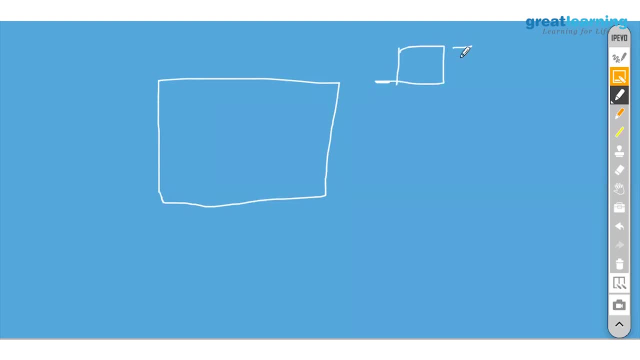 The problem is we are using one tool a lot. name it again. We are using a tool that is pretty expensive- for me, Yeah, and we are catering this tool to some of our internal clients, or, let us say, external clients. Now, those clients are also finding it difficult. 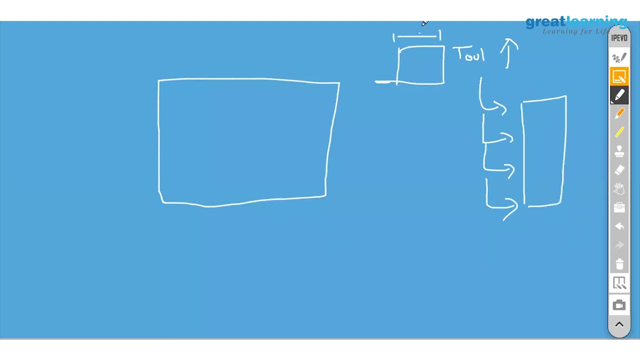 Why this is a end-to-end tool. on to DevOps, for example, it paid to. now What is my problem is not my, not all the features, because this tool has n number of features and capacity, but we are not using it to the fullest. but we are paying for the license for the fullest. to be very frank, 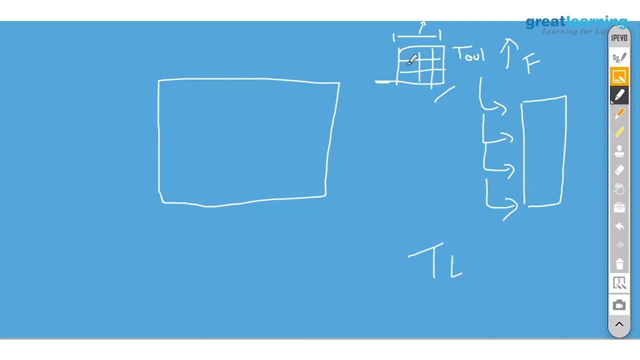 So what are we doing is as a transformation leader. What do you guys have to do? is you to find slow-hanging fruits like this first of all? Yeah, so I found out that, yes, this is a problem for me. now what to do with it? 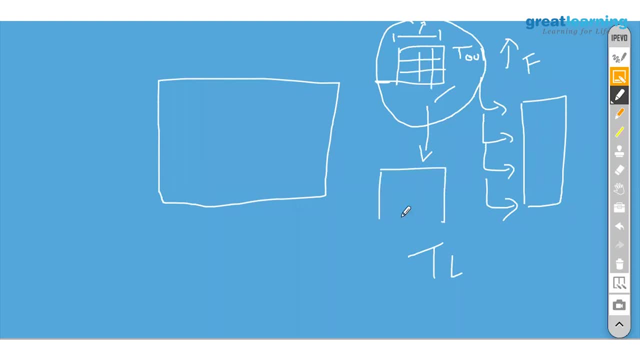 So what I'm doing is What basically this tool does is, when you have a code, know, when you put the code into this tool, what's going to happen is it's going to give you some health factors. health factors Like: how secure is your code? is your code optimized? is your code test friendly? 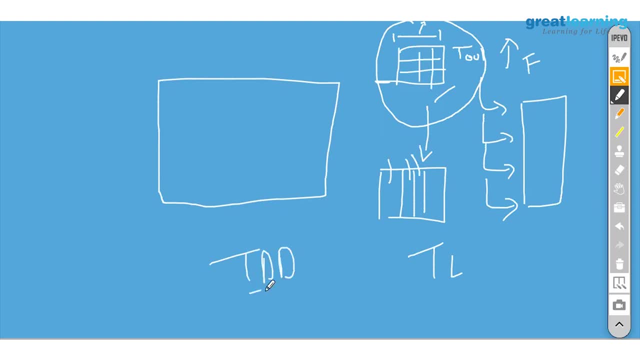 If you, if you heard about a methodology called TDD, test-driven development- Yeah, next is your code. What do you say? So, TDD, we have done. Yeah, is your code optimized? Do we have any Doops into that? is your code technology friendly? 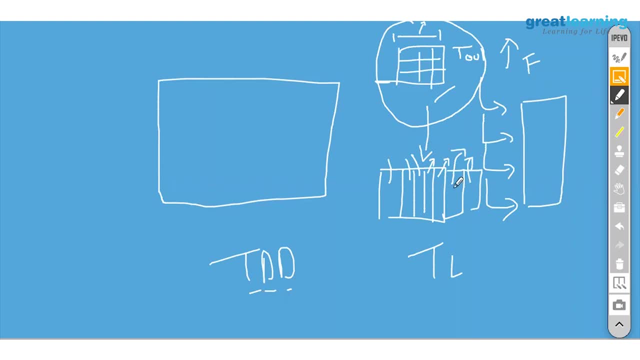 Is it transformation friendly tomorrow when we make some changes? how it is linked? basically, you know. so we have this tool, does it, but beyond this, this tool does a lot of other things also. now what is happening is some of our clients are focusing on your security. just check security for me. just 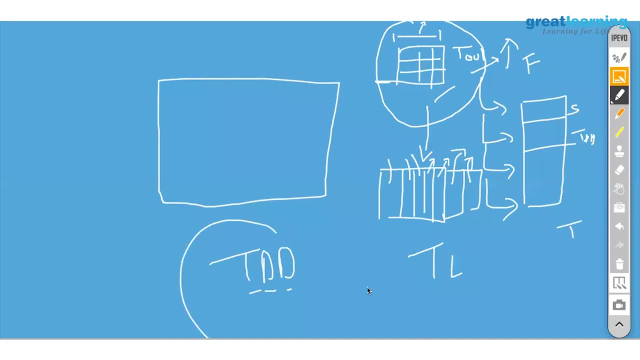 check TDD for me, because they have a dedicated testing team. Let us say, and if the developer, the code, is not test-driven, that means the testing team has to rescript and lot of automation thing happens on the other end. So what I did was I picked this up. 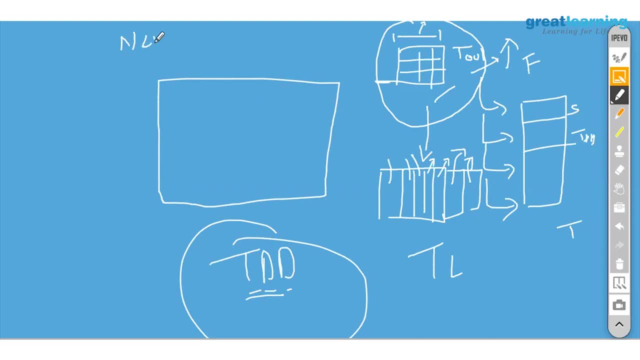 I made one simple NLP where we were able to find, we were able to learn, what is an optimized code, What is the secured code, What is the best practices of coding. We did all this learnings first, So it took some time to gather the data. 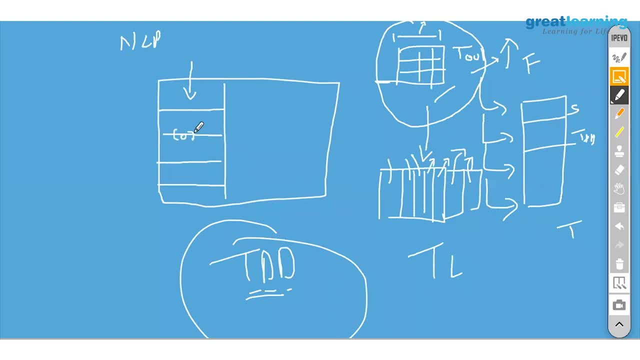 But once we had it we put it as a corpus. corpus is nothing but a reference file. Then we got the new code, the latest code that we want to compare, and then, using NLP, We try to Find out bits and pieces here. So let us say if, if an org or if a client wants me just to do security analysis, 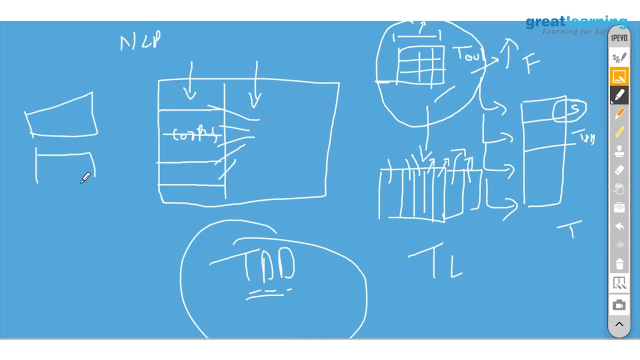 What I will do is using NLP and try to find out places where there are penetrations going on, penetration in the sense where there is a data penetrating in the code or where the data is going out of the code. We'll try to find out those pinpoints and then we'll try to assess, using this corpus saying that. 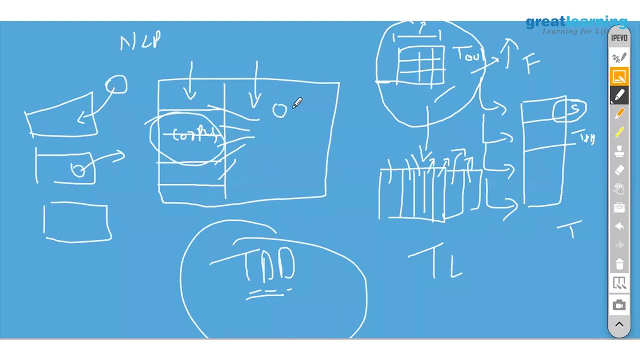 whether this is a secured way or an unsecured way. on it completely, I will not say open source, but a freeware. So the license Costs which we used to pay. what we did immediately was we reduce our licenses by 50 plus, for example. 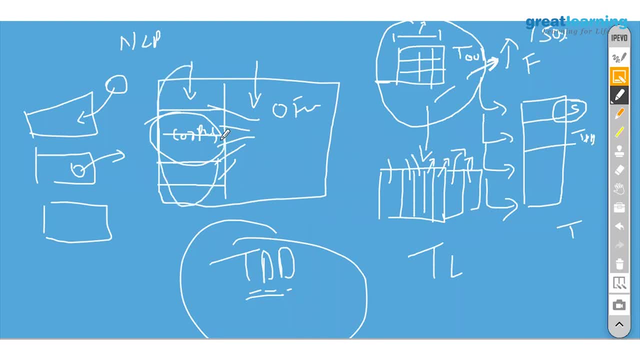 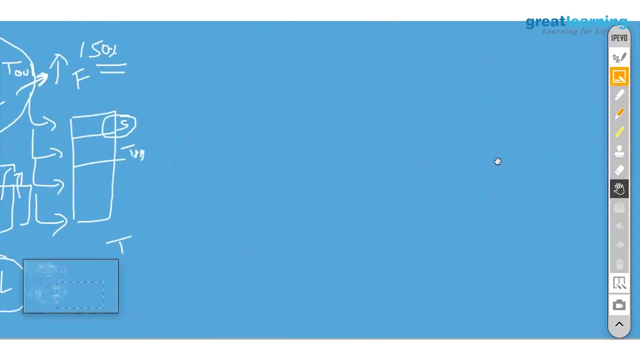 So what happened was they spent some money on my development here, but the ROI was pretty quick by reducing this. Okay, guys, this is how what I call it is a transformation. Now, if some of you are from marketing point of, or more from the marketing side, 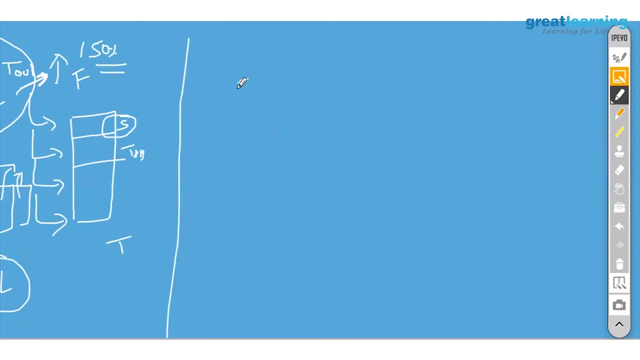 what you guys can do is you can run a very simple customer sentiment analytics model Where you will be getting some comments from the customer daily in an email or in a feedback, or the customer is writing about your organization on web. You can pull all this data together and, let us say, the customers BMW, for example. 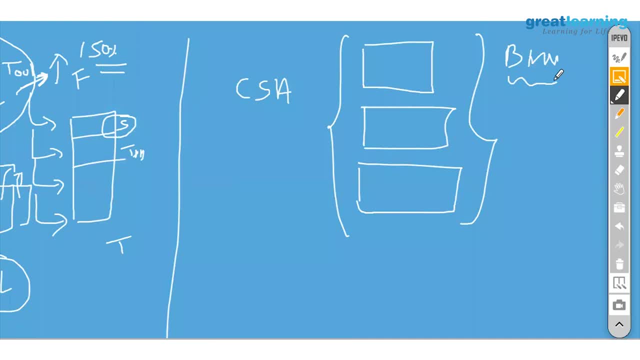 or if you are looking for BMW, what BMW is doing in market. you can pull all this data together and you can do a customer sentiment analytics. They didn't even this. analytics will tell you whether the customer is talking positive or negative about you are the feedbacks. 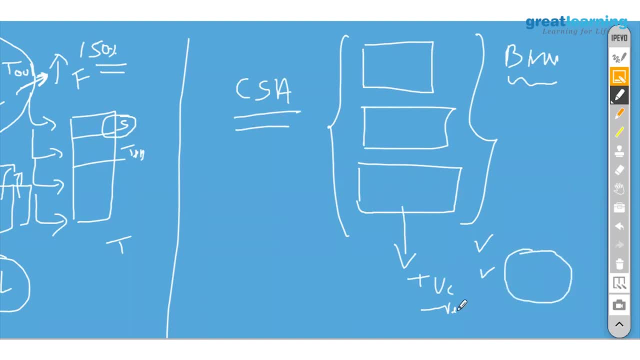 Okay, not okay. If it is not okay, what is he pinpointing at? let us say, some of the emails are pinpointing at delivery time, delivery time, delivery time. What does it mean is it's a hit on that? the customer is not happy with us on delivery time. 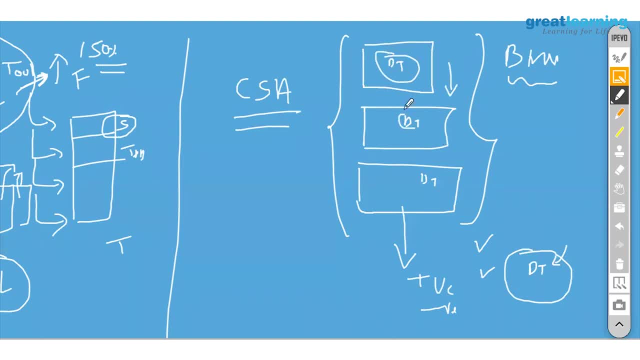 and I'm not saying on small data, because on small data anyone can pinpoint this. I am talking about a place. Let us say there are 1 lakh tickets raised by client on an every feedback on the ticket support ticket. He is talking about this from this. 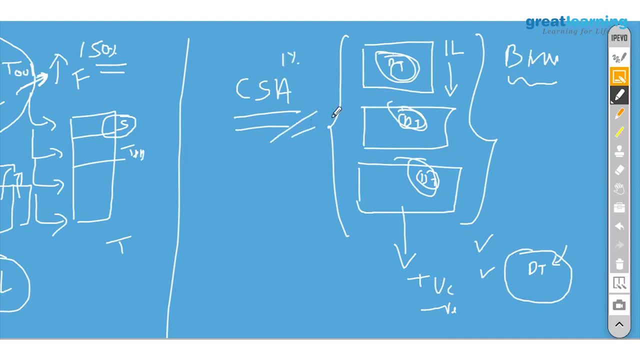 You can pull out all of them, just talking 1% of customers and demand analytics. If you want, I will take a session on this also. I've got some models to show you guys. Okay, So this is what I call a transformation leader. transformation lead will pick this problem up. 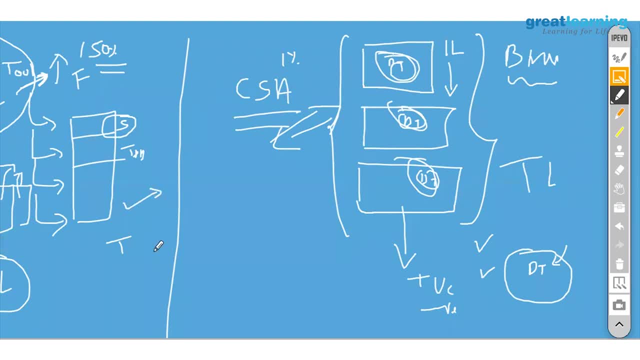 and will solve the problem using some of these techniques. So for that you should know which algorithm to use. you are not supposed to know Python, but for that you are supposed to know where to hit on to this. So you cannot say: do linear regression on to this will make no sense. 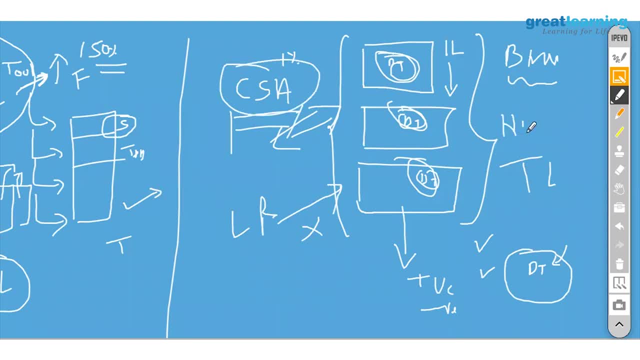 So you are supposed to know, Okay, we are supposed to use NLP here. Okay, fine, in NLP, What all we need? we need AI, Okay, we need CNN. Yes, we need tensorflow- Yes, So you need to know the know high-level view of it, and then you can employ guys who can code for you. 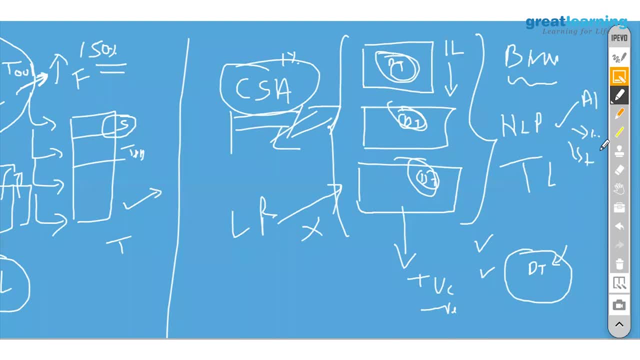 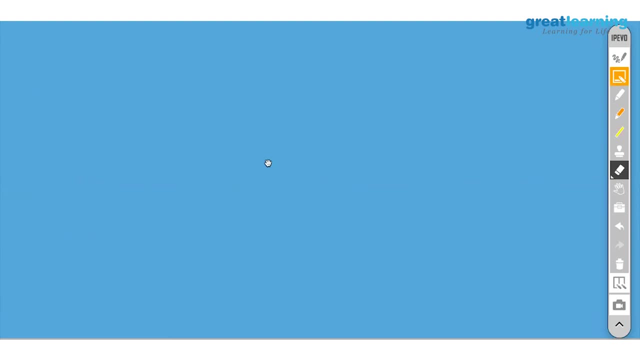 Coding is not a big deal at all. I hope you got my point. Yeah, I have a lot of experience. I'm talking about what I was asking. I can't understand Should how our preparation should be, because now we are in the learning stage. 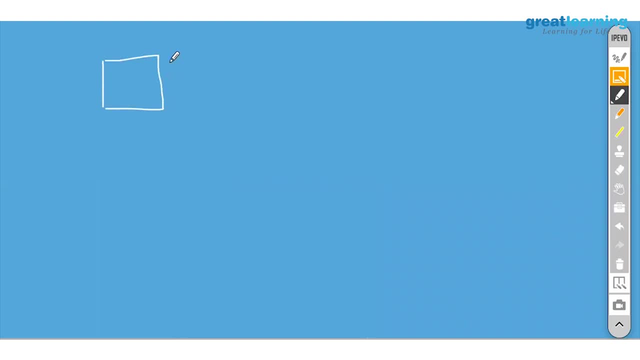 Correct. Now what I would suggest you. first of all, you try to put the puzzle together. Let us say: if you are talking about classification, what classification solves. if you are talking about ensemble techniques, how are the difference between ensemble and classification? Okay, if in case somebody comes to you with a data. 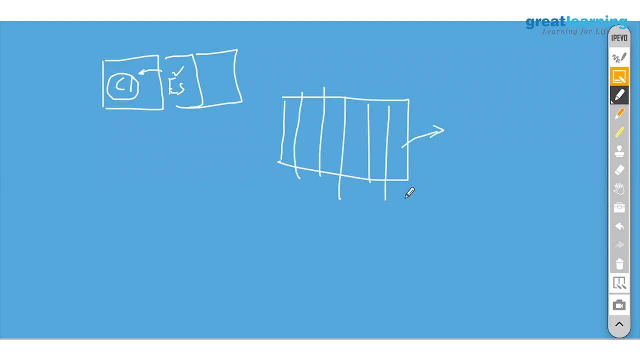 for example. yeah, you should be able to propose Algorithm for that. that okay. as far as data, I think you use decision tree. It should work, but why that? you should be knowing it. Okay, Yeah, so you'll be like directing the team: exactly what to do. 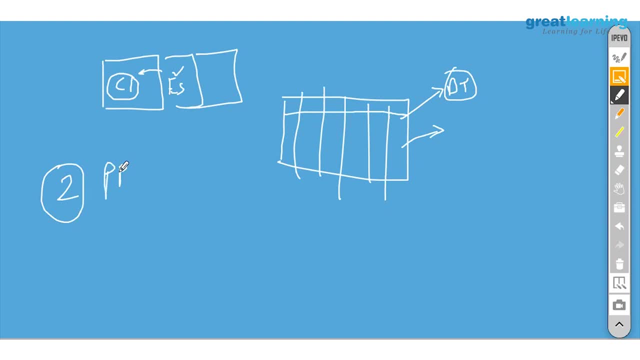 Secondly is: you should be very good in pinpointing problems and giving a solution, with framing a solution. This is the biggest problem. Why? because not every org is ready to accept that. Yes, This is the problems of, I'll tell you for me to convince to reduce the licenses to 50%. 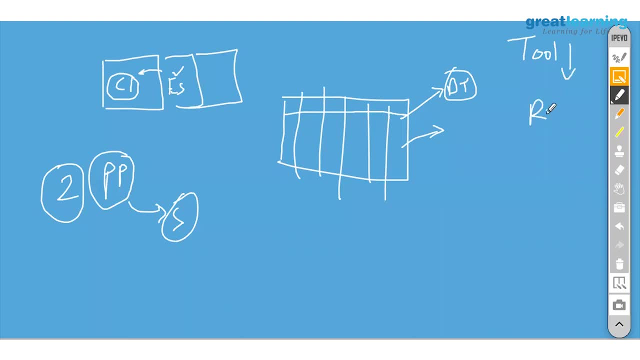 You know, I had to go a lot of pain. They made me predict ROIs on this part of it, where even I did some fake part of it, But, yes, it turned out to be good somehow. Okay, So this is where, so initial kickstart will be very difficult. 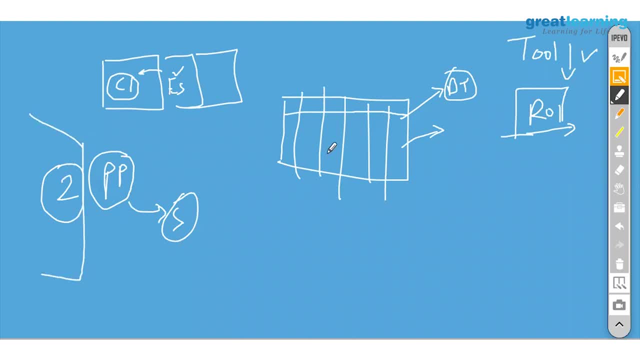 I again I will tell you because not all organizations are ready to accept that something can predict future with a very accurate stuff. The first challenge is finding the problem. second is finding the data, Again, the companies that recently, whatever company service companies that we work for. to be very frank, the data is pathetic. 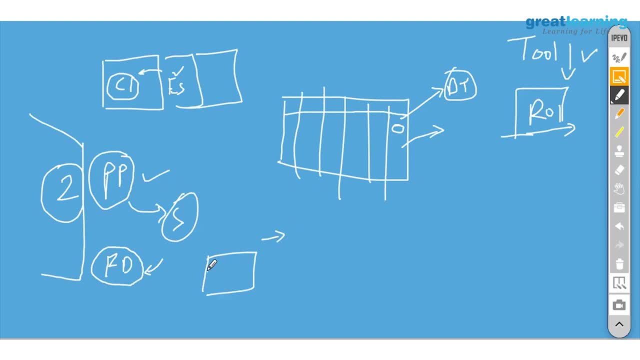 So either you have to kick start and give yourself a time of six months to gather the data, else you have the data. you try to transform the data. whatever is it with you. Okay, Was that? applying these techniques is not a big deal at all, because it's pretty straightforward. 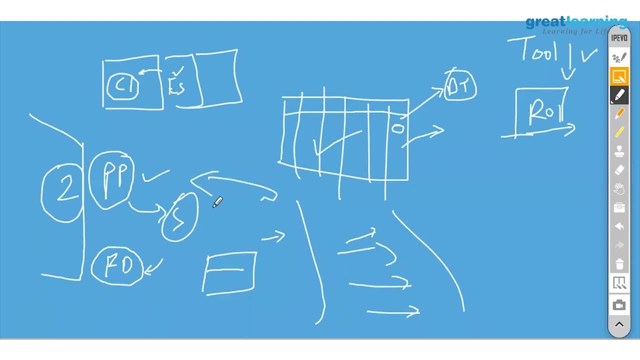 This is the easiest part. the before this, whatever we do, is the difficult part. Yeah, Yeah, Yeah. So this is what I would recommend for all of you. again, I have- I have my own of my colleague is around 41 years of experience. 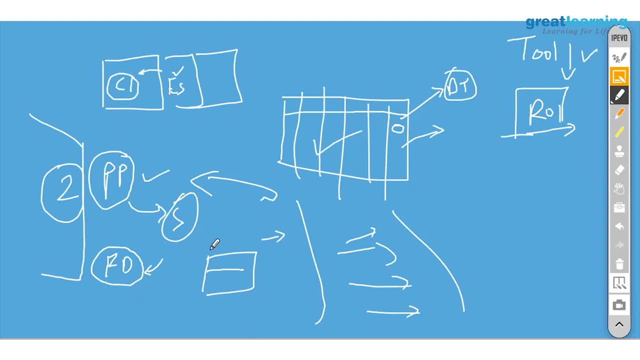 He sits in Netherlands, that fellow is still coding. He, he likes coding, So he's doing it. So again, I will say it on preference. but, as of me, if you want to excel on to this, I will say you need to be something like a transformation leader or a transformation director, like that. 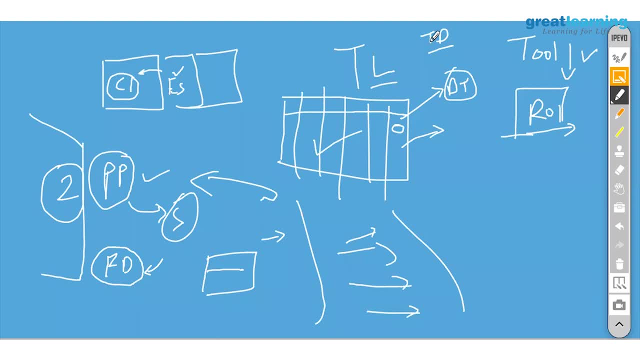 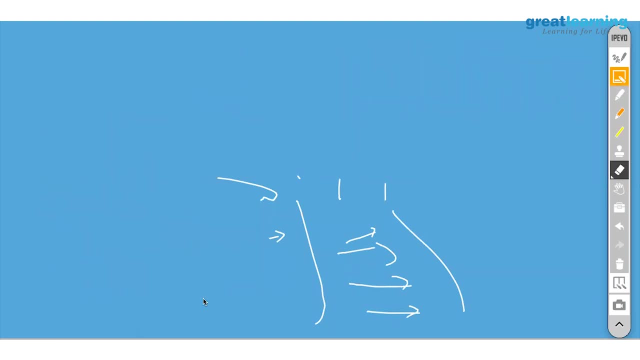 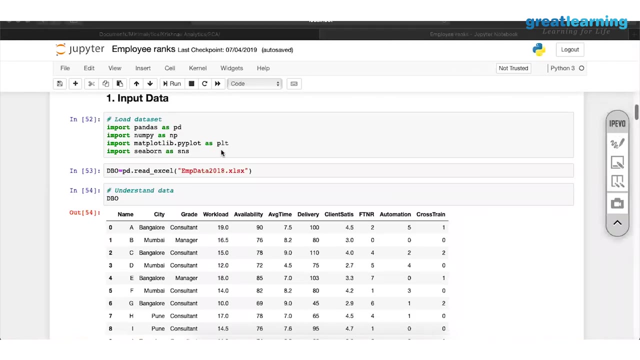 Try to find a problem and automate it and try to find something. Thank you, Perfect, Okay, so I think we are good. Let's close down then. Yeah, I will share all the files with you. Okay, and try to create that Google dumb that you are talking about. 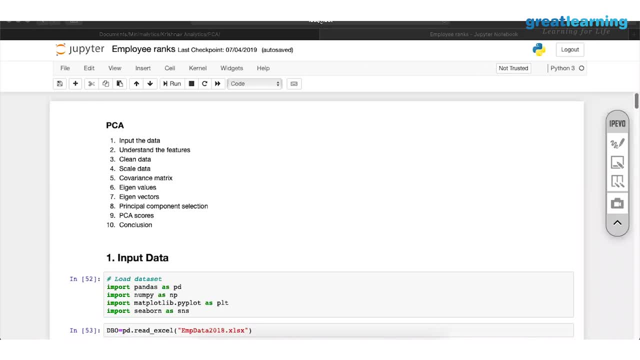 We'll try to put all the files over there. I'll do that. Yeah, perfect guys. Thanks a lot If, in case, you have got any feedback. if I'm fast, slow, Too much detail oriented or too much code oriented, whatever it is. 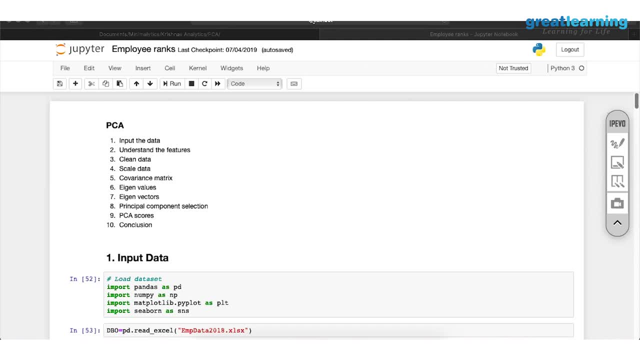 do let me know on face itself so that I can improvise immediately, because it's like very small improvisation But yet if I try to do it, no, it will be like I want your sessions to be smooth Basically. I don't want you guys to be wondering after the session. 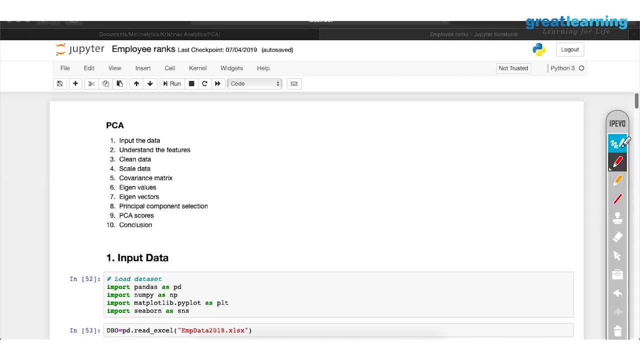 Okay where we went, and the most important part, which I feel is to which I focus on, is to put this puzzle together. This is this is what is important. So if, for example, if you talked about PCA, what is this PCA? What is the puzzle about? 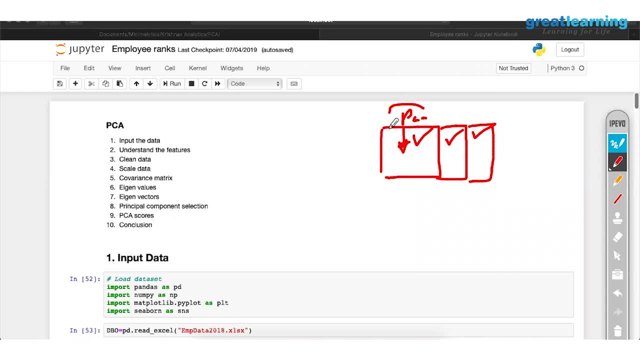 Why it is needed. This is what I focus more on. if, in case, you are not okay with it, Do let me know. I'll try to improvise, Okay. Okay, Perfect days after what. you're using IPEVO So we can get this with. this will be very useful when we are teaching something- this, this, this one. I got it from my 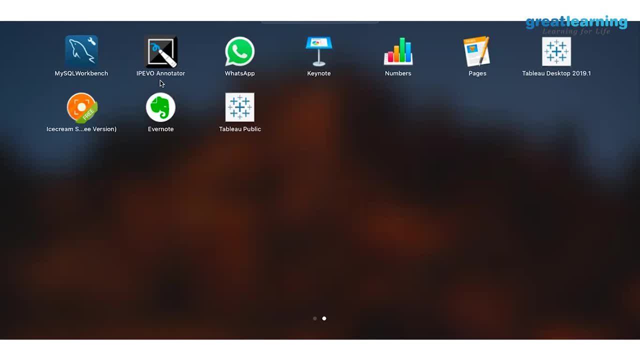 Mac store. It's free of charge software. Oh, okay, IPEVO annotator. annotator: Right. Okay, It's me, Of course, and it is no having more upgrade. an add-on. society is good. Okay, Thank you. 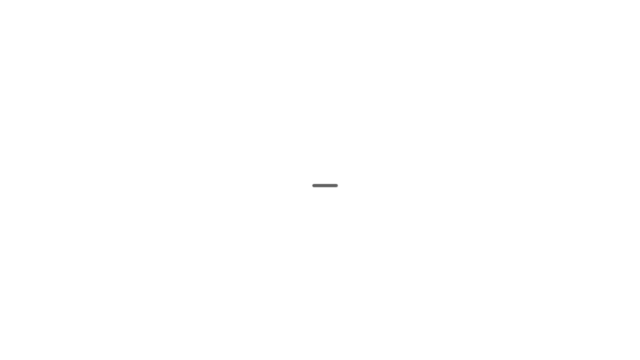 All right, Okay, Thank you For today's session. What we are going to do is we'll start off With unsupervised load of this thing. Sorry, there are clear clustering, which we have not done so far. It's very simple. 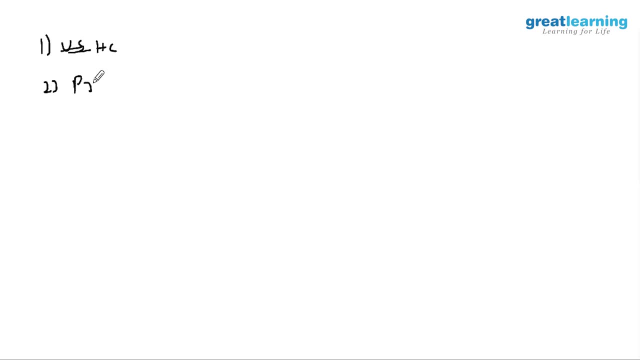 Again. Secondly, we'll discuss the project. So we'll discuss this in detail: What exactly you are supposed to do, What is expected out of the project, step-by-step Okay Post that I have got to show you. So we'll start with something onto your next module. 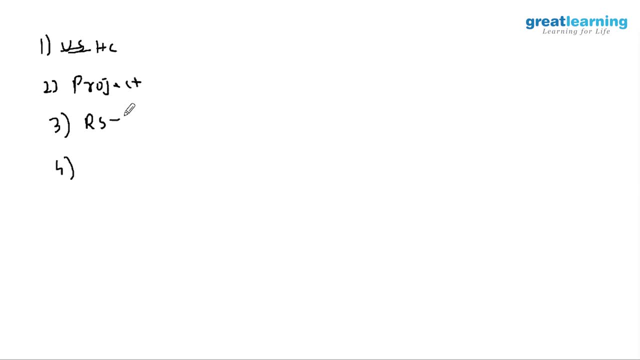 Will not start the videos and all this part of it. I'll give you implementation On what is recommendation system and what we are supposed to do So that your next or whatever upcoming videos will be easy. Okay, This is a little sorry. 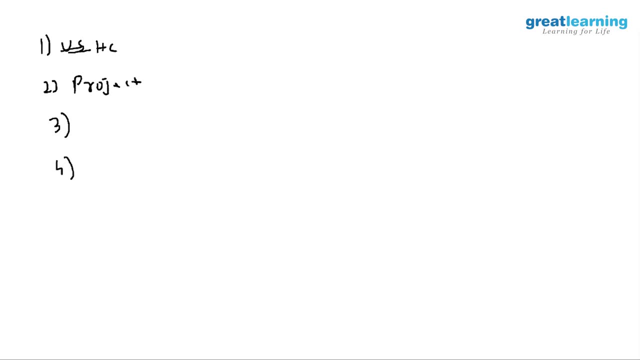 Sorry, Sorry, Sorry. Why is learning right? So your next thing will be feature engineer, Yeah, Or will be feature engineering? Is it released any, any, any idea on this? No, right, No, no, not yet, Not yet. 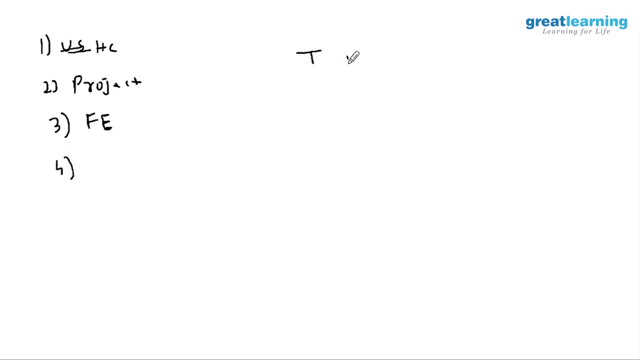 Okay, And have I discussed anything about testing on machine Learning or cross validation on machine learning? I think we have not discussed on this, right? No, no, right. So I'll show you what exactly we mean by what we mean by this. 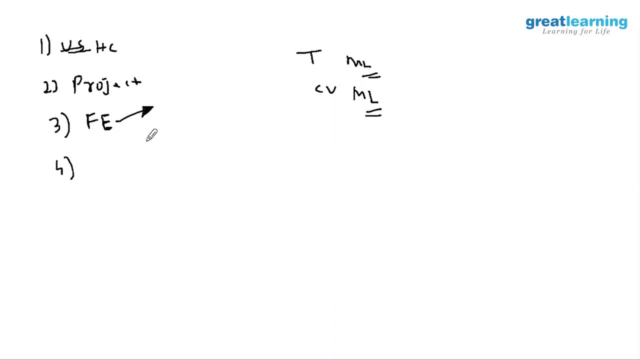 And I'll also show you some some implementation onto that so that you get the idea of it. Okay, post that. if you remember, we built, we had built up a simple chat bot, So today I will start up with a very simple AI based chat bot. 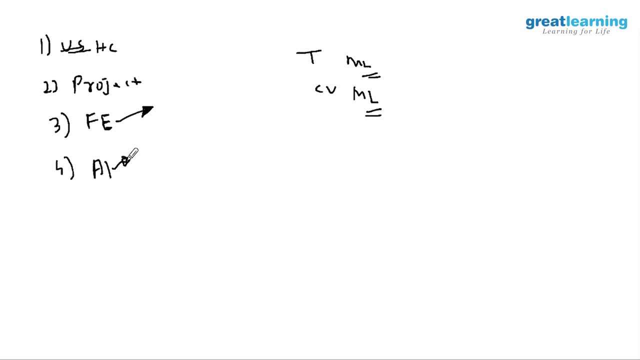 So we'll, we'll have a foundation of what is AI first, Yeah, and then I'll show you how we can, How we can do that, Yeah. so I think we'll spend around 20 minutes on this, say, around 20 or 30 minutes on this, 30 minutes on this and probably 30 minutes on this. 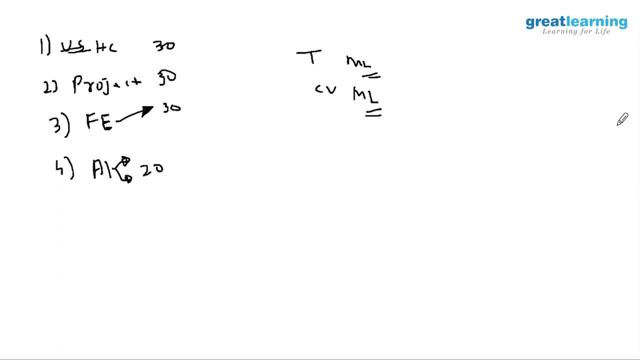 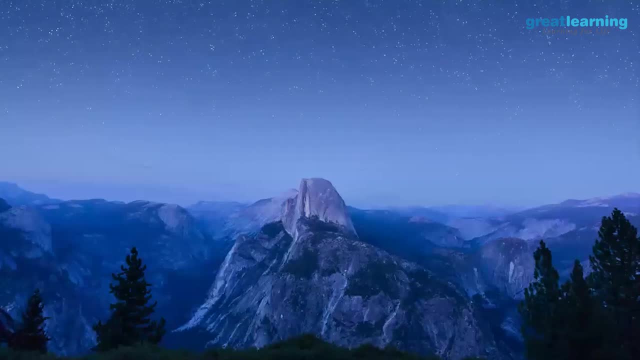 Yeah, Okay. so everybody's okay with PCA and all other things, right? No, no, no, it's onto that. Perfect Good, Okay. So, starting with hierarchical clustering, again, it is very simple and again I would say it's a old-school. 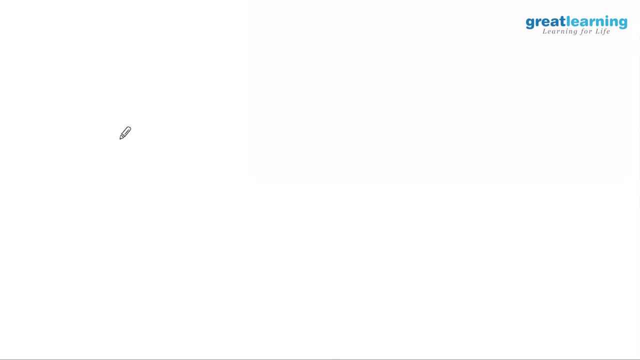 Algorithm that we. it's not that popular nowadays, But yes, it's good to know. Sometimes some of the applications you know we can solve it in a very simplistic way. So let us see it using this graph first, and then I've got some visual things to move on. 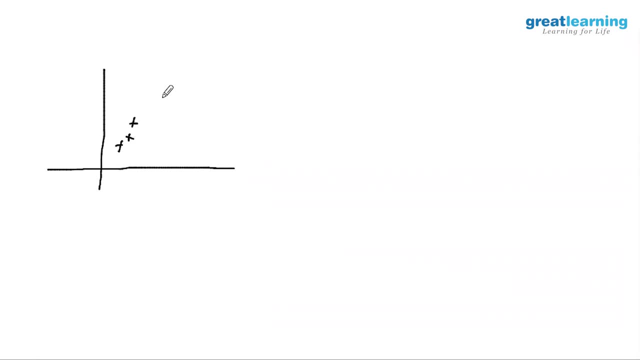 So let us say: you have got some points, Okay. let us say there are some points like this, Okay, like this, For example. let us say: you have got some points like this And if in case, we don't want to go ahead with our normal clustering technique, let us say: you want to move on with hierarchical 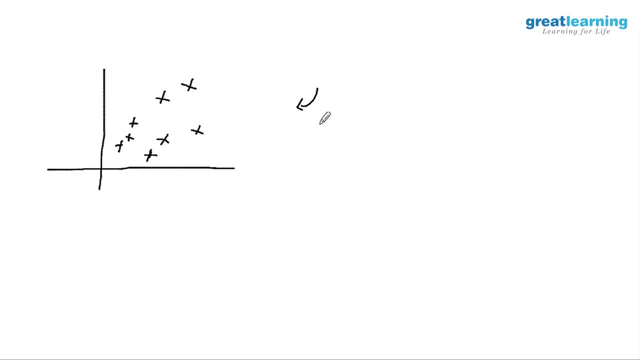 Now how do we decide whether to use hierarchical or whether to use clustering? again, depends on our application. in the weight, I will say: normal clustering is little heavyweight. hierarchical clustering is little bit easier as compared to the normal plus. Now what do we do here is the concept remains same. Euclidean distance and Manhattan distance comes into picture first. 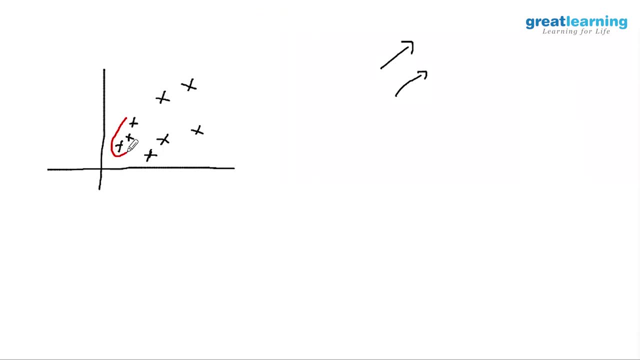 We'll try to find out The nearest clusters. So let us say this is one cluster which I will call nearest. This is another cluster which I will say it's near. This is the third cluster which I will say it's nearer and is the fourth cluster that I will say it is single dates, not near to anything. 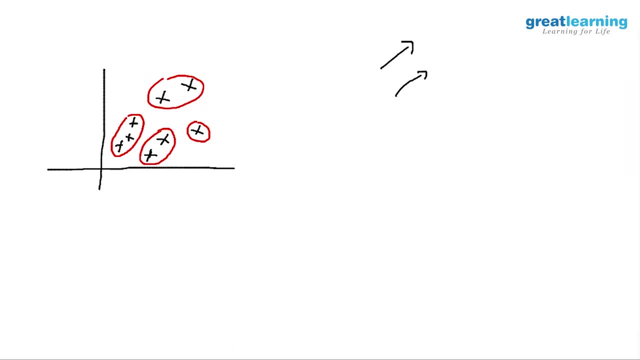 Now, once we've built a what is the clusters, then we can say: let's try to find out nearest clusters together. So in that case I will say the nearest clusters, Let us say, are these two. So I will name them as: 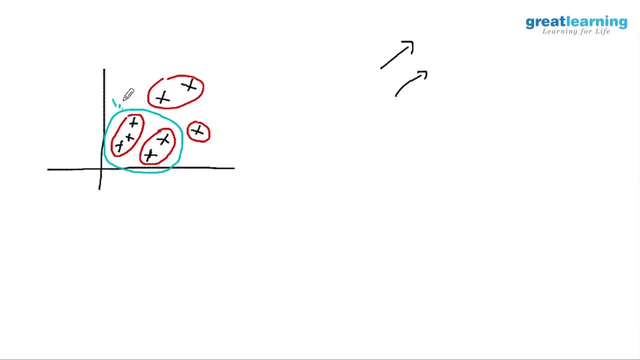 So this is cluster number one, cluster number two. So this will be combination of cluster one and two. Now, once I do that, I can say that this cluster is nearby to my cluster. So I will say this: I will build us as a one cluster. 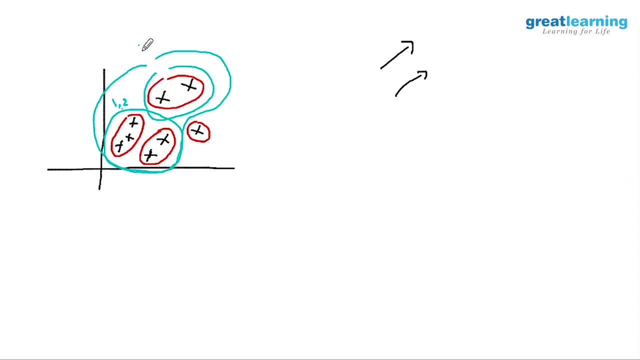 So this is a combination of cluster number one, cluster number two, cluster number three. Okay, and if you see this, this is little far away. So if you want to include it in the final step, We can say that this is a whole cluster. 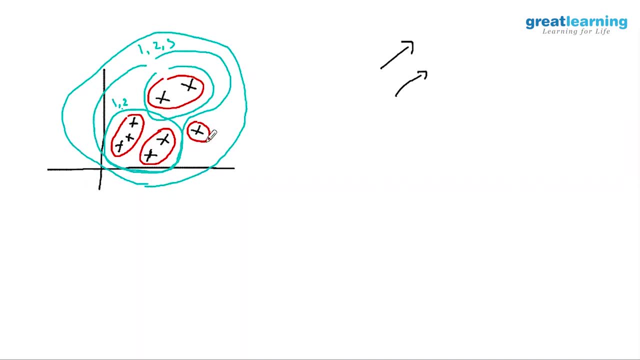 So this is a combination of cluster number one, two, three and four. So if you look at it actually, you can easily make out that there are three different clusters, Cluster number one and two. combined is one cluster, cluster number one. So this I will name it. 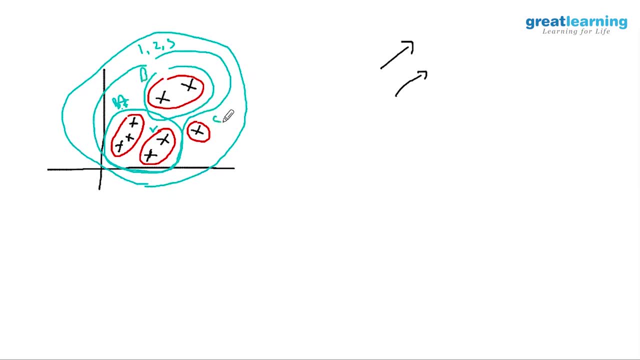 So let us say this: cluster, number a, number B and cluster. So this is how we can build up the clusters. Now, if you want to see in a visual way, it's very simple. Let us say: this is one, two, Three, four and five. 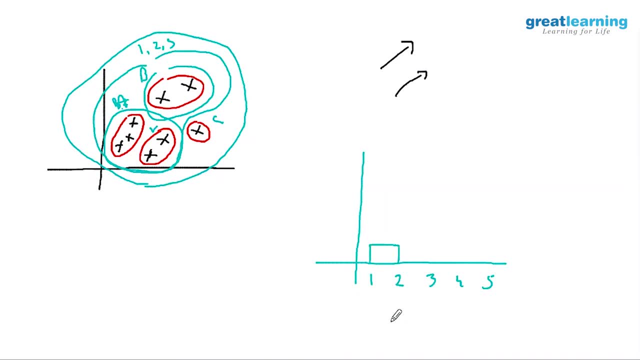 For example, you can say these two form one cluster with some distance between them. Let us say this is distance and this is number of clusters. I will say three and four is a cluster where they have good, good amount of difference between them. That's why they are little higher. and fifth one: 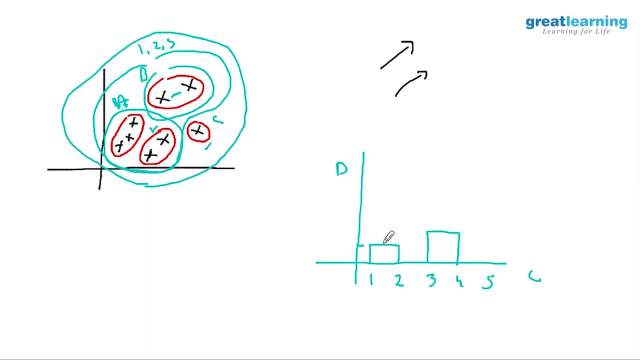 I will say it's nothing, because it is a single one. Now have will find out the distance between these two clusters, which I will name it like this, and I will call it as one cluster, Okay, and then I will combine it with the larger cluster. 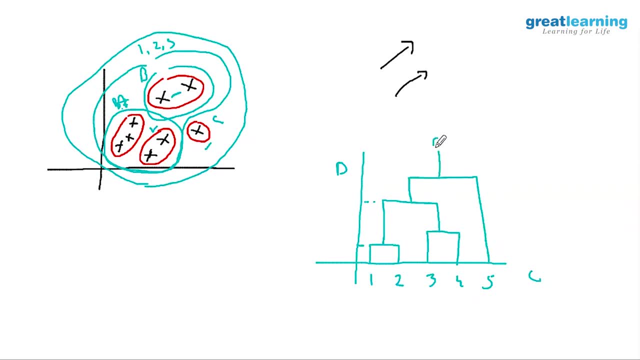 The fifth one, and then I will make the whole data set can be one cluster, which can be broken down into multiple clusters. Yeah, Now how do we know how many clusters to select here? So how do we find out? So, in that case, what we can do is try to extend all the lines that we have. 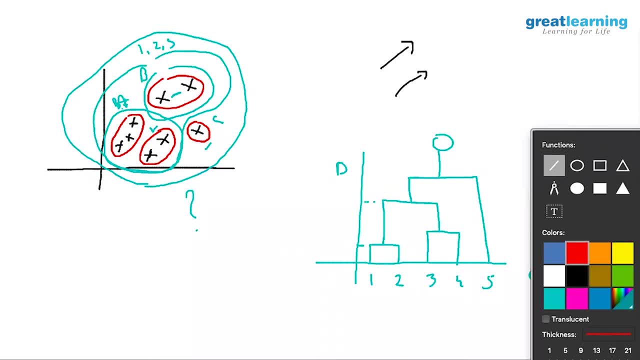 So let me make a line: Try to extend all the lines, Both the sides. So this is one extension, This is another extension, This is the third extension. Yeah, so we'll try to find out one particular place where none of these lines intersect or where none of these lines cut the horizontal axis. 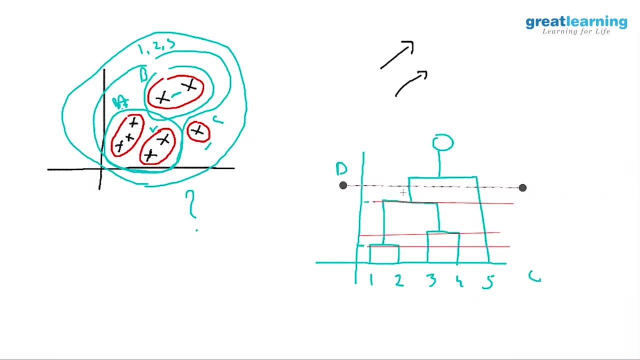 So in that case, I will say: this is the place. This is the place, I will say, where none of these vertical lines cut this particular line. So I will try to Push my line from here. and wherever this line intersects, it intersects at two points: one point and two points. 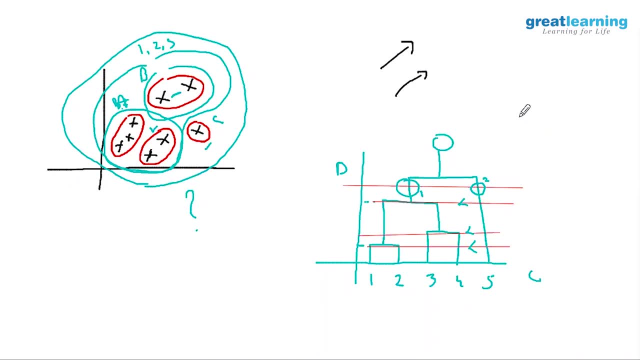 So I can say, for this particular cluster, optimal number of clusters are supposed to be two. That means a combination of one, two, three, four will be one cluster and five will be cluster number two. Simple Yes, simple right. 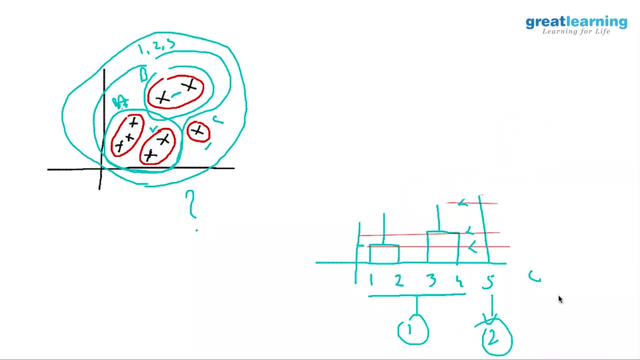 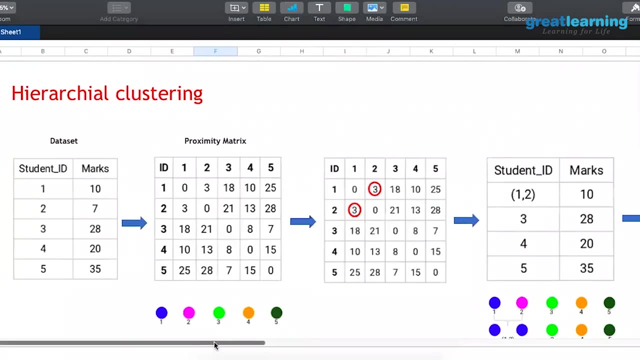 Yeah, perfect, As simple as that. So it's very basic and very primitive also. So, keeping this in mind, I've got a very good visual representations where we have taken some distances, So it will give you some feel of how exactly distances are calculated. 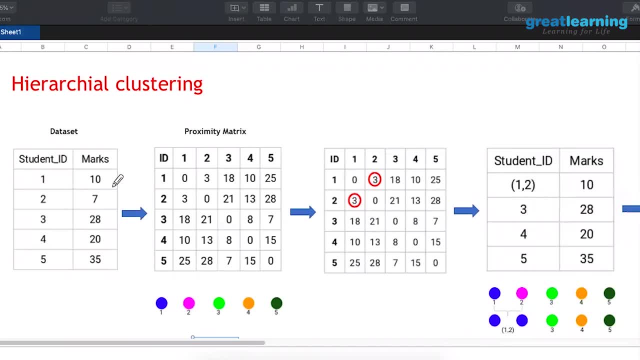 So if you observe this particular thing where we have got five observations, okay, And next, what I do is I'll build a proximity matrix. Proximity matrix is nothing but your covariance matrix. How this is dependent on this, basically, So if you subtract 10 minus 10, you are going to get zero. 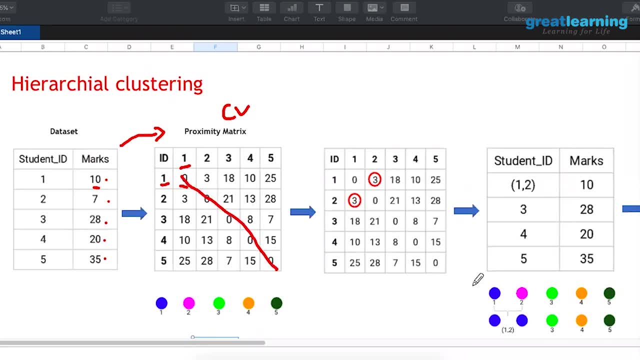 That means it's the same point. So all the diagonal elements definitely will be your zeros, So ignore them. So if I want to calculate distance between one and two, that is one and two, the distance is three. That's what I've measured here. 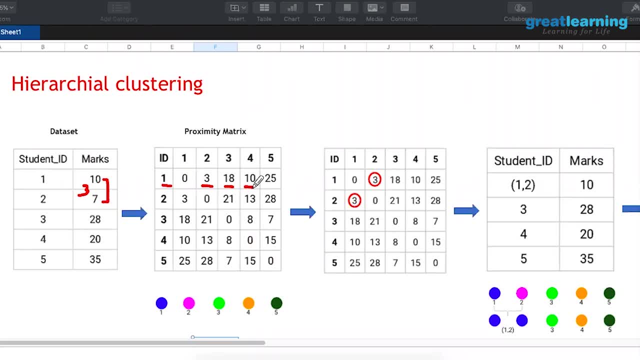 One in 318,, one in 410, one in 525.. Like that I have made the whole proximity matrix Very simple. Now try to find out the shortest distance. here The whole proximity matrix will try to push the shortest distance. 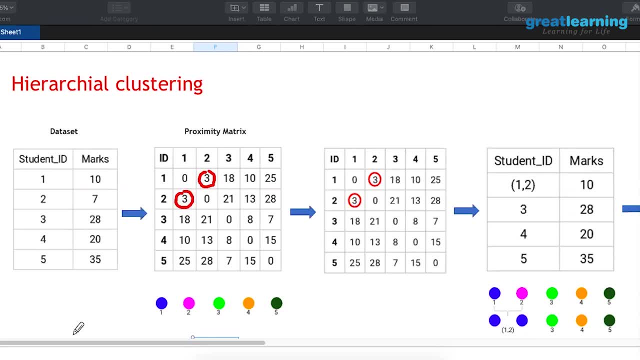 That is. can I say three and three is the shortest distance. Agreed, What is three and three mean One and two. So basically I will say they are at the shortest distance. So now I will club one and two together and my reading will become one comma two. 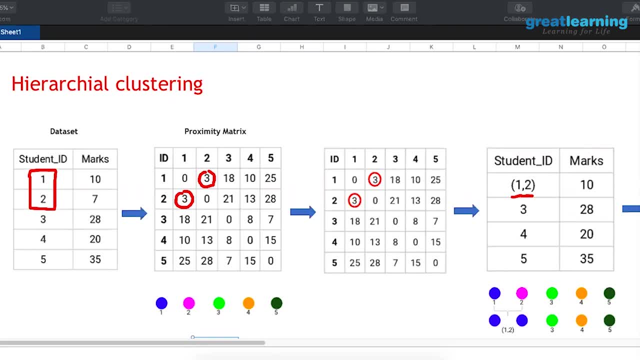 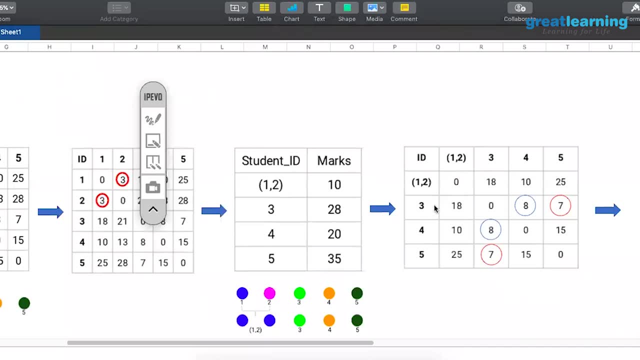 Very simple. Yeah, Next, again, keeping this in mind, build a proximity matrix. So now we'll keep this particular table In mind and build a proximity matrix again. So if you, if you see here, the new proximity matrix will again have some distances. 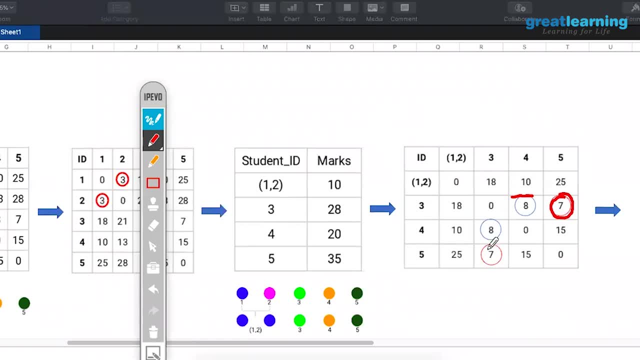 So, apart from that, we'll find out the shortest distance. If you see, here seven is the shortest one, So it belongs to three and five. So now what I will do is I'll put three comma five as my new cluster, And if you see, three and four is also there where eight is there, but still eight is more than seven. 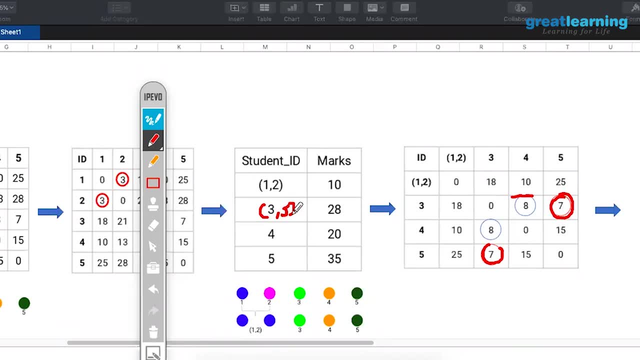 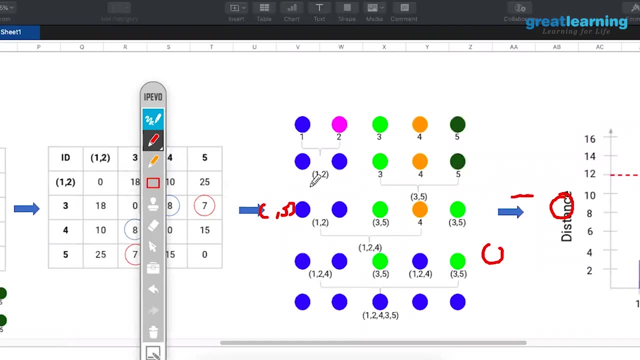 So I will say three is more nearer to five than eight. So my new cluster is three and five. So like that, When I keep going by the proximity matrices I find out one and two is one cluster. three and five is another cluster. four is left out. 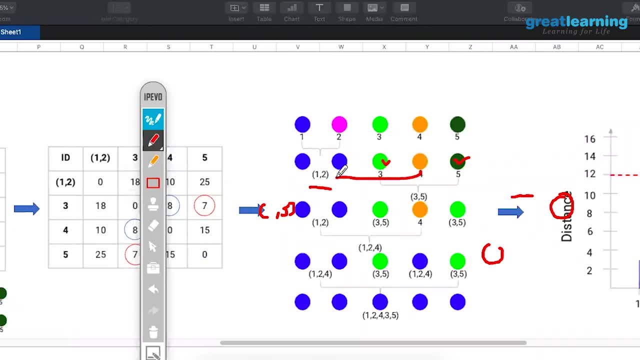 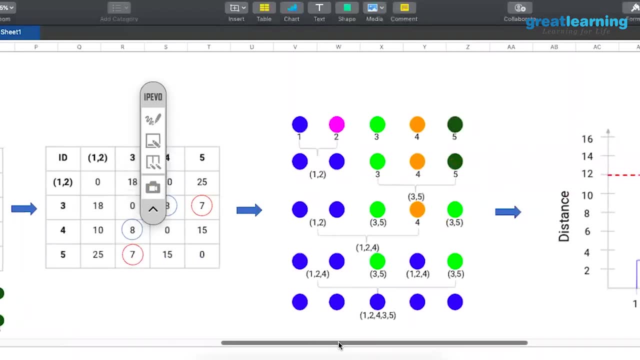 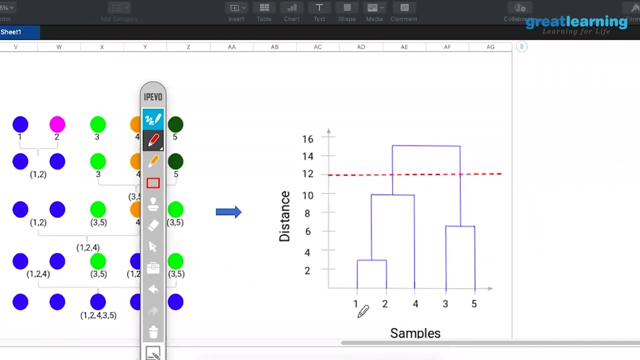 So what will happen? automatically, four will get clubbed with your one and two. So now we'll have one, two and four and three and five as my two different clusters. Yeah, And if you look at the dendrogram that we are going to have is initially we started with one and two. 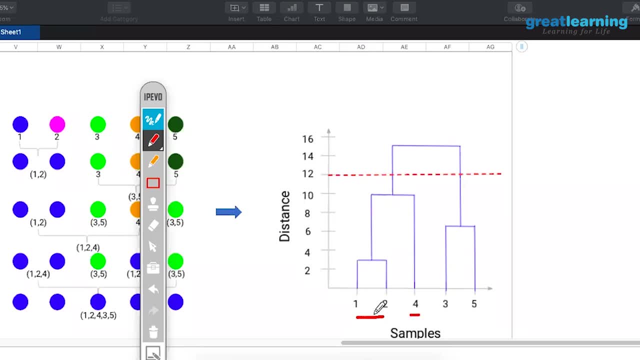 Okay, then four. So now we can say that one, two and four, over here They converge to become one cluster. three and five, the converse here to become one more cluster. Now, if you extend the lines, to extend the lines, if you extend the lines, this is the only place where none of these lines cut. 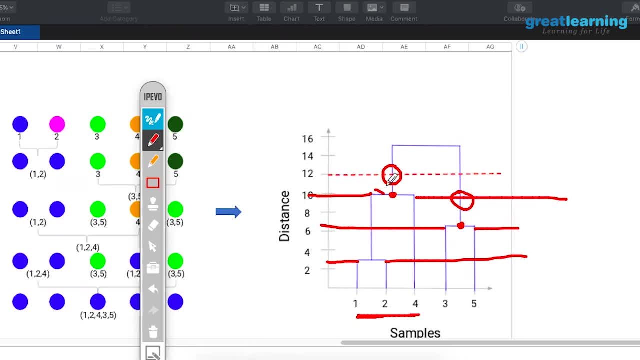 So if you see this particular line, the line is cutting here, but this is the only highest vertical line or longest vertical line. when there is no cut. in that case I will draw my- you know- threshold over here. So it cuts through Two clusters. 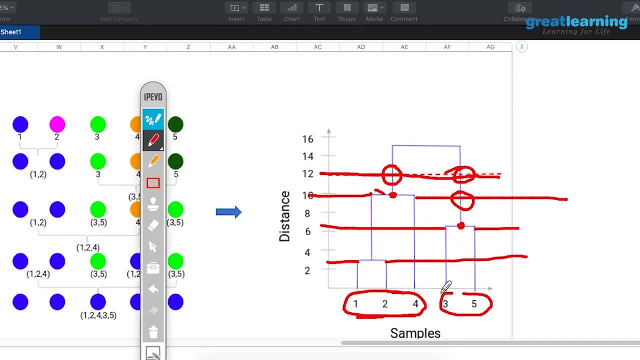 So, definitely, we have two clusters: one, two, four, three and five. Okay, So, if you remember, in our k-means clustering used to use that elbow method basically, and we used to go one step above, one step below to find out the optimal value of K, how many clusters we want in this case. 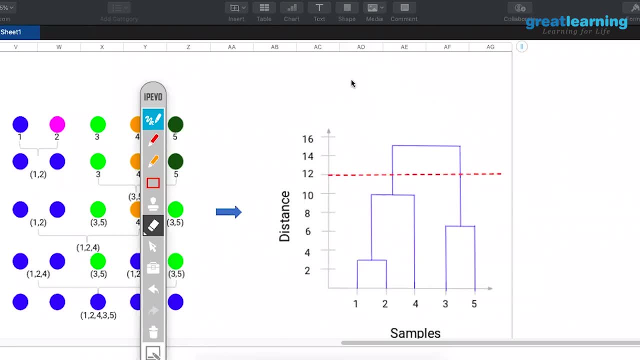 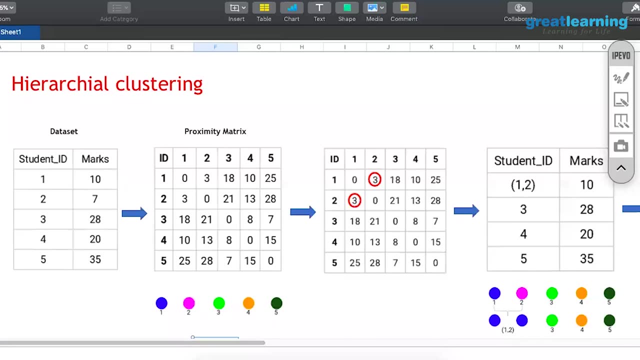 we can find it using this dendrogram line. as simple as that. Okay, So this was your hierarchical clustering. any questions on to this? No, no, Okay, perfect. Now coming to the applications. Okay, Okay, Let's, I think let's wrap up the python code also. 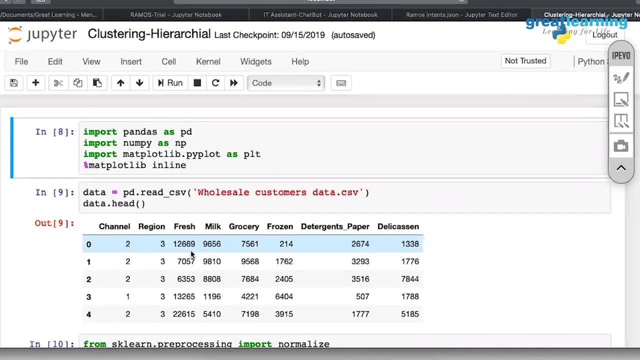 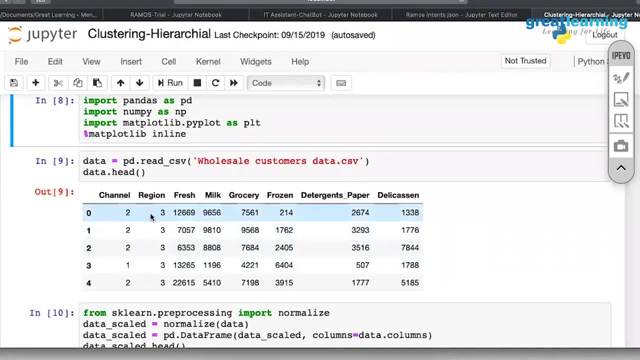 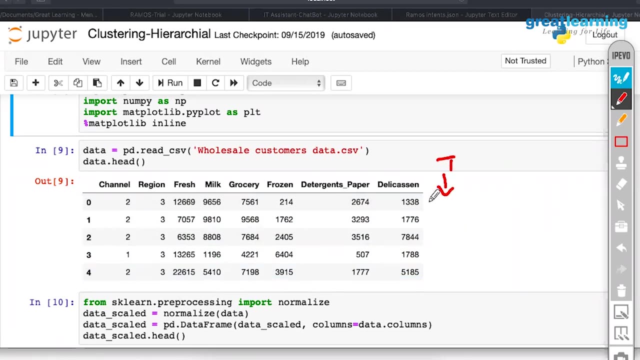 and then we'll talk about unsupervised learning in their applications. Okay, So under a hierarchical clustering, I've got a very simple example where you have got a data set where the target is missing, Definitely. That is why we are doing unsupervised learning. else, 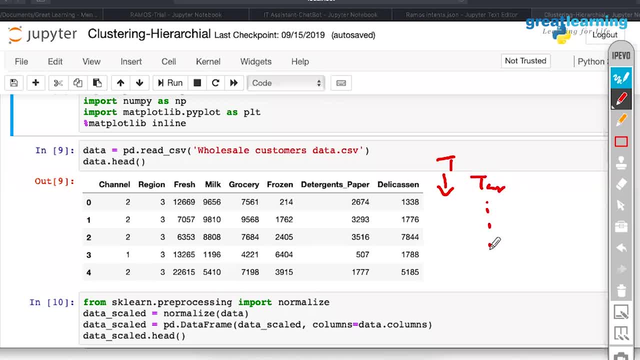 Sometimes, if you feel target is there and if you feel target is not accurate enough, you can ignore this. you can delete the target column and you can regenerate the target, depending on your new cluster, unsupervised learning, hierarchical or clustering method, data. Yeah, So all what we are going to do is we are going to replace it by some clusters here. 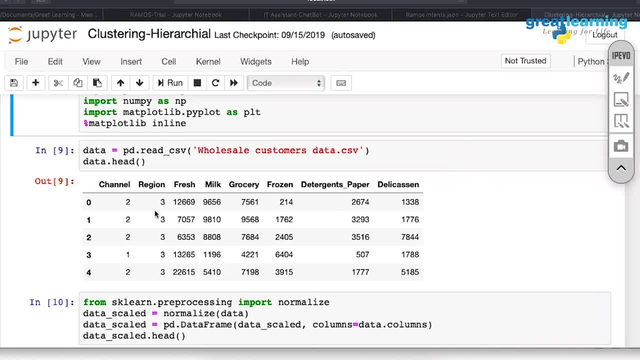 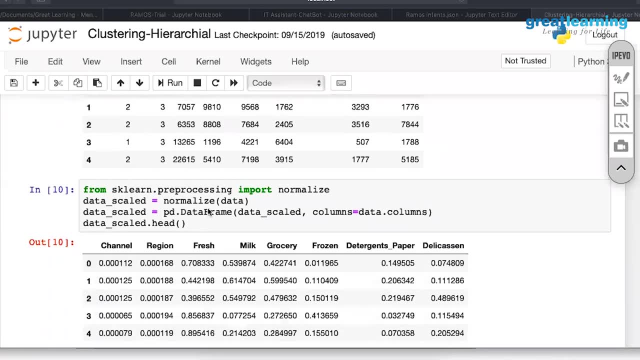 That's some classification value, as simple as that. So these are the total number of columns we have here. Next, What are we doing is the first thing, if you remember, in unsupervised learning that we always talk about is your scaling, or normalization, or regularization. 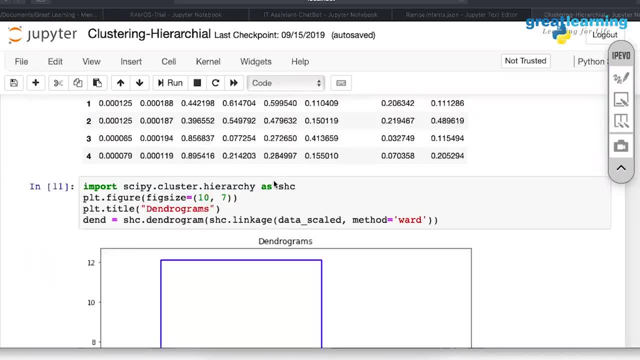 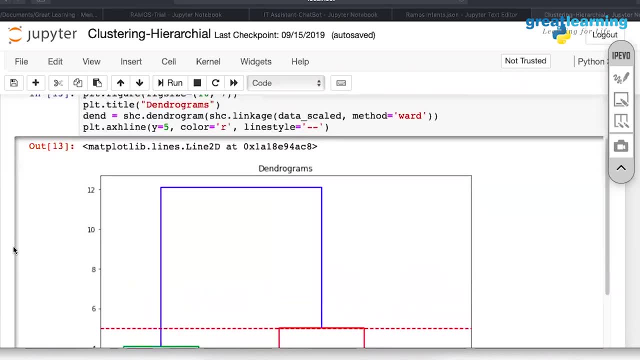 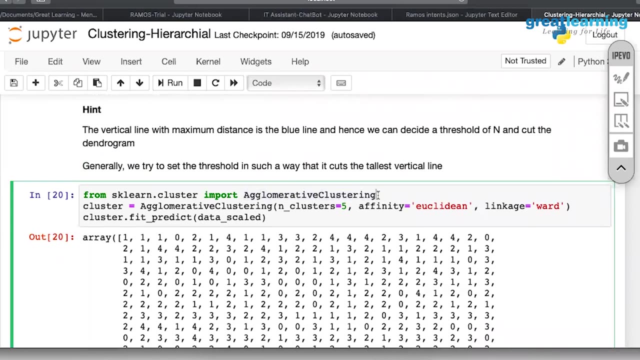 So, first thing, you're supposed to normalize the data set. next, Once you normalize the data set, if in case you want to understand, okay, we'll come to dendrogram later. wait. next, What are we doing is we are going to apply our agglomerative clustering technique, the same hierarchical that we basically so, but I know. 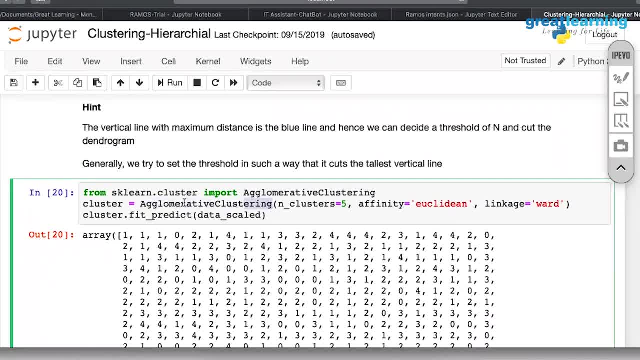 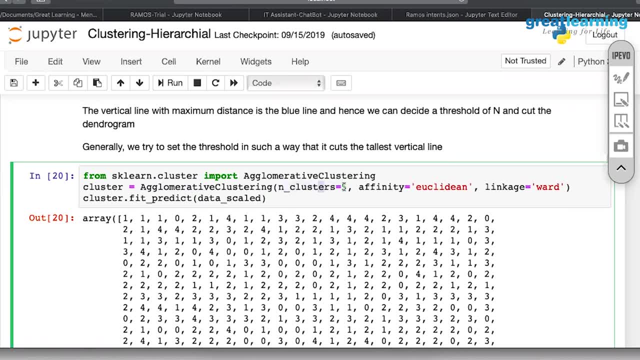 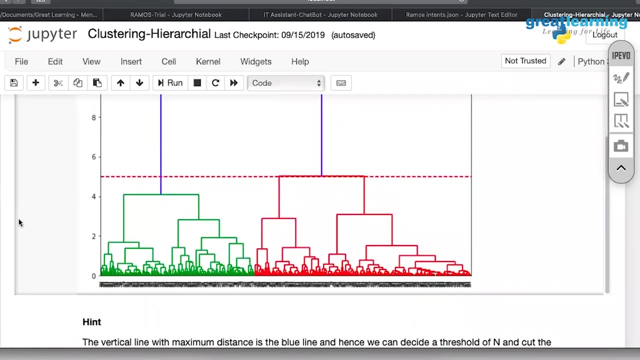 we have agglomerative and we have got hierarchical, but the functioning is almost similar. So here what I've done is I've clearly said I need five clusters. Now, however, I decided I need like five clusters via this dendrogram. If you observe here When I have my dendrogram placed here. 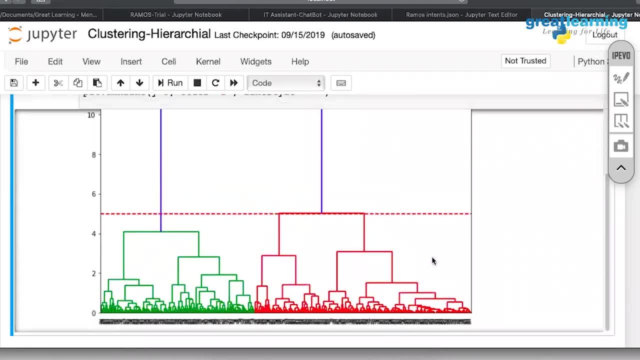 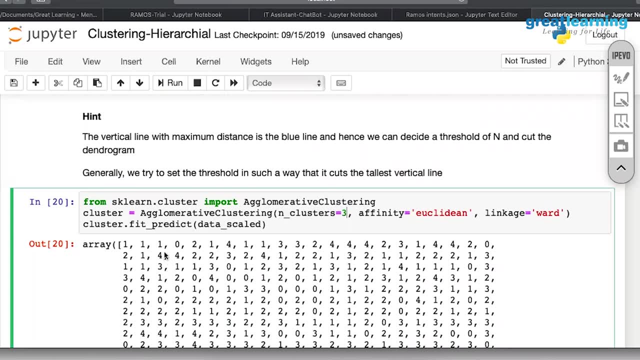 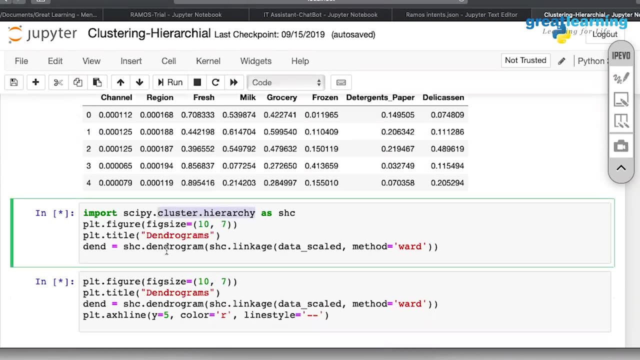 it is one, two, three. We have anything more. Okay, No, I'm my mistake, It should be three here, Sorry, Okay, So let me run it one minute. So, basically, we are do applying hierarchical clustering here and we are getting the dendrogram. 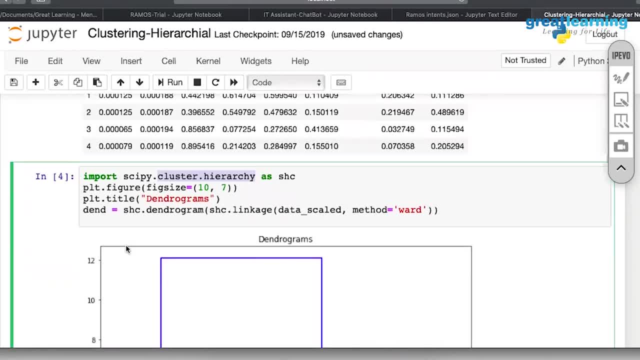 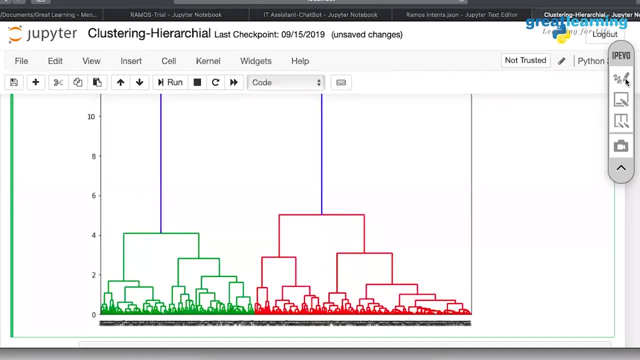 Now it might take some time. I'm just checking if we have done correctly. So this is our dendrogram. next, What are we supposed to do? is we are supposed to find the line using which it will pass. So definitely the line will be from from here itself, right? 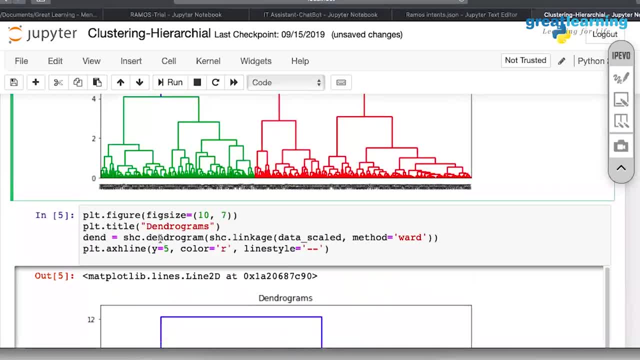 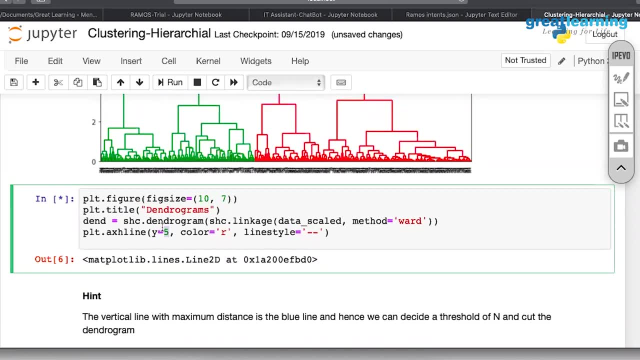 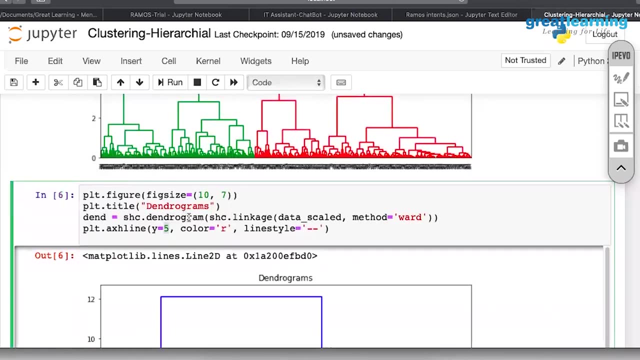 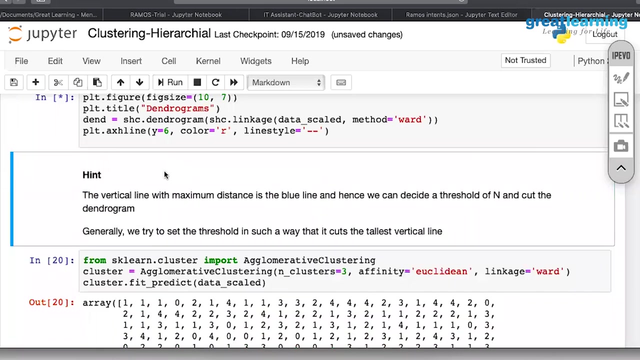 So it should be ideally two clusters, if I'm not wrong. So let's see: Okay, I have written y as five. My mistake. Okay, I have specifically given y is equal to five, but actually y should be equal to six, because we are not supposed to intersect any of these lines. 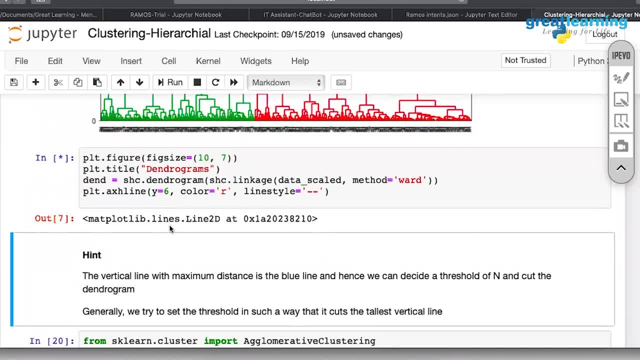 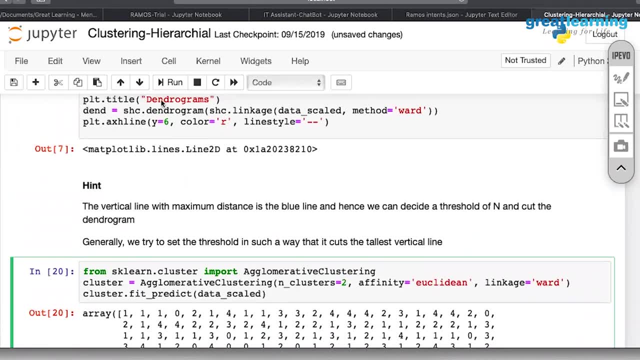 So it's supposed to pass from here. So in that case we'll get only two clusters. visually, only they can confirm this thing. So here, what I will do is I will change this to two. Okay, so I think let it come here. 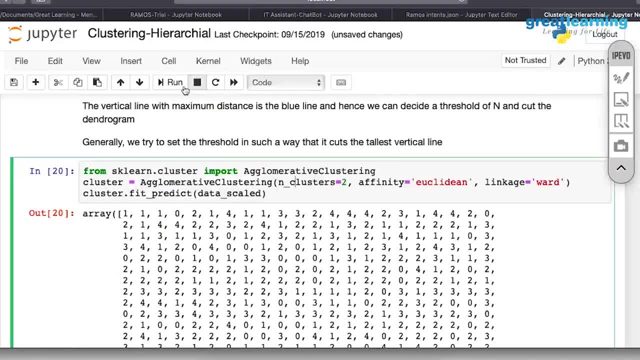 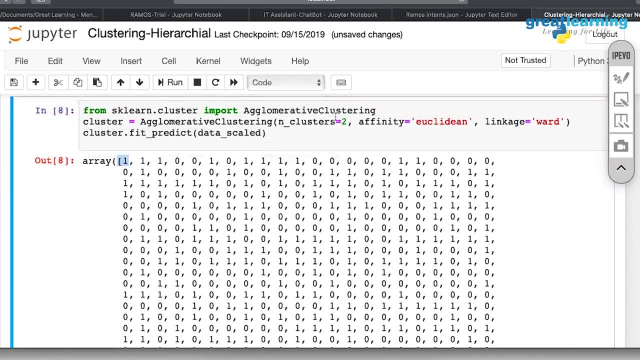 So it is cutting through lines. So definitely there are two clusters. and when I read on this model, yeah, we are going to get either zero or one, because the target column is nothing but number of clusters is two. That's it, And the distance we are using is Euclidean. 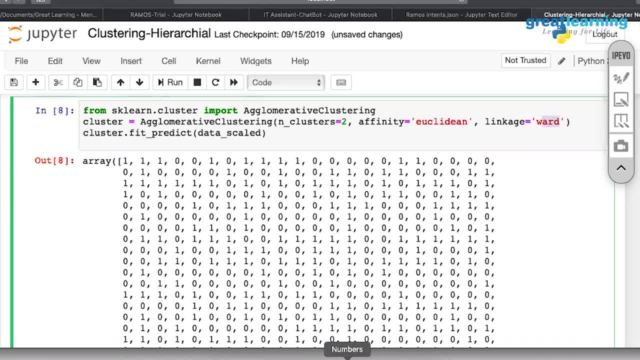 Okay, and the linkage: if you see, over here we have used proximity matrix like that, that having some ward technique over here, that having some ward technique over here, that having some ward technique over here, to find the linkage as simple as that. 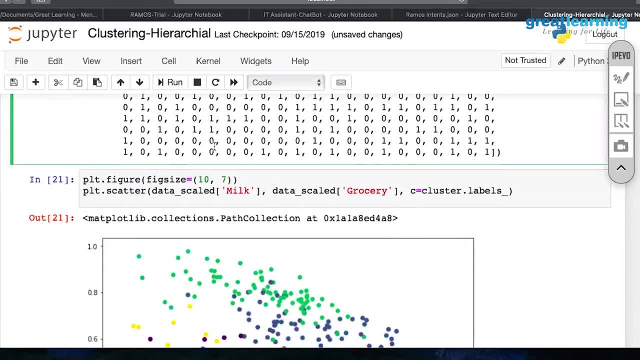 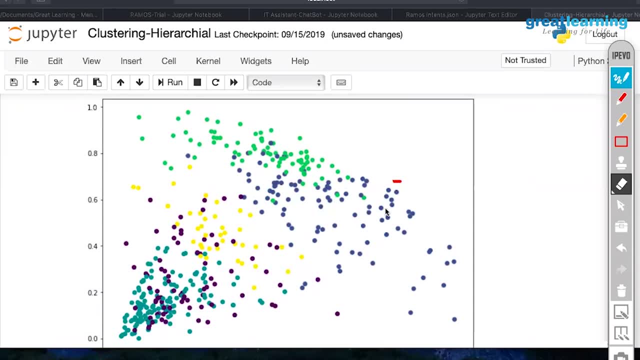 Okay, so this was your hierarchical clustering. If you want to plot the same amount of points, you can use a plot here, but I don't think so It's going to make a difference, because definitely none of these clustering techniques will give you separate plots. 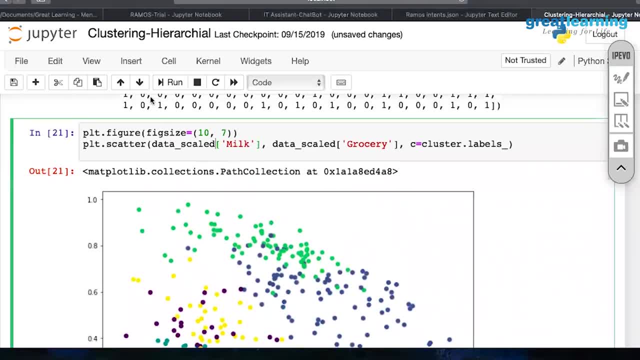 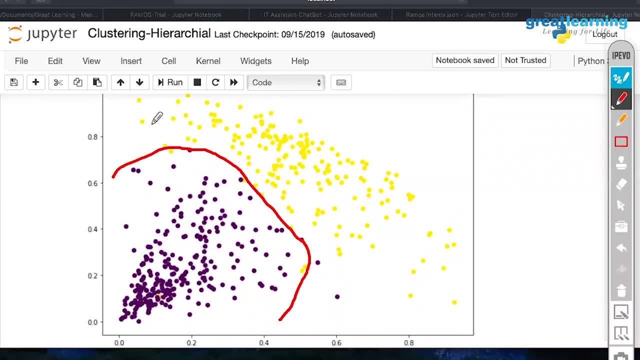 So here we had done a number of plots as five. Let's try to see if we can plot for two. Yeah, So if you have got only two clusters then I will say, yes, there is a good amount of difference. Okay, so majorly you can see this type of applications could be used. 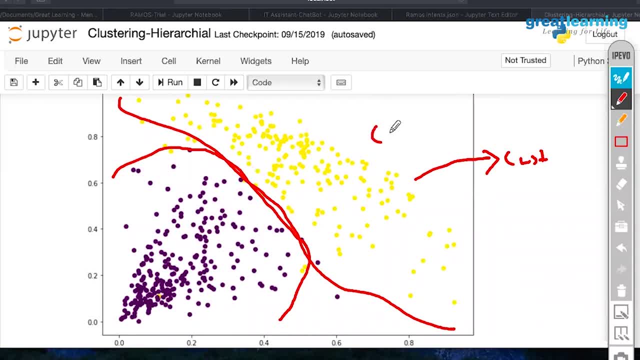 to classify customers into marketing techniques. So if, in case, you are running a campaign, you can easily use this to basically separate them, or else worst case will be your project. in this project You can observe that example where you already have a target variable. 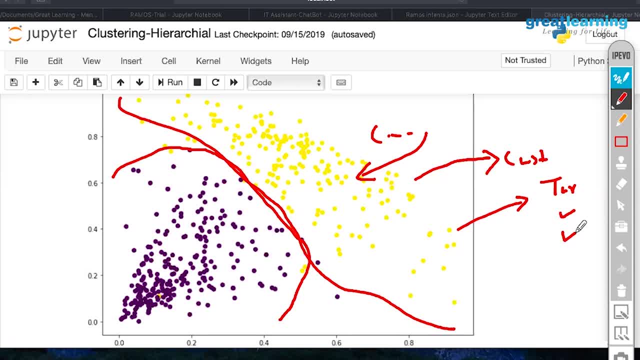 but yet we are not sure whatever we are given as a target is correct. In that case, we'll bring in unsupervised learning to reassure that it is our target variable. Okay, so I will discuss about that right away. Okay, so for now, any issues with hierarchical. 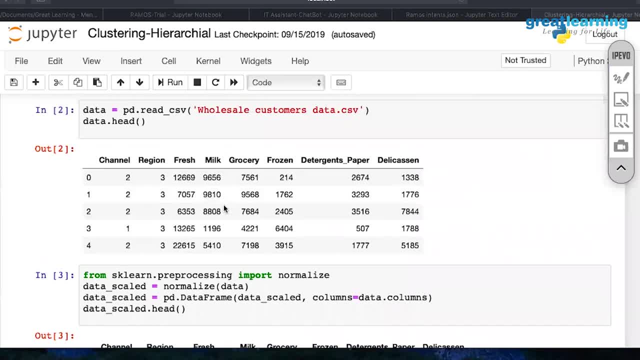 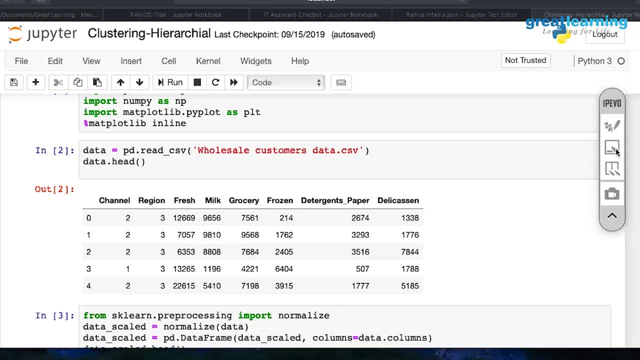 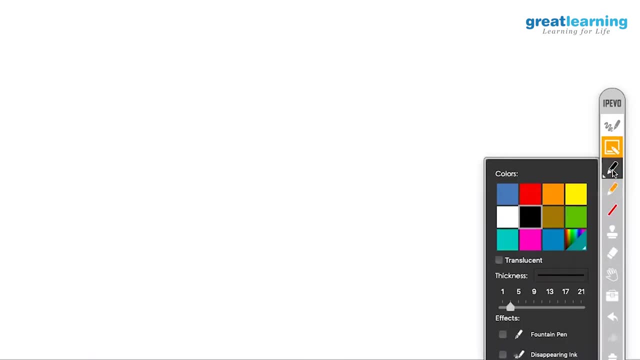 this is the simplest form of clustering that we can use about. Okay guys, fine, Perfect. Now coming to unsupervised learning. So I think we are done with machine learning. So now you guys are good with super Wise and you are good with unsupervised learning. still, we are supposed to do. 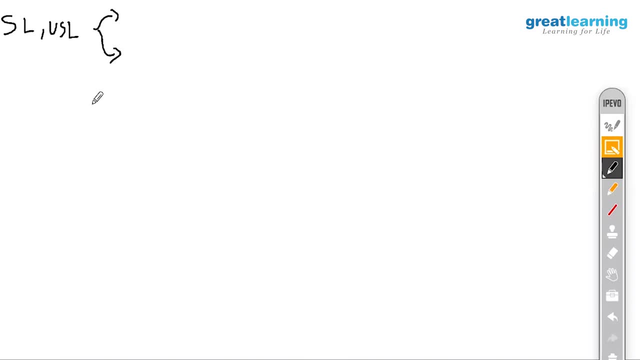 I'm supposed to show you, or I want to basically show you, two more techniques. One is called SVD and one is called factor analysis. So if you remember, we had discussed about PCA. So this is another version of that is called factoring. 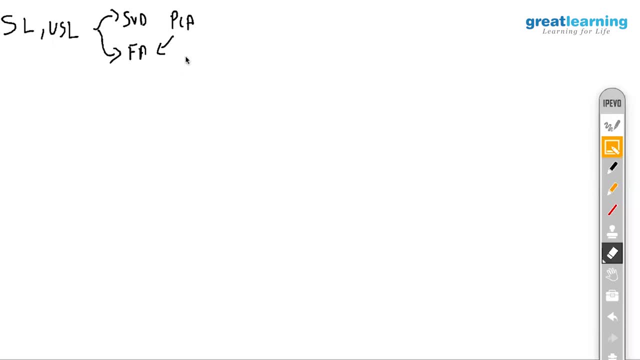 So, one by one, I will show you. Okay, So if you complete these two algorithms also, then they can say you have mastered unsupervised learning completely. Yeah, now please remember one thing: do not stop or do not keep in mind that unsupervised learning means no target variable. 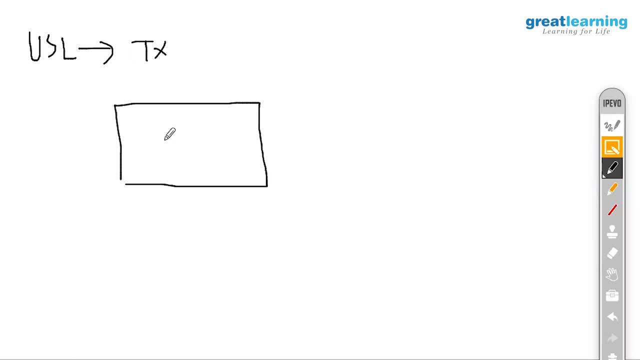 Please don't do that. Sometimes what happens is when you have a data set, So sometimes even the client is. let us say, this is an independent set of variables and this is your target variable. So sometimes when you observe the target, it is not necessary. 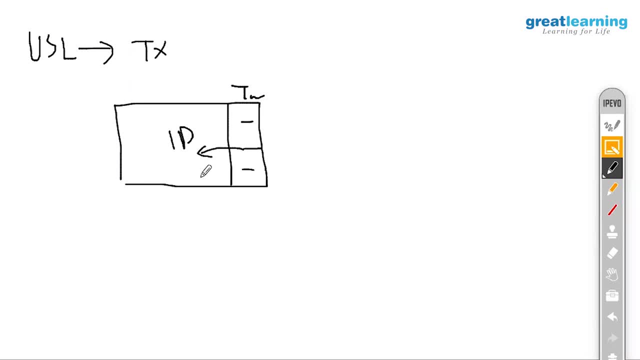 that it's going to be hundred percent. as for your independent variable, Sometimes there are errors in this. In those cases where you are not sure whether the target variable is good or bad, try to ignore it, or try to retain it, but ignore it in the data set. don't use it. use this particular thing. 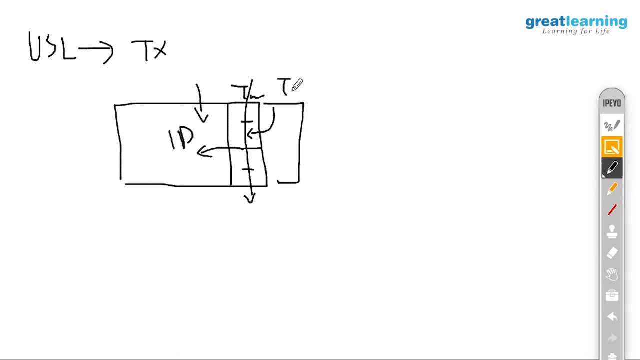 on unsupervised learning and try to create your own target variable. Okay, Once you do that, try to compare the difference between the this and this. Okay, How do we do this now? So let us say you have got an original actual target variable and a predicted- predicted in the sense. 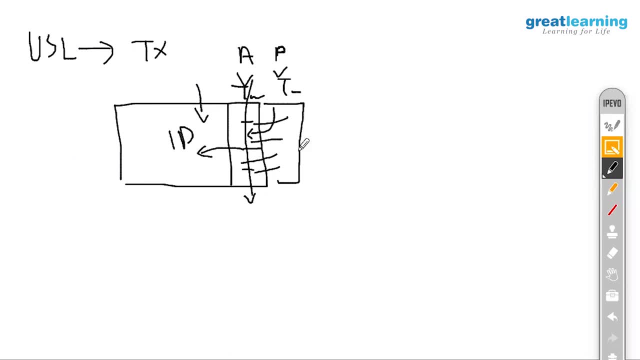 I will say clustered target variable. So how do we do take a difference is very simple. You can bring in the concept of RMS. Do we know RMSE? What is RMSE guys? How do we compare two columns? Basically, if I want to very simple, root mean square and error. error is what actual minus predict. 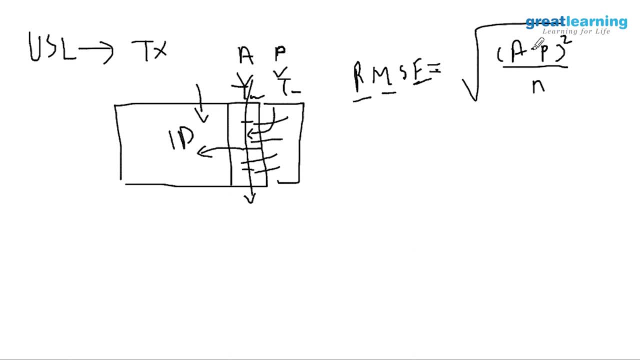 Or whatever you can say: old minus new, or new minus old- anyway it's square. So when you do this, I say, if your percentage is between 0 to 10, you can say that both of them are almost similar, But if you have a huge amount of difference here, 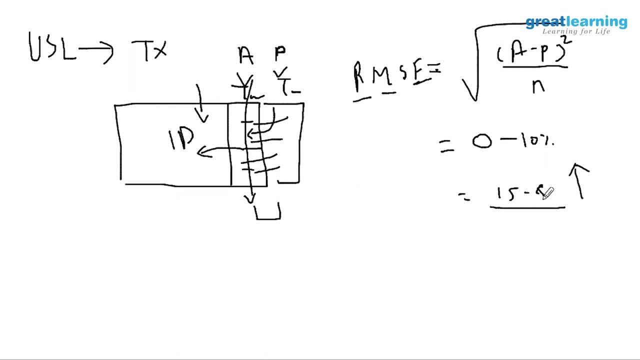 let us say 15 to 80,. let us say: then you can definitely say that both of them very pretty high, Okay, So this is one way to check. another way to check is using your dot describe function. You will find a mean, median and mode for this. 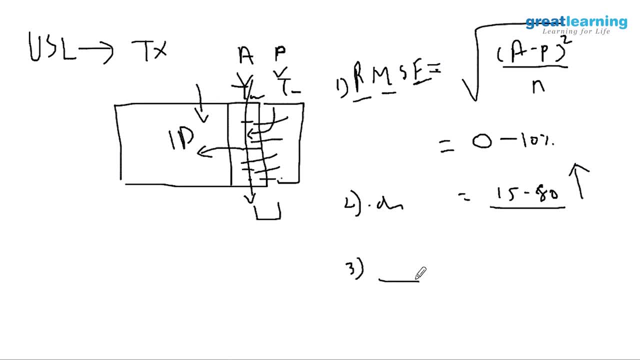 You will get it. or else you can put a box plot. It will give you the complete picture, so you can use one of them. If you want actual numbers, I will say: use RMSE. Yeah, so RMSE is very simple: just convert, just put a for loop, basically. 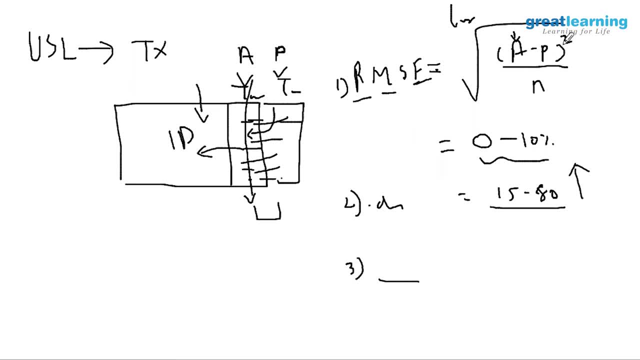 and bring in every time one value from this data set, one value from this data set, and do this operation onto it and store it in a number. Okay, So this is what you can do to value Date. whether you have done is good or bad. 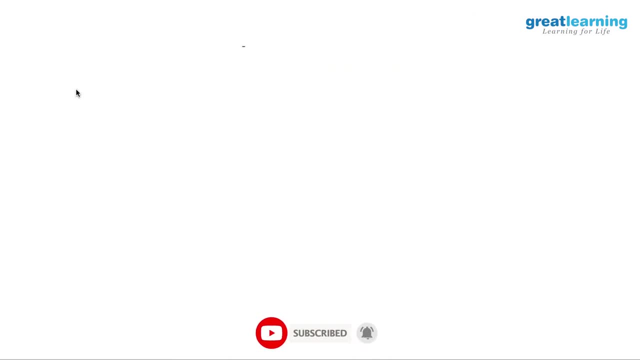 So this was your unsupervised learning. So you guys now are throw with machine learning. This is what machine learning does, Yeah. now coming to one very simple concept was, if you talk about ML, Yeah, what did you do? keeping Target in mind? 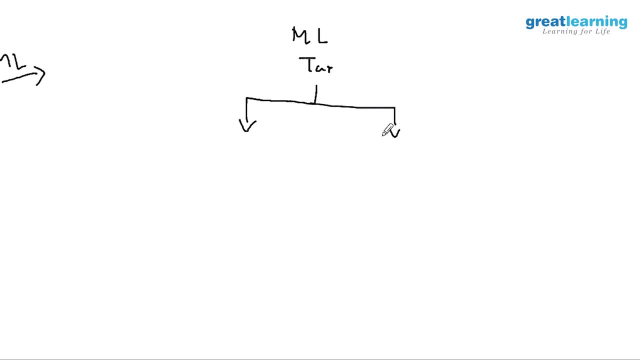 We splitted our ML into two parts. one is called supervised learning, one is called unsupervised learning. Again, keeping the Target in mind, We had split into continuous Target and categorical Target. Okay, continuous ones, all wear regressors and categorical one, or wear classifiers, as we had done. 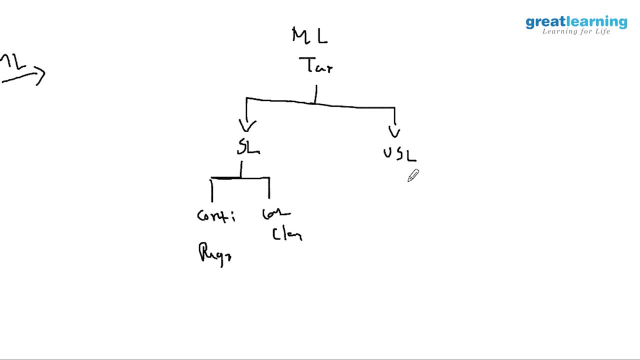 Yeah, post that. when we come to unsupervised learning again, I will say we can spread this unsupervised learning into two parts. One is called dimensional reduction, one is called clustering. inside clustering You can have multiple types of clustering. So we have got K means agglomerative and hierarchy. 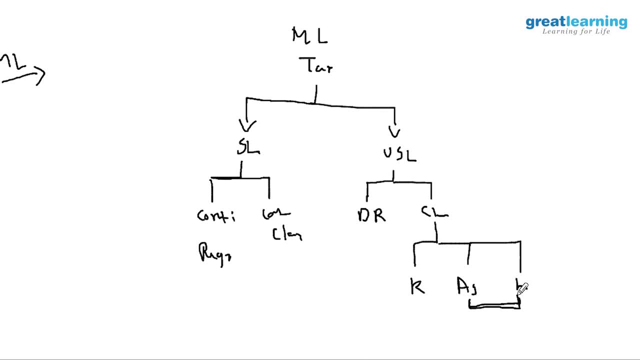 They both are almost similar, except some part of it. If you want still the difference onto it, I will. I will give you something in the next session with an example. Okay, and if you are looking for dimensional reduction, again, we have got multiple techniques here. 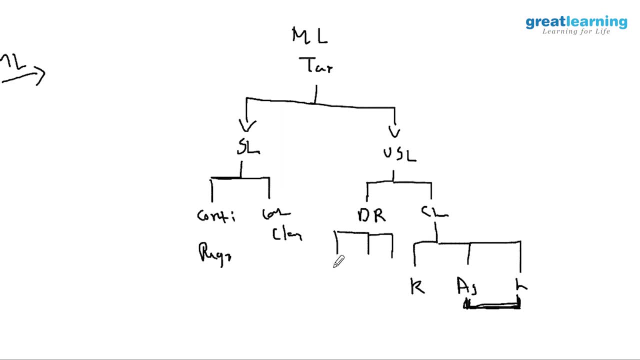 So if we are looking at dimensional reductions from columns, keeping columns in mind, we can have PCA. If you are looking dimensional reduction keeping rows in our mind, I will say factor analysis and if you are looking for overall dimensional reduction, we, whether it's column or a row, 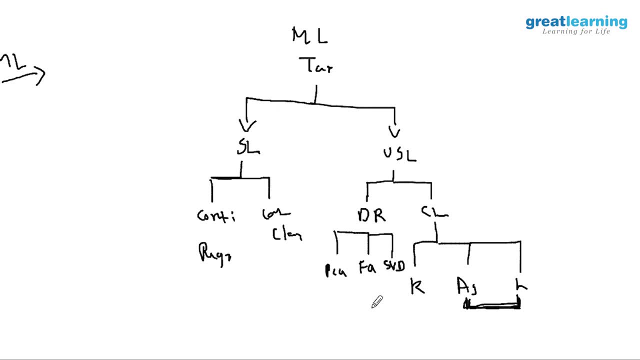 We don't care about it. We call it SVD- singular value decomposition. Yeah, so we. I will show you SVD and FA. anyway, today, if time permits will talk about SVD, I will show you one live example on SVD and how we do it post. 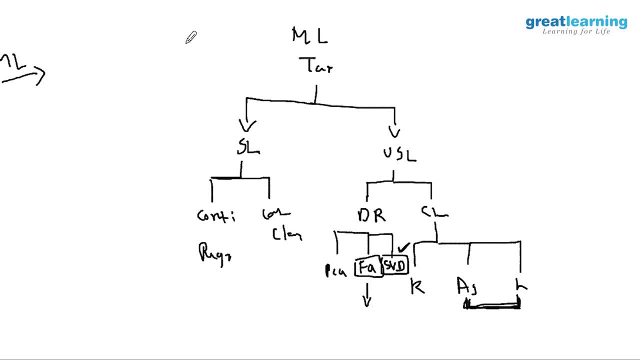 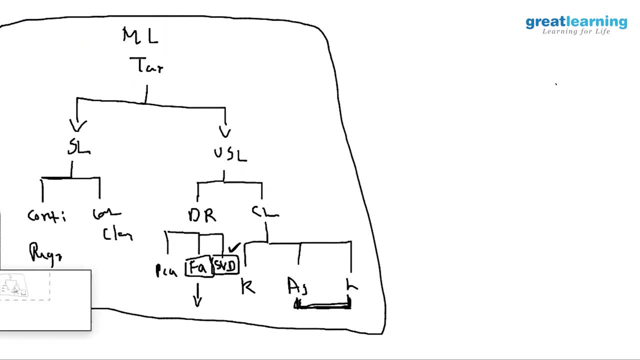 That we can. we can see a fail. So this was your overall machine learning. Okay, Now, please remember guys, whatever, whatever we are doing here, the concept remains almost similar, wherein you have got one box, you train it, you learn something. So this is your learns and this is your prediction. now disconnect your training, put in your testing. 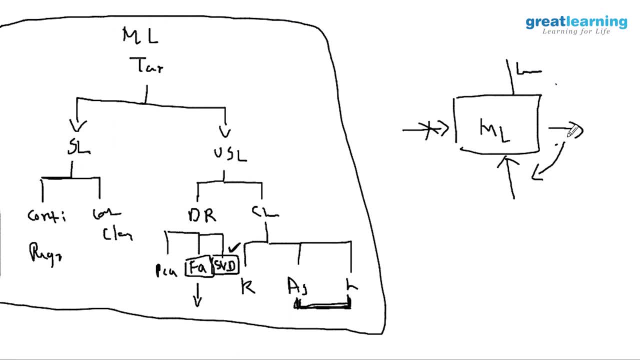 and do the prediction so that the accuracy or the recall or a precision Is calculated using comparing your test versus your. Okay, so this was your machine learning. So any questions on to this guys. you want me to repeat anything on to ML or you want to revisit any concept and be happy to do it. 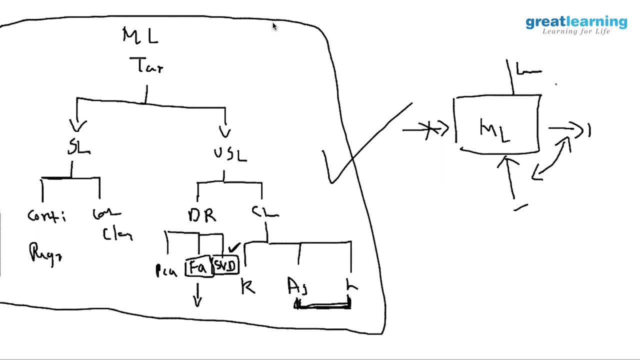 I have one question, or question No, I will just was going through some article in that The internet like the most possible algorithms. what we use in the industry mentioned Maybe, I think, four or five algorithms on that very regular, Is it true? 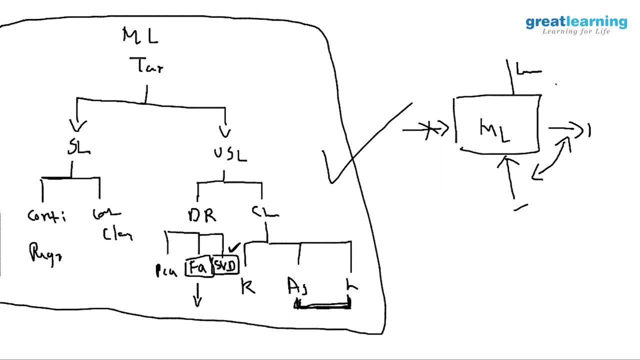 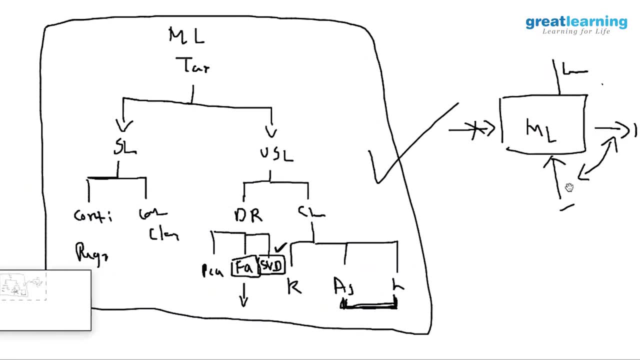 Yes, Again, I will say it's a generalization, but yes, they are. they are kind of true, So I'll give you. you want an example on to that or you want to discuss on to that? Yeah, Yeah, if you can use some examples. 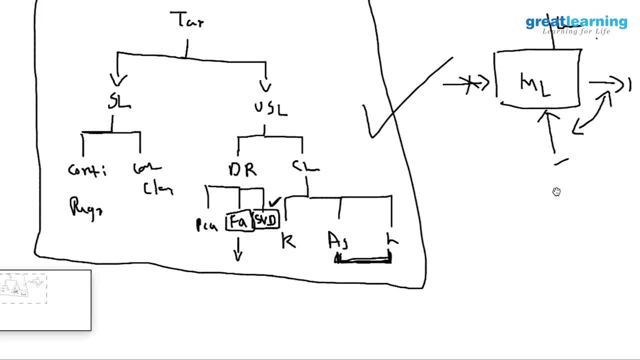 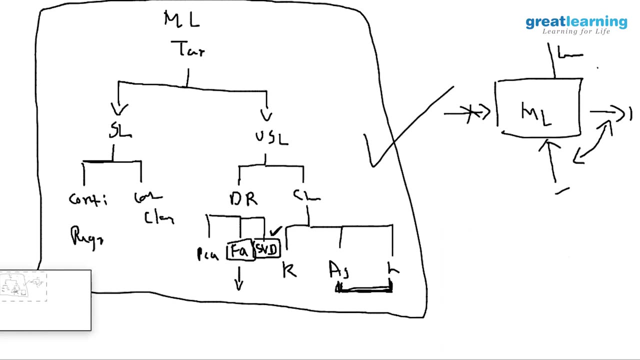 Okay, linear, and I was reading that in your logistics decision tree- and then correct base and random for this other algorithms They use very frequently, Correct, Correct, You are right. So now let me show you that. those things. one minute, give me a minute. 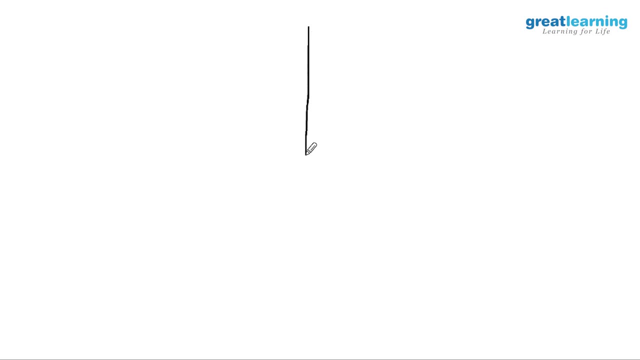 So let me divide the domains and then we'll check about, we'll talk about what all algorithms are going better in which domain. But in the, in our project and all what we have seen is like you do all the EDA activity and later just you are putting a code of particular machine learning. 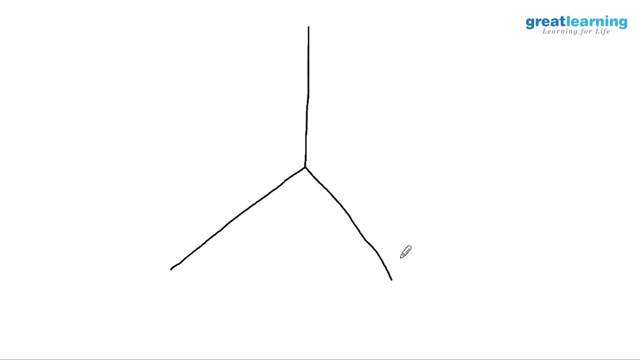 That's it. That's it, That's all. even in the industry, It's the same thing. Whatever codes I have delivered to you know the same codes. You can use it on your industry side. So that means no more than algorithm. 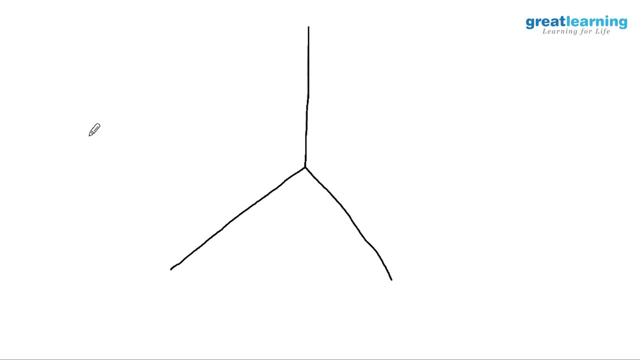 You need to understand the previous, the work more. Yeah, I will say both the ways, Okay, both of them are interdependency. Why do I say this is, let us say, this is your data, Okay, So the first thing we are supposed to do is we are supposed to prepare the data. 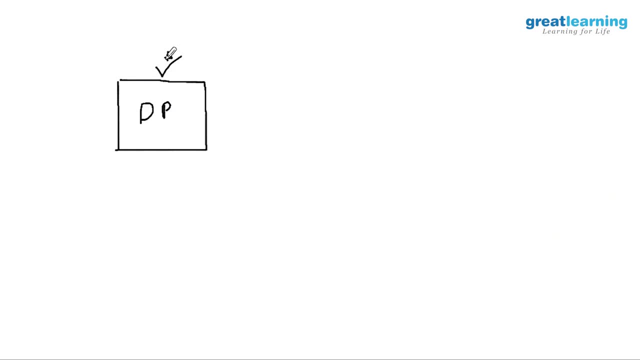 The data should be good enough. So, yes, it is highly important, Definitely. next comes your modeling. So I will say machine learning modeling. now again in machine learning modeling, If you remember, under decision tree, let us say we take decision tree. Do you remember all the? 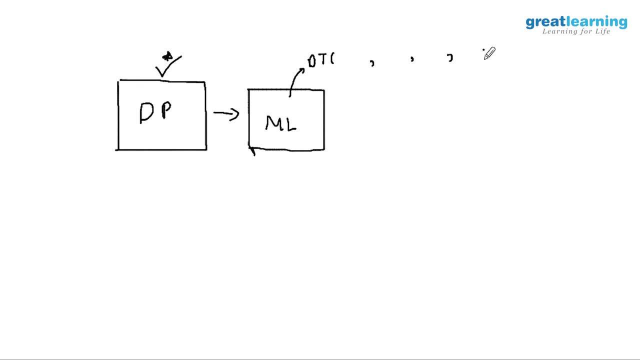 Hyper parameters inside decision tree. What all we use inside decision tree. Do you remember maximum number of leaf nodes, minimum split per leaf node, Max depth: Do you remember all those things? Yeah, how many of them we used. Did we use all of them or we use only very few of them, very few of them, exactly. 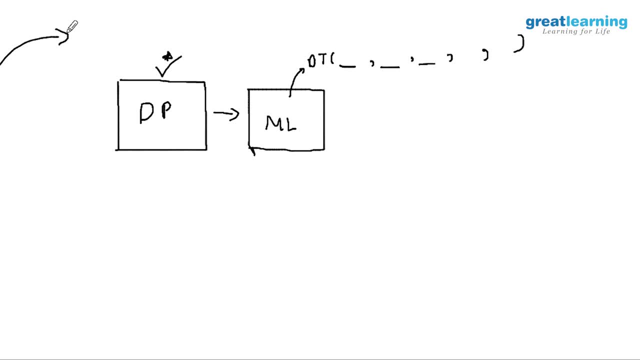 So now the next module that you have after this unsupervised Learning is called feature engineer. So they're in. we will fine-tune this thing. Okay, as we fine-tune this, we have never, ever fine-tuned our models, Have we done? we have never done it. 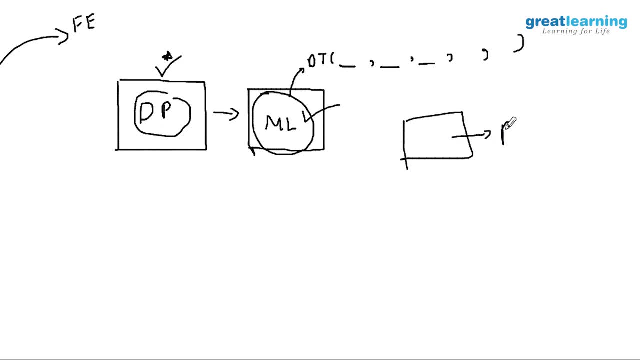 We just implement one patch of code, We get a prediction or we get an accuracy, and we leave it there, right? So your question is perfectly valid, that how come a very complex thing is just a box. Now the complexity will start where we will fine-tune these. 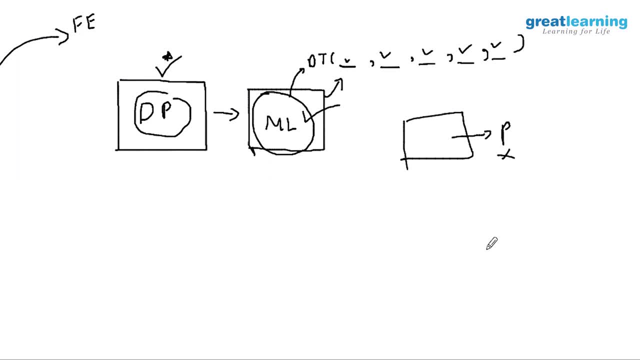 Okay, Yeah, it's like, if you remember, you know in this older, The cost if you go for this PUC certificate. Yeah, so my dad had an old 17 year olds then. so once when after service, when we went for PUC. 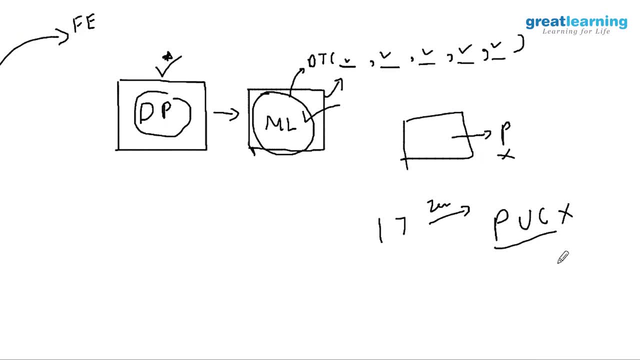 you know, the certificate failed. the PUC was. the person was not able to validate. it is saying this: the carbon content was pretty high. So what happened was my dad called this Maruti guy and there is certain stuff which he knows. there were certain screws and all in the carburetor which he just, you know, loosen it up or I. 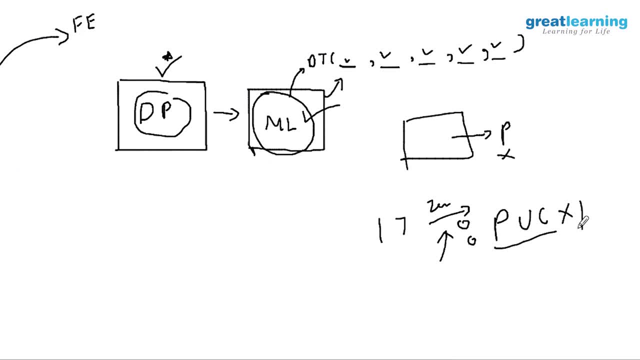 think, tighten up something. He did such a way that the carbon emission had exactly come down. So this is what we are going to do now here, fine-tuning part of machine learning. So in our decision tree, or random for us, What all, we use, Max, we used how many estimators we want, not in decision tree, random forest. 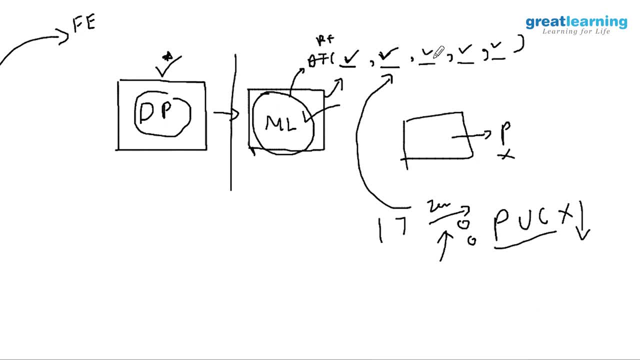 right. Do we want? do we consider OB error, Yes or no? and that's what we used. now We will get introduced to almost all the features in random forest, How we can play around with this numbers and increase the accuracy. So let us say, when you did your random forest, the code that has given you with just two. 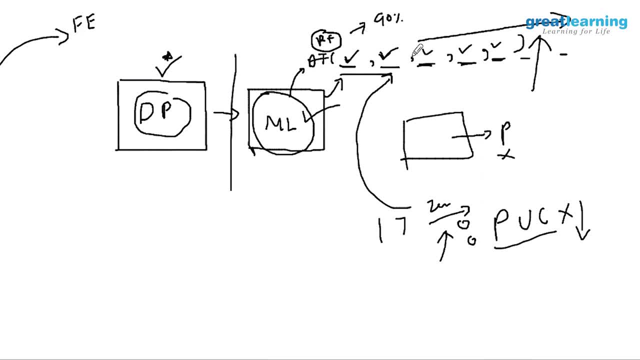 features. you got an accuracy of 90%. say what if I included all of them? I fine-tuned them and I was able to improvise accuracy to 95%. this is what we call feature engineering. Yeah, and this is a little troublesome topic because here we have to do a lot of understanding. 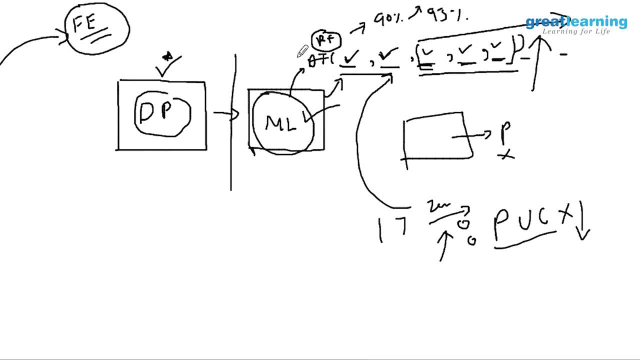 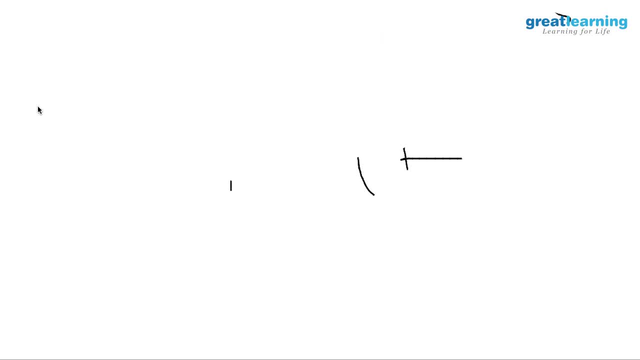 on mix matching and all. Yeah, I hope I answered your question. Yeah, yeah, perfect. So thinking that no, in the video also so mentioned. or you can use couple of other machine learning tools to make X and Y and train and test and then they can put any code. 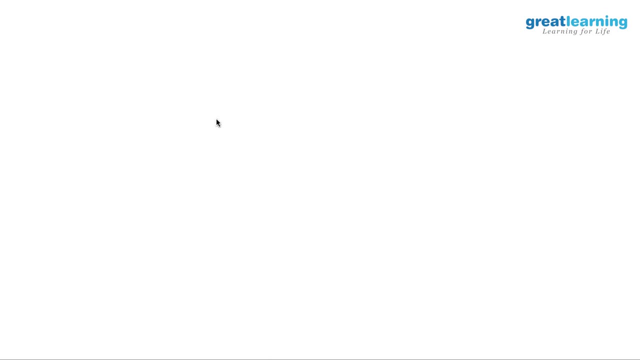 Yeah, correct, You can put any code, but not all the codes will fit on to a good accuracy. So we can fine-tune. and what is my the good thing about my codes is my codes are universal. So, if you observe, some of the codes are given you. there are no dependencies that accept. 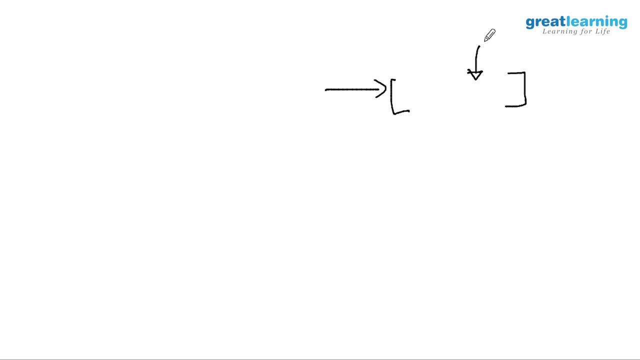 input the data that we are giving. that's yeah, so that is the best. So now we will learn about in the next one. So today I'm going to discuss the same thing with you guys on what exactly is next module and how we can differentiate it. 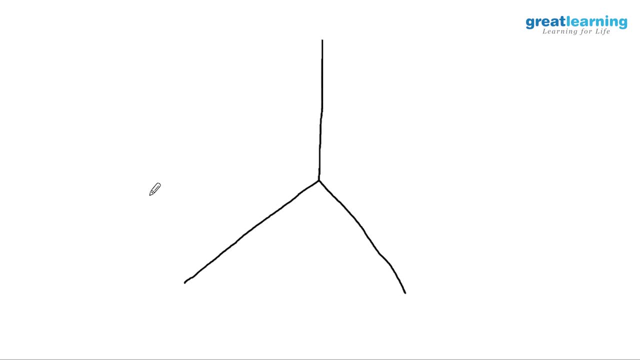 Yeah. Now let's try to understand machine learning with popular algorithms, in which field we use? Yeah. So the first one. let us say we are talking about sales, Yeah, And marketing. I'll put these two together. Okay, then I will say production environment, a, I will say testing environment. 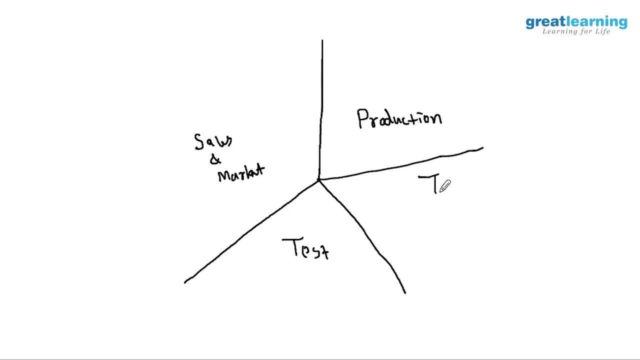 Then if I want to okay production and test, I'll put it here. It'll be unfair for me to create a new domain. Then if, in case, we are talking about finance, financial domain- Okay, what if we are talking about automotive domain? What if we are talking about what do we call that? 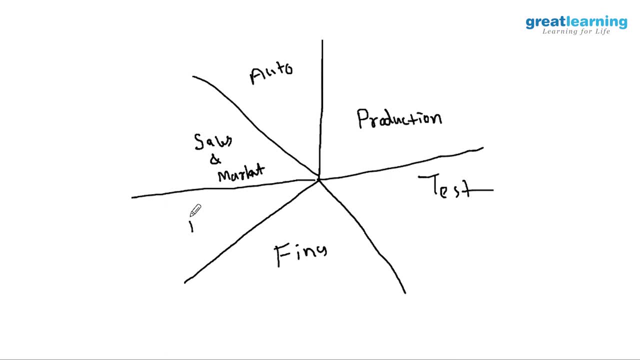 This online Amazon and all what, what do we name it? Amazon, Flipkart and all those sectors? Yeah, so we can divide our markets into multiple stuff. Okay, So let me say production and production plus testing and market. Okay, Here we can say HR and policies. 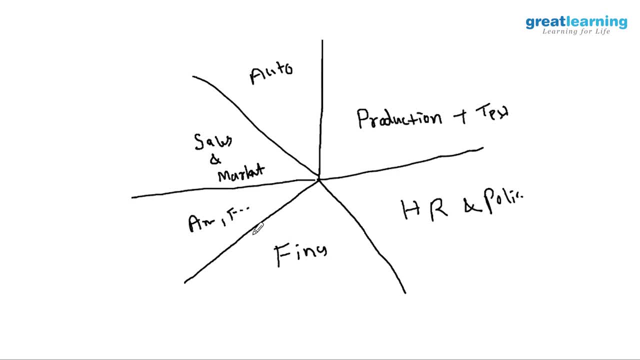 Okay, So we can have multiple domains like this. Now, if we are looking at sales and marketing, for example, then what? what will we do? is we do revenue focus, revenue deficit? then if, in case, you want to do a campaign, how do? 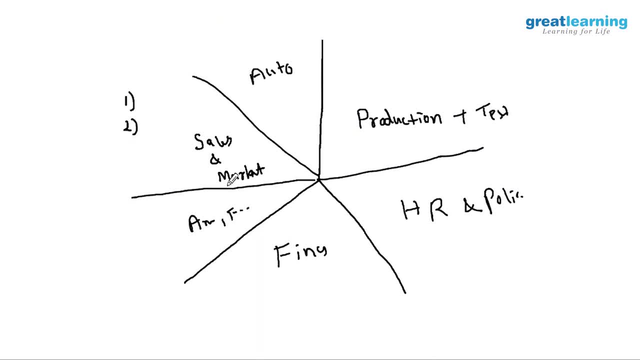 we cluster the people whom we like or whom we think they are going to convert, and all this. So in this case I will say clustering, We will play a very important role for market- Okay, and sales are in my model- We'll play a very important role. 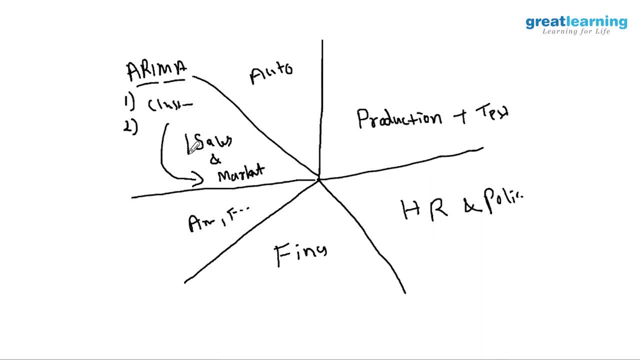 What is Arima is basically it's used for, and this is the only algorithm which will give you exact sales predictions. Okay, so I'm not sure if I've discussed this algorithm with you guys. so far, I think I am not. Yeah, I'll soon do it. 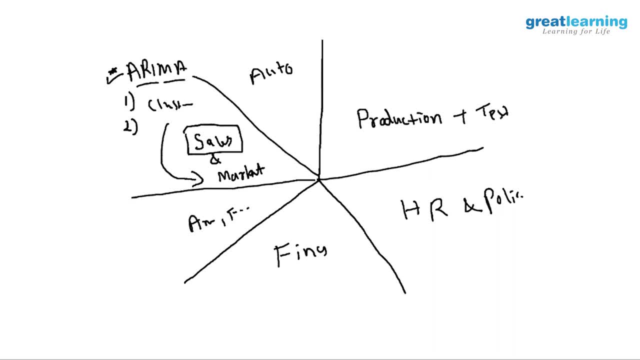 We'll soon take. some will try to find a time slot and we'll do it, Because I need at least 45 minutes to go through this, this topic, Yeah, Next, if we are talking about HR and policies kind of thing. So here we have a separate domain called HR analytics. 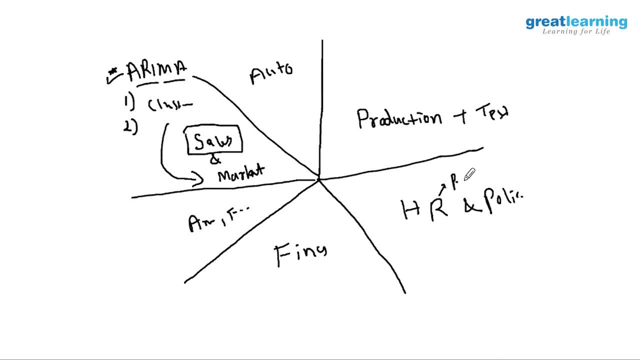 So again here what what we'll do is. we can predict performances. We can also predict when the person is going to leave lot of things up. So in this one I would say we'll not use pure analytics, but we'll purely use Edie. 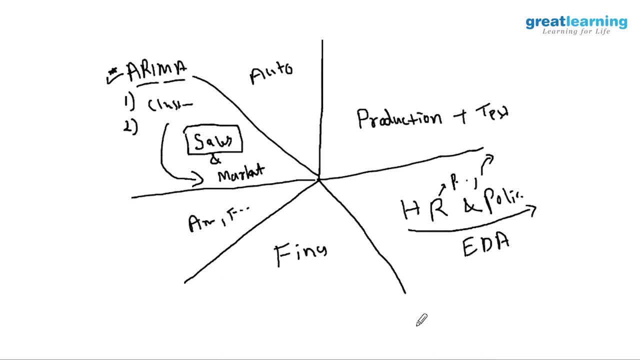 Explore A tree data analysis will try to put some plots of people who are on this side, of people who are on another side. For example, for financial domains, I will say a regressors, majorly linear, quadratic, polynomial regressors or logistic regressor. these decision tree regressor random for us. 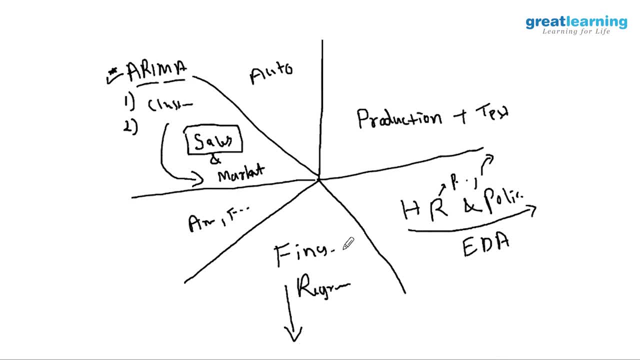 all the regressors that you have. you are going to see definitely on the financial domains. No more clustering here, but they're again. now. what is happening is, since cluster classifications Are Becoming a better part of it, So from regression they are now going towards a little bit about classification. 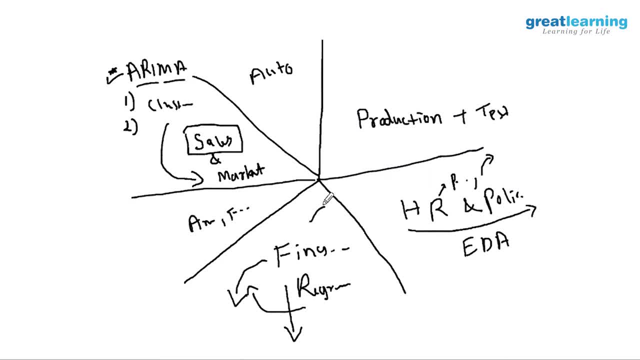 So if you talk about finance, who are going to, basically, which customers are going to default, who are not going to default, or which customer is going to buy our load, which customer is not going to buy? So on those applications you can use classification. remaining majorly on financial insurance domain, 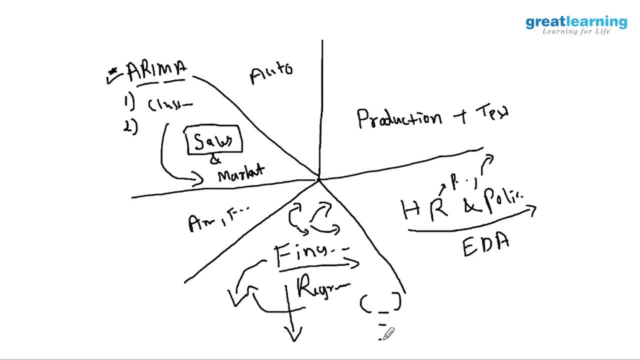 regressor size, because we need an exact number of loss that we are going to make from one customer. Okay, next is if we are talking about these online stores. So in this case we are going to use the recommender systems majorly and again we have classification. 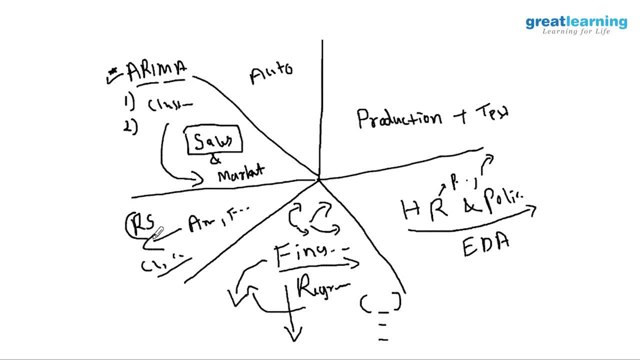 and clustering also included into it. So the recommendation system is nothing, but it's a part of our course Anyway. so basically it it recommends a customer. It's like a virtual sales agent for these guys. ever discuss this? earlier recommendations? No right. 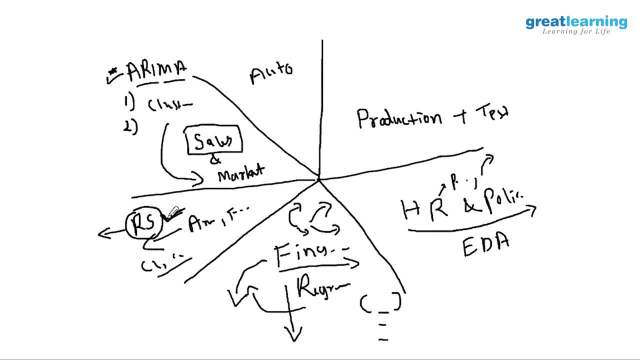 Yeah, you guys told me yes, No. So I'll also give you an overview on what our recommendation systems. if you guys, if you use Netflix- Yeah, you remember, when you, as soon as you log into a Netflix account, it shows you some. 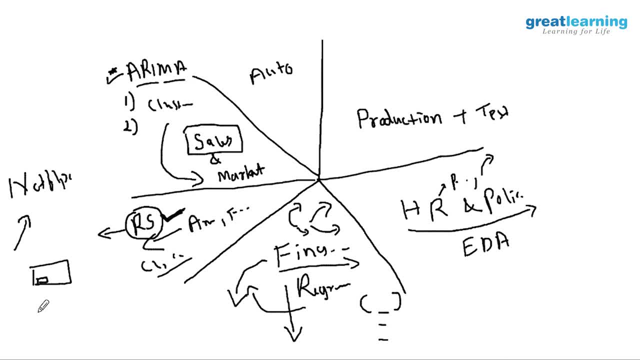 recommendation movies with some percentage. Have you seen that? Yeah, Yeah, this is what is recommendation, same with the mobile sales, Exactly, Exactly. So one question to you, the people who are using Netflix, Amazon Prime and all: have you ever searched a movie on Netflix? 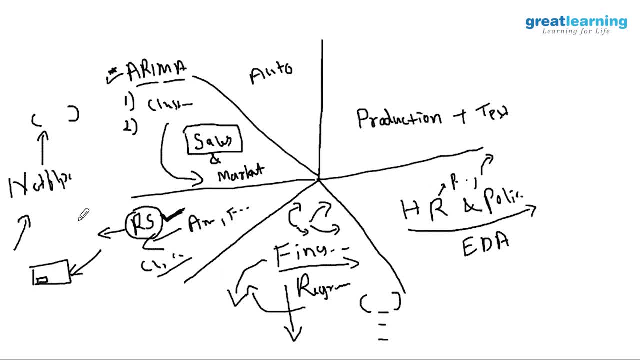 Or you, you go ahead with what you see on your screen. We have such does, both your such Okay. So, as per Netflix's survey, 90% of the customers, they go ahead with the recommendations. They don't go and search it because, because they don't, they don't get a time to search. 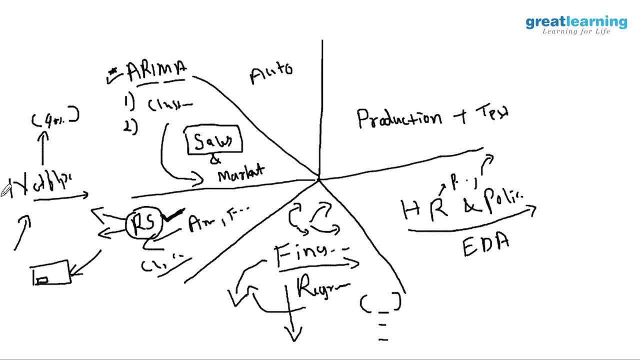 other than I'm one of them. you know, lazy guy. So whatever they show me, I just eat. Yeah, so this is one. we'll discuss about this In detail, Yeah, and next coming to production and test, So majorly, what we do is we used AI over here? 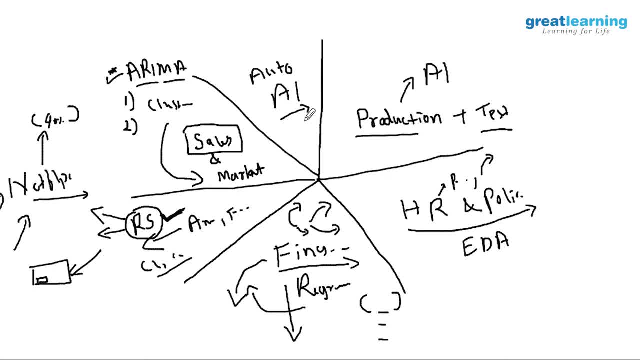 So automotive and this one we used, we are completely depend on AI, artificial intelligence. So probably after three modules we are going to see artificial intelligence anyway. So again I will say, yes, these are more popular algorithms, but you cannot say that. 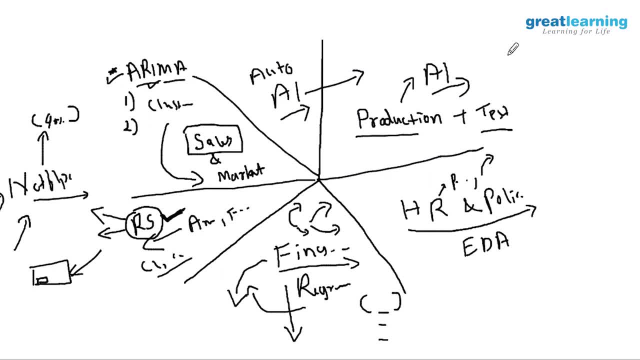 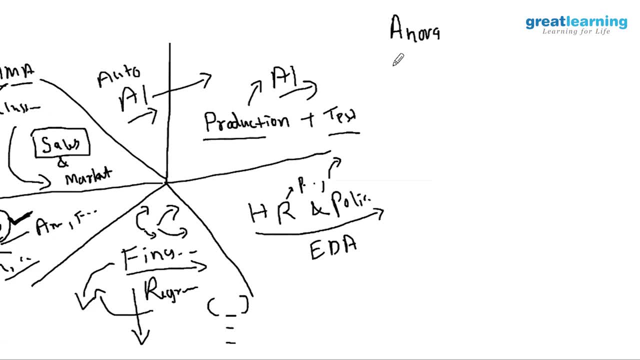 Okay, if you know this, you can master it. sometimes a very simple algorithm like ANOVA. We have done ANOVA, right guys? Yeah, sometimes I use ANOVA just to understand how different is my. let us say, I've got two. 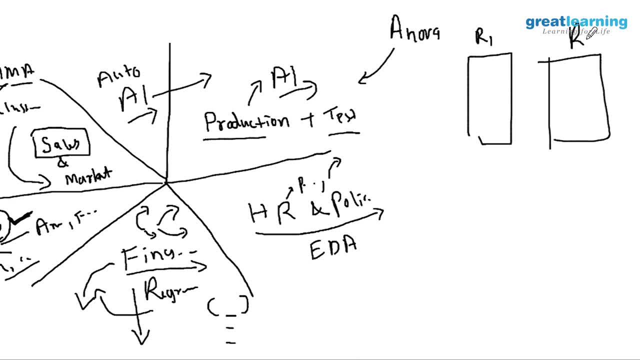 releases: release one of my code and release two. Okay, what I will do is I'll try to find out certain number of loops, certain number of pings or DB queries and lot of things. I'll try to find out and make a data set now. 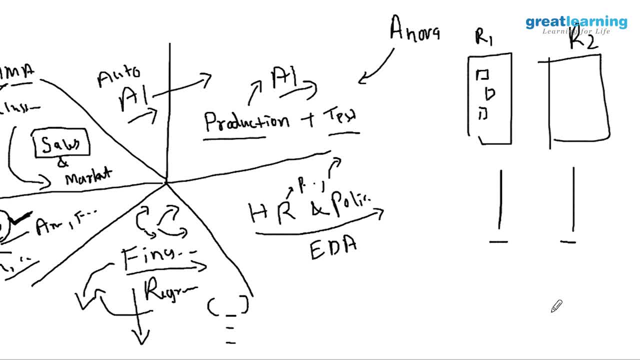 My duty is to compare how similar these two columns are. in that case, I will bring down As simple concept as ANOVA also, or I can say t-test in this case. agreed, right, What was t-test compared to columns? How similar they are. 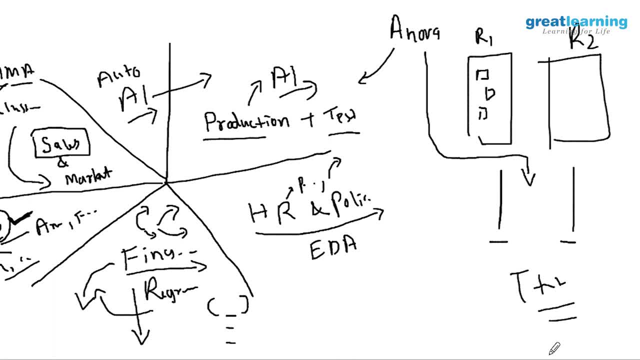 Yeah, that's it, Krishna. I have one question here, See, since we made this complete differentiation. like you know, I go in my production, you know NCG here, the know we have read to such a stage And okay, now with the basic is done. 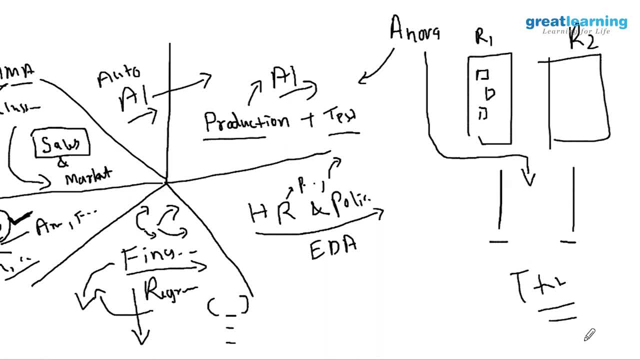 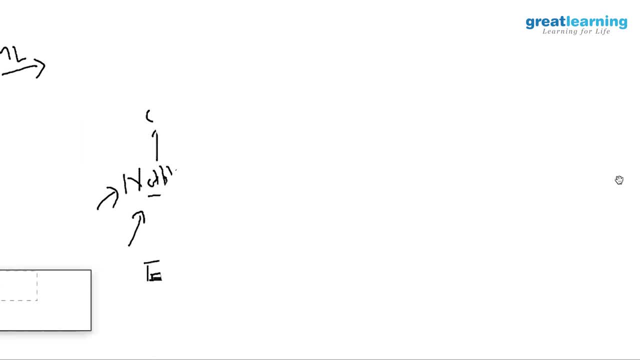 Do you suggest to know? we need to put more time on our domain area? Yes, Yes, you can do that. We are mixed here. You know some people are from sales Correct, So may I know from which background you are from? 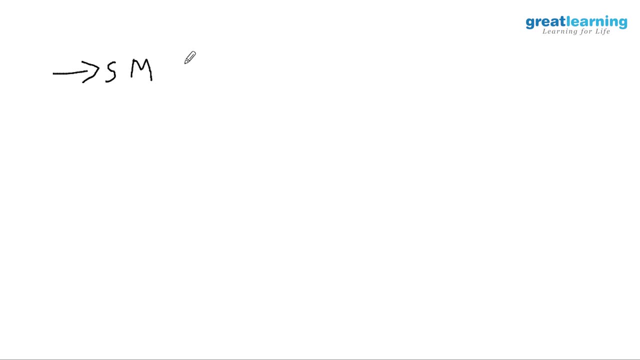 I'm from sales and marketing- sales and marketing, Exactly. So you will benefit the most out of this thing because you will have an amount of data available with you. So I will suggest you can pick up some of your client data sets or some campaign data. 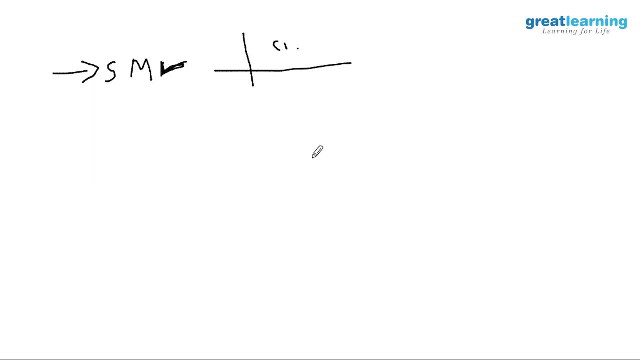 sets and try to start with the clustering. Yeah So try clustering, tries aggregating, try understanding how customers are getting separated, whether we have two clusters or we have three clusters or five clusters, how I can shift people from one cluster to another cluster. The strategy is part of it. 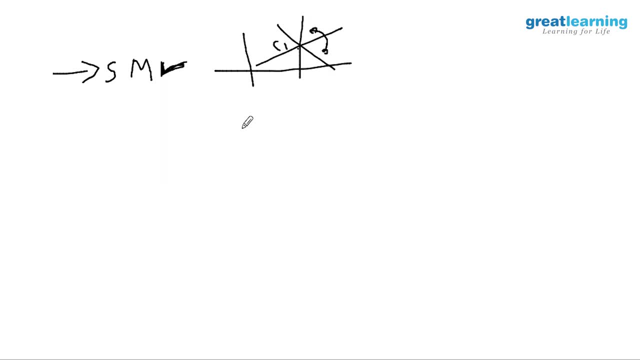 So for the strategy preparation anyway, you will need this: graphs, numbers. Second is for marketing. again I will say: Classification is another set of good alcohol, So you can pull out some of your campaign data And if, in case, you have got repeated customers on which you are doing campaigns, you can. 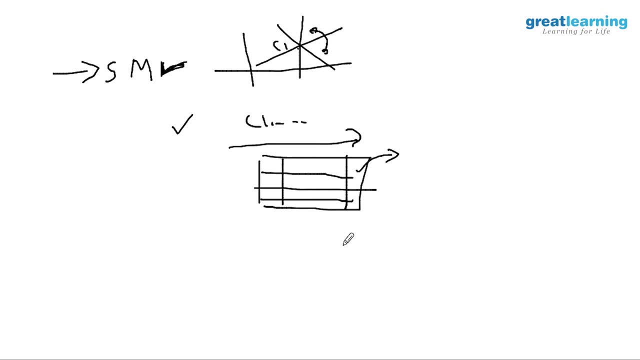 definitely come to know that which customer is going to buy what, depending on the attributes that you are collecting. So definitely you can start on to this, but I am not sure how niche the data will be with you, But usually these guys are the most beneficial ones because they have a good amount of data. 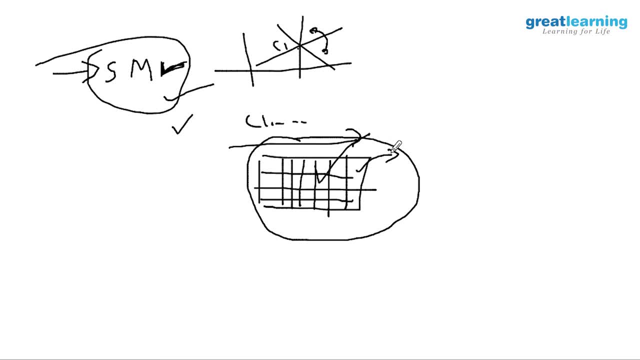 Yeah, So if you remember, we have we done any code on this and we done a project. we have done that portuguese bank project right, Or Portugal before Portugal. We have done one bank project is back Marley Ample project on miracles. 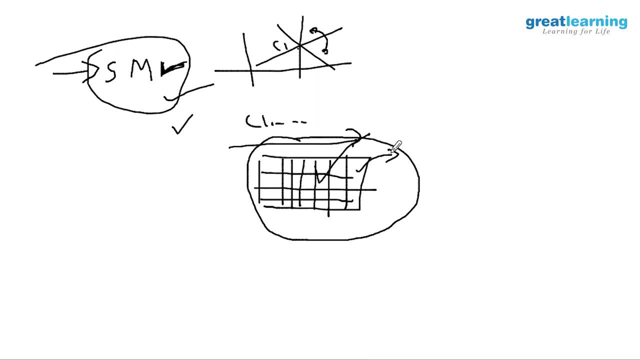 Correct, So you can use this, this concept, again. Yeah, Okay, And have I shown classification using AI anytime to you guys? No, I don't know. Right in last session Did I show you a prediction using AI? No, right. 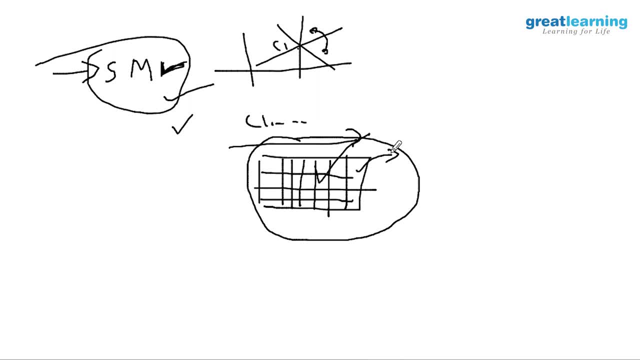 No, no, no. So today I will try to show you. I know you guys are not comfortable with the AI, So there will be some friction. That's the reason I was holding it back. But if, in case, you guys want to start it up in your own domain, I'll be very, very helpful. 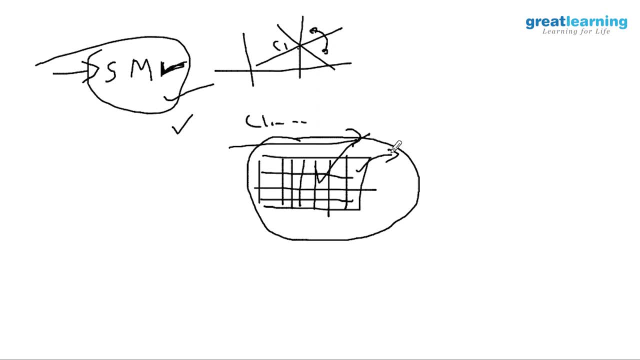 guys. So again, as I keep saying to all of my batches, don't wait for certification to get over. try to get hands-on to whatever data you want, or you have it, and try to start implementing your project itself. you know you will grow and you will. you definitely will, you will. 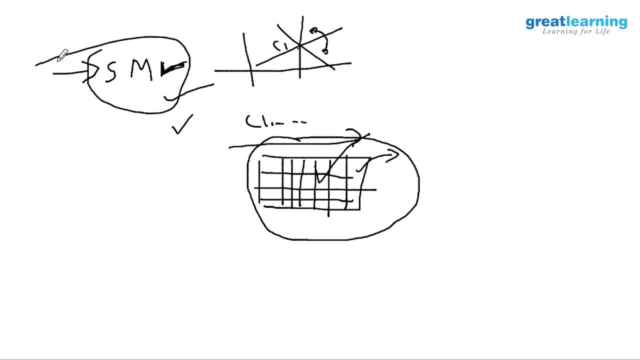 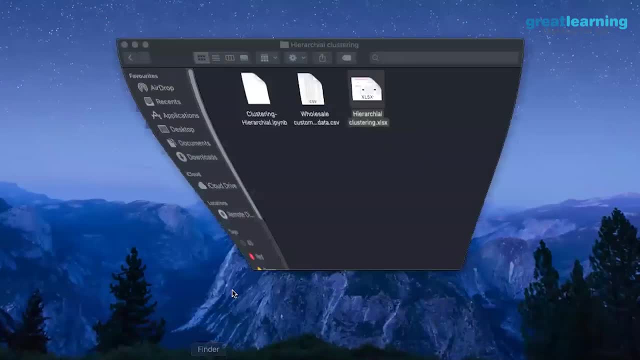 benefit something out of it. It is not from project point of view, but your own understanding also. Yeah, So if, in case you guys are interested, then as a common group I have got a very good implementation or a case study to share with all of you. 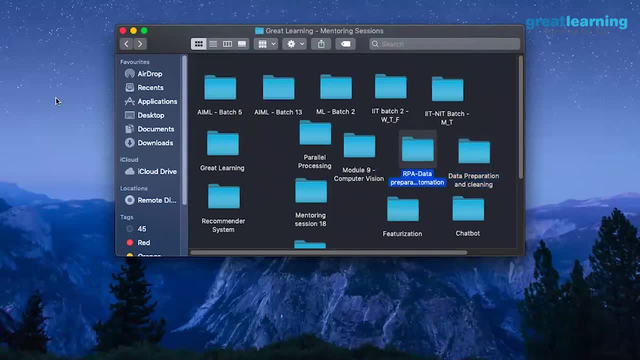 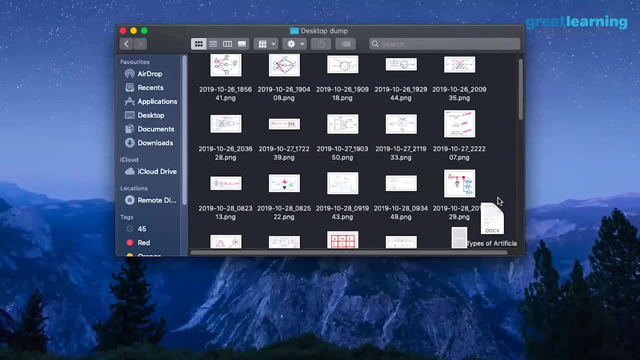 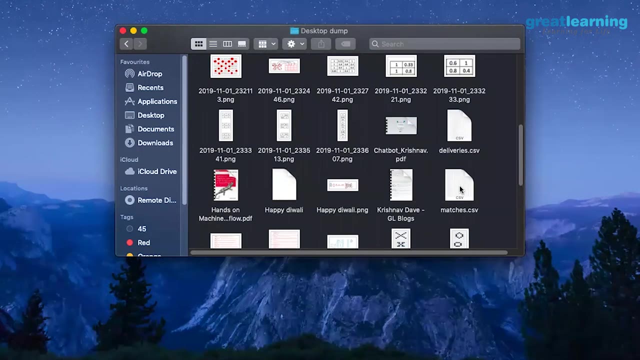 You guys can start from a scratch. This will be something extra, not a part of your assessment or anything. Give me one minute I'll try to pull that data out. There are- there are many projects solved and kept in the internet. you know that also. 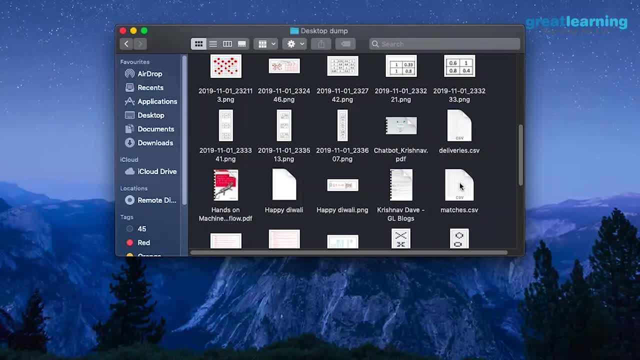 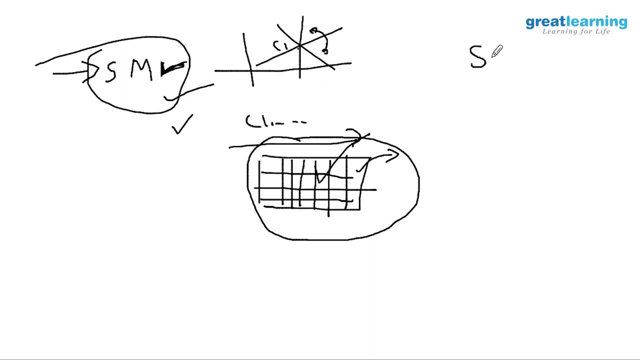 will be helpful. right for us. Exactly, Yes, it get, there will be, get will. you will get a lot of products on to get, or else, if you know Siraj Rawal- there is a YouTube channel fellow- whatever he explains, He has got a ready-made code on on kit. 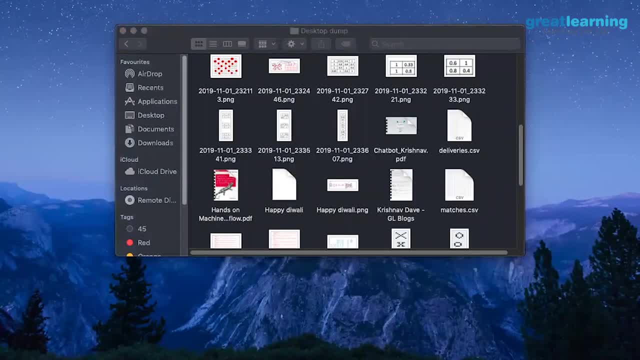 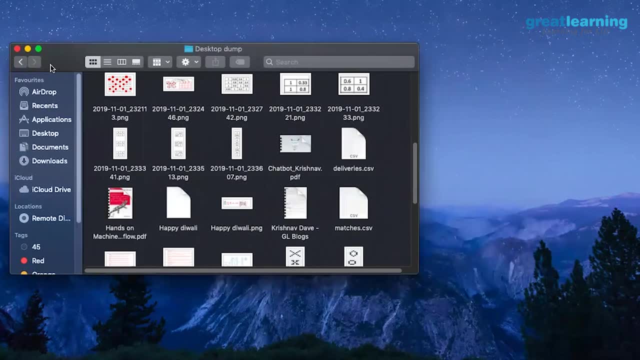 You can go and check it out. and one, one more thing: order understood is like this: projects and all how you analyze the project. that is important. right, Analyzing In the sense create the business problem or something, or you know, in the last four projects. 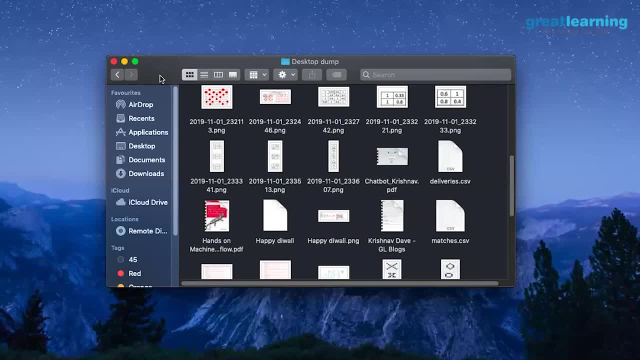 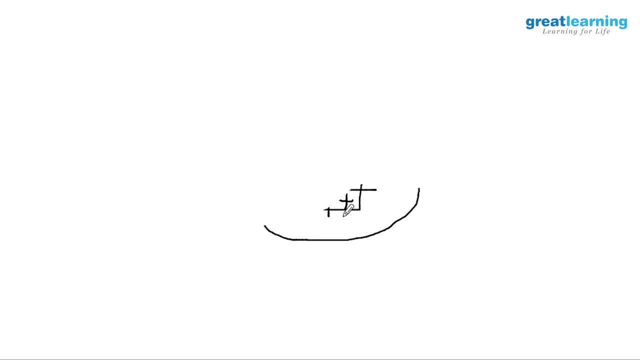 what they have given to us in that, the main, the like. the point was: like: you have to, you need to analyze the, the data, like how they are related each other. Correct, Correct, Yes, we are writing that. know below the how they, how they are related, all those things. 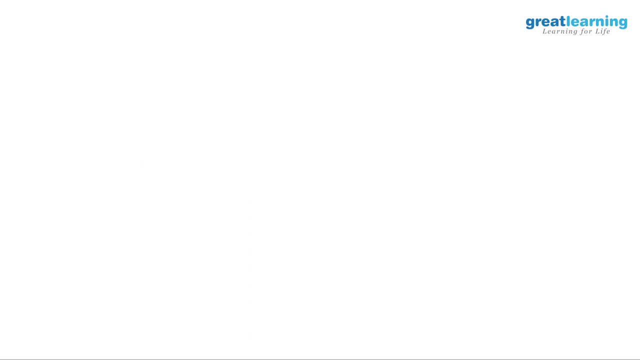 are writing, that means they are analyzing that and we are giving that to the customer. Correct, That is important. Yes, it is very important. So keeping that example. let's try to take a very simple example. So let us say you have got some data set. 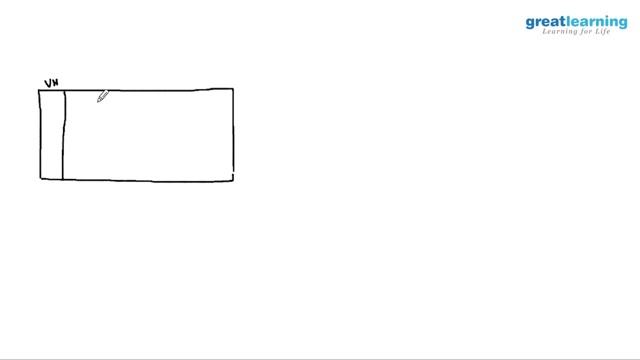 Okay, let us say these are user needs. for example, say: this is the age, Okay, this is the year of birth. Let us say or, but what? which year? you were born, basically, and there are some other attributes attached to you, for example, 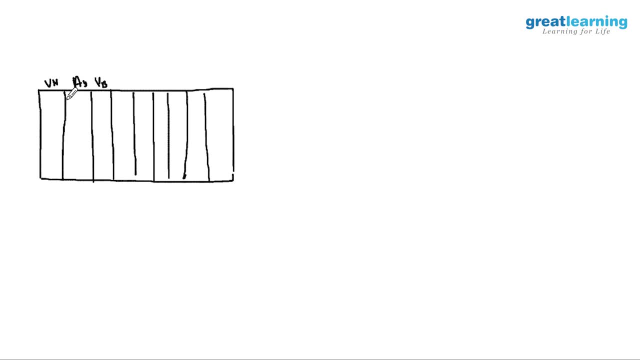 Yeah. Now what happens is not all of us are conditioned enough to understand, by looking at the data set, that some of these are similar. or let us say: this is your yearly salary and this is your monthly salary. So what happens is: what do we do? is we say, okay, we have got good amount of numbers? 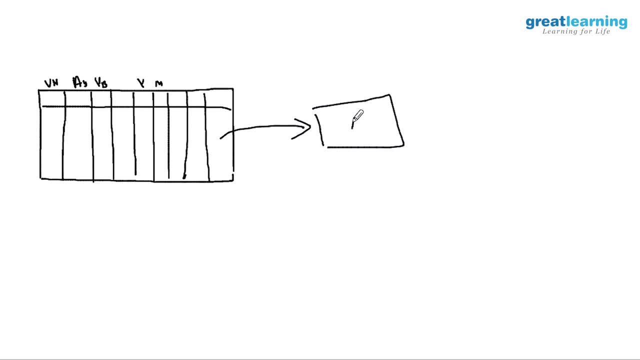 Let's push it on to data model. So machine learning will definitely take this model. but because of the presence of these two columns together, you know we are going to find a lot of multicollinearity. Have you guys heard about multicollinearity? 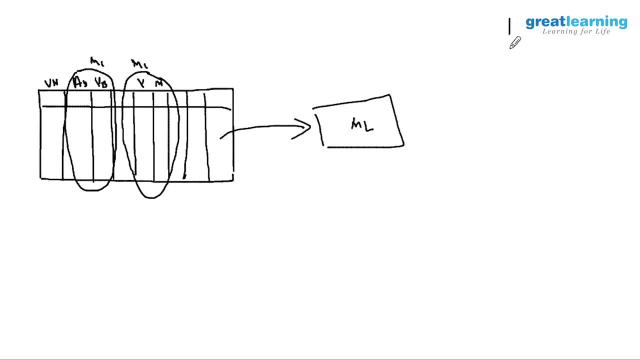 Yeah. So what's going to happen is it is like, let us say, we are a group of five people right now, for example, So when I am talking, let us say I'm explaining you PCA, Parallelly, there is one more guy who is explaining PCA. 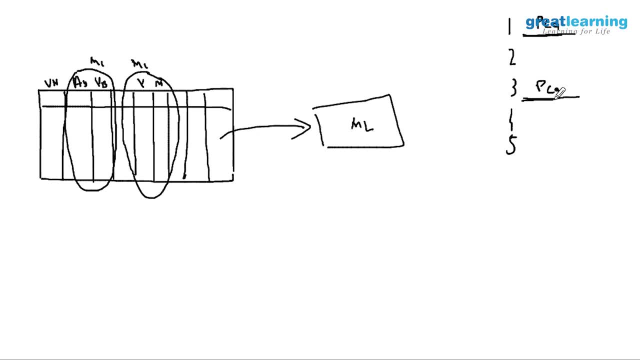 So you are taking my concept also and he's also explaining similar to this, but not exactly similar, but almost similar to this. So what will happen? There will be a lot of noise for these three guys. whom to listen to, whether to listen to this concept or listen to this concept. even though the concept is same, thing happens here. 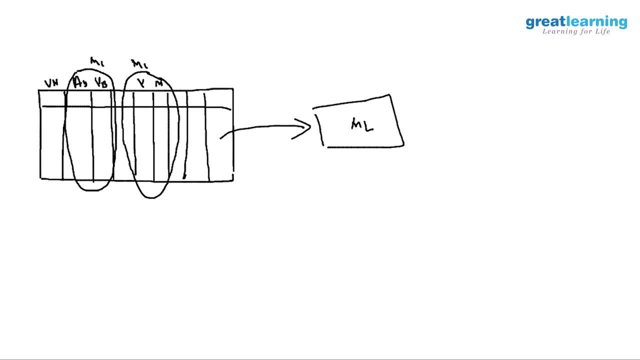 when two columns are perfectly or almost similar. at that point of time, machine learning back-end algorithms will have some unwanted noise because they are almost similar. So in that case, why these guys are pushing right? they pushed you for first four projects to do all these things- is they wanted you to understand that? don't blindly take any data set. 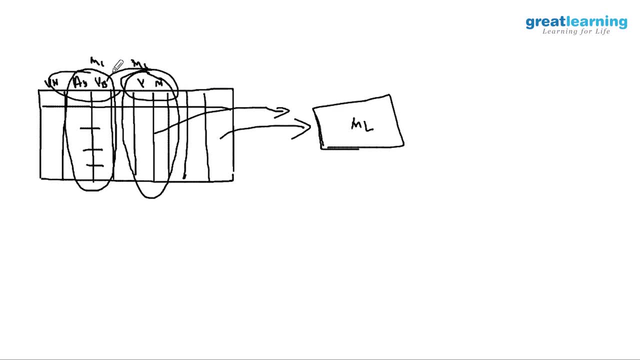 and put into a try to understand these kind of nitty-gritties and try to remove some columns on your own or try to enhance certain columns. So again, let us say, if all of your data is in three-digit and one of the column is 0.000. 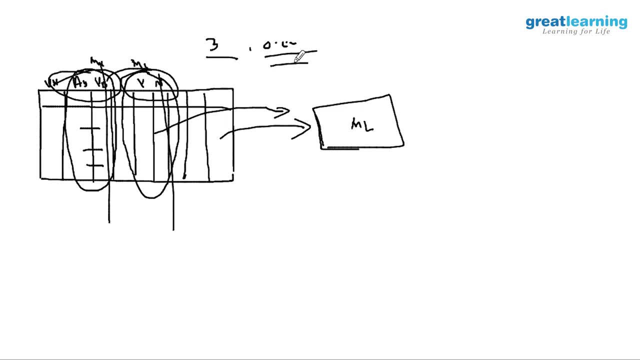 in this kind of decimal point again. it's not that so we are supposed to upscale this fellow. Otherwise, what will happen in inter? you know, collinearity or covariance kind of thing, This and this will have a very local, even though in its own world. 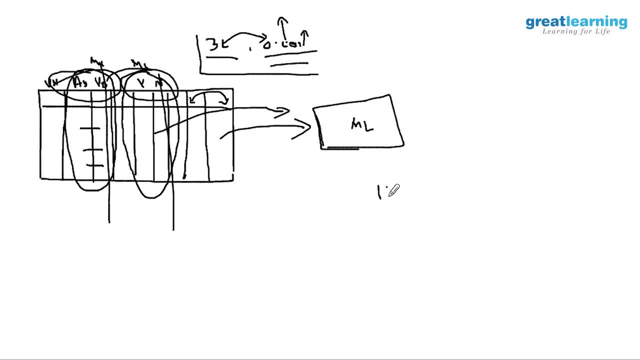 This will be a very good number. So it's like I can say 1 kg of rice, 1 kg of saffron, Or else I will say how much rice I will get in thousand rupees and how much saffron I will. 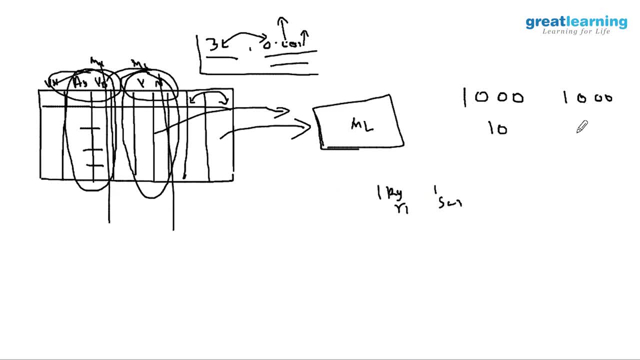 get in thousand rupees. So this will be, let us say, 10 kgs, and this could be 0.01 grams, For example, even though it's very important, but python will not get it that the scale is less, but it's very important. 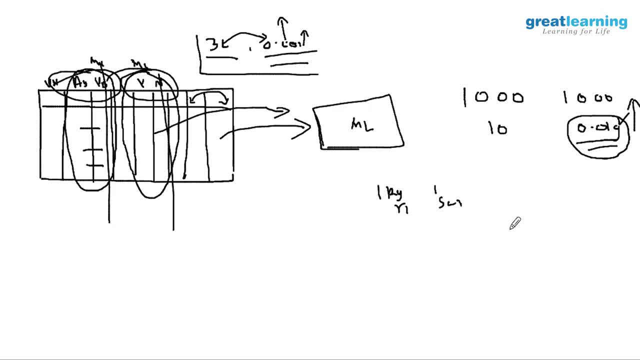 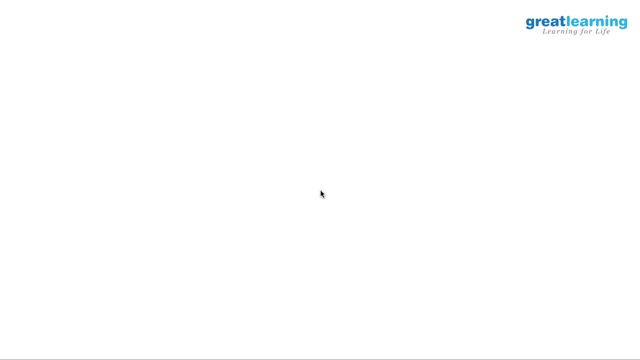 So in that case, we are supposed to scale it up. So this is what they were trying to make you do, Yeah, Yeah. So that is the reason why, initially, these projects were focusing on, on, on to cleaning the data or understanding the data. univariate analysis, multivariate analysis. 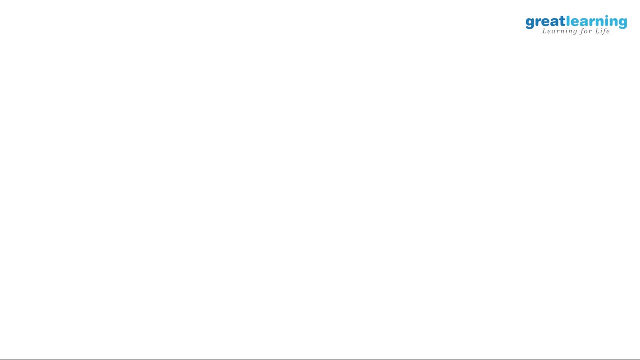 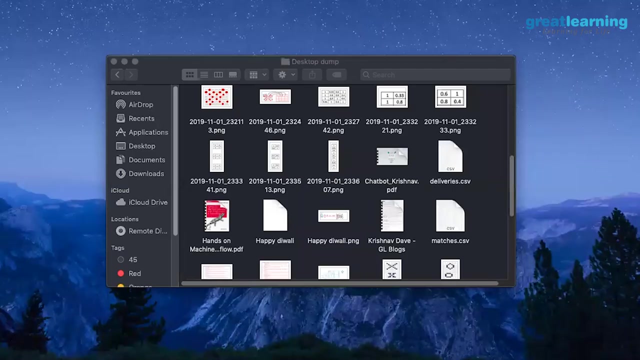 Why did we do multivariate analysis? To understand how one feature is related to another feature and if you feel they are perfectly similar, ignore one of them. Correct, Yeah, So this is what is a little important. But again I will say I be like nobody can say okay. 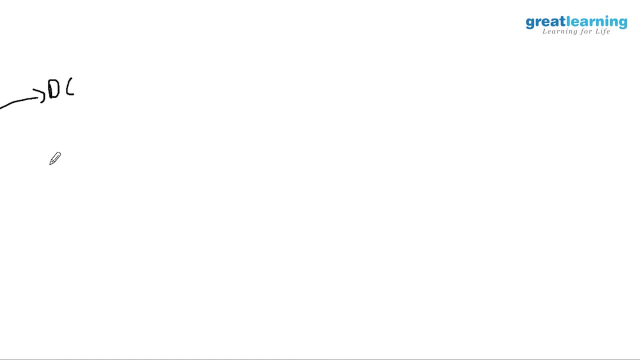 We are perfect in data cleaning. Everybody goes through the similar process. Some of us find out the problem, Some of us we ignore the problem. Now you may ask: Okay, What if I ignore this problem? What if I am not able? because? see, imagine in real industry. let us say you have 1 lakh. 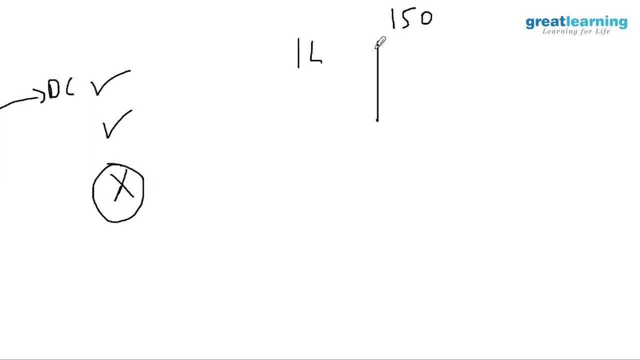 rows And 150 columns. It is not possible for us to go through, understand everything, that sometimes we might miss certain problem stuff. So it's okay. So what we can do is, if we are the our data is having a loss, We are putting into our machine learning. 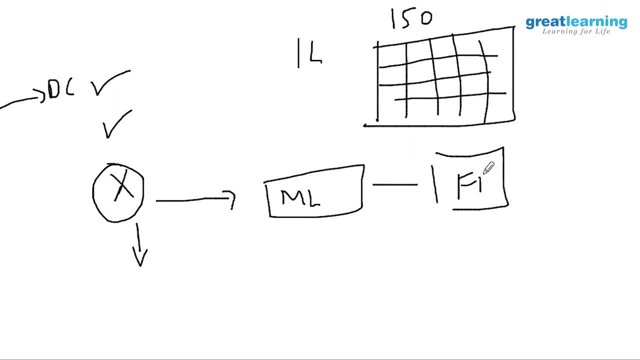 Okay, post machine learning will do something called feature engineering, where we'll try to cover up for this loss, How I will show you. but if we are losing something, Don't worry, at the end We are having some extra features to even improvise on it. 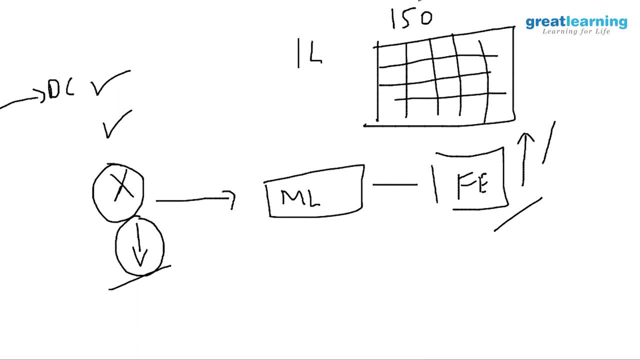 Why? why? why I'm saying it's okay is because, anyway, at the end of the day, it's a human who's designing this model for a human to process this in certain amount of time. It might not be that accurate. We might also lose or we might also do a wrong assumption. 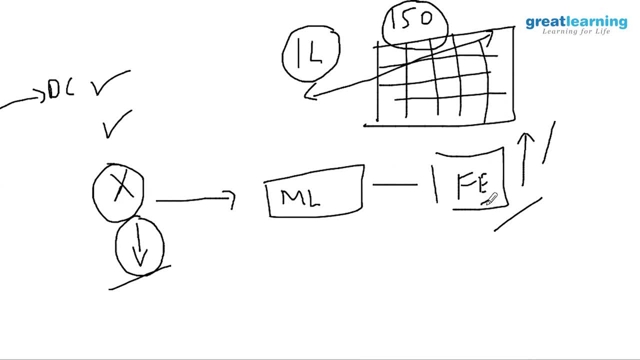 It's possible, We don't know. Yeah, so that's where we'll bring in an extra booster over here to improvise our activities, whichever we have lost because of this. Okay, perfect. Now I'll give you one more example. 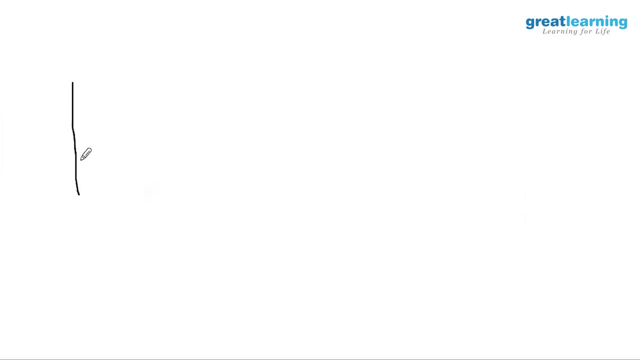 What do I mean by multi-collinearity and all those things? So let us say we are doing linear regression, The easiest algorithm. So I will say this is my independent data set And this is my target value, Okay, and say this is my monthly salary. 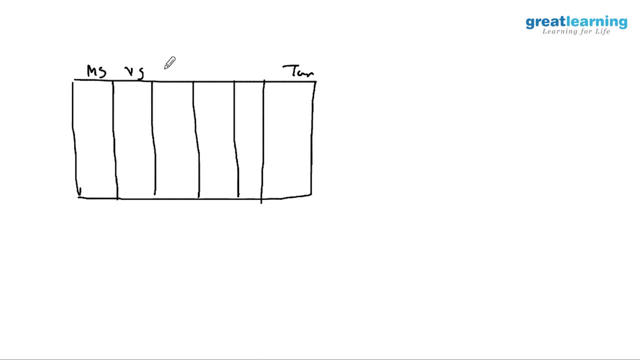 This is my yearly salary, This is my gender, for example, This is my marital status and this is the loan amount that I have taken. So my target will be how much I will default something that let's, let's say we are doing linear regression onto that. 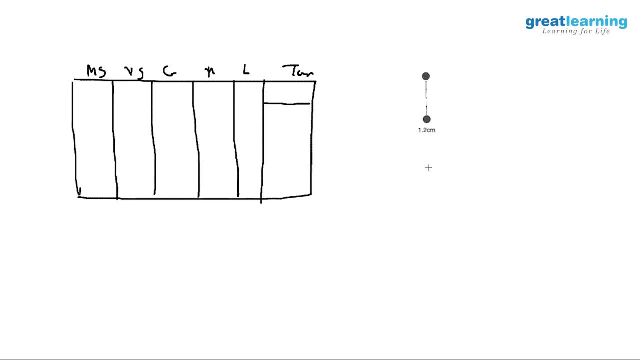 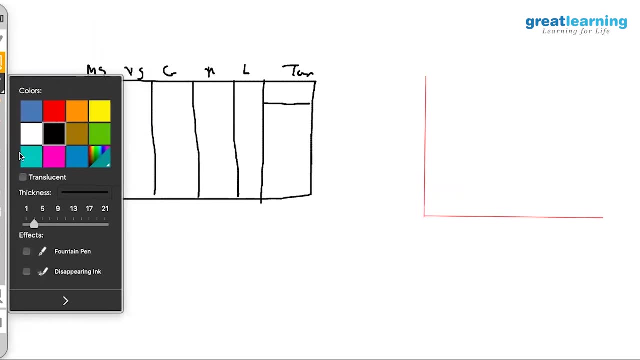 Now what is going to happen is when you plot. if you remember the linear regression plot place, do you have? I shown you this? anytime, my way of linear regression, No right might be no. Okay, Let's say this is what we have got. 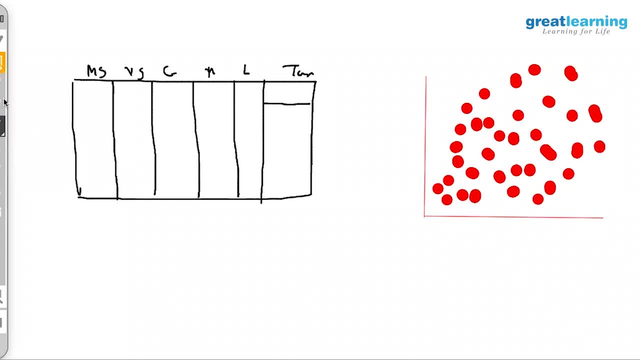 Okay, Now what majority of people will do is they will not check for linearity. First of all, as we say, linear regression, the first thing we are supposed to check is for linearity. is the data linear or not? If I look at this data from industry point of view, I will approve it. 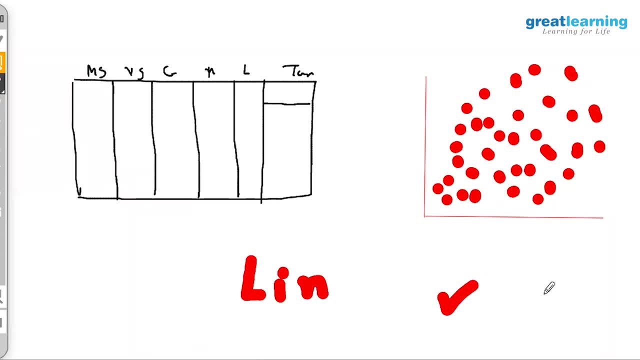 It's a linear data, but from our academics perspective we will say it's not a linear data at all because it's going in the circle. It's not perfectly linear. Now, there might be many reasons why it might not be perfectly linear. 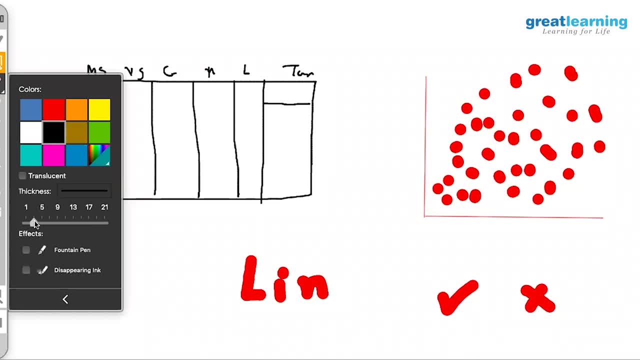 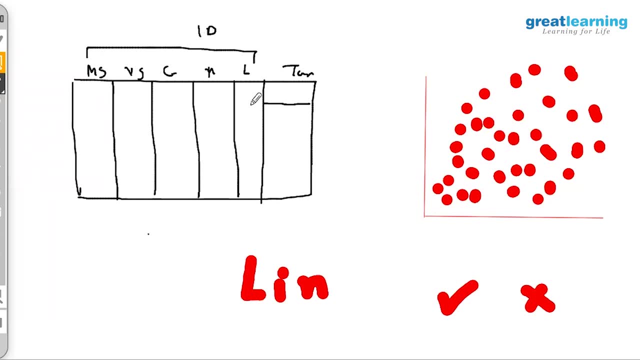 The first reason, if you observe here, is there is multicollinearity present. Now, what have we given name to these things? independent, variable, right? Are they actually independent of each other? Look at these two: monthly salary and yearly salary. Can I say they are highly dependent. 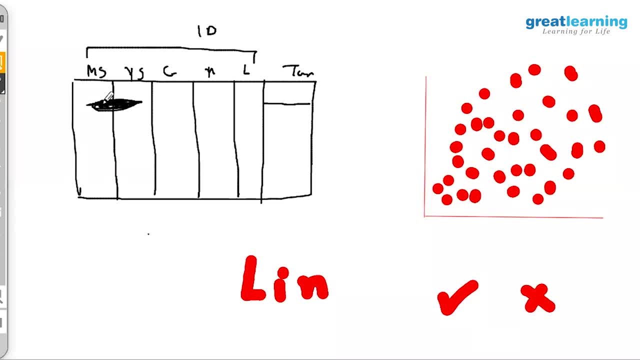 Not independent, right? They are highly dependent on each other, Correct? So in this case, I can say that one of These columns might be a reason of these kind of scatters that we see. Okay, so when we check for linear regression, the first check should be your independence or linearity. 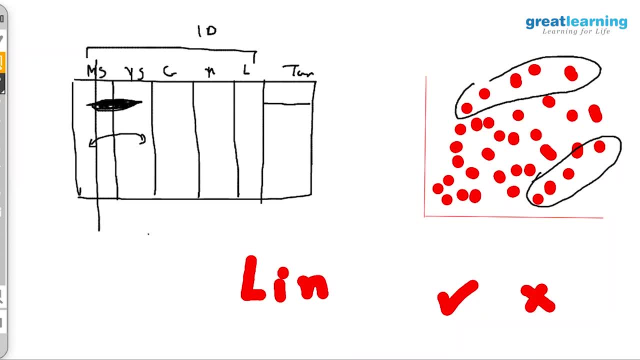 So when you do this, we understand it, We remove it. Definitely. The new linear regression graph we get will be much better. Now again, I will say: we will get answer even if you use our older data set. Even if you would have used both of these columns, you would have got a linear regression answer. 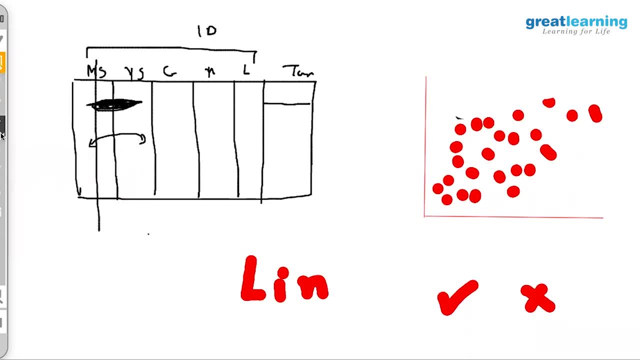 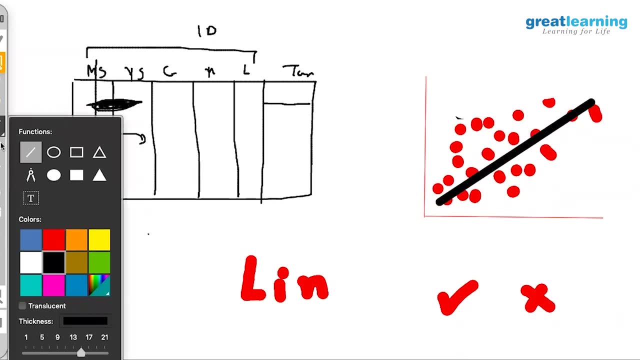 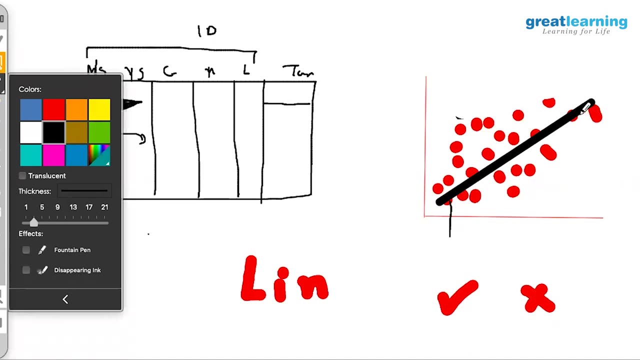 Definitely. But what would have happened if you people remember that line, you remember the virtual line the mentor would have shown you in your sessions? Yeah, Yeah, Yeah, this particular line is what. this particular line is very simple: If you take the lowest point on the line and if you take the highest point on the line, let us say this is called variance captured by the line. 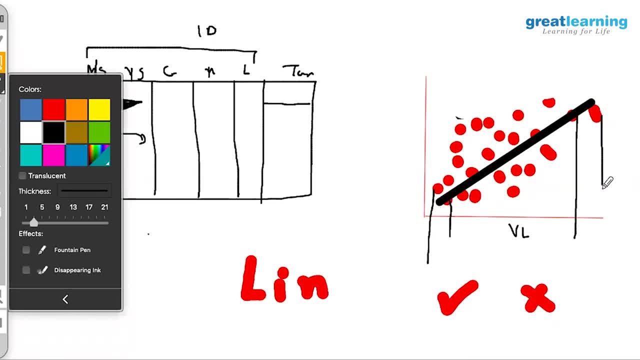 If you take the lowest point on the whole data set and if you take the highest point on the whole data set, this is called variance captured by data set. Correct Now, variance captured by line is equal to some X value into variance captured by data set. 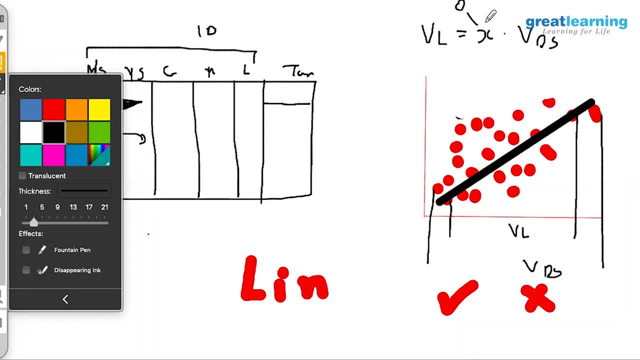 Do people agree with that? Sure, This X can be between 0 and 1, correct? If it is perfectly 1, I can say linear regression. So data variance captured by the line and data set is perfectly same. If it is 0, I can say nothing. 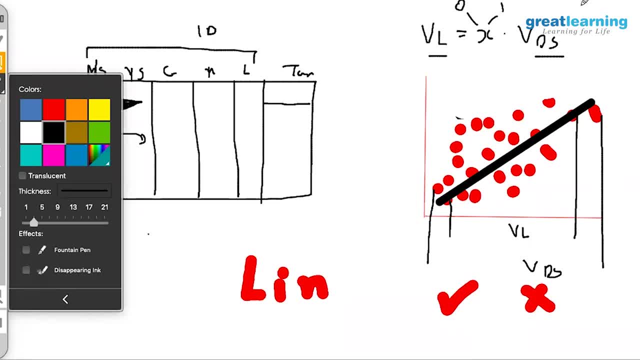 But if it is in one of these middle, that means let us save. the value of X is 0.8.. That means 80% of the variance of the whole data set is captured by the line. Do people agree with that statement? 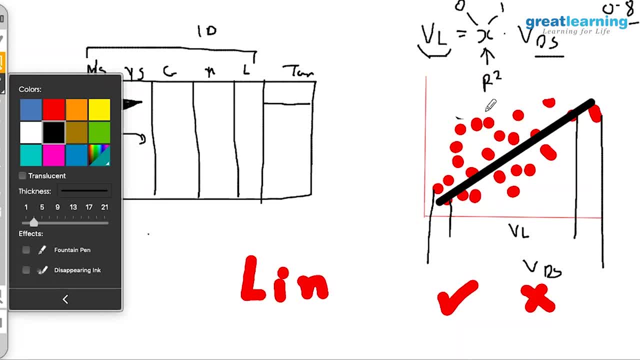 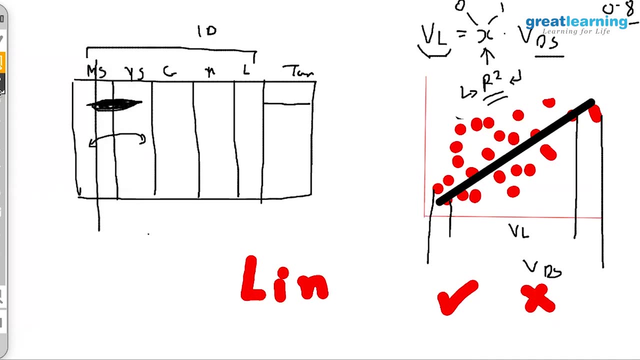 Yeah, Yeah, What is this? This is R squared. You remember R squared In linear regression? the accuracy check. Yeah, Yeah, this is your R squared value. We don't know the exact meaning of that. Yeah, we heard about that. 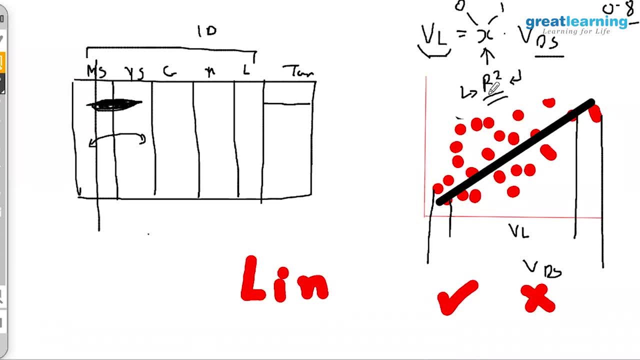 We know that. Yes, So this is your R squared value. R squared is nothing, but how much variance. See, basically, what are we doing? We are putting a virtual line. So this is all virtual world. Now we want to understand that, if in case, tomorrow I am representing this line. 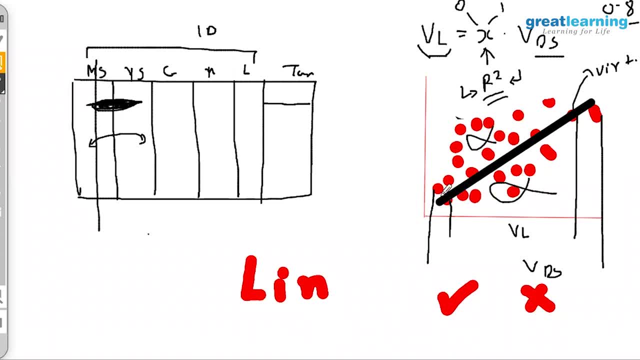 By the data set. I'm saying I'll remove the whole data set. I don't want the data set. I am just saying the whole data set is equivalent to a line. First of all, is it correct? Visually, I will say not at all correct. 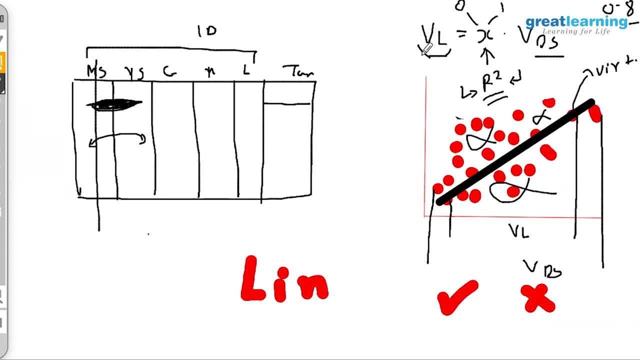 How can a line represent the whole data? That's where we are saying that Information means variance in data science. Please remember that Variance or standard deviation is nothing but your information. So if I can prove somehow that the line that I'm plotting captures 80% of the information or variance of the whole data set, 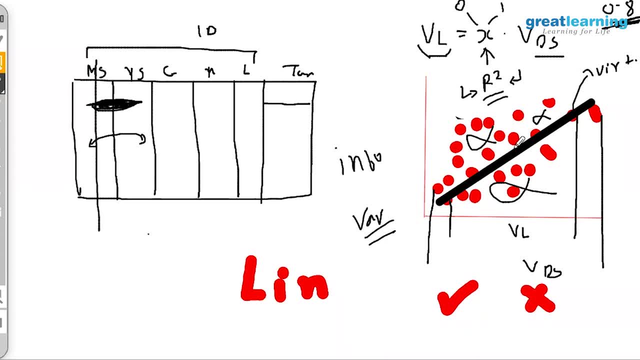 Then we can say that, yes, a line is possible to represent a data set. Correct, What is this line? Y is equal to MX plus C. We did it in school days, guys, if you remember. Yeah, this is your linear regression equation. 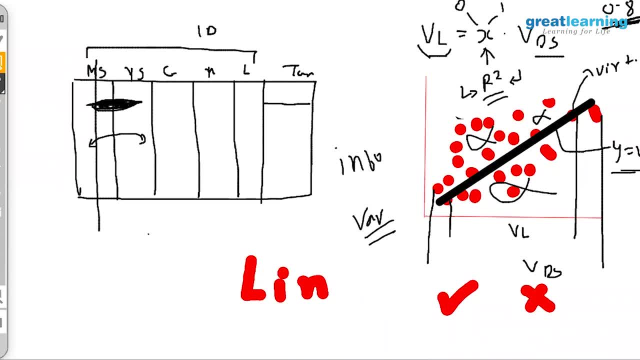 Confused. So why did I show you? Why did I show you guys? this was if in case we did not clean this. No, if in case we did not understand this problem and we wouldn't have cleaned it, our R squared would have come down. 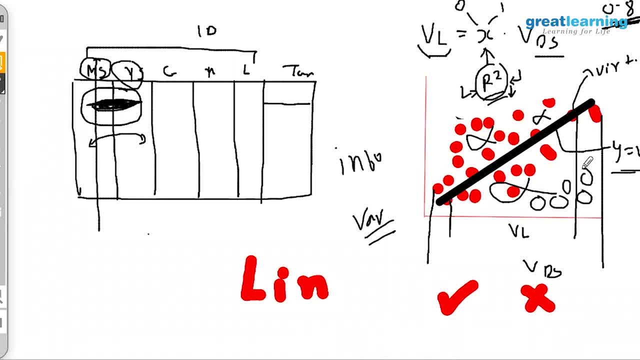 Why, if you remember, we had got some extra points here. That's true, That is going to increase the error. This is nothing But the error: error between the actual point and our plotted line. the distance is called error. So if we don't take care of this, error is going to increase. and if error increases, my R squared is going to decrease. 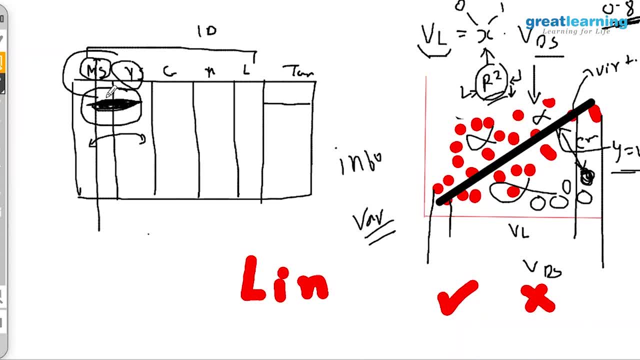 That's it. That is the reason we say that before starting any algorithm, please go through some of the data. It might help us to improvise. I will not say: if we don't do this will not get the algorithm. algorithm will work. 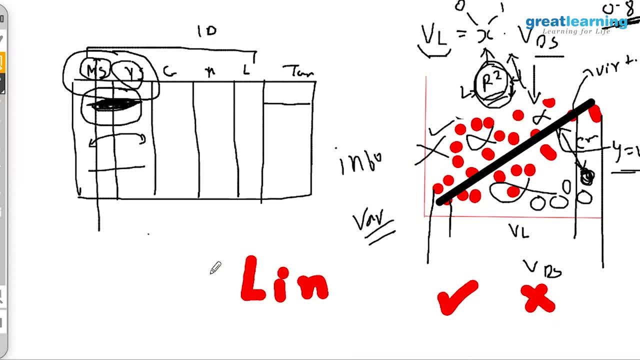 Anyway, the only thing is accuracy will be a problem. That's the reason we drop some of the columns, Exactly, Exactly. So if, if, in case, I found out multicolinearity, and if I drop the extra points, and definitely I am going to reduce that error. 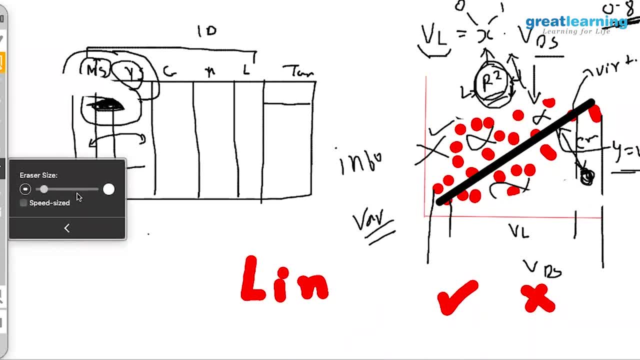 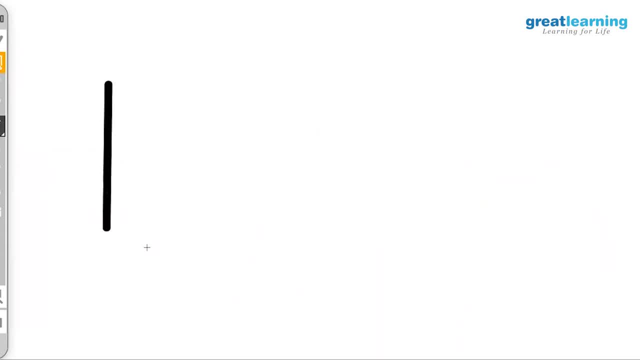 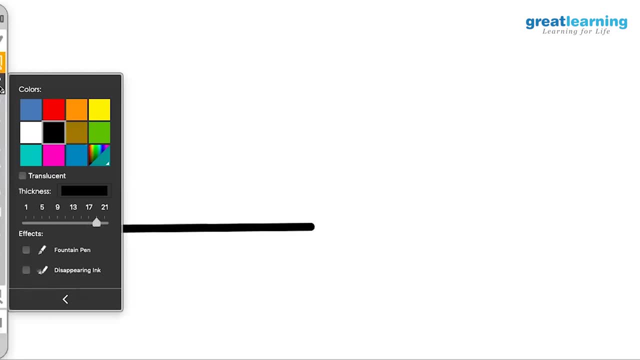 Okay, one more thing then, since we have touched this. if I don't show you, this will be unfair, So give me one minute, Because this linear regression I take it very seriously. This is the first algorithm that we learn, So People are supposed to know the in and out of linear regression at least. 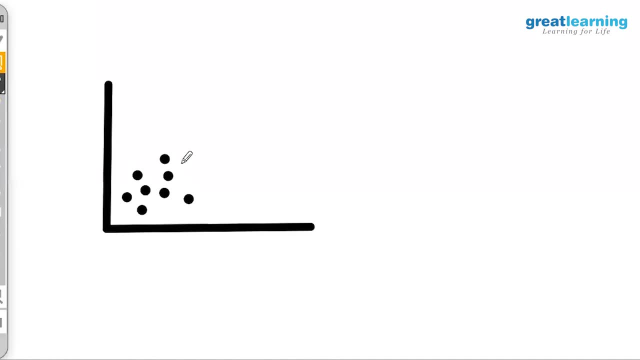 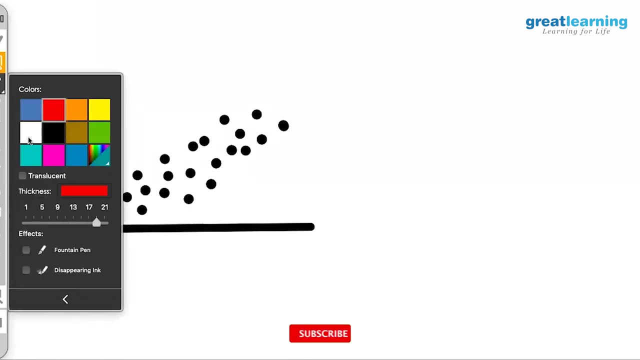 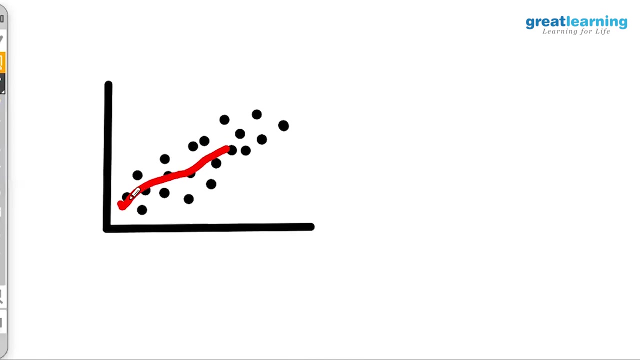 So let us say this is my data set. Now, as I told you guys, The line rotates. I don't know whether have you heard this topic or not, but please remember one thing: the line rotates. I'm sorry, Please ignore this. Yeah, what is happening is the line will rotate this side, or line will rotate this side. 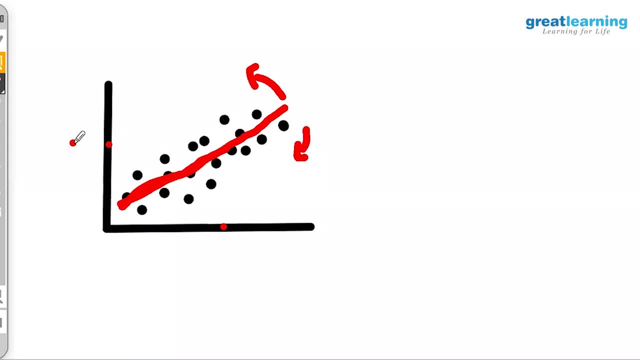 How Find the center point of this? find a center point of this extended. This will be the center using which line is going to virtually rotate. So if I plot this line like this, it is going to rotate around this axis, Now a place where line comes to rest. 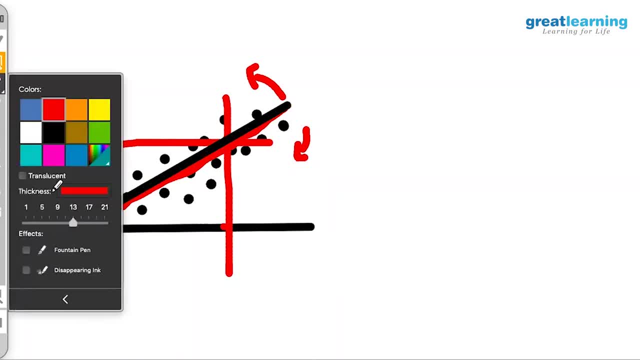 Let us say this is the place where the line comes to it. What does it mean is it has found the maximum R squared value. So, out of all the R squared value when the line was rotating, that means V. L is equal to X into V. 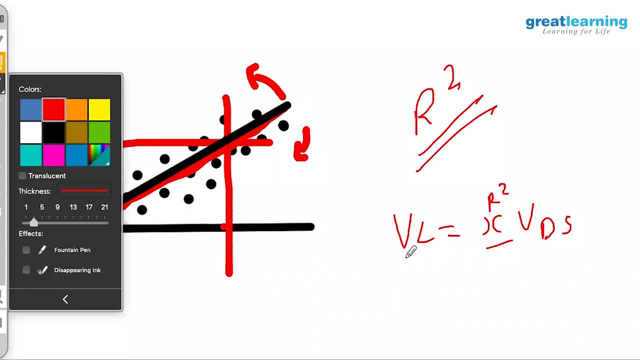 D is that we just saw. X is nothing but R squared. So we would have rotated our line many times and we would have calculated these values many times. right, The best value that we get. that is where the line comes and sits on the data set. 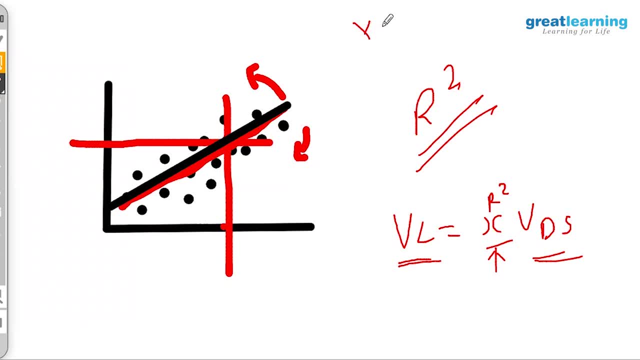 Yeah, Now, theoretically, the equation goes like this: Y is equal to MX plus C. For linear regression, I will come down to your original equation, But for now, imagine this is the equation of linear regression. Now what is M? the slope of the line? 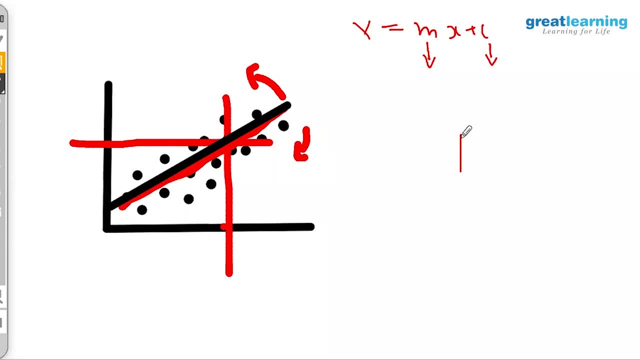 What is C? One constant. So what if my machine learning Dabba that I usually talk about, we learn something right? What are we learning? We are learning M and we are learning C here. Agreed guys? Yeah, Now, depending on the value of X, 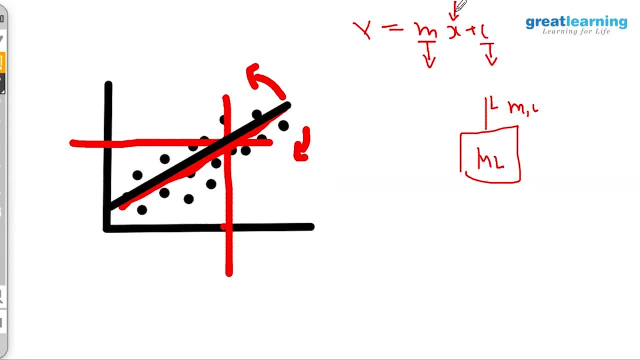 So I have already learned M. I have already learned C. Now, in future, when I change my value of X, what is going to happen? We are going to get a predicted value of Y. This is how linear regression works out, Okay. 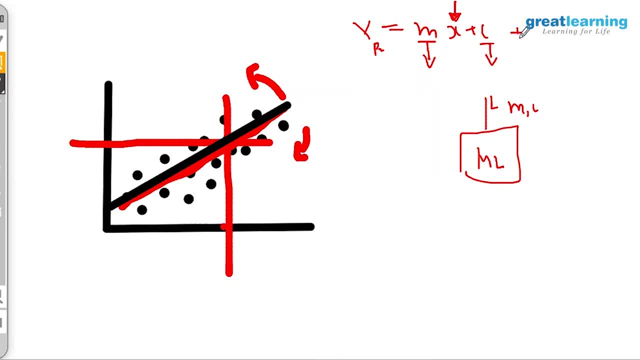 Now, keeping this in mind, We have forgotten One extra term in linear regression, which is called mean square error or residual error, or whatever error you call. So let us say we call it residual error, RSE. Now, if I don't want to confuse you guys, but this is the equation you would have seen in your sessions. 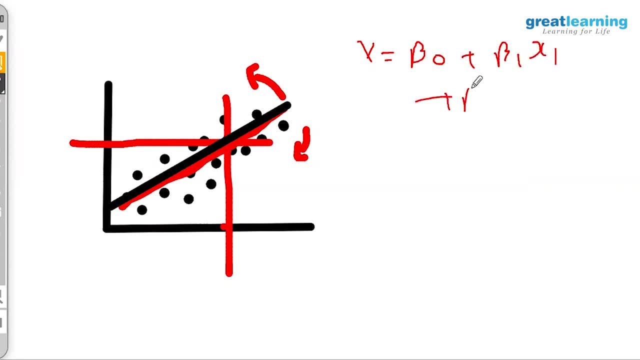 Beta naught plus beta 1 X 1, plus beta 2 X 2, plus residual sum of errors. Correct, This is the equation You will be familiar with now. What is this equation? This equation is nothing but Y is equal to. 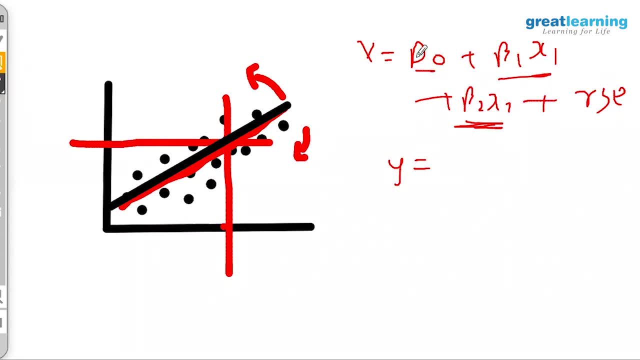 MX plus C. That's it. C could be a combination of beta naught plus RSE- We don't know, but the same our school equation can be transformed into this. Now, what is RSE? RSE is, RSE is nothing, but you take the sum of an error. 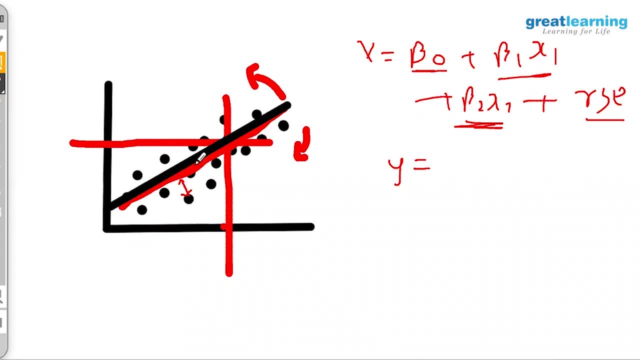 This is an error. See, some of the points will lie on the line. They are not error, but some of the points are far away from the line agreed. So the distance between them you compute and if you observe, this distance and this distance are going to counter each other. 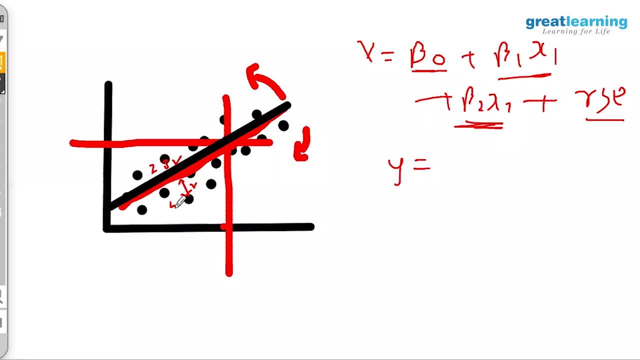 Do you people agree? Let us say this distance is 2 and this distance is 4.. 4 minus 2.. They are going to counter and we are going to end up with a distance called 2.. So what do we do? 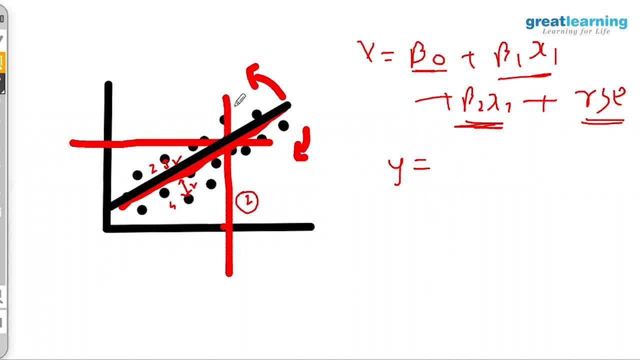 This is, we are trying to plot a line with symmetric points on both the sides. So when we have symmetric points, what is going to happen? RSE is going to come down to 0.. Do you people agree? Let us say one point is here which is a distance of 4 and one point is here which is at a distance of 3.9.. 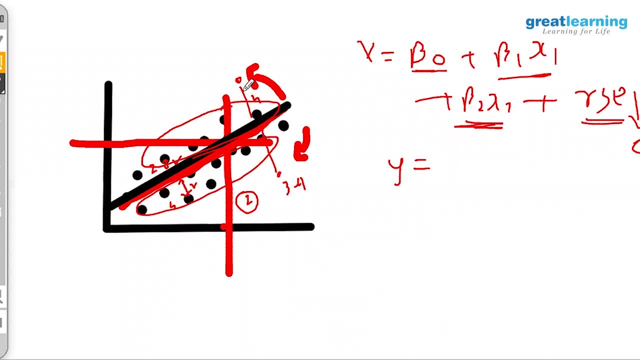 So when you add or when you calculate the distance between this to this and this to this, they are going to counter each other and the residual sum of error is going to come down to 0. And this is our aim. So if we don't remove multicolinearity, RSE is going to increase, and if this increases, our predictability will go also high. 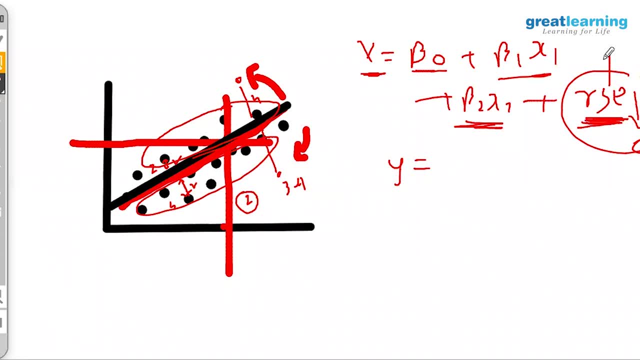 Why? Because it is a part of equation. So if this is more, this will also be more. If this is more R square is going to also to be less predictability. We go down. This is the relation. that is the reason we are supposed to do the cleaning part of it. 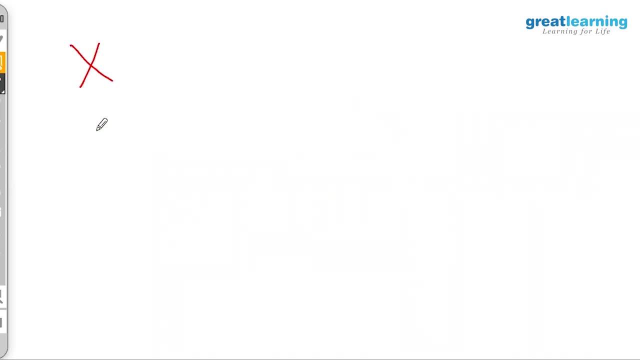 Okay, Now what if we have missed it? What if we guys missed it? Then what we could do, Let us say linear regression. We missed understanding this multicolinearity, part of it. So what we could do now, Any idea? 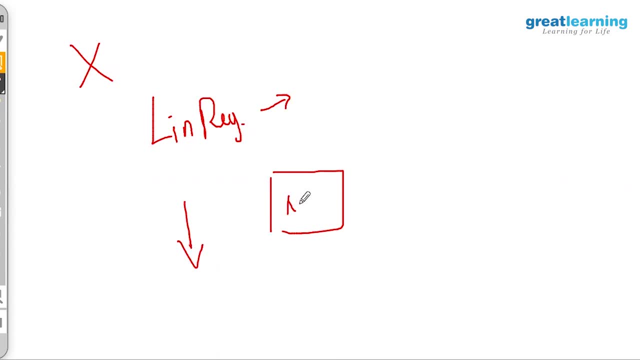 See, I told you guys That if we are losing something before machine learning, then there is something coming at the backside We could improvise on to that. Yeah, feature engineering definitely will be. So how do we use feature engineering here? 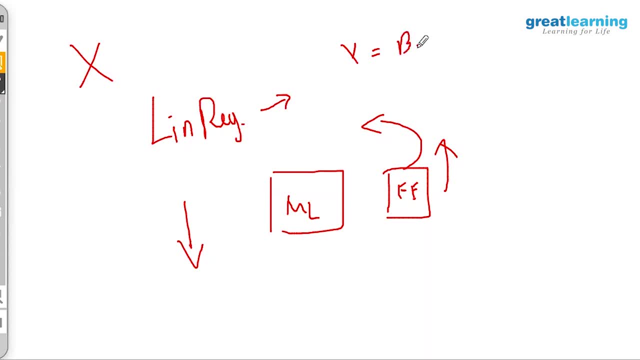 What see we have? We have an equation like this: Y is equal to beta naught plus beta 1 X 1 plus beta 2 X 2 plus RSE. Now we are supposed to do feature engineering here. We cannot do any. 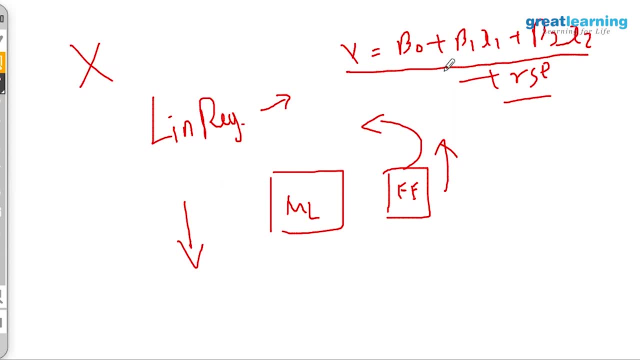 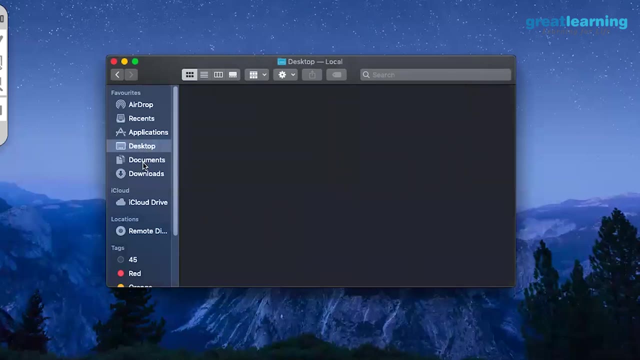 Magic. We are just supposed to alter the stuff. So what we'll do, Any idea? Okay, just give me a minute, I'll pull up my guys. If you remember, I've shared with you my linear regression Excel file. You remember that. 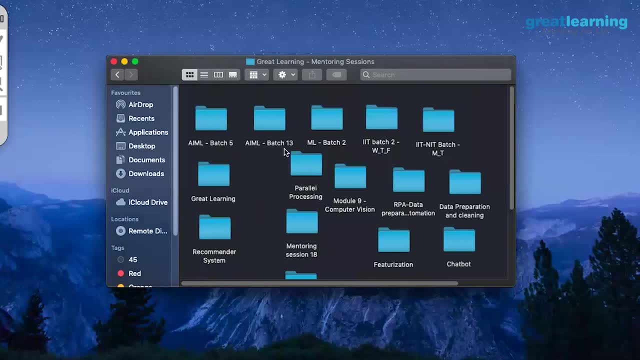 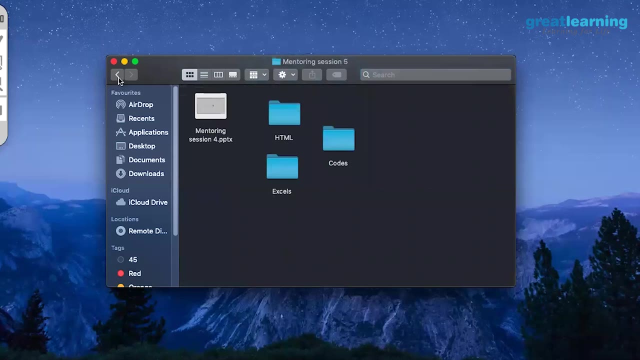 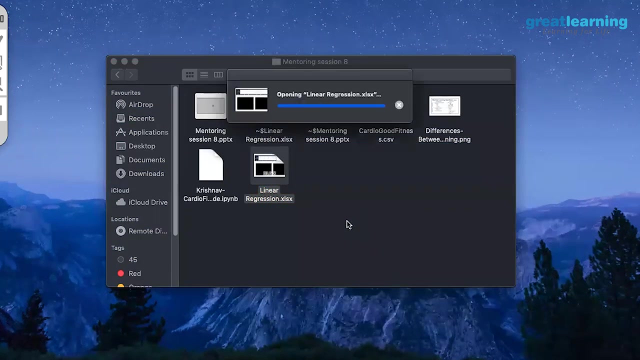 Yeah, Yeah. So where is it? Batch 2? Session number 5? No, 6?? No, I think it'd been 7 or 8.. Yes, yes, here it is Open with numbers. Okay, so, if you remember. 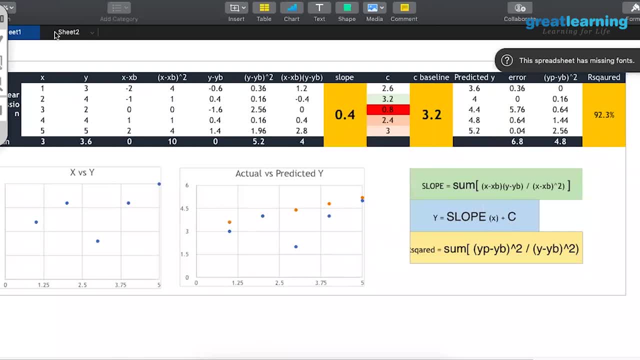 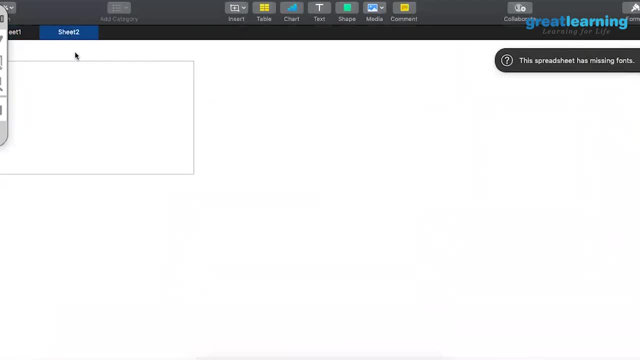 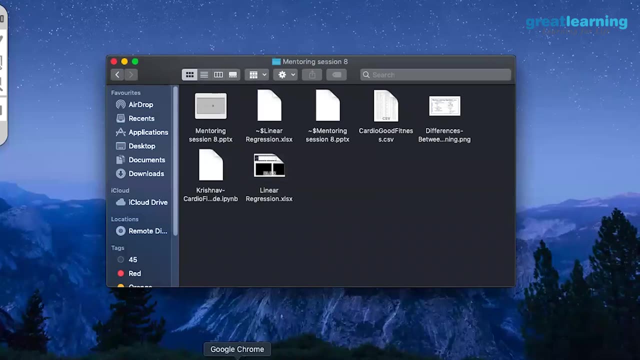 shared this files with you guys. Now what if I would have missed out? It is not working proper in numbers. I'm supposed to have an extra sheet here. Okay, No problem, I'll explain you. I don't have currently Excel on my system, I just formatted it. So I'll explain you this. 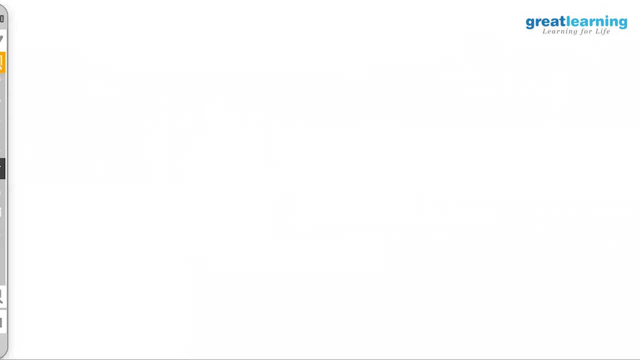 way Did your mentor teach you about P value in a linear regression? Yeah, Yeah, So do you remember each column? So let us say these are independent features that you are using. Let us say we are using one, two, three and four features and one target variable. So did he? 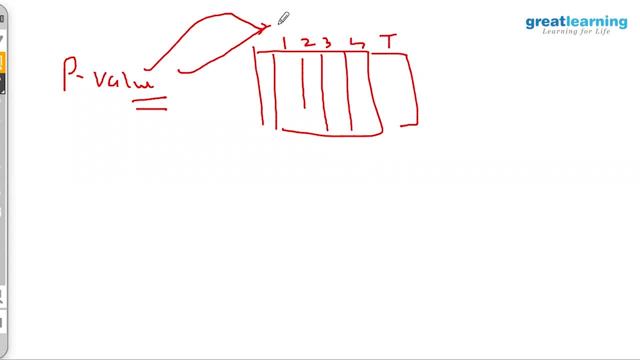 teach you about how we can choose this features depending on P value. No, right, Yes or no? Okay, What is P value now? So, for example, what do you mean by P value? Do we know this, right? Okay, No problem, See, just observe here. Let us say I have got a data set, a normal curve. 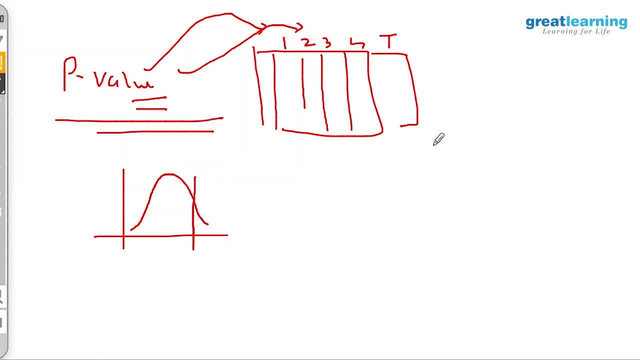 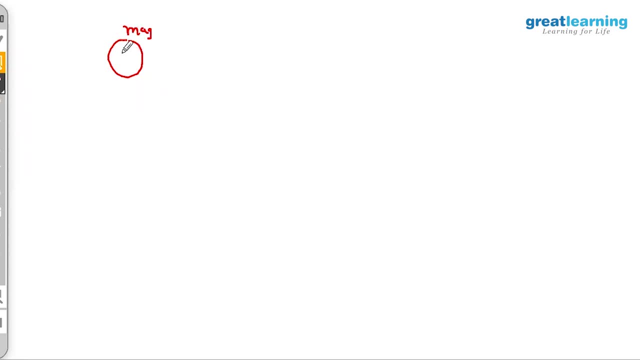 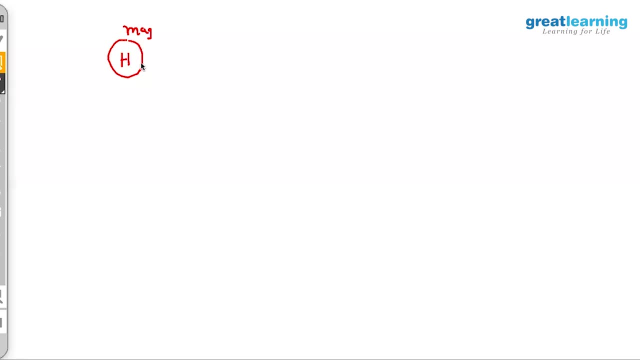 interpret it. it's very difficult. so have I explained this example earlier to you guys. no right, okay, no problem, just just observe here. from now your P value concept will be very clear. so you will also understand way to use P value. see, let us say I have got a coin. I call it as a magical coin. now you guys will say: 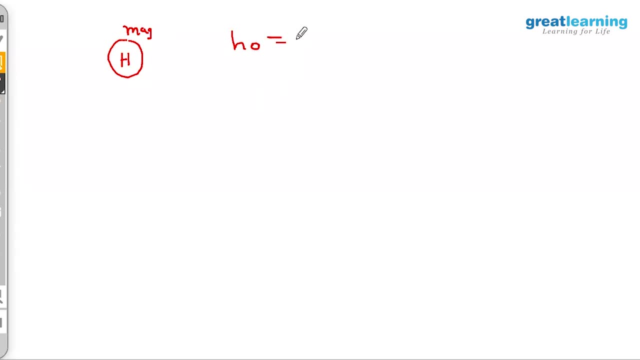 as per my hypothesis. I am saying this is a magical coin, okay, and you guys are saying it is not possible that if you toss this thousand times, every time you are going to get a total heads. it's not possible. so you will say: not magical. now how do we take a? 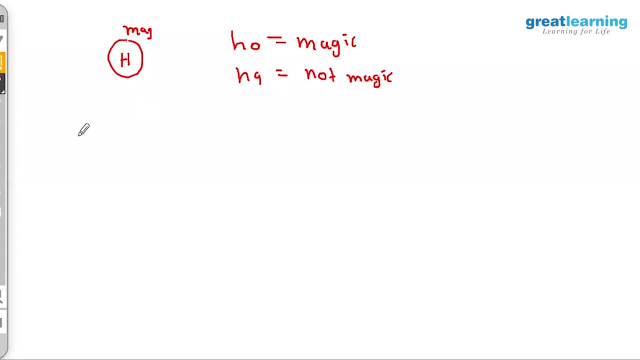 decision on this? do we use a primitive method that every time I want to, you know, debate, I will do thousand tosses. is it? is it practical enough to do it? not practical enough? right, and also not smart enough, yeah. so how do we decide whether this is magical or not magical? for that reason, 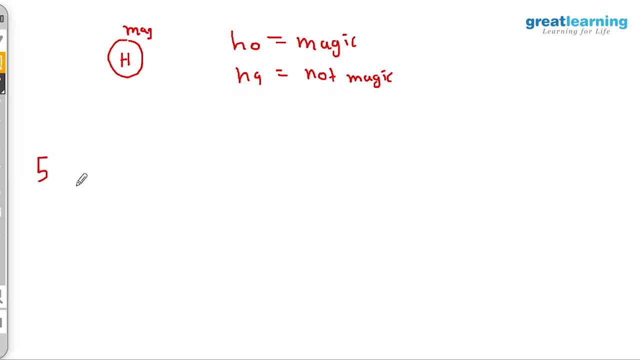 what you do is you say we'll do a five trial run. so let us say I toss my coin for the first time, what is the probability with which i will get heads? can somebody tell me, when i toss my coin for the first time, what will be the probability of getting heads? 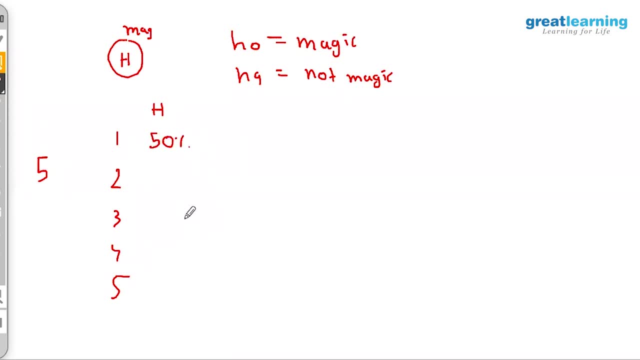 0.5, so 50. can i say yeah? now, when i toss my coin for the second time, what will be the probability that i will get heads for second time? no, no, think about it. i am talking about two consecutive times. we are talking about multiplicative probability, so whenever you want an event occurring twice, 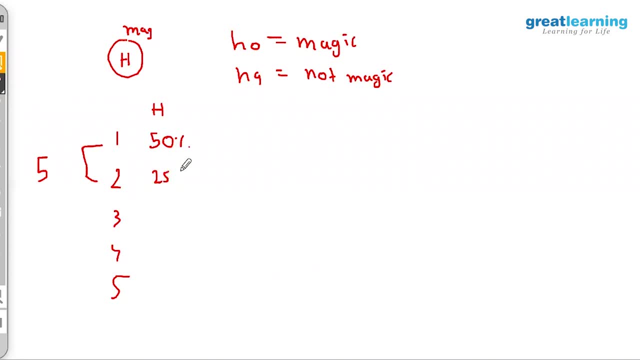 you have to divide the probability of above by 2, that is 25. 50 into 50. yeah, exactly, 0.5 into 0.5. exactly what is a probability three times in a row? i can say 12.25- correct. four times in a row: 6.125. five times in a. 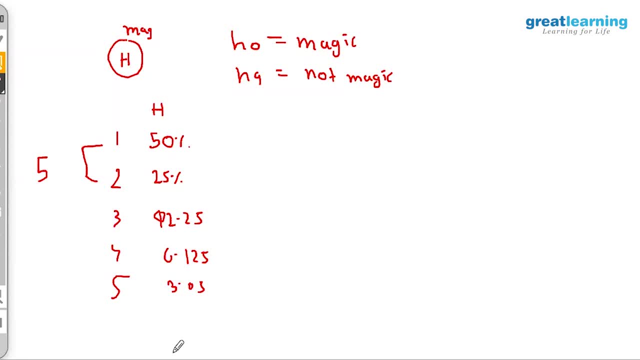 row 3.05. we can go on like this, but there is no fun. let's be smart enough. from this five you will be able to find out which one is correct. now, as per the rule of p value, what does p value rule say is very simple. let us say this is a probability distribution graph. i am going to have a barrier. 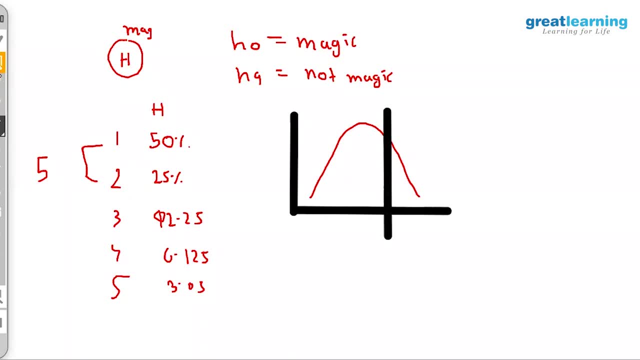 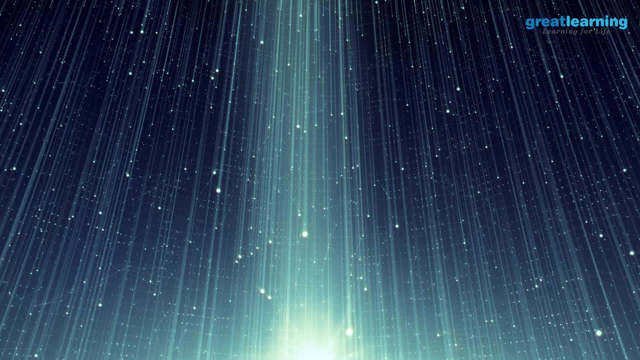 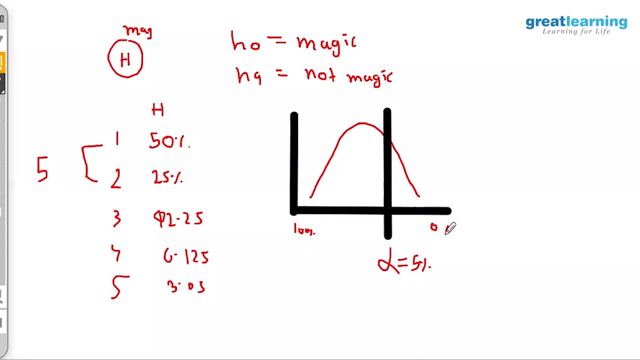 i will decide a barrier. that is what you people told critical value, alpha value. usually in industry we put it five percent. okay, now, if this is hundred percent probability, please remember this is not zero. if it is hundred percent probability and if this is zero percent probability, i will say that any of my answer. 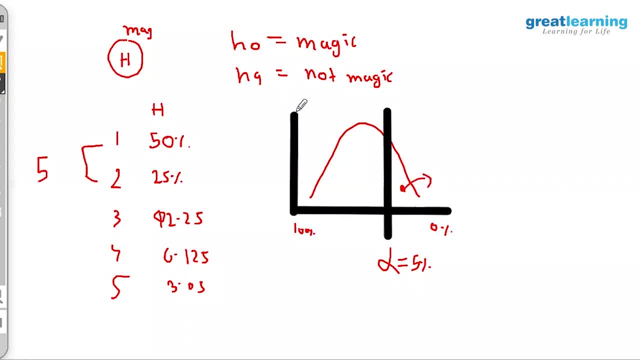 which lies in this area. i have to accept ha, alternate hypothesis. yeah, okay, why? because the probability with which we are claiming is pretty low. okay, and if my coin or my answer falls in this probability zone, i will accept h zero. clear. now. what is my p value? the final, 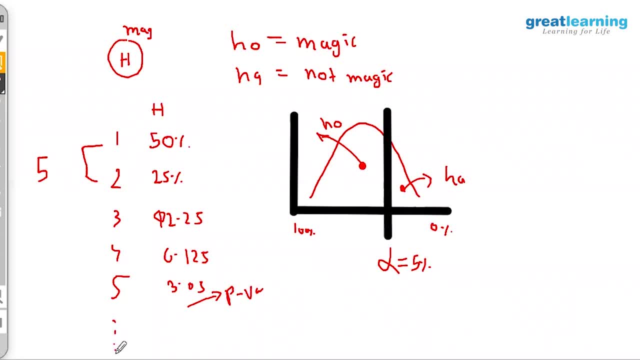 probability value will be your p value. if i would have gone till 10, then whatever answer i would have got would be zero. so i will accept h zero. so i will accept h zero. so i will accept h zero at 10 will be my p value. but since i'm going with five, this is my p value. agreed. what is my p value? 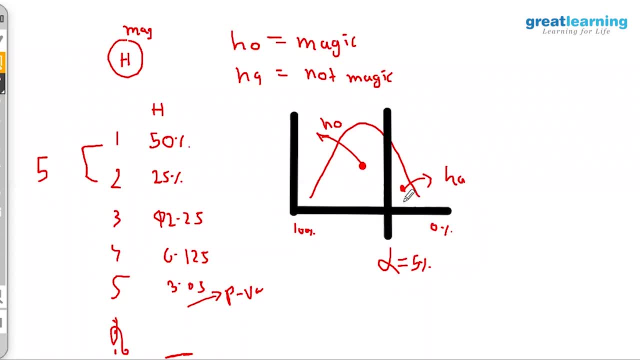 three percent. where it? where is it going to lie? can i say in this zone, yes. so, logically, what are we doing? we are saying that, statistically or logically, the claim that you are making is not right. why? because the probability with which we are saying that five times in a row heads will. 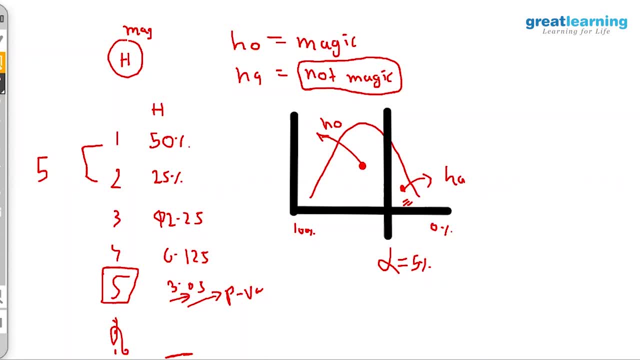 happen is just three percent. i hope you got the p value now. the probability or the confidence with which we are saying that heads will come five consecutive times without any break is just three percent. okay, that's the reason we will say it is not magical. see, sometimes there is possibility when he's checking it. 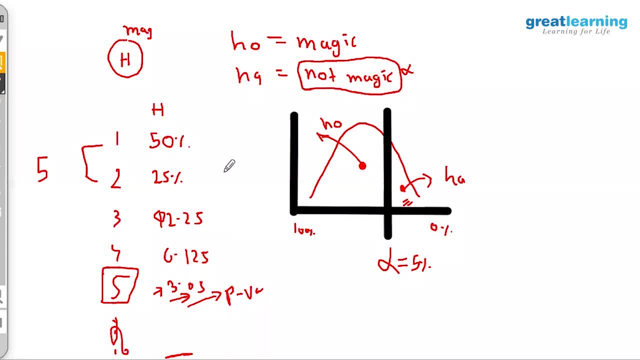 randomly. you know he might get five times. that is a extra, you know, exceptional case, but theoretically it is not possible at all. so i hope you got the p value now. the probability, or the confidence, with all the probability, is very low. okay, now keep this idea in mind. i will show you how to improvise. 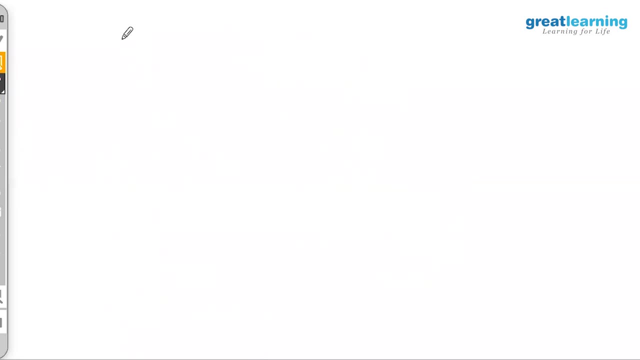 p value onto linear regression. now, did you people observe the linear regression output? one of the parameters were p value. did you, do you remember that? okay, if not, i will try to show you next time i load up my excel file and i will show you see, what happens is. we will make a probability distribution graph of what 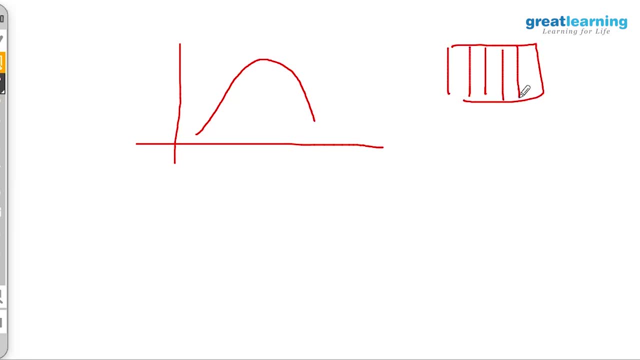 of our independent variables impacting target variables. so let us say independent variable one, two, three and four. i want to understand that. what is how one is impacting p? with what probability percentage i can say that variable one is having a high impact on p? got it the business problem. 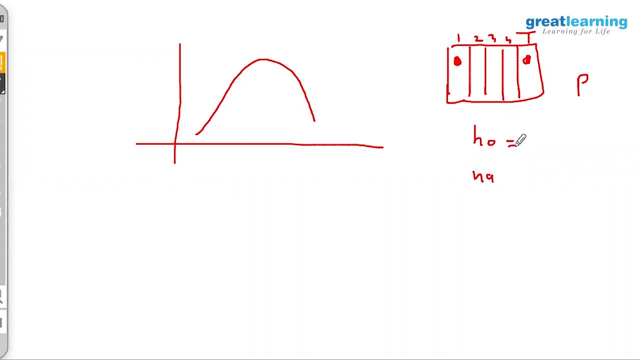 so i will write my hypothesis saying that there is no, no impact of one on t and h a will be. there is a high impact of variable one on t. okay, so when you generate your so what if we would have missed that? as i said, there might be multicolinearity and we would have missed it. yeah, in that case, 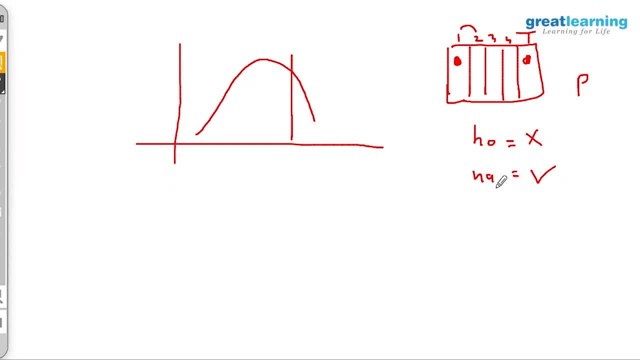 what we can do is we can get a p value. the linear regression output itself will have a p value. so let us say, the p value for variable number one came out to be 2.5 percent, for example. yeah, in that case, this is your alpha, this is your hundred alpha is five percent. this is your zero. 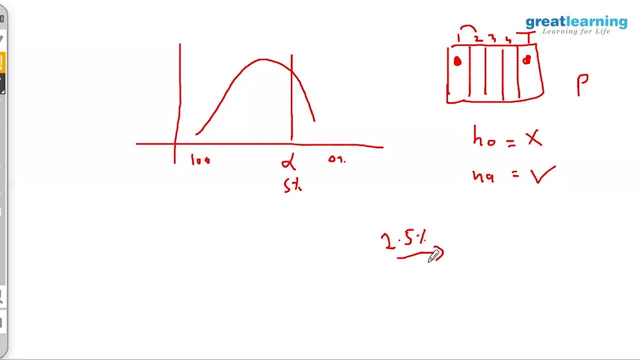 percent. so where it is going to lie, my p value is 2.5 probability. the confidence or probability with which i can say that one impacts t is just 2.5 percent. yeah, so in this case we will say h, a is accepted. so i will say, yes, the probability is low, but still it is in acceptable zone. why? because we 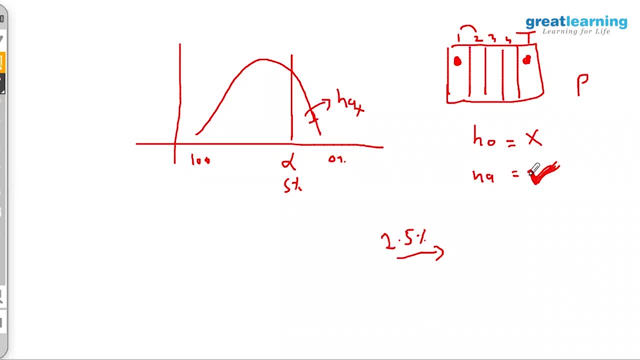 are getting h in h a. we are defining that, yes, there is a impact. yeah, but what if i would have got a probability of 30 percent? now, where will my answer lie? can i say my answer will lie in this zone. now, guys got it. what is this zone? h zero zone. so now i can say that i can clearly using 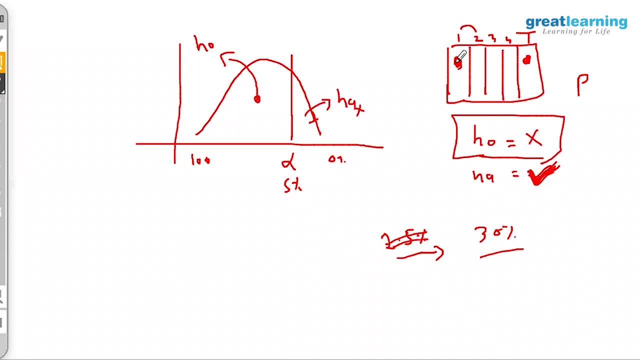 probability or p value. i can find out that variable one number one on t is in acceptable value. i can: Variable number one has no significant impact on target. Remove it from our classification or our linear regression model. When to do this, If we have forgotten to do that initial check. 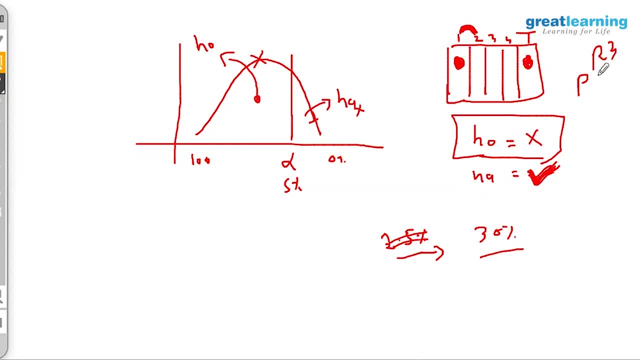 even later on, after implementing it. if you find R square is less, try to catch on that p-value, And if the p-value is more than 5%, remove that variable blindly. Okay, Yeah, I'll show you an implementation on this. 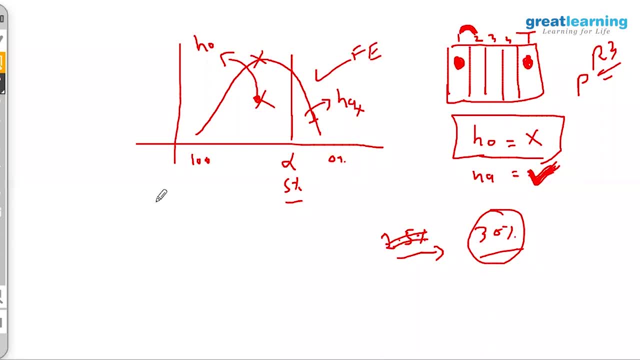 in feature engineering. We will go through this also. Okay, So this is the minute. granularity: you can go on to each and every algorithm. There is a fix for everything. to be very frank, I hope I did not confuse all of you. 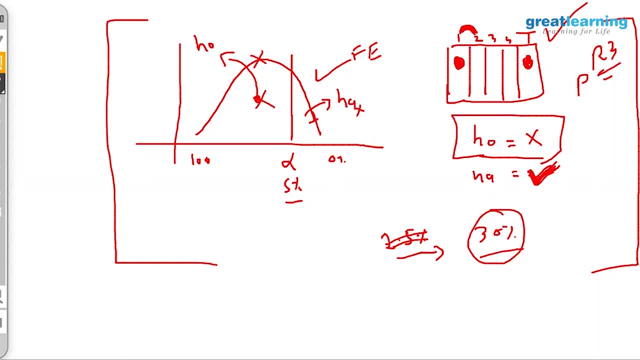 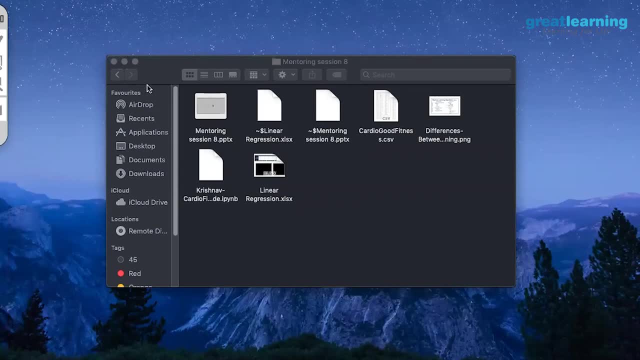 Only thing is my Excel is not working. It will take some time for me to download. I just formatted it. So in feature engineering I will make sure I take all the algorithms like this for you. The guys will come to know how to process. 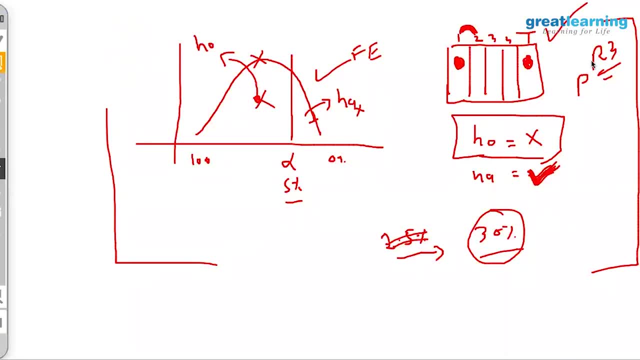 how to play around with an algorithm. Okay, Perfect. So any more questions on to just machine learning, part of it, Only machine learning. No, no, no feature engineering. Yeah, we are kind of clear, And yeah, so I was going. 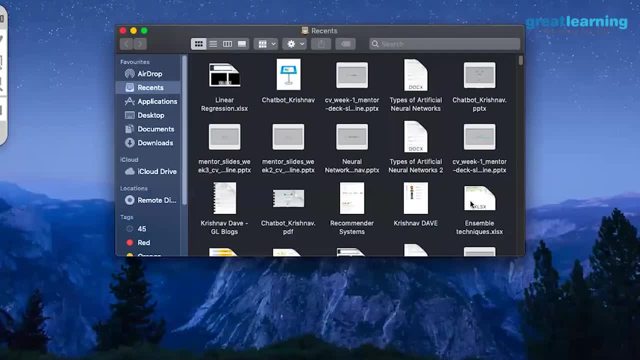 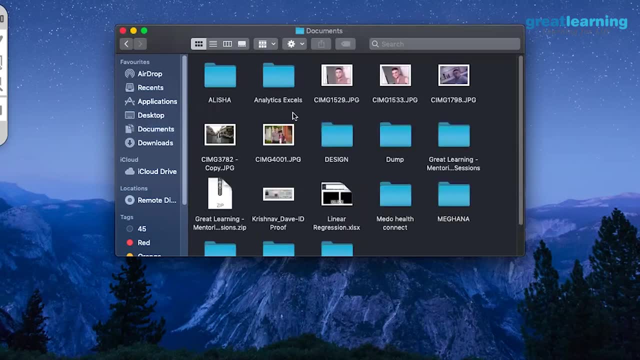 I was trying to show you one data set which I have. You guys can start working on that. Since you people asked me long back know that you wanted some project to be done, I have got my hold on to one of the projects. 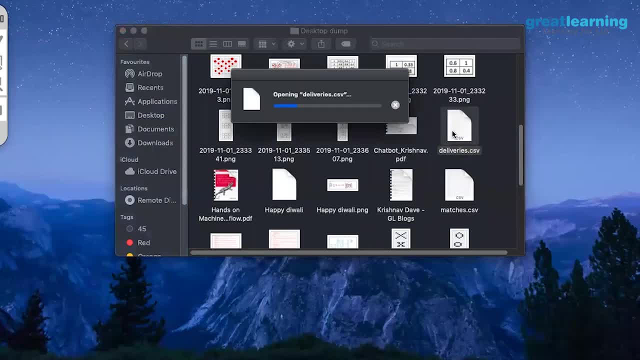 So I'll explain you What it is and then you can take it up. So this is an IPL data set. Again, it will open in CSV. You have opened it Sorry. Well, open something. uh, Python, I have seen some file. 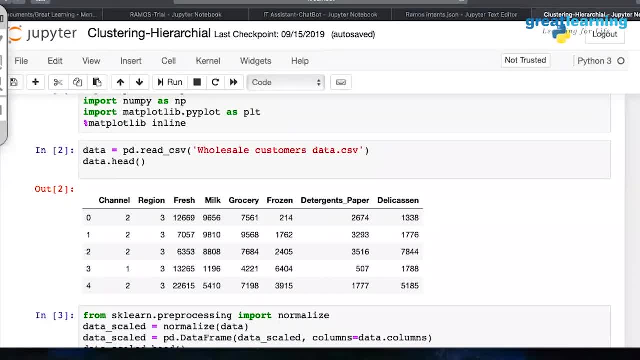 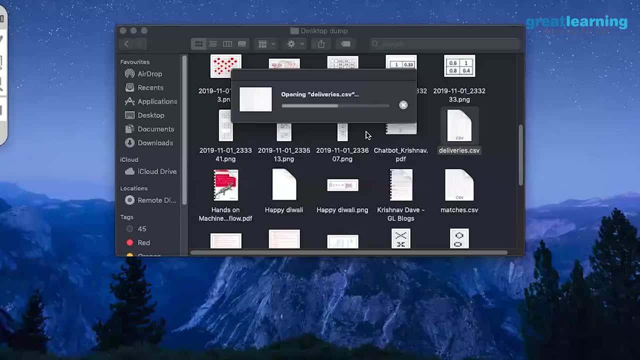 You have opened where this is the one, not this. Yeah, yeah, this is the one you're talking. No, no, no, no, I, I I'll just show you. I'll show you the data set. Okay. 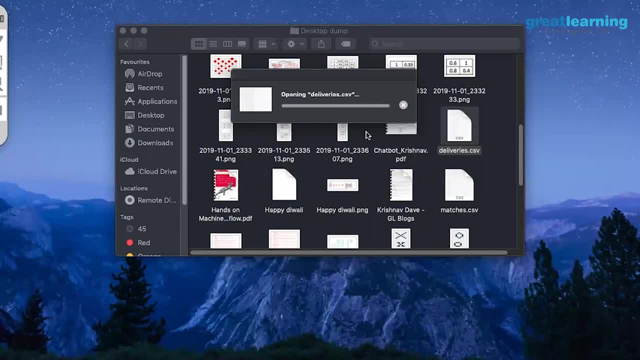 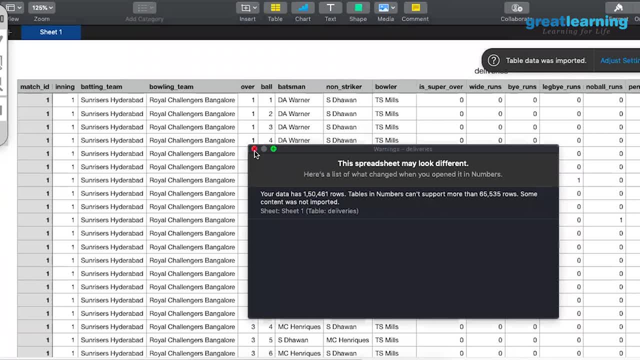 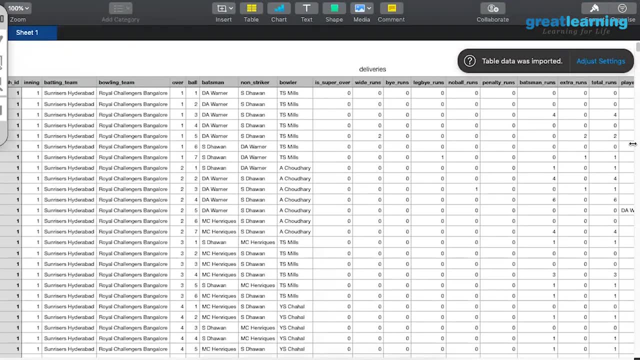 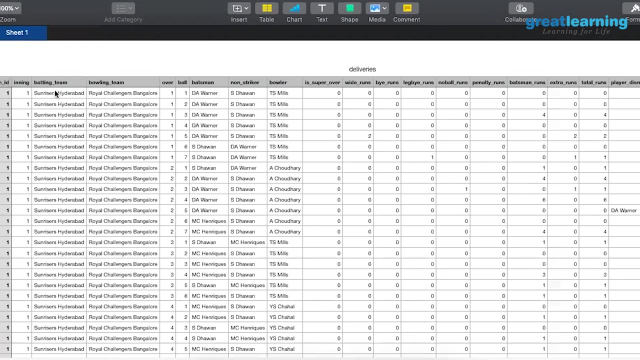 Yeah, If you can see, my screen may look different. Okay, Uh, 100.. Yeah, So this data set basically comes from our IPL website. Okay, Now what is the business problem here is, we have got so many teams, So, if you see, 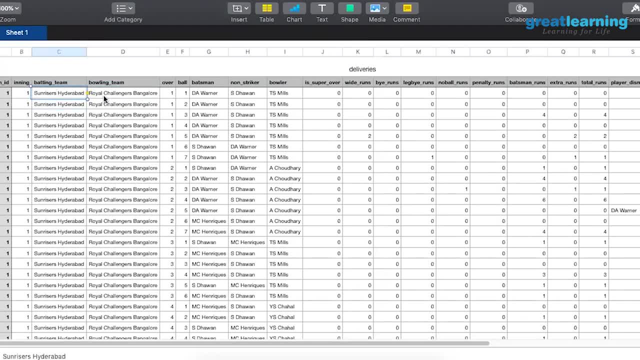 we have got teams, multiple teams, who are playing against other teams. Yeah, Okay, Uh, how many balls they have taken. Who's the batsman? Let us say the batsman is this guy and the non-striker is this. 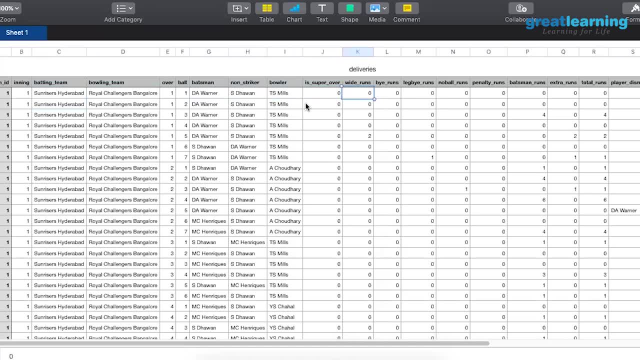 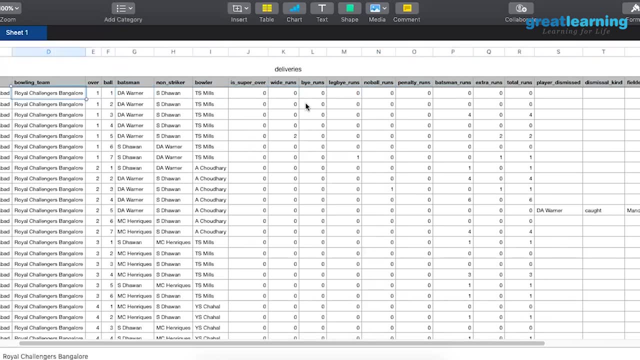 the bowler is this, uh is. is it a super over how many runs they are making? So different variety of runs we have? Yeah, So this is one data set. So what if I want to understand which team is the best team? 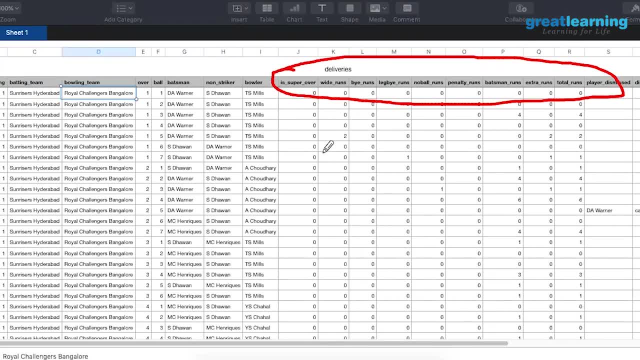 Keeping all of this different type of scores in mind, which is one of the best teams, or rank top three teams? One, one problem. Second one: who is the best batsman? Let us see, We don't know how to calculate. 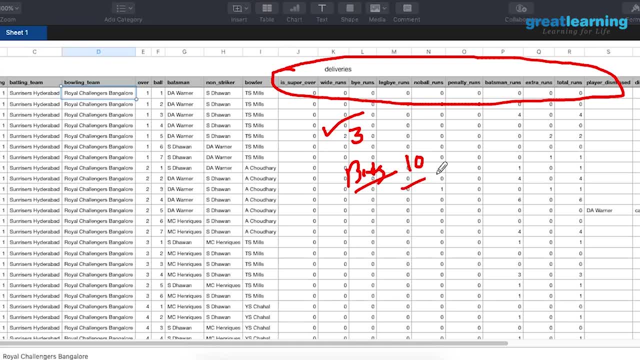 but this is the data set we have. Let's try to find out the top 10 batch men, for example. Yeah, Let us say who, uh, who were the top five bowlers or worst five bowlers? We can say something: who gave a majority of the runs in? 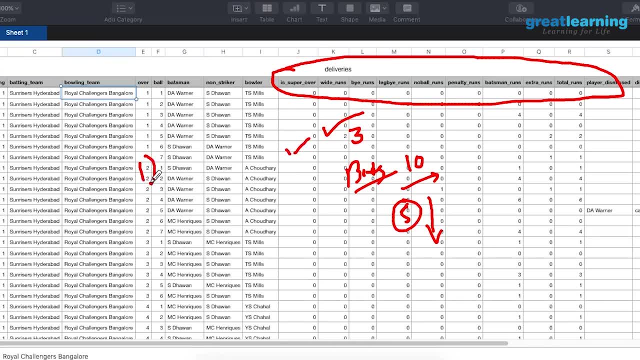 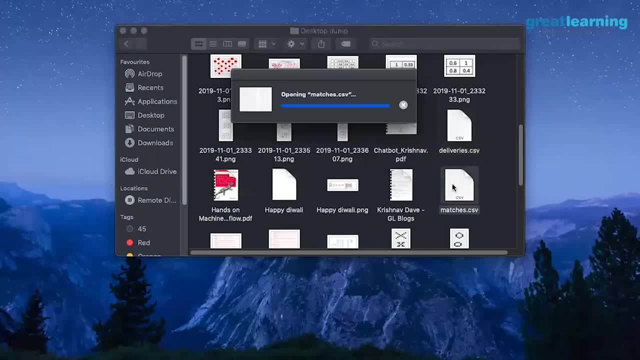 Limited number of balls. This is one data set that I have: batting and bowling data set. There is one more I have is on winning and losing. So the same IPL, which team won the most and which team lost? So if you look at this data set, 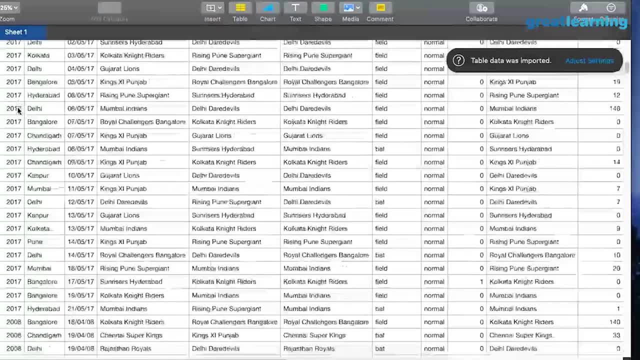 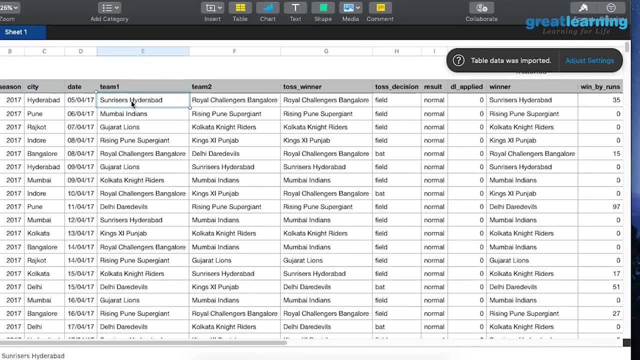 it is covering from, I think, 2008 to 2017, wherein they are saying: in this season, this is the city, this is the date, this is the team. So this is the team. one, team two. they played together, basically opposite to each other. 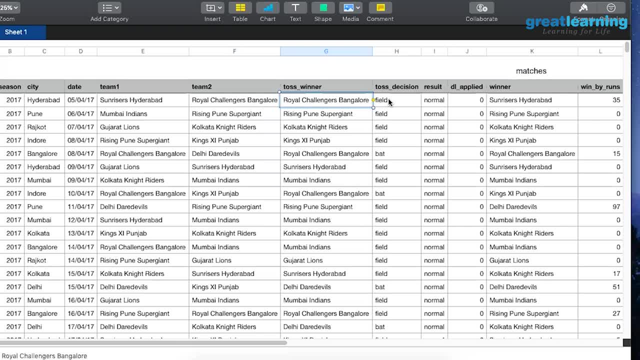 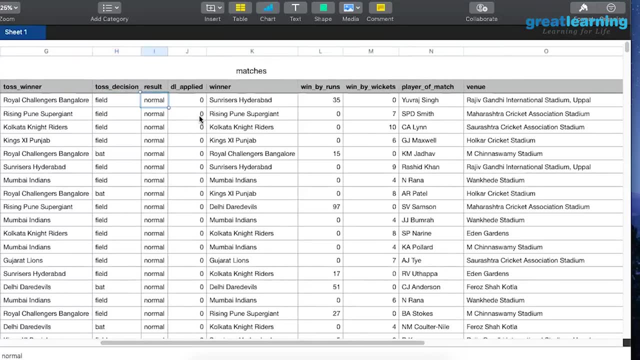 Who won the toss and what did they decide to play? Yeah, Post that there'll be multiple data. What was the result? Okay, Who won? So what's the result? Normal, normal in the sense there was a normal victory, or they had to do some extra hours to get it winning. 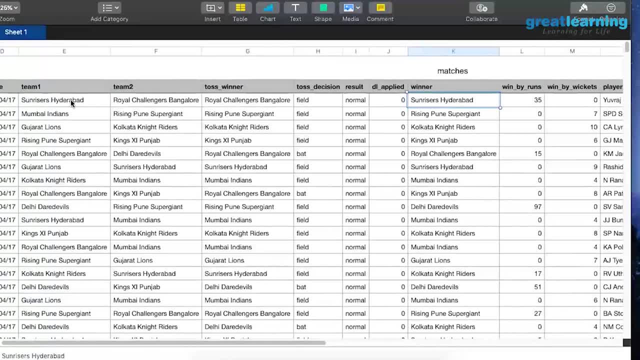 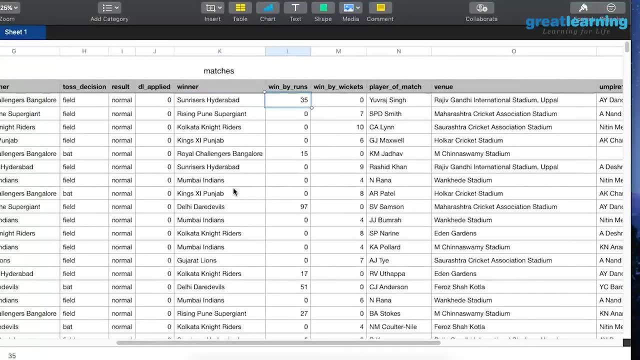 Who won the match. So if you observe here, the person who did not win the toss won the match, something like that: Yeah, Next day one by number: Number of runs, how much, a number of wickets, how much. 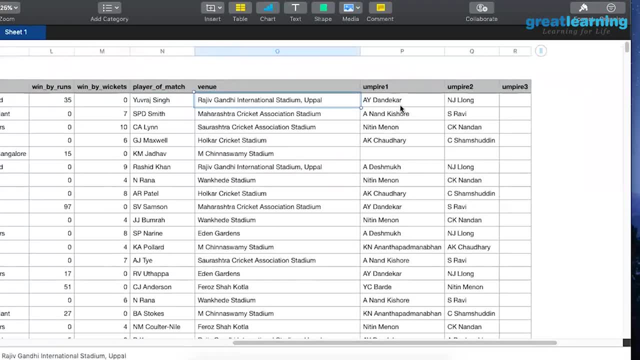 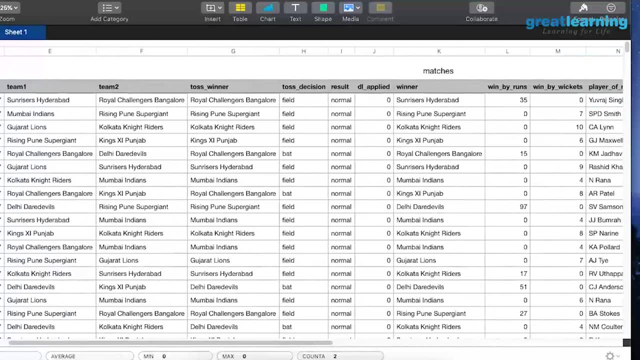 who was the player of the match? What was the venue? Okay, Who was the umpire? I'm trying to siting. This should not make a big difference. So now, what if you are working in a financial advisory company and one investor comes to you with this data set asking you that I want to buy an IPL team? 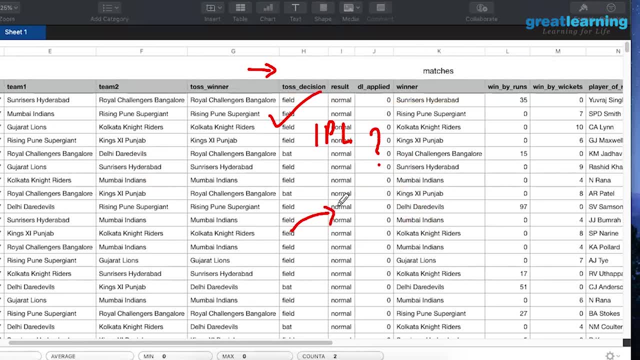 which one should I buy? Or let us say one existing IPL customer team owners: Okay, And he says: I'm having not good players. which players I should choose? Or let us say BCCI itself comes to you asking us that: What do you think is the impact of TOS team location and umpires? 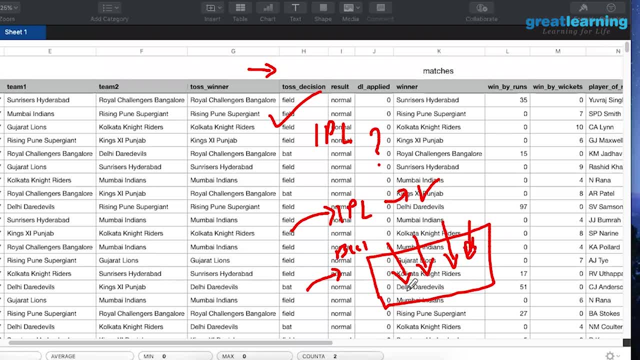 For example, worst case, I don't know, I'm not being sense. Okay, What is the impact of the the month they play, The place where they played and who won the TOS on winning and losing of certain teams? Do we have any patterns onto that? 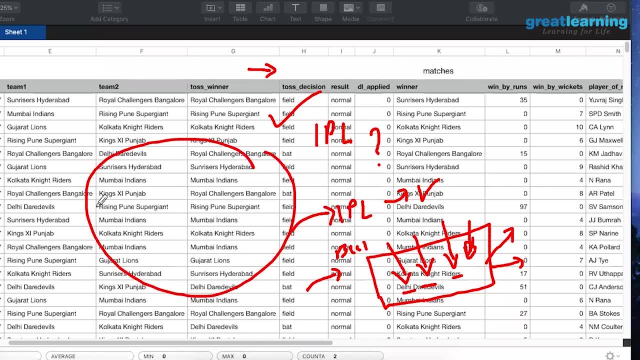 Can you show us some patterns? So this is a very good data set and I can say it's a challenging data sets and industry level stuff, But how we can understand this? Like you know, it's a very good. uh, what do you have? 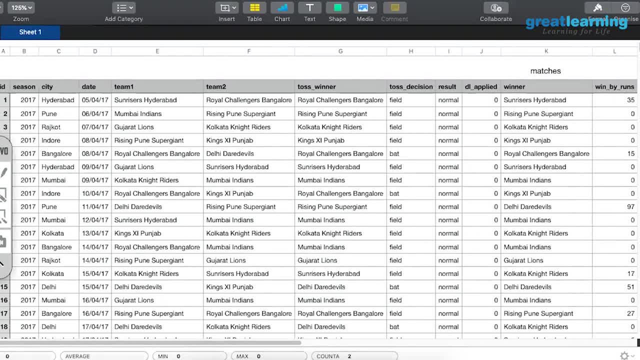 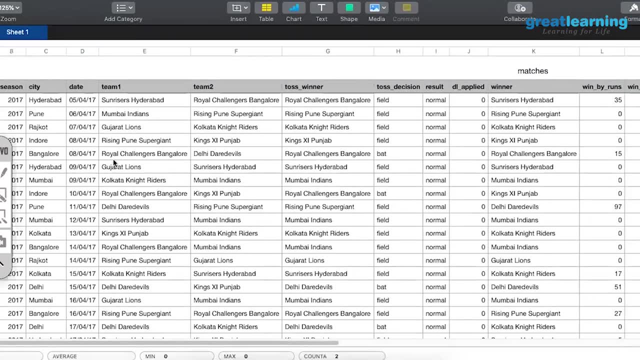 I was like that is more like this step of data sets and where we have to see the uh couple of solutions also before we getting into this solution. Uh, no, I will say you guys are capable enough to do it. Only thing you have to sit. 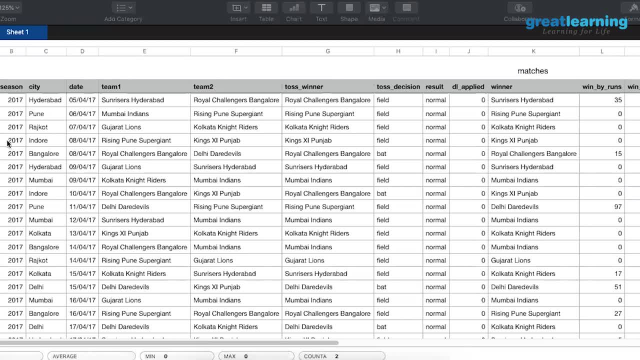 you know, dedicated onto this. Now, how do I, how do we start? Let us say so, what's the objective? What is the objective here is basically, let us say if, to give you a industry experience, this is something extra from my side. 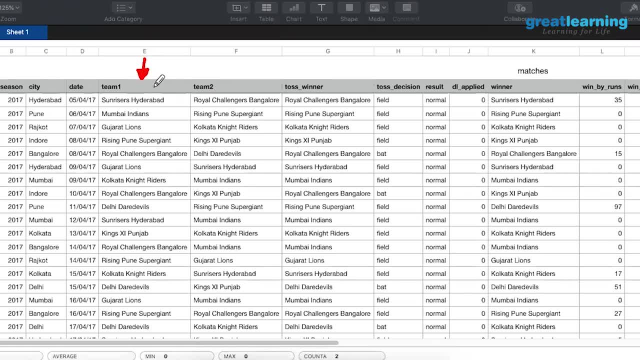 It's not a part of our curriculum anyway. Just to give you a touch of industry data: see the data that we guys give you in in our sessions. No, that is a very good data. You know cute data. We can say it's pretty cute. 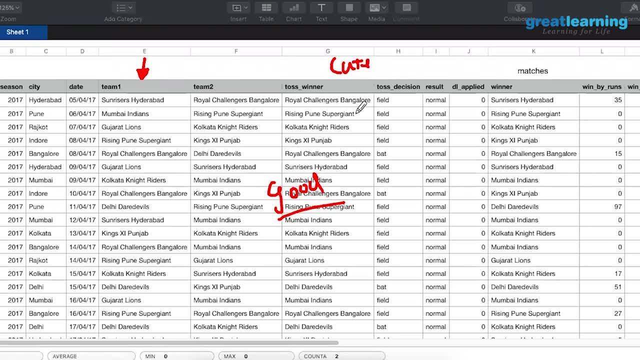 It is straightforward. There is there is no mess up over here. This is what I call a real data, where you have bought n number of columns and number of rows, And each column is very informative. So looking at the data set itself, will be confused where to start with. 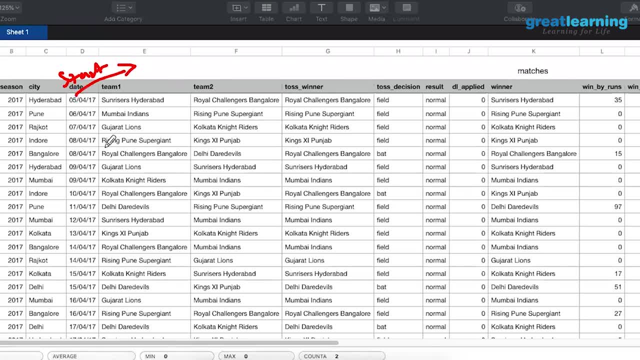 Whenever you have this feeling, no, just understand. you have got hold of a a very good data. This is what is the objective. My objective is to give you guys an exposure. No, no, no, So, no, no. but my question is the objective of this data set. 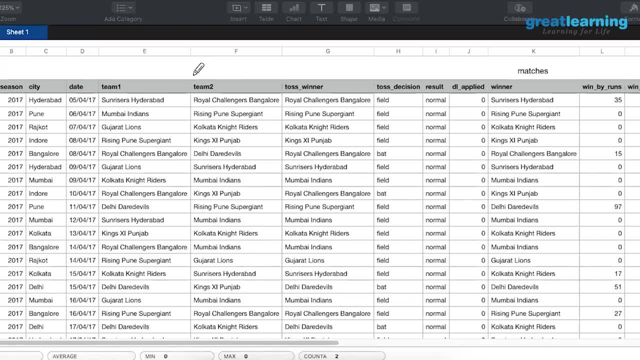 Is it just an EDA or no? let us say I want a machine learning model. So if I, as an investor, if I want to understand class a players, so who come in top class, who which are the players which I can say they are in top class. 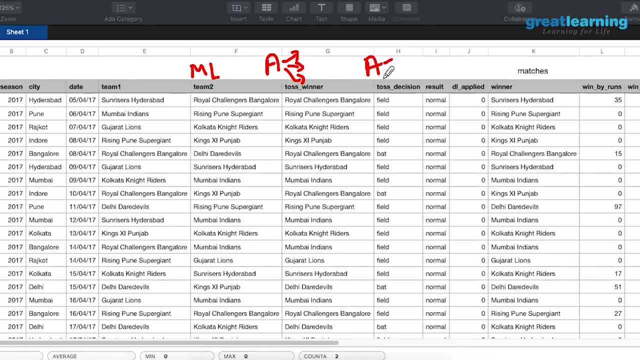 or if, as an investor, I want to say class, I want to say a team. So let us say: out of 10 teams we will divide into four, sorry two. How can equally divide two, two, two, two. 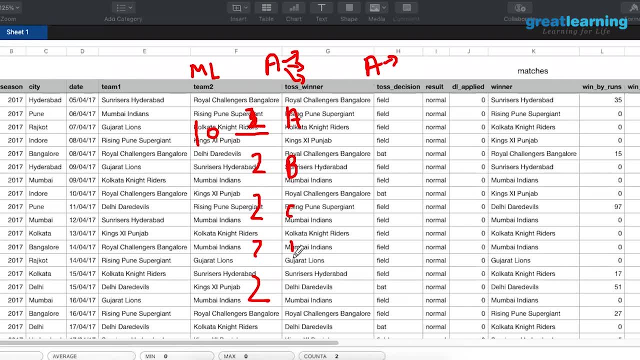 two. This will be top notch teams. This will be B, C, B and E. Let us say, as an investor, let us say: you want to understand which are the top performing teams. Give me the list of, or give me the recommendation of, that. 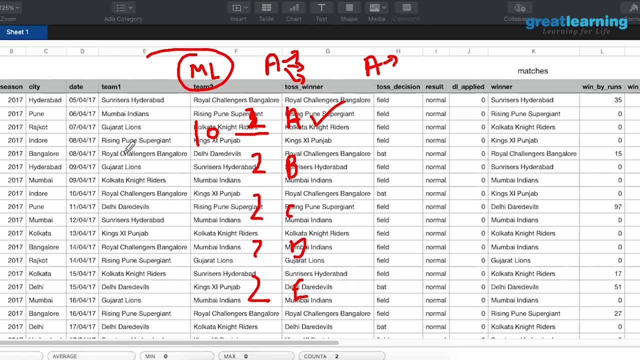 So you can build a recommendation model for the client using machine learning. This is not an EDA. I got your point. EDA will be good here. You can do good number of EDA, but EDA is not going to solve our problem. 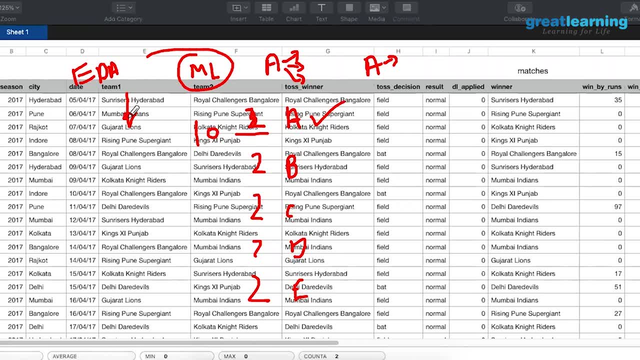 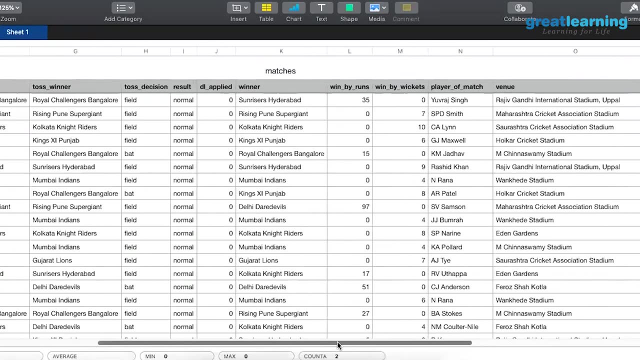 Here. we can use classification algorithm here to find out which is the best team. Or, if you observe here, do we have a target variable here, Like, do you see a target variable here? Are you able to spot it? Okay, Is anybody able to spot target variables? 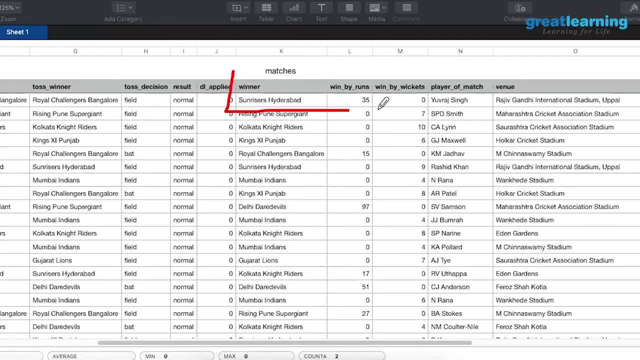 Winner? Exactly These three. I can say one of them can be taken as target variable. Okay, So you can keep this as target. You can put remaining as your independent variable. build a machine learning model onto this. Now you may ask me which machine learning model you guys can suggest me, which one you will use. 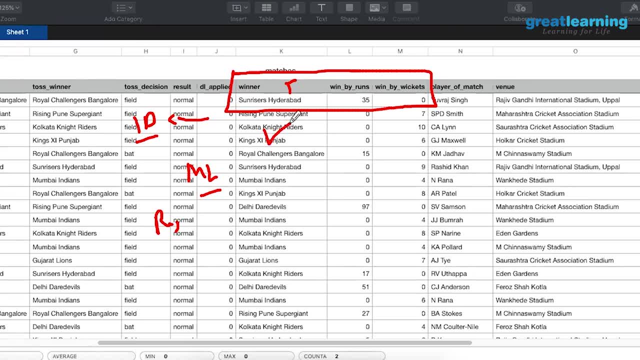 Can we use regression here? Look at the target variable. Let us say, if we are choosing winner as a target, what will you use? It's a category. It's a category Exactly, Classification. you can use Correct. But if we are using one of these, 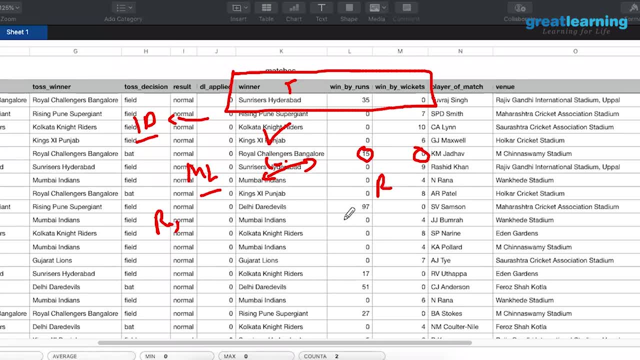 what will I do? I will use regress. as simple as that. So tomorrow, let us say: if the investor tells you that if my location is Hyderabad, if my team one is Royal challengers and team two is Mumbai Indian, and if we are choosing to back, 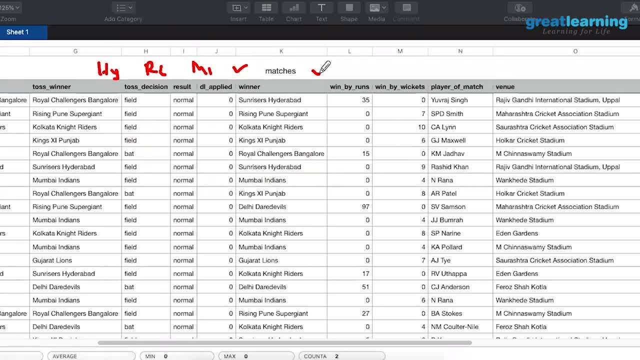 first. if we are winning the toss and choosing to back first, by how many runs will win Linear regression? Yeah, Yeah, By how many wickets will win Linear regression? But if we ask you whether we'll win or not, 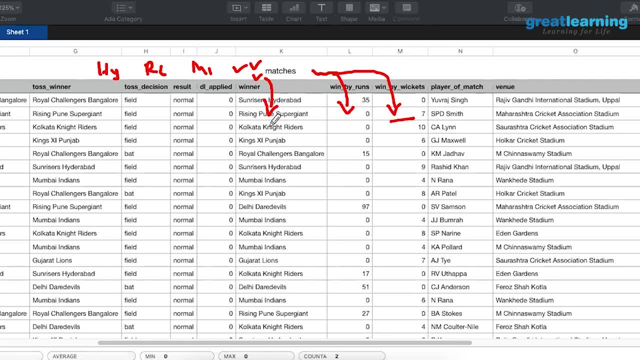 in that case you can say: it is a classification problem, That's it, That's it, That's all you're supposed to do. But it's not as simple. So again, you guys will struggle a little. The only good thing. 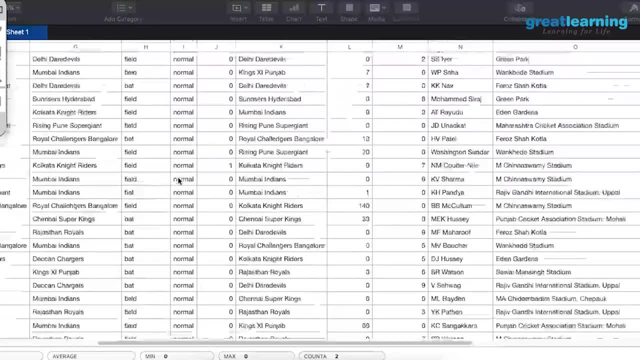 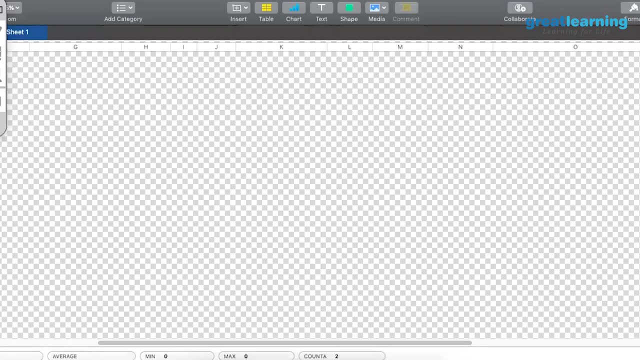 the data is clean, First of all. that's the best part I like: the data is pretty clean and the data is as big as industry standard. So, if you remember, there are some big PR companies working on sports analytics and all. So this is. 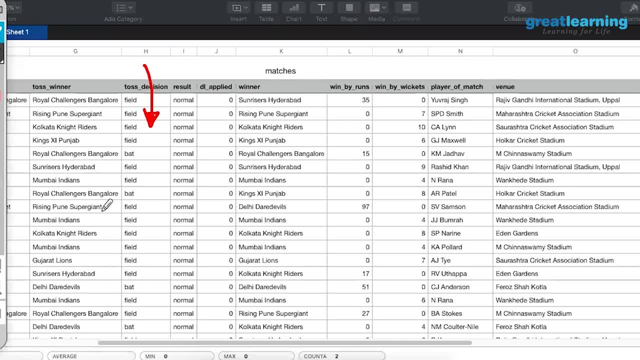 you can say you're getting a live experience on to that. Yeah, You want to do it. I will share it with all of you. Yes, yes, yes, That would be nice. So, Krishna, just curiosity on the on the topic of cricket. 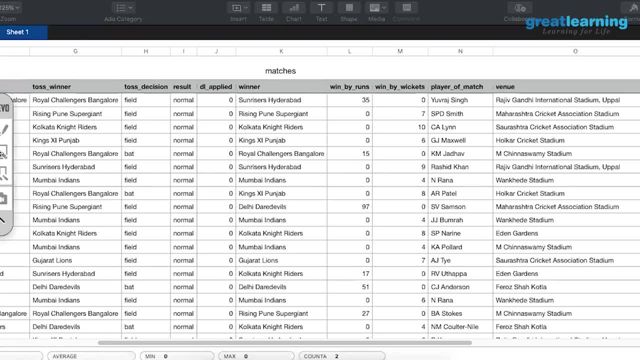 right. So you mentioned the score predictors. For example, if you've seen when India bats second and we don't call it scores 35 or above India. So how do you do this? complex predictions- What kind of Okay. So again, 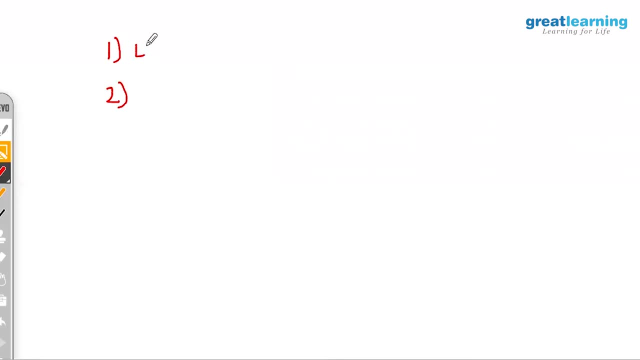 depending on what type of data it is. but let us say the data is linear in nature, linear in the sense. What if A number of matches played by Virat Kohli, let us say, and number of runs made by Virat Kohli? 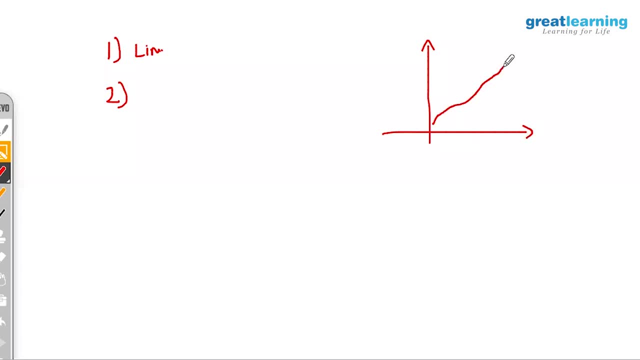 In that case i will say it will be a linear relationship. yeah, but let us say, if we say number of matches royal challengers played and number of matches virat kohli played, for example, it might not be linear because sometimes he might not be in the team. so we'll we'll. we'll see some dips ups and 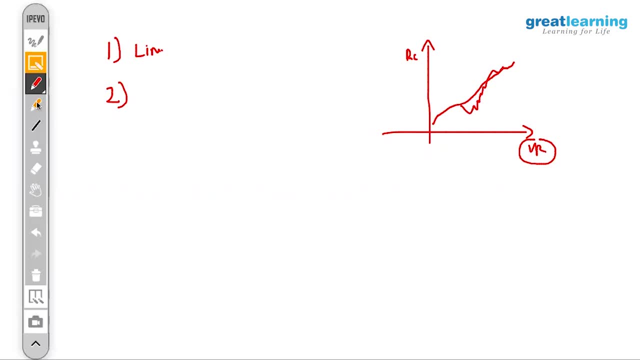 down now from your question. how will we predict that? so, again, that that's a very difficult thing. so what are we supposed to do? is for that question is, first of all, we are supposed to get all the regressor independent variables ready. now, what all independent variables we can get over here? 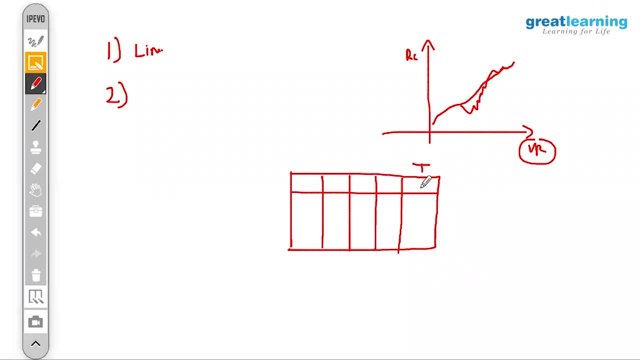 yeah, the target variable will be what number of run correct. now what we can do is which team he's playing. for first question, yeah, which place he's playing, which year or which time of the year he's playing, number of balls he played and let us say, if you want to make it a little more complex, what. 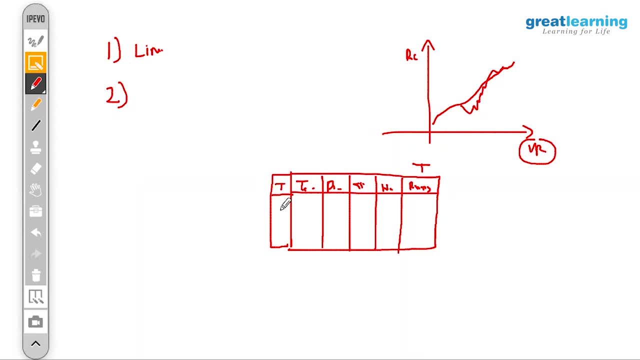 was the toss decision to field first or back. so if you observe, this is categorical, categorical, categorical, categorical and numeric. did you people observe that? yeah correct, all are categorical. yet we are doing regression. why? because the target is regressor. now, how will we do it? one hot encoding: 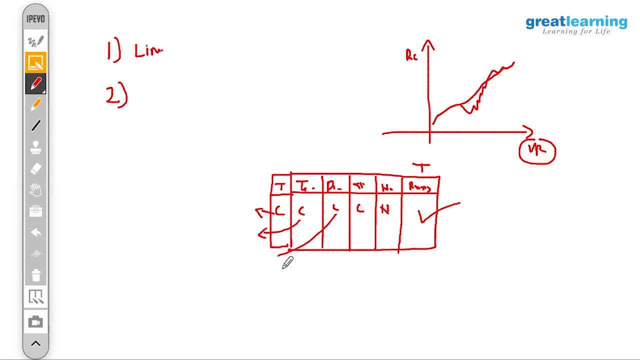 label encoder. you can use any of these techniques that we have done so far to convert categories into numbers and then try pushing linear regression. first, because as per me, it will be linear data. try to push, push regression and, once you push regression, measure our square. our square value should be around seventy percent and above. if you get this accuracy, then you have 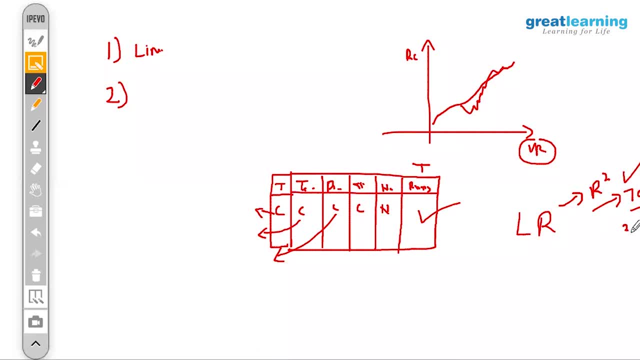 nailed it, probably if in case, we are getting thirty percent, forty percent in all, but it means that it's not a linear relationship. in that case you can go with quadratic regression or polynomial regression, where you will be designing your own equations. i know we have not shown you. 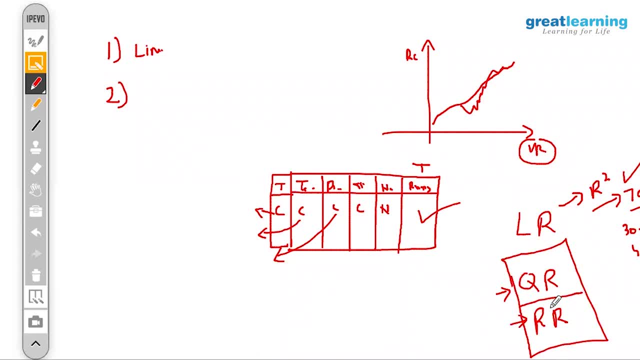 this. if you want it, i will show you this in future. what is qr and what is pr? okay, i think they covered something about this in svm. if that's not what you're talking about, yeah, quadratic to just to just show how higher dimensions uh can help in um identifying a. 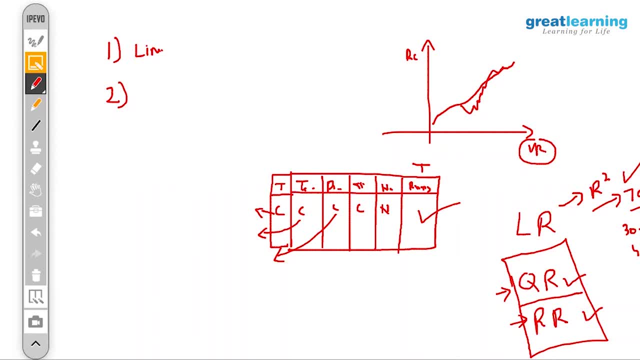 plane to separate. okay, correct, might be. yeah, okay, so this is how you can push or you can start with the regression now. if you want to show how you can start with the regression, okay. so this is how you can push or you can start with the regression now if you want to show. 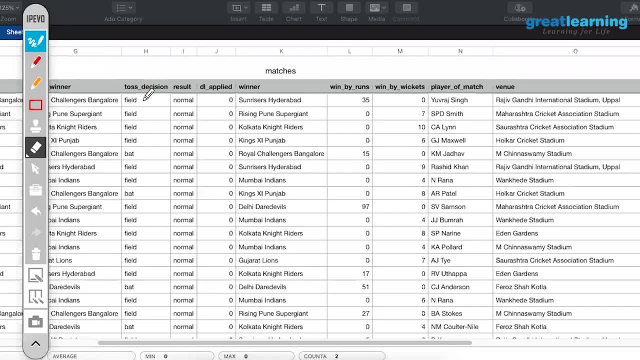 again, i will say: it will be not, it will not be a piece of cake. why? because it's a difficult data. as per me, as per my standards, i will say: even for me it's a little difficult data. yeah, so you can try classification, you can try a regression or, if you do not want, target variables. 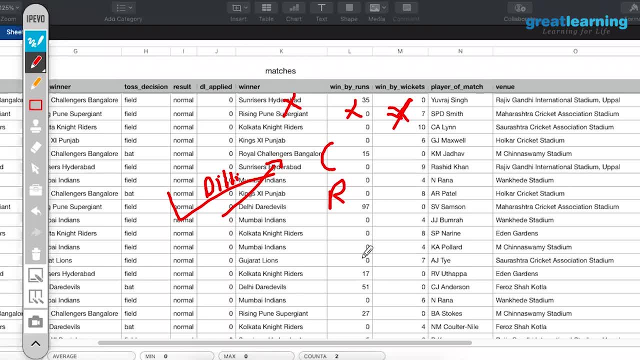 if you do not want this, you can do unsupervised learning also. yeah, now have i shown you guys my pca implementation onto employee ranks. have i shown you that? yes, yeah, so why can't we do the same thing for players over here? where are our players? where is not this data set? let us say we're talking about that other data set. where is? 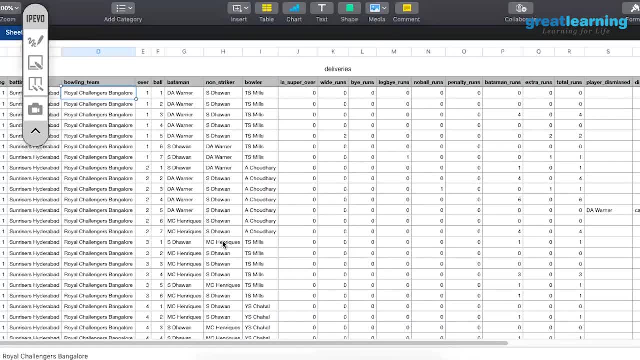 that. yeah, if you remember this data set where each and every player is having its own runs scored, something like that, right so that employee ranks. what was it having? it was having the name of an employee and it was having some attributes attached to it. agreed, and what we did? what was our target variable? 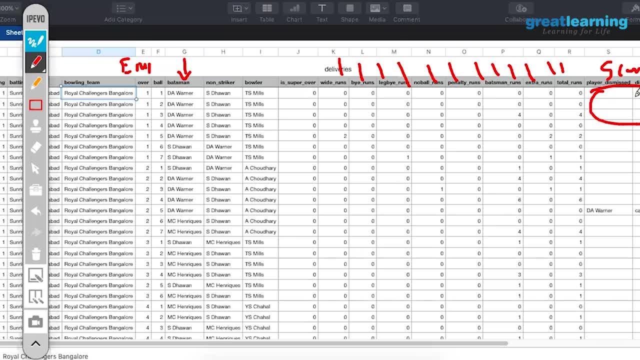 what did we give them? that's cool. performance rating, yeah, exactly so. instead of performance rating, you can use the same code that i've given to you guys to rank an employee. i'm sorry, to rank the ipl player. i'm giving you the hint over here. 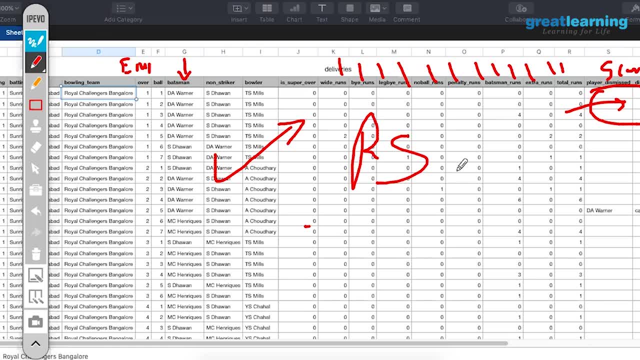 so this is the way you can build a recommendation system. this is nothing but a recommender system. if a client comes to you and says, let us say you have given the scores here. now let us say in the scores: so you used my pca code and you have given some scores, now we will. 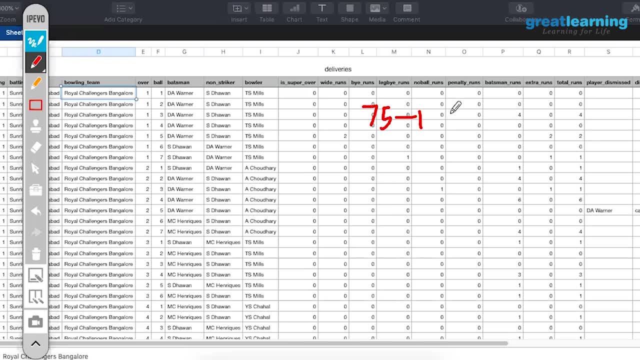 say, anybody who is from 75 to 100 score will call them class a player, anybody from 50 to 75 will call them class b and anybody less than 50, let us say we will call them a class a player. let us say we will call them as secret player. so what you have to do is you have to make a simple 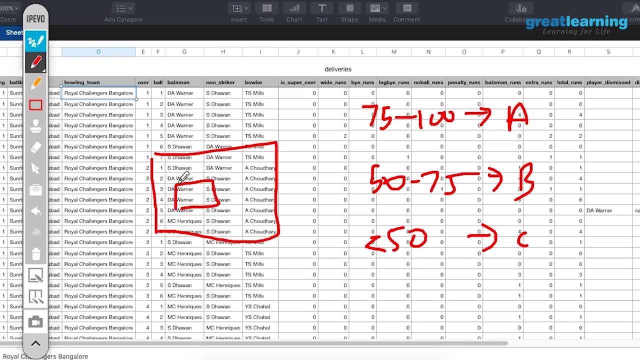 api for the client. the client has to give his requirements. the requirements will be: let us say he is a batsman, okay, and i want a class, a player, and how many? how many i want. let us say he wants five players of. so what you have to do, you have to push this data inside your code. if he says class, 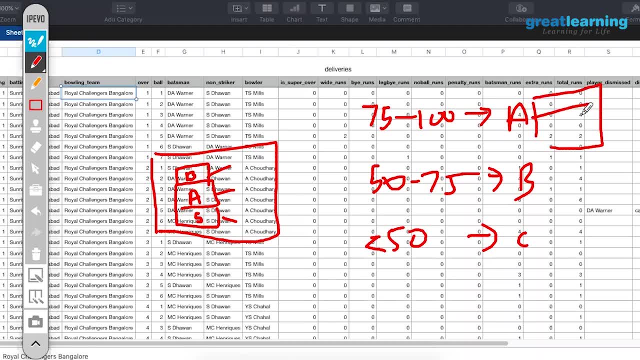 a. you will already have a list of class a players. give the top three players a class of a player and give the top three class A players over here. very simple, this is your recommendation system model and this is what the sports analytics companies do. yeah, okay, cool, awesome. so yeah, one. 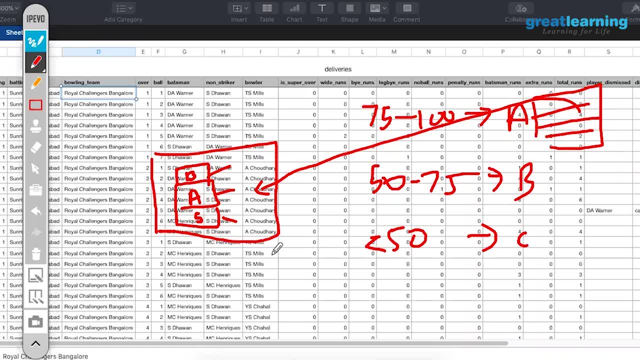 question is: see now all these data that we get. it's all like a, like a single table, single rows and columns. what if we have a relational model where we have multiple joins and you know it's a data model, real data model, how do you go about that? 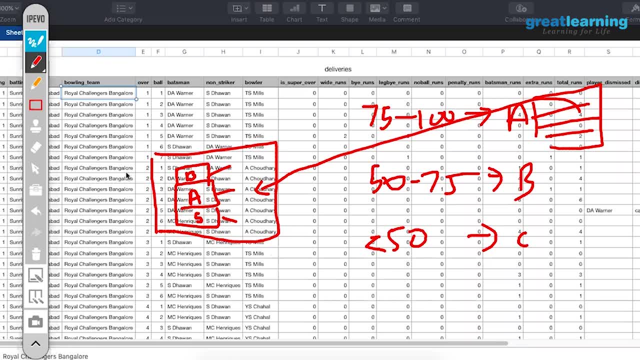 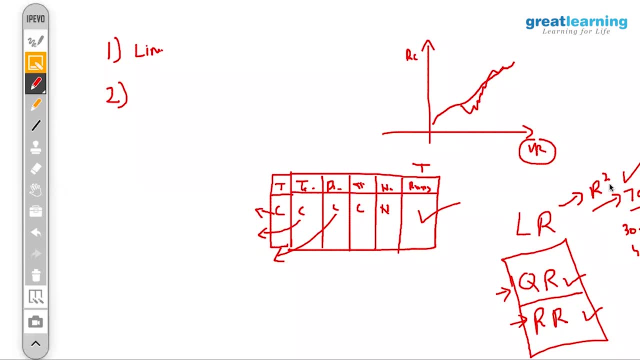 okay, so in that case, again, the knowledge of SQL will be the must. I think that's what we are talking about, right, joining the data sets and all that. yeah, there are multiple tables and foreign key, primary key, master table. so in that case, what I usually do is I sometimes play around with 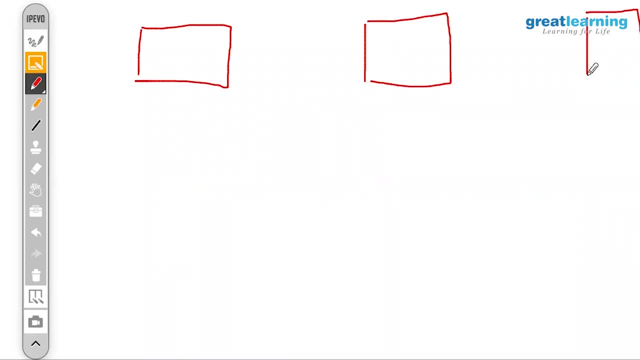 this data from multiple servers. now what is happening is luckily for me. please remember one thing: a relational data set will have some unique IDs as a relation. I hope everybody agrees with me that right. so unless and until this is present, we call it as a relational database. that's it. 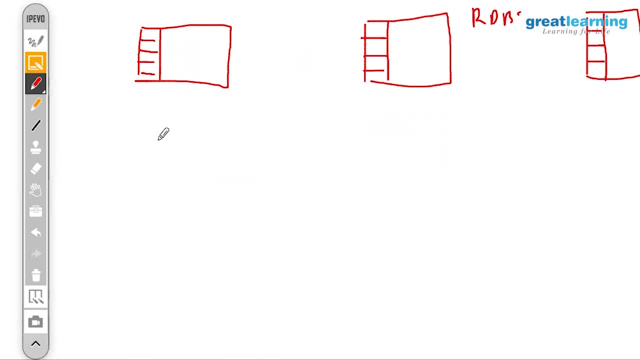 my SQL part will come. yeah, so what is our job is to very simple is: have I shown you our SQL implementation anytime? I have not shown you live connection with SQL, right? okay, I have a data set which I actually I have shown this for my other batches. 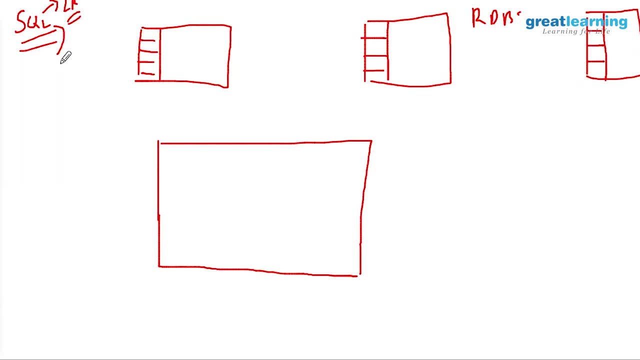 in linear regression implementation with a very old implementation. you know, I mean, we just started machine, but no problem, I'll show you guys again. so what do we do is inside Python. we have got my SQL connections. so what we can do is we can fire up our Python with my SQL. 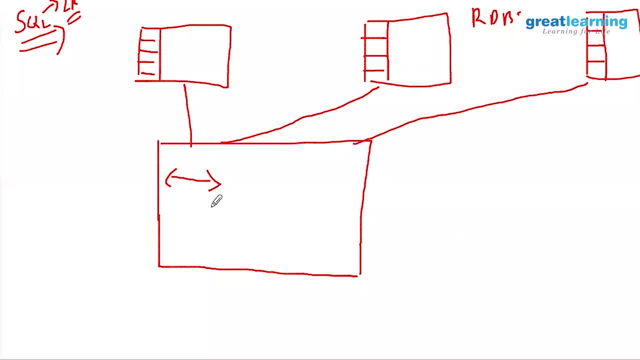 very simple. okay. next, what we can do is we can either query here itself. if, in case, you want to remove something else, we can do a querying here. now, once we do a querying here, what are we supposed to do is, let us say, I imported this data set. I will. 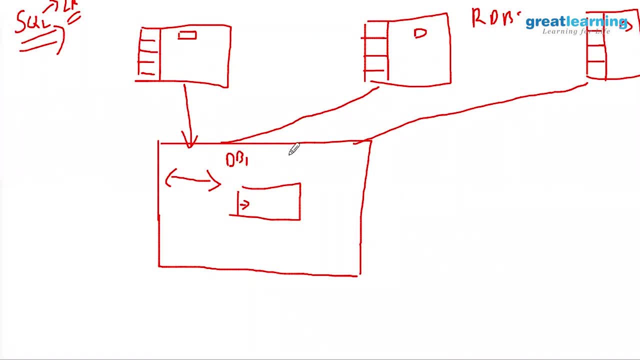 call it pandas, data set one. I will call this pandas, data set two. I will call this pandas, data set three. agreed, everybody. I'll show you how do we call and how do we input a note, but it's very simple: the way we read an excel file. 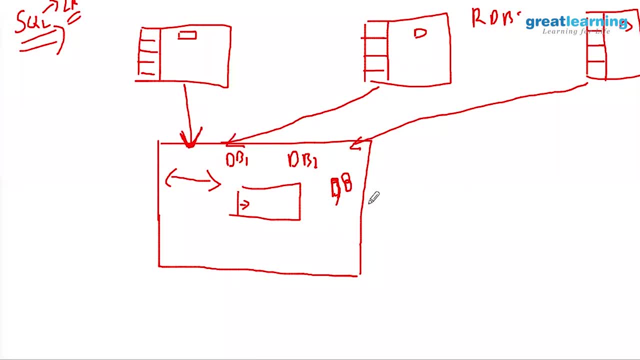 similar to that. we can read our SQL stuff. so now I have got three panda data frames. now how do you think we'll join them? what does this data frame have? yeah, it hasn't ready. could do one kill sir sequel, select, start from. you can do exactly. so this is the way you have to. 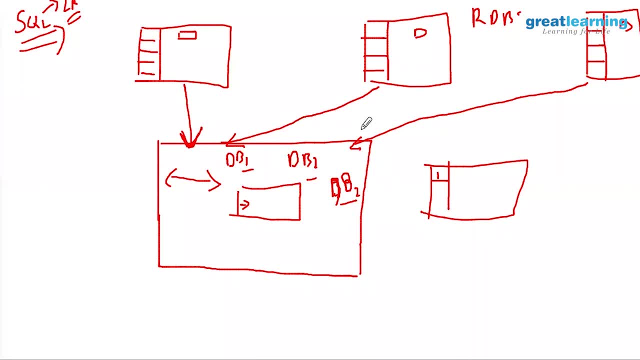 do it. yeah, now, I'll agree with you, it's a pain taking task. actually, this is a very painful task. why? because not all of data is in sequence, the ids, yeah. so we are supposed to find out the matches and then we are supposed to join them. okay, i will show you an sql implementation. definitely it will. it will get. 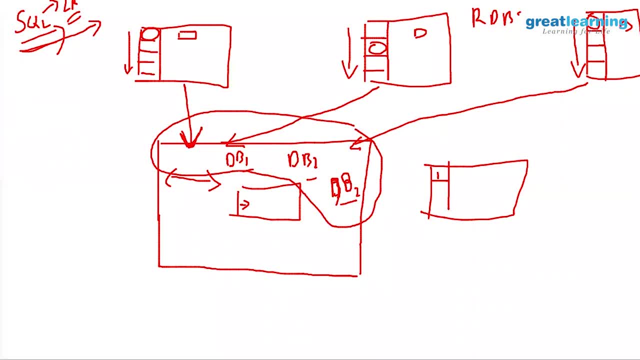 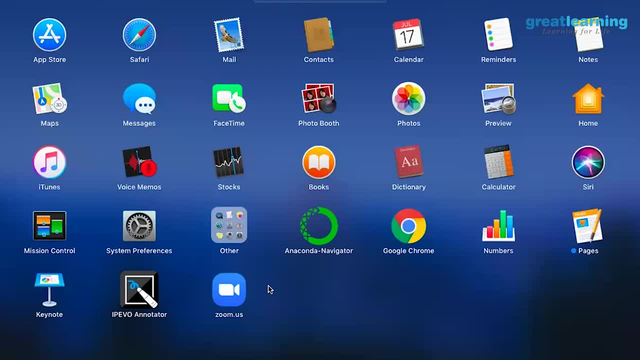 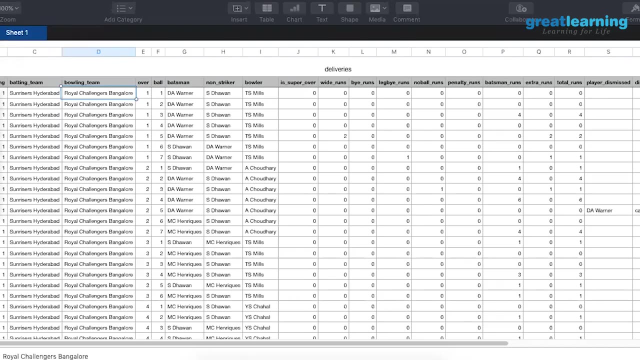 you going: yeah, so the only problem is, since i reinstalled my mac os, my my sql server is not installed on this, so i have to just fire it up. okay, so i will show you guys this thing once my mac, once my sql server is ready. but yes, you can definitely do it. if you want me to do it, i will. 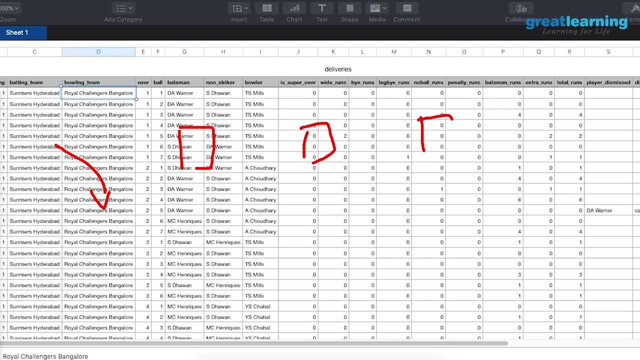 definitely show you multiple joints. no, i mean see if you can do a multiple join and get a whatever result set and then use that result set as this excel. that's okay but correct. but is that the only way to do it? or because if it's a large data, right, and then having so much of data? 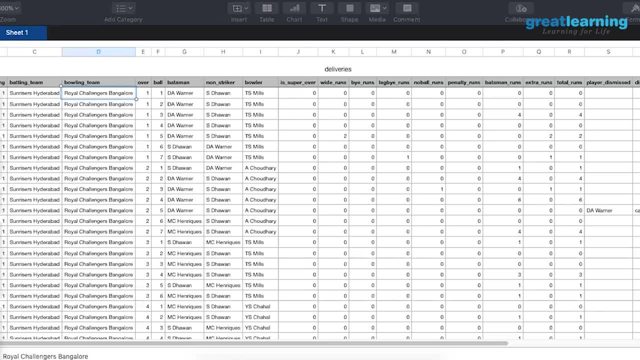 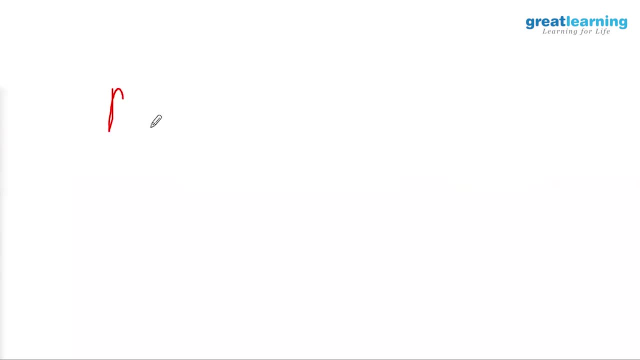 uh, in memory i don't know how that performs. in that case we bring in two new concepts. so one is internal python concept called parallel processing. so what we do is our one of like. let us say, if we see, currently this parallel processing works on gpu, if you guys have, 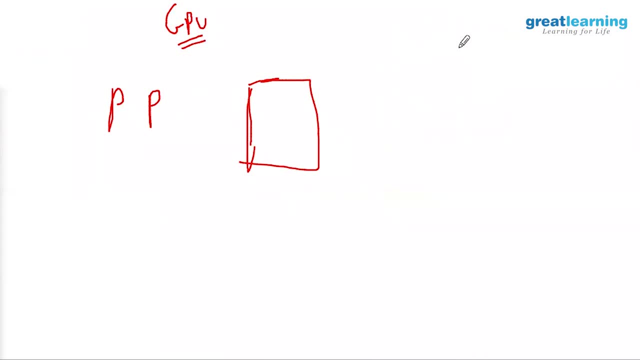 heard about gpu. right, right, yeah. or else even in our normal cpus, like i have i5, we have one port which will be little empty. so usually this port is kept empty. so in this case we can know the size of the port and we can do a parallel processing here if in case, we don't want to. 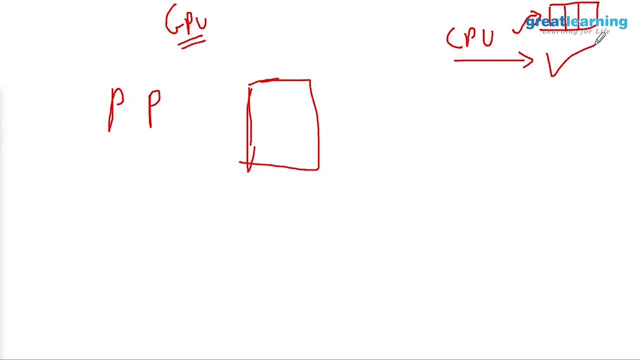 go very complex. i have an implementation on this too. i will show you guys someday. yeah, else we can bring in the concept of hadoop here we can connect our hadoop parallel processing map reduce system with our python to process our data parallelly and call whenever a chunk of data, as as, got into pipeline of hadoop at that point of. 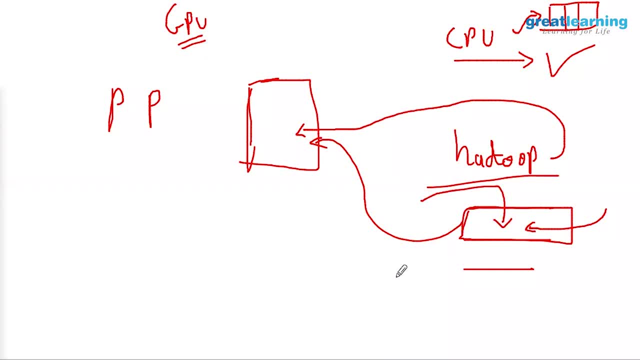 time we'll invoke our python function, get the ml done and throw the output even. we can do this also, but for that we need to, you know, go and understand the hadoop structure and all that. so usually companies like walmart, uber, ola when they do this kind of machine learning thing. 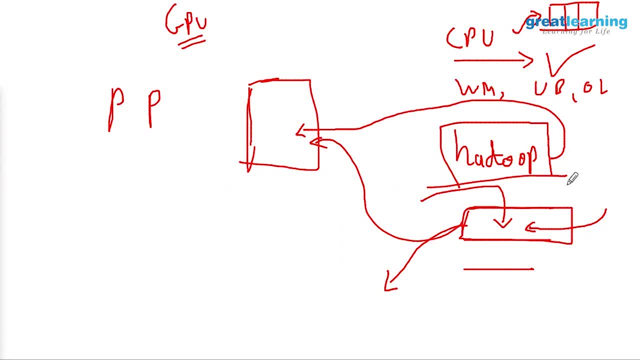 the input is not via simple python. the input comes via hadoop because of the computation power, or else i will say in my org: what we do is we fire up multiple vms together, worst case. i know it's an old school method, but still it works. it's not as sophisticated as hadoop. 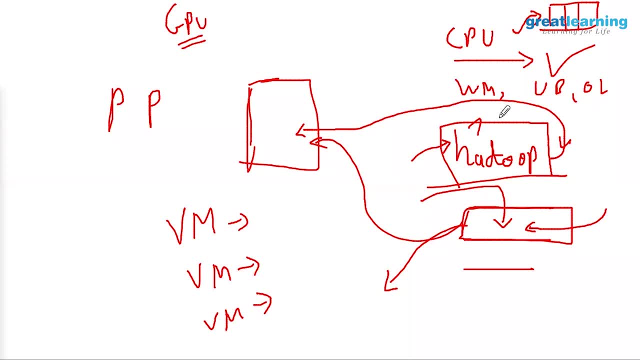 right now again, hadoop is nothing but vm itself. if you guys have worked on it or if you have seen some of the hadoop implementations, it completely works on virtual machine because none of these computers have that capacity, you know, to perform, or the hardware in that way. 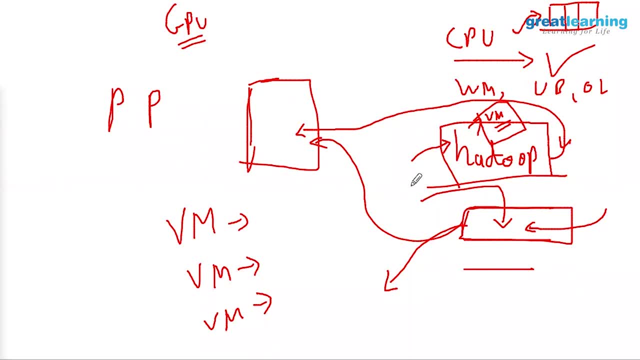 okay, i hope i answered your question how we can parallelize the data. yeah, yeah, because, see, see, ml is all about having more data, right? so, um, so it's important that we we look at how we can run these models on on complex or large data, etc. having five thousand, six thousand, this is good, so yeah, 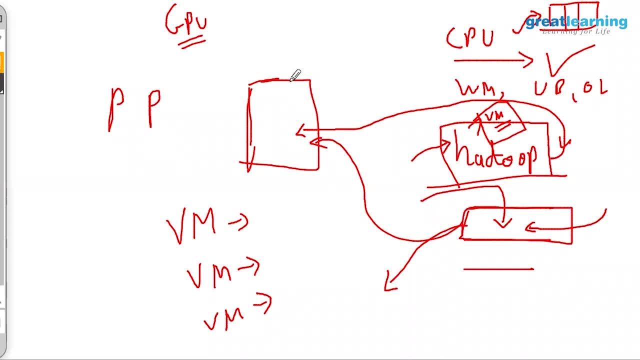 exactly. yes, in this case, my recommendation will be, once you finish this certification, you can get trained on hadoop also- not hadoop admin part of it, but hadoop developer part of it, so that will be an extra advantage. that you can get trained on hadoop also, but hadoop developer part of it, so that will be an extra advantage that 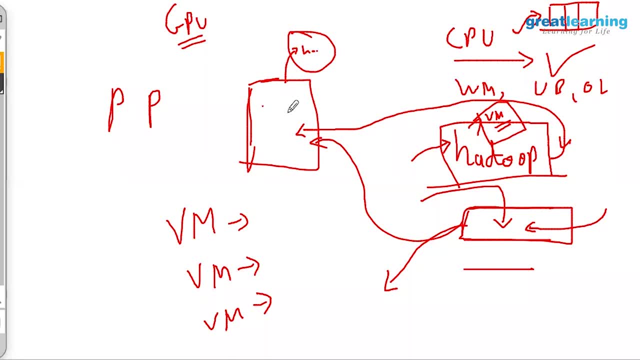 tomorrow, if a company has a huge data set and still they want to stick with ml and go ahead. they don't want to use map reduce. if you remember, if you know what is map reducing, yeah, yeah, you don't want to do that. if you want to use pure ml, then this skill will give you an extra advantage. 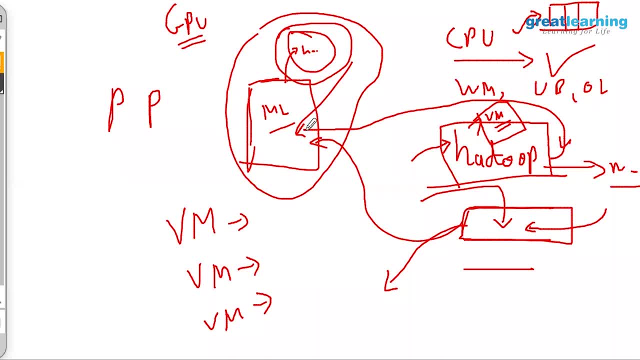 on it because you will be able to parallel process or basically reduce the processing time of your machine learning. okay, you can just spark to very similar to what we load the data. we could use park. so too, yes, i can use park. yes, so each uh, each uh tool that we have in real world- no hadoop has its. 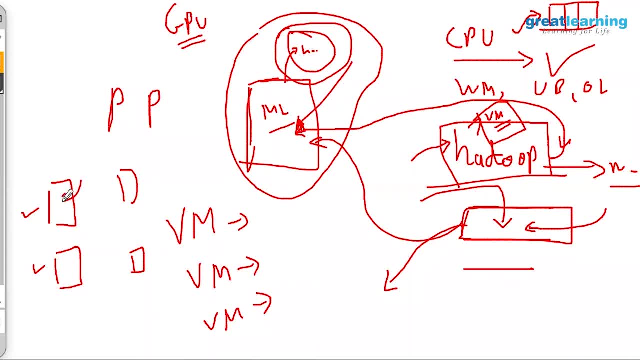 own version in itself, like: uh, if you, if you're talking about mysql, hadoop has park onto that and pig hive lot of tools it has. so if you talk about no mongodb, if you've heard about it, yeah, hadoop has its own version of uh, non-relational data from database. 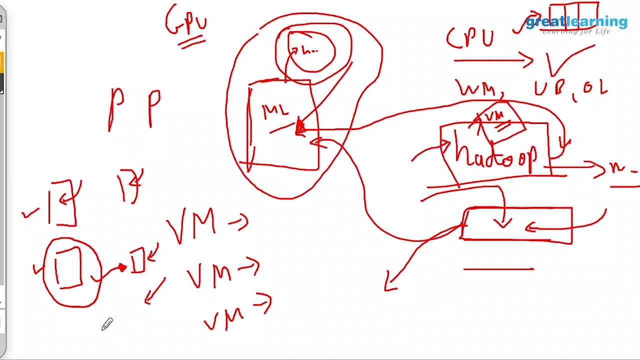 no rdbms, okay, so it's again a very big topic. and still people: there are very less people in the market who know both the technologies to be very fun. either you will find a lone data scientist or you will find a hadoop developer on admin, but together it is, i feel it's a little. 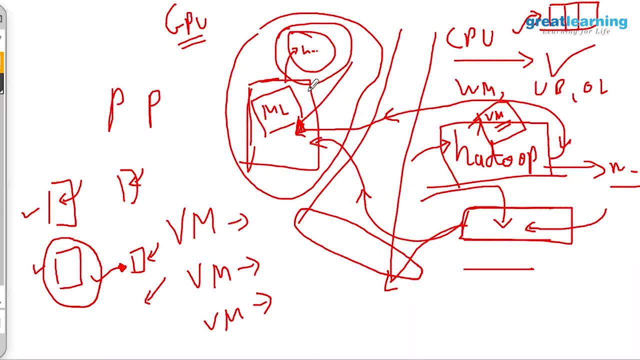 difficult. why? because to expertise, this itself takes three to four years on industry and this one again four to five years on industry. so right now there are no people who who might say they have around 10 or 15 years of experience combined on these two. okay, but i think you can. 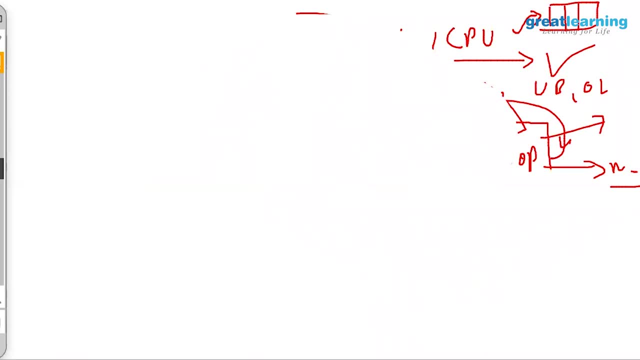 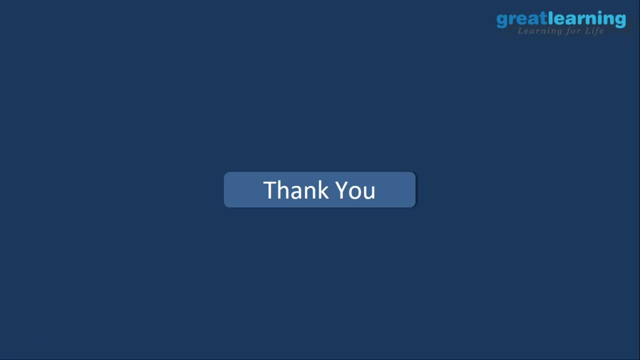 start this, this course, once you finish your ml aiml certification. this brings us to the end of this tutorial on clustering and data mining. now let's have a quick recap. we started off by learning about ml in brief, then we learned about k-means, we followed it up by pca and finally we